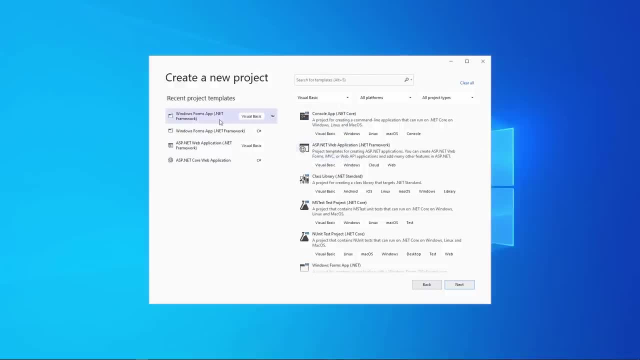 On the right-hand side, I can see a number of different languages. You can see that I've installed a number of different project templates which I can choose from, And I'm going to create a Windows Forms app. So, with the correct option chosen, click Next. 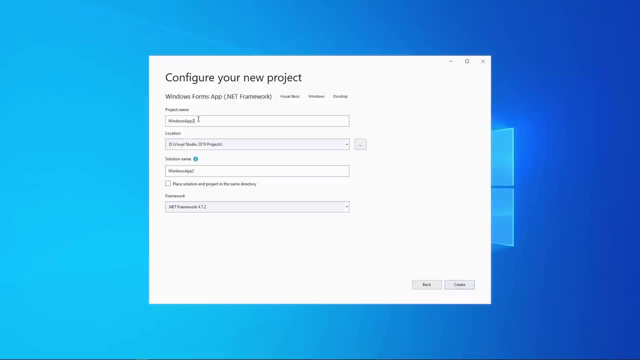 You're now invited to give the project a name. It's offering me the name Windows App 2.. This is because it's the second application which I've created. It's not a very meaningful name, So I'm going to change that. 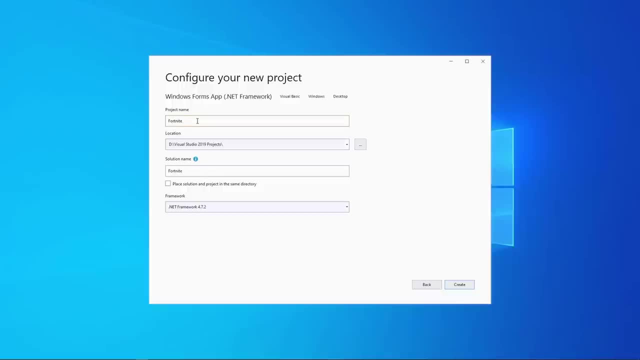 Perhaps, perhaps not. I think that's been done before. That'll do for now. You also need to be mindful of where the project will be saved, the location of your project. You can see the location of mine will be D Visual Studio 2019 Projects. 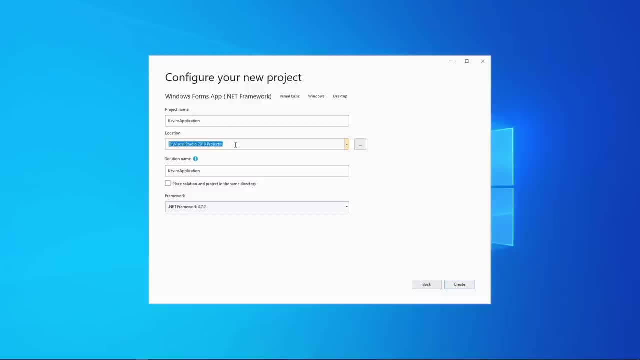 But you can change this. In fact, I'll show you later that once you're in Visual Studio, you can change the default location. This is particularly important If you're working in a school or a college or an organization. it may be that you only 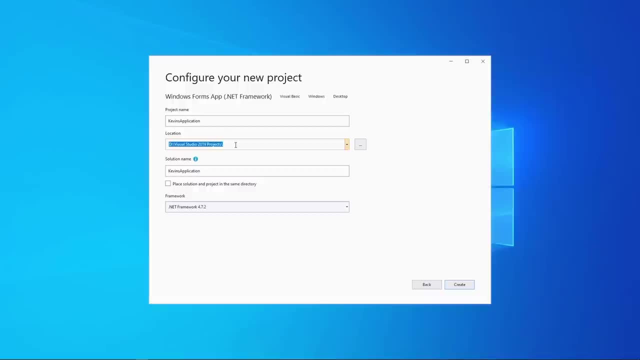 have permission to save Visual Studio projects in particular locations. Notice there's a Browse button here if you do want to change the location. My solution has the same name as the project. I'll say a little bit about the difference between a solution and a project in a moment. 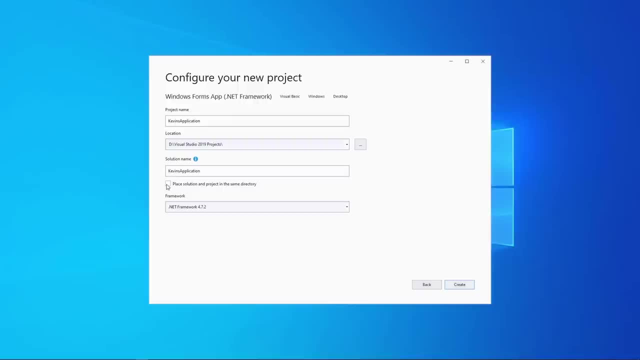 And I'm going to say that I want to place the solution and the project in the same directory by ticking this box. Since this is a brand new project, I'm not going to worry too much about which version of the NET framework I'm using. 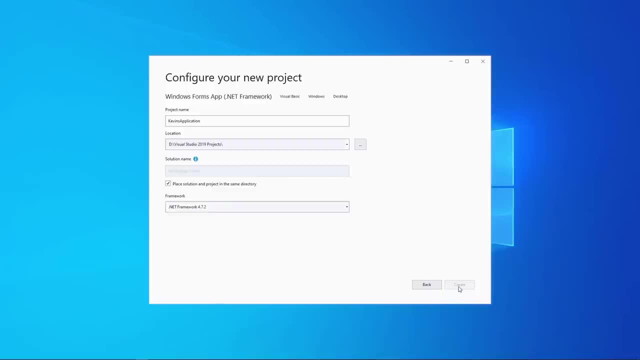 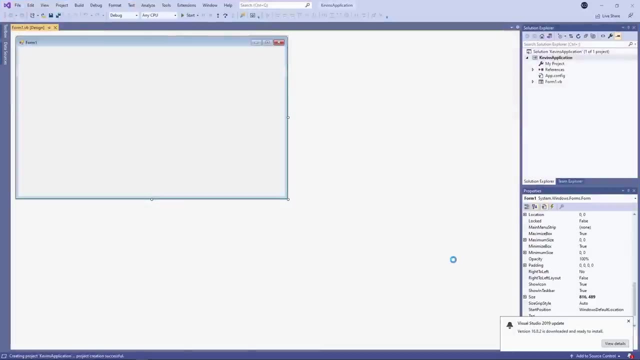 More about that later as well. So let's hit Create, And here is Visual Studio. I can see a little message on the bottom right there telling me that there's a new version of Visual Studio which can be downloaded. I'll maybe do that a little bit later. 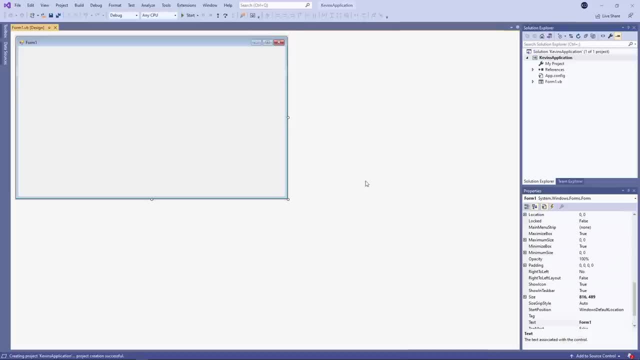 I'll just ignore it for now. Now, there are lots of options here which I'll be talking about as we go along, But suffice to say for now. we have a menu of options across the top, And each of these has a number of sub-options, which, in turn, might have a number of sub-options. 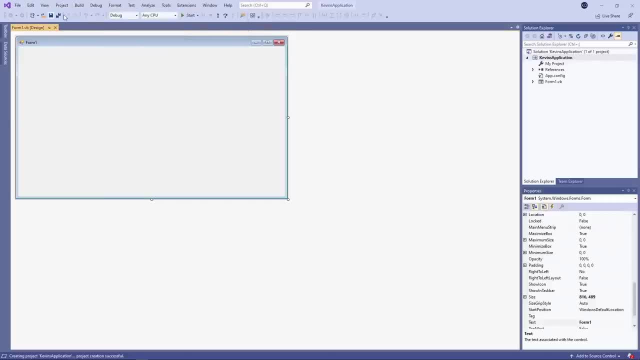 There's a toolbar. I can add extra toolbars, which you'll see later, But the most useful one is here to start with. On the right-hand side, I can see my solution explorer And I can see my solution explorer. A solution is a collection of files that make up my application. 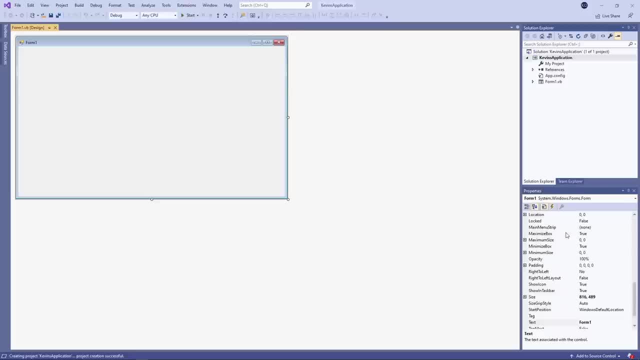 And we'll take a closer look at these files later. I have a properties window, which will become important when I start building my user interface, And on the left-hand side there's a toolbox. If I just click on this, it will move into view. 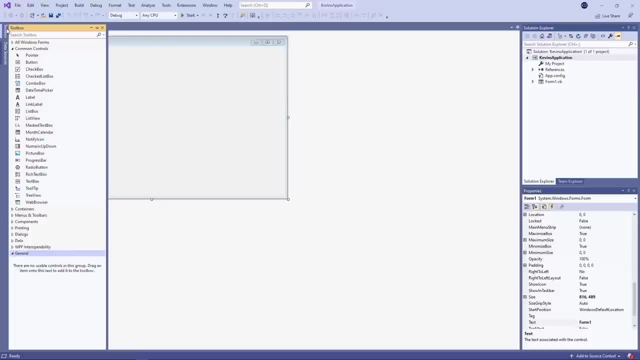 If I click away from it, it disappears. I actually like the toolbox in place all the time, So I'm going to click on this little drawing pin To keep it there And I can resize it if I need to. In the middle I've got my form. 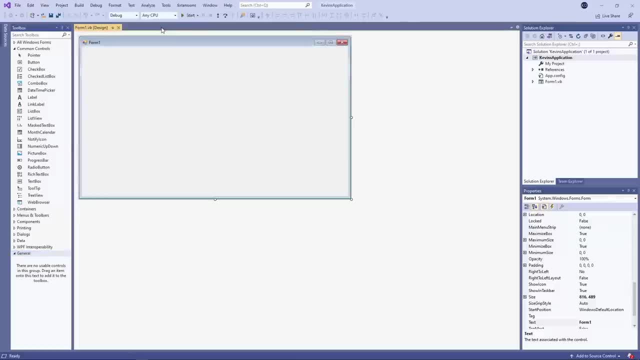 This is where I'm going to start building my user interface, So let's write some code. I'm going to start by dropping a button onto the form. So from my toolbox I click on button, Draw the button onto the form Because the button is selected. I can see properties of the button in the properties window on the right-hand side. 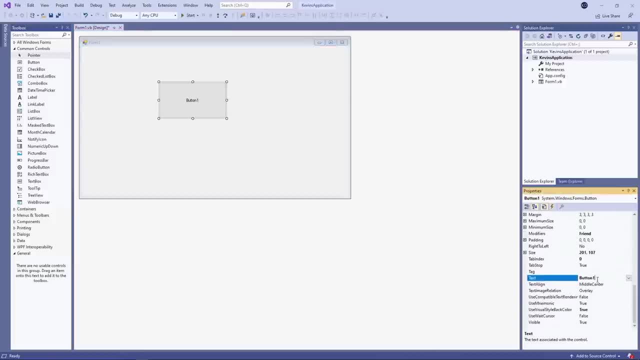 I can see. for example, we have the text property of the button, which is currently button 1.. I'm going to change that to press here And notice how it's changed the appearance of the button on the form. The other thing I want to change is the name of the button. 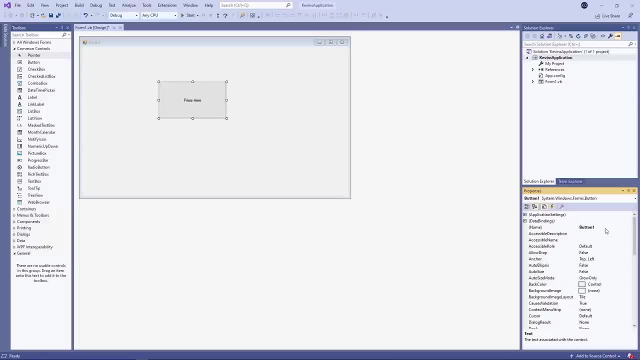 Every option has a name, So I'm going to change that. Every object that you place on the form will have a name property. Now it's currently button 1, because it's the first button which I placed on the form And I could leave it as button 1.. 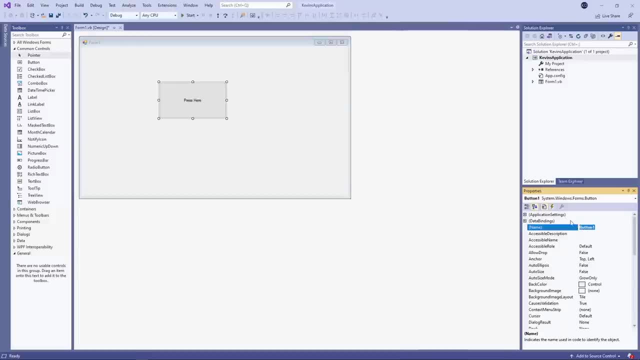 But I want to start using a naming convention- BTN in lower case, because it's a button- And then something meaningful which tells me what the button does, For example start. You could call the button pretty much anything you like, as long as the name doesn't start with a number. 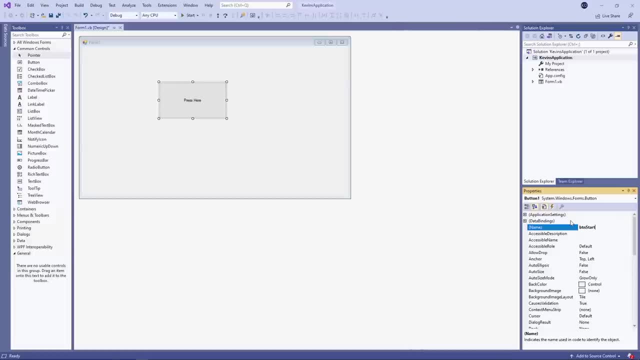 And as long as there are no spaces or special characters like question marks or exclamation marks in there. This naming convention makes it clear what the button does, And it also makes it clear that it's a button, And that will become important later on when I start writing code. 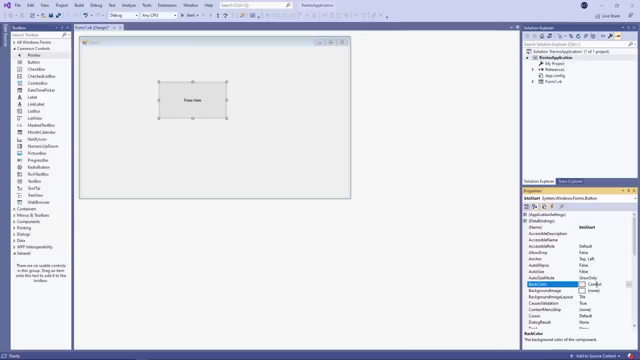 There are other properties which I can change as well, For example the background color, And I have a color palette here which I can use. We'll stick with this for now, But you'll learn about other properties as and when you need them. 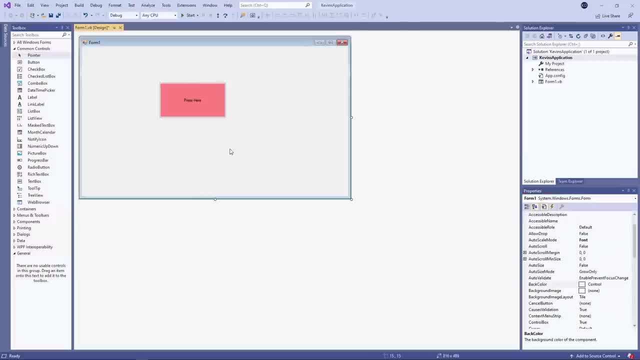 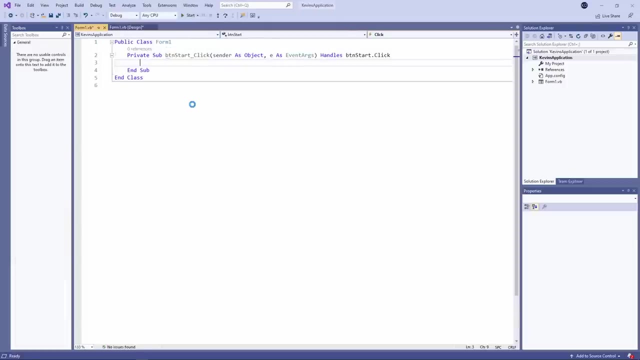 What I want to do now is write some code that will run when the user of my application clicks on the button. To write some code for the button, I can double click it. The way to think of this is that the code is behind the form. 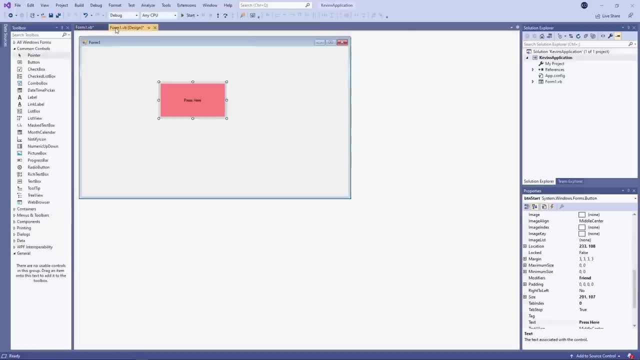 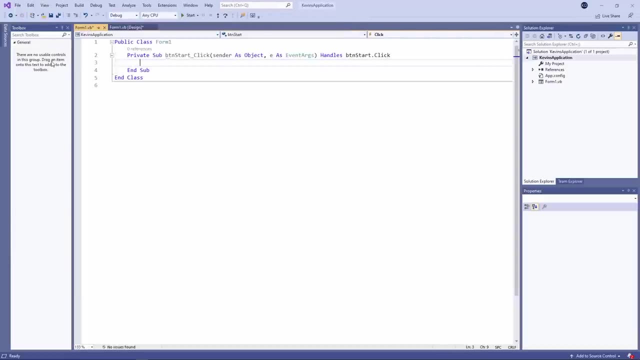 My form is still there. You can see there's a tab here. That's the design view of my form And this is the visual basic view of my form. Notice that the toolbox no longer has anything on it because it's inappropriate to use it while I'm coding. 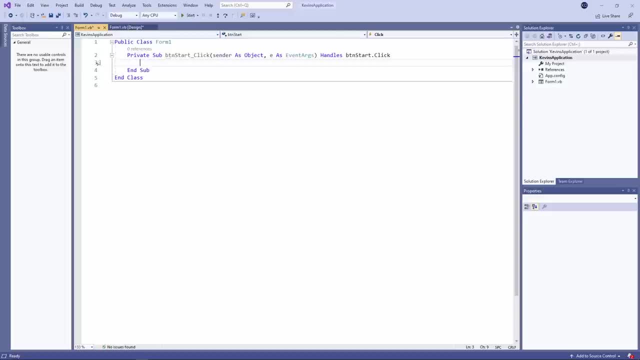 I have line numbers down the left hand side. To be honest, I don't like these and I'll turn them off in a moment- And I can see some code already there And I have to be very careful not to break it. For example, I can see public class. 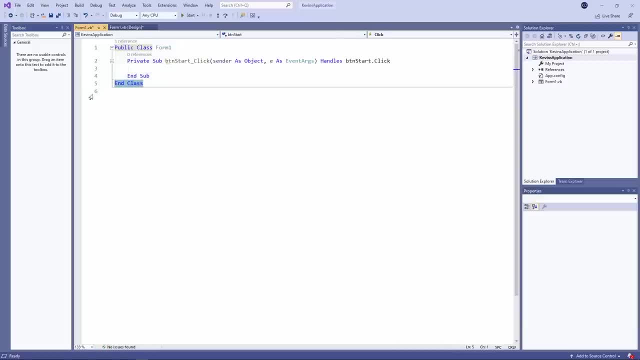 Form 1 at the top and end class at the bottom. I'm not going to change this. These need to be in place in order for the form to work. Later, when you find out more about object oriented programming, these two lines will make more sense. 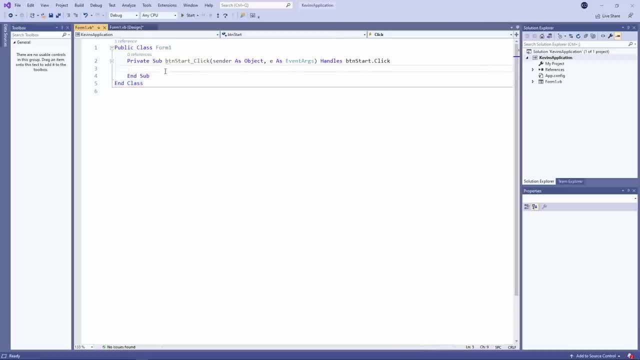 I can also see the stub of a procedure which will run when the button is clicked. Private sub button: start- click. Notice that's the name, That's the name that I gave to my button, And notice that it's going to handle the click of the button. 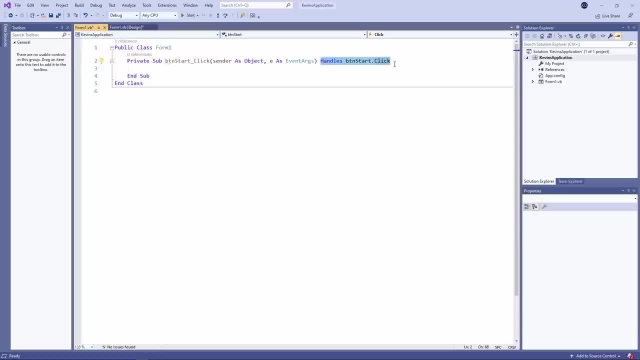 To be more precise, it will handle the click event of the button object. There's also some stuff going on in brackets here. These are called parameters, and you'll find out more about parameters later. Suffice to say, leave this exactly as it is for now. 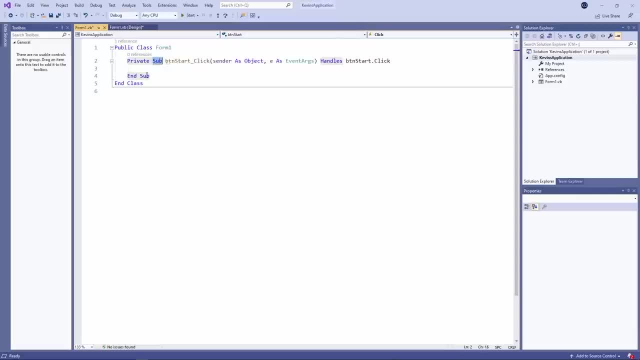 We're going to write code between sub and end And end sub, So I'm just going to press the enter key a few times and give myself some more room. I can also give myself some more room above the procedure and below the procedure. 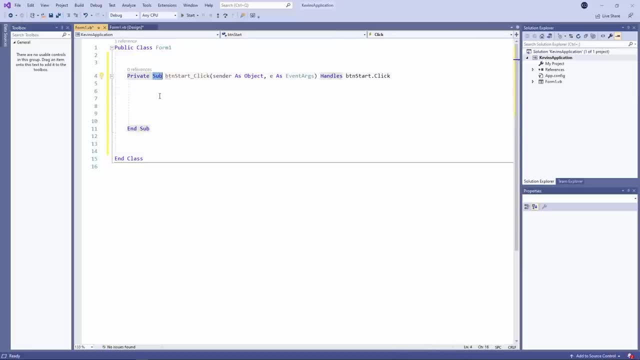 Sub, by the way, stands for sub procedure. So let's write our first program. I'm going to use the message box command. Notice I'm typing in lower case And as I type, a list of options has appeared. Visual Studio is looking at the letters I'm typing and offering me a command to choose from. 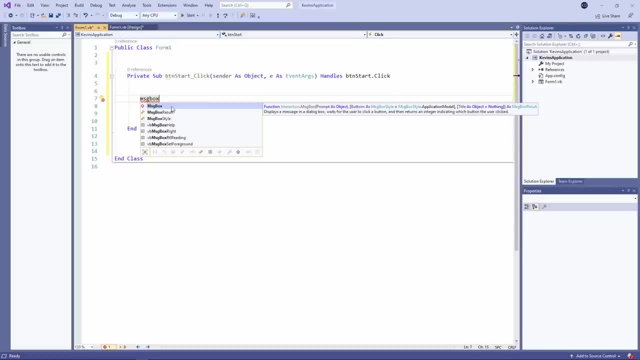 So I can see MSG box here. I can ignore it and carry on typing, or I can actually select it from the list. I'll show you how we can do this more quickly in a moment. I'll just press the spacebar and I'm going to open a bracket. 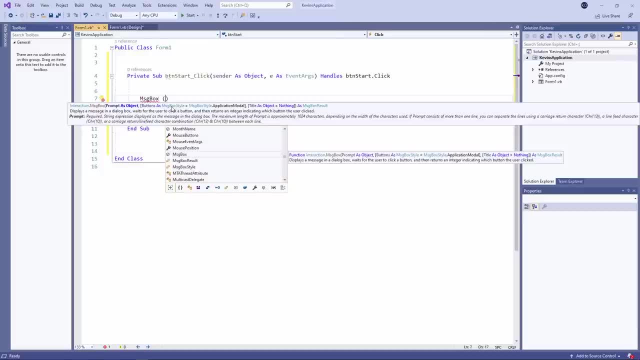 And again there's some more information appearing on the screen. It's quite daunting The first time you see this, But as you get used to it, you'll find it's incredibly useful. Again, I'm just going to ignore it. 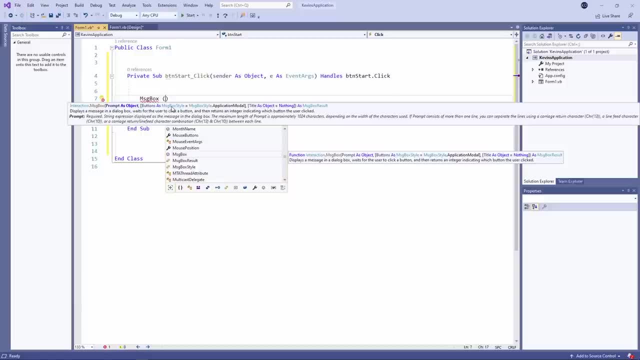 Notice how Visual Studio has automatically put the closing bracket on there for me. I'm going to open a double quote And again, Visual Studio has automatically put the closing double quote on there. And finally, I'll type the text of my message. 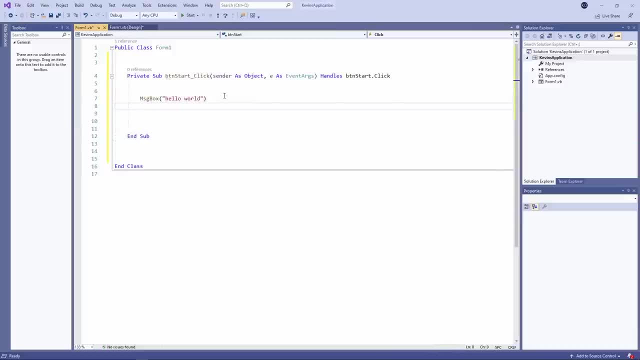 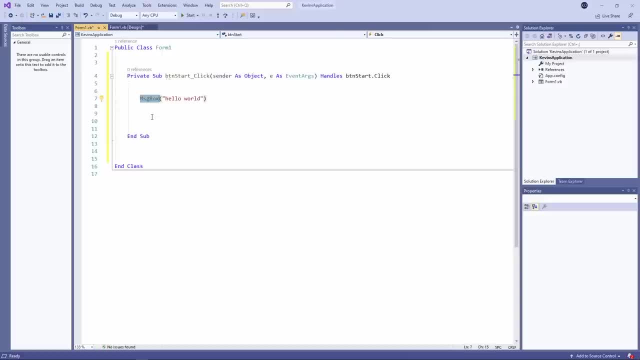 I'm getting visual feedback. Notice also the color coding. the literal string which I'm using in my text message is colored differently from the command itself. Again, I'm getting visual feedback on how to use this. This is why it's called Visual Studio. 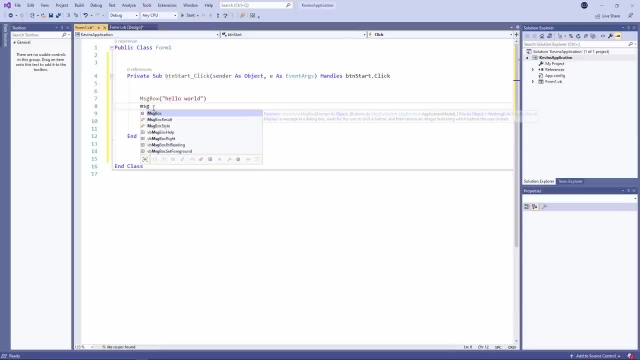 Let's put another message in Now. I've just typed the first few letters this time and I'm going to press the tab key on my keyboard to select the rest of it. I've saved myself some typing. When you get used to it, you can write code very, very quickly. 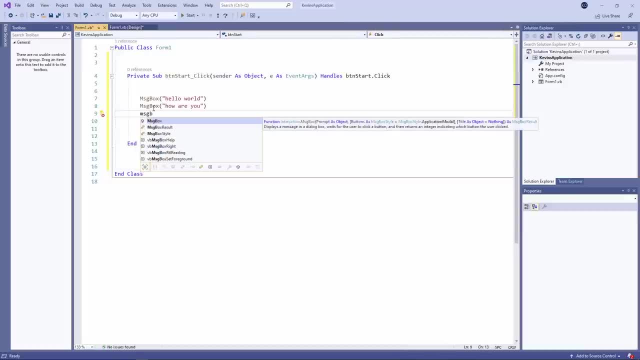 Hello world, How are you? And one more Spelling mistake there. I'm just going to hold down my control key and tap the button, And then I'm going to use the left arrow key, which will jump me one word at a time. 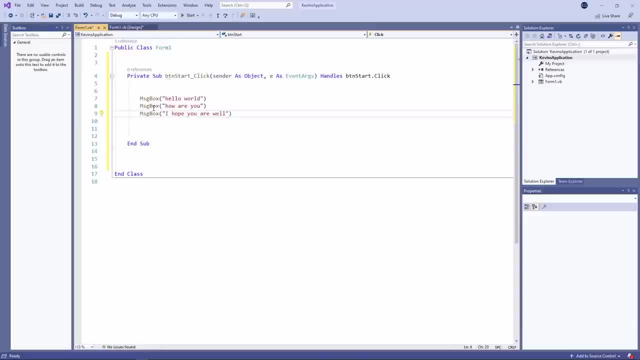 through that text And then I can correct my spelling. To be honest, it doesn't matter what I put inside these double quotes, It won't be a problem. If, on the other hand, I miss type the command, I see a red wiggly line underneath it, telling. 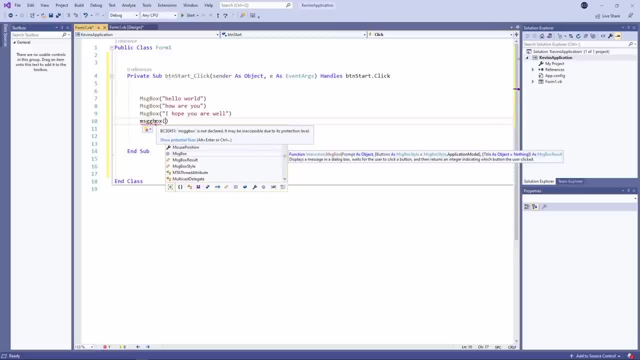 me that I've made an error. This is what we call a syntax error. I'm breaking the rules of the programming language over it. I can see some kind of error message there. MSGG box is not declared. Visual Studio thinks I'm trying to use something called a variable and I haven't announced that I. 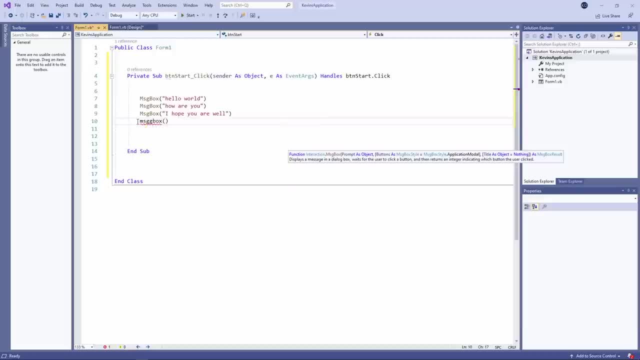 want to use it More about variables later on. Let's just get rid of this line altogether. Okay, so there's my program. I'll just close up a little bit of the white space- I don't need it- And I'm going to run the code. There's a start button at the top And my form is: 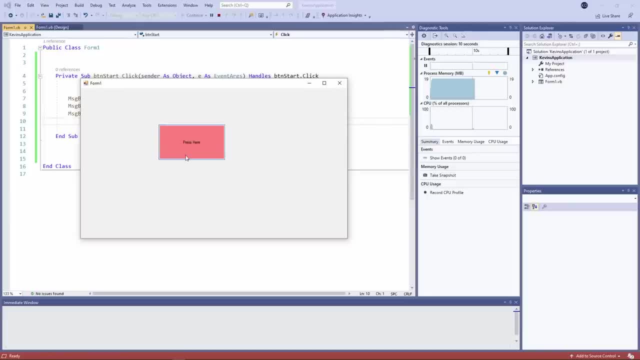 now on the screen And to test it, I'll simply click on the button. There's my first message, There's my second message And there's my third message, And the program has stopped running. My procedure may have stopped running, but the application itself is still running. The form is still. 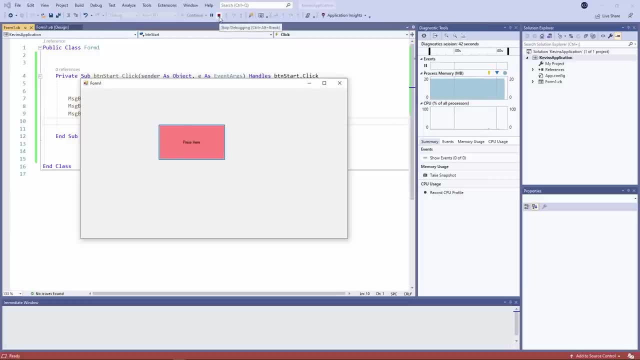 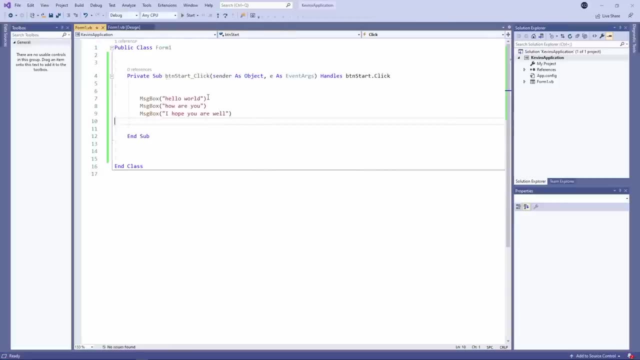 on the screen, And I can stop this running by pressing the red square up here, Or I can simply close the form with the red cross here And everything has stopped. So there we have it, Our first program, which is just a sequence of messages, But it's a program. There's one. 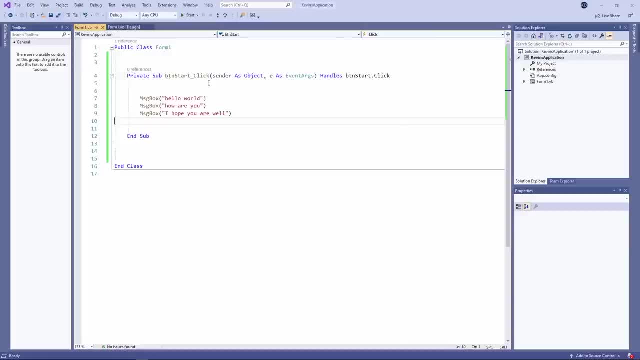 more thing I want to do now, And that is to save my work. Remember, a Visual Studio application can consist of several files. So, rather than just clicking this little button here, which will save the form, I'm going to click this button which will save all of the files in my application. I can. 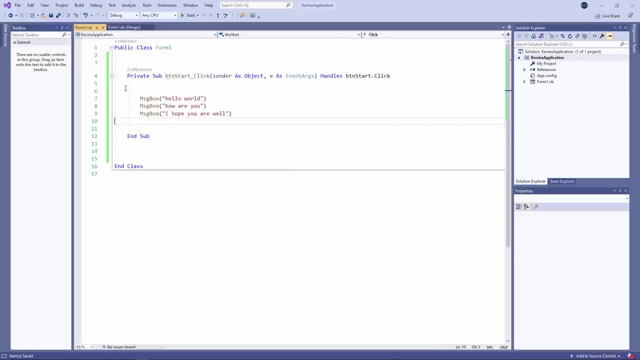 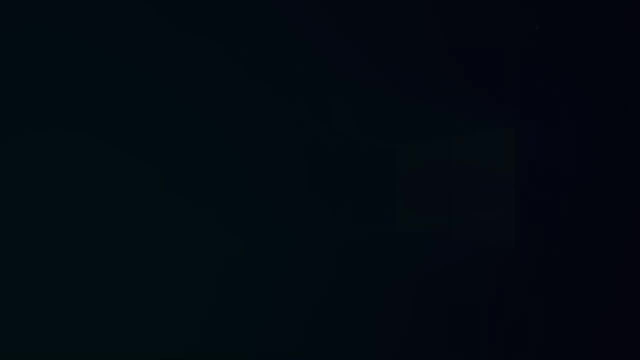 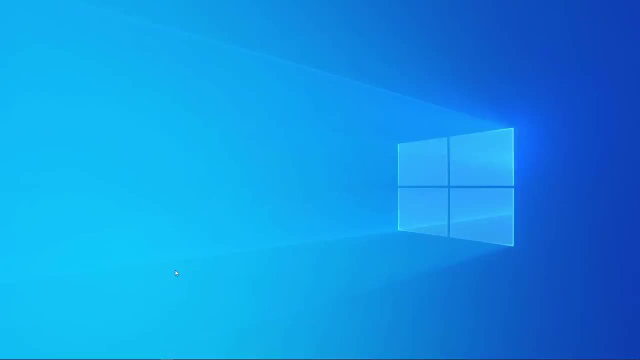 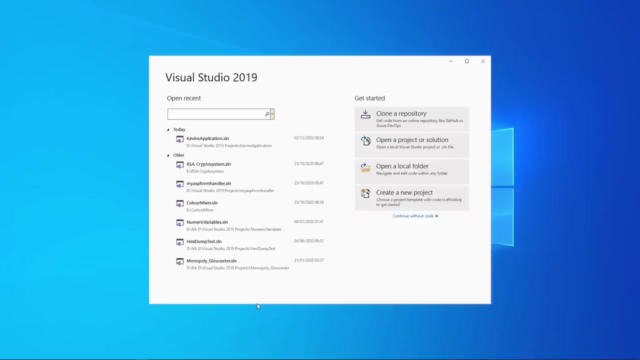 now close down Visual Studio and return to my application tomorrow. In this video, I just want to show you how we can customize the integrated development environment, the IDE That is Visual Studio. So let's start it up again, And I'm going to open up the project that I was working on last time. Notice that it's in the recent 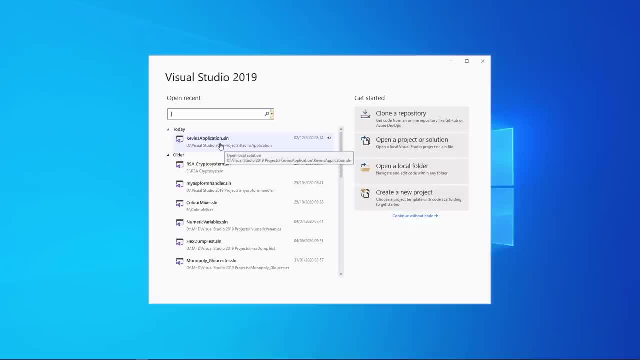 files list, So I could just click on it here. Alternatively, I can click on update And then I can now see that I've created a new project And I can now open it up, And I can now see that I've created a new project And I can now see that I've created a new project, And 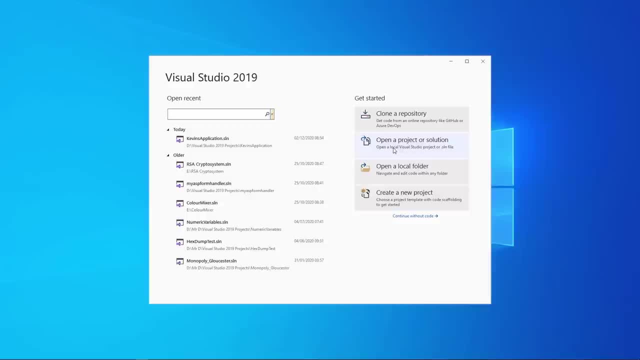 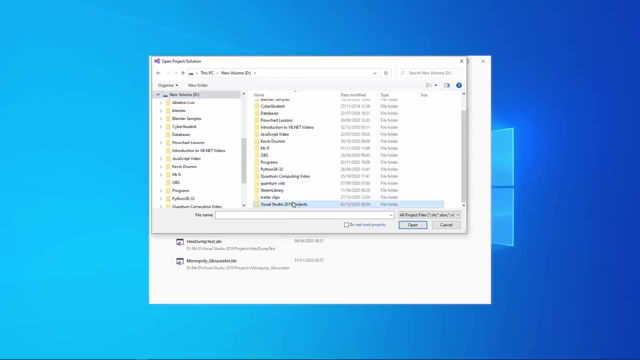 open a project or solution. Let's do it this way for now, so we can see which file we need to open up. Here's my D drive. This is where I'm storing my projects, And here's the one I was working on last time. Notice it's a folder. Inside that folder, there's a solution. 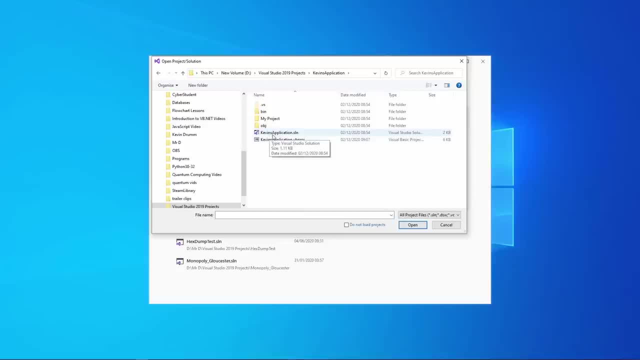 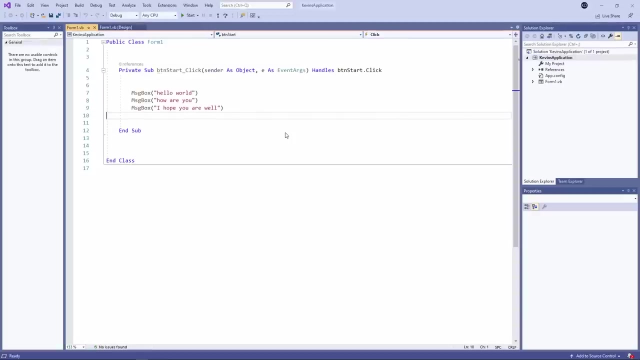 file SLN. That's the file which ties together all of the other files that make up my application. That's the file which I need to open And here's the application I was working on last time. Here's my form And here's the code behind it. A little word of warning first. 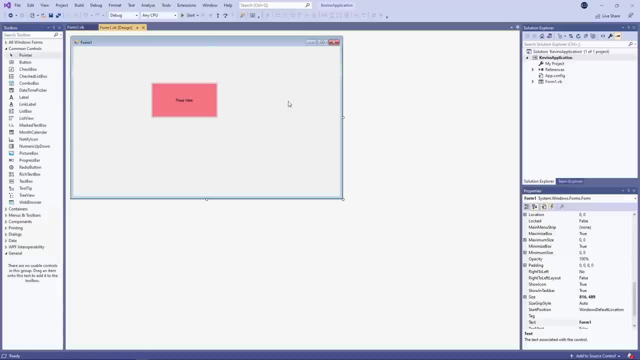 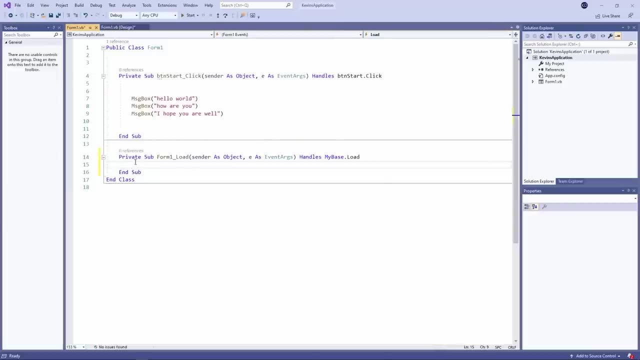 of all, Sometimes you might accidentally double-click on the background of the form itself. Watch what happens when I do this. I've got another procedure stub here called Form 1.0. Form 1.0. Form 1.0.. 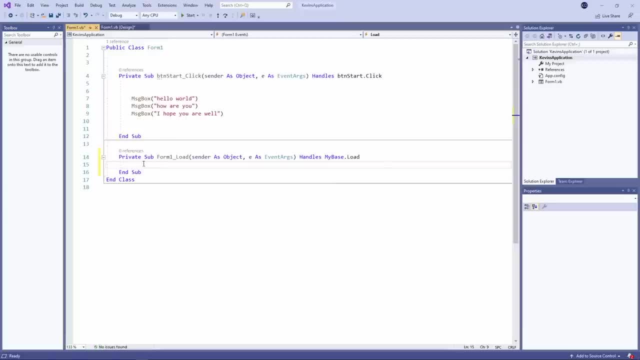 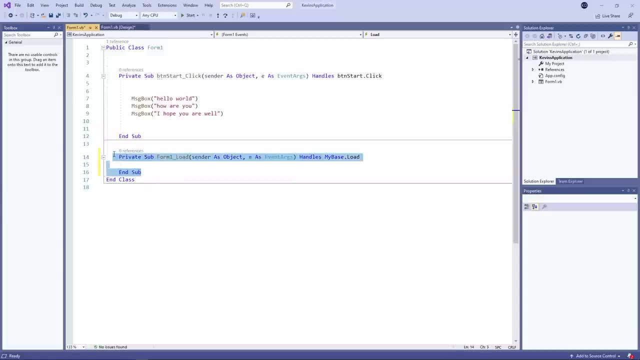 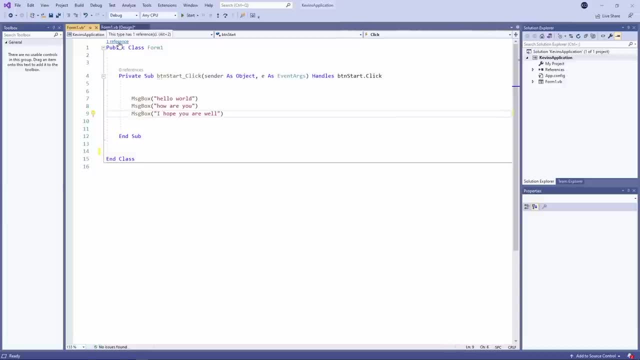 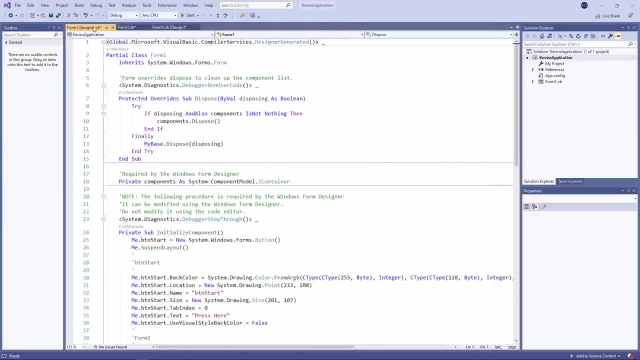 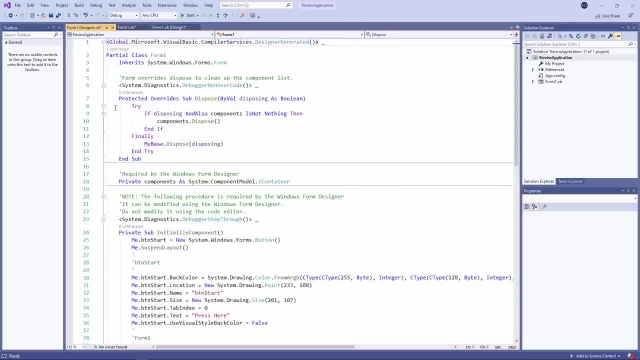 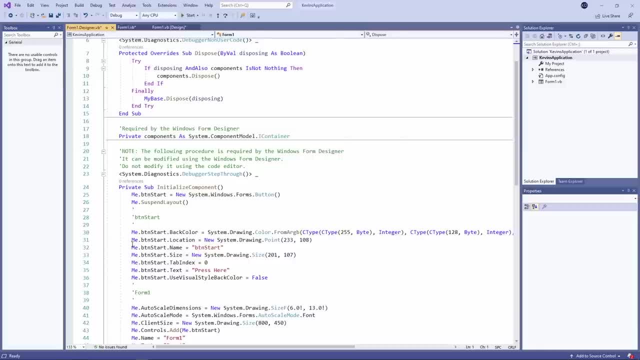 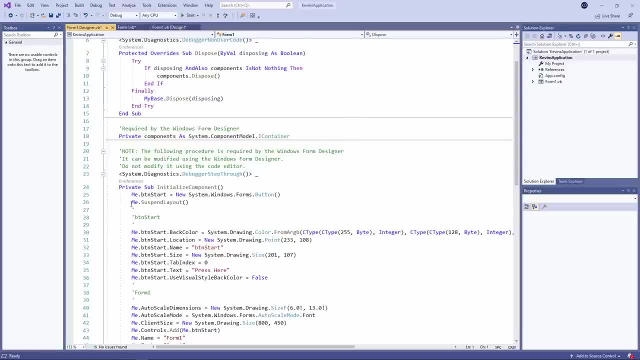 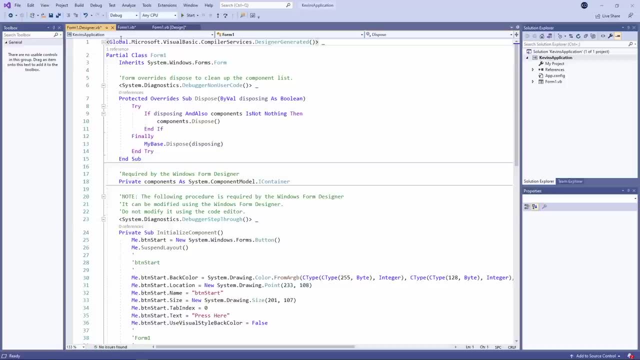 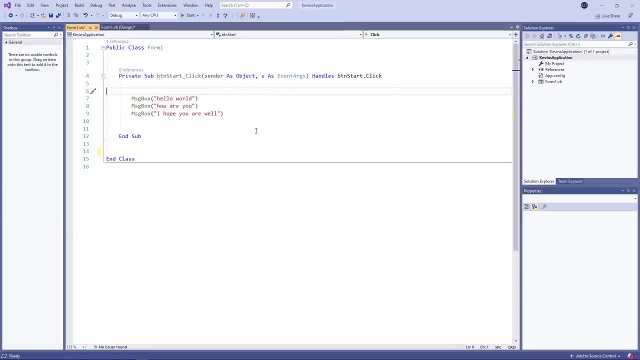 Anyway, what I want to talk about now is how we can customize this programming environment. You were given some options when you ran it up for the first time, but you can change those options inside Tools Options. Notice I'm using a color theme- blue- but you can change it to dark if you wish. 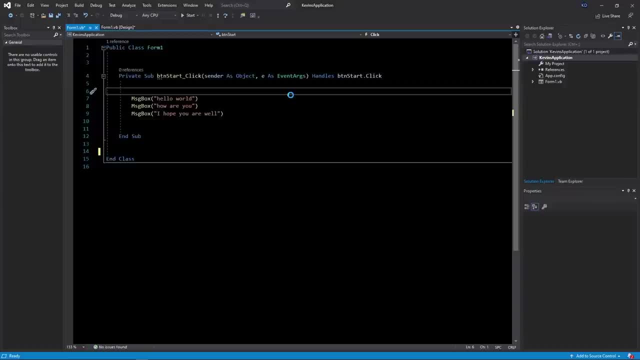 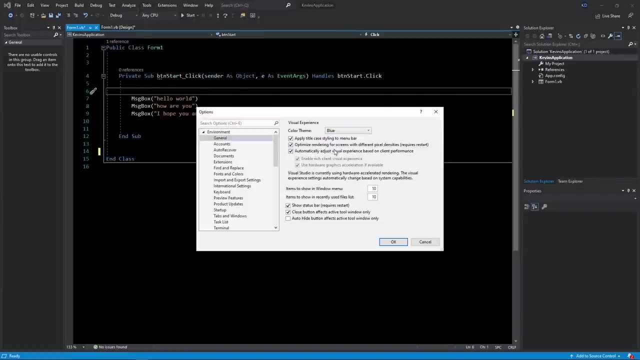 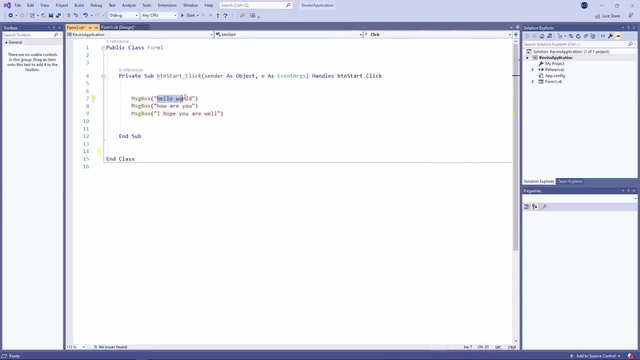 Some people much prefer this. To be honest, I don't. I prefer black on white, not white on black. It really is a matter of preference. I'm going to switch it back to the way it was. I can also have finer control over the keyword colors and over the text colors and any other. 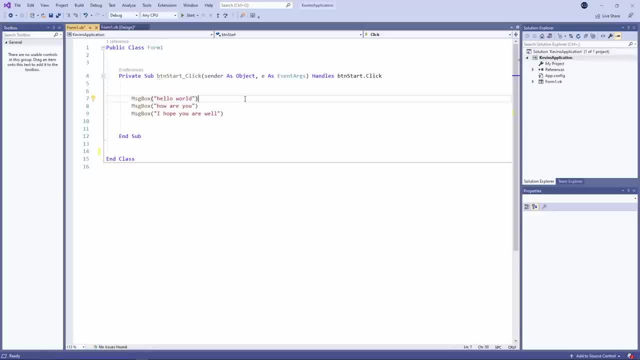 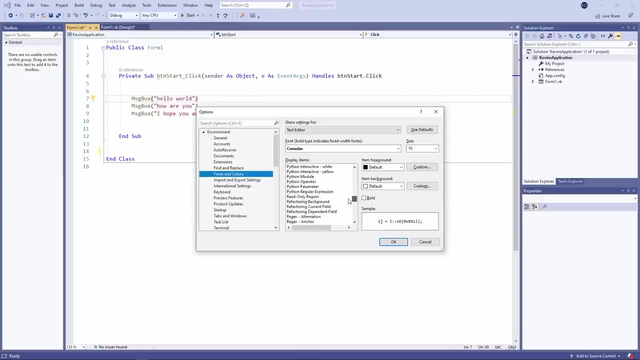 colors that you see on here. for that matter, We can do this by selecting Fonts and Colors. You can see there's a lot of options here. Keyword- the default Keyword. The default color is blue, And I can switch that to magenta. 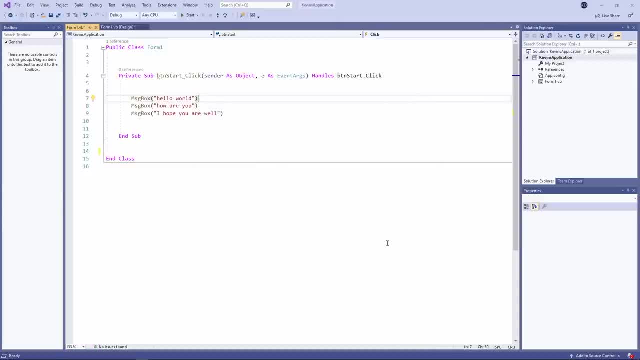 You do need to be a little bit careful, though, because some colors have special meanings and it can start looking very messy as well. If needs be, you can change things back. Notice there's an option here to use defaults. Some people like to increase the font size as well. 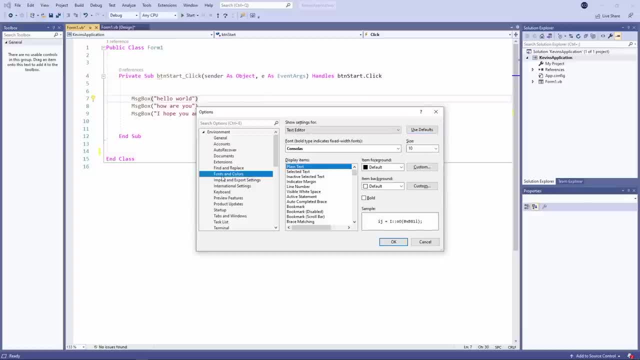 It's entirely up to you. Something else I want to change- to give myself some more room on the screen- is to switch off these line numbers. I can do that by going to Text Editor, All Languages, and then here, Line Numbers. Notice I can have different configurations depending on the programming language I'm 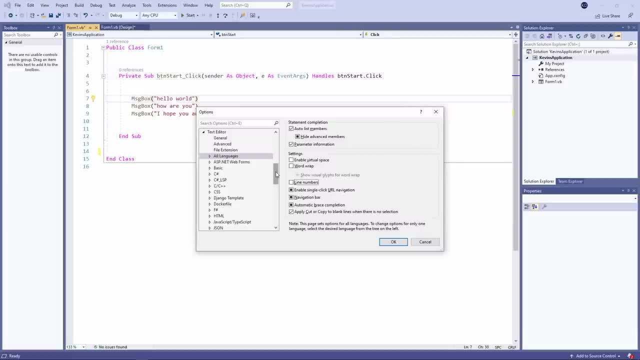 using. And there's one more thing I want to change, and that's some of the default file locations. I can do that underneath Projects and Solutions Locations. You can see I've already set my Projects location to my D drive. Needless to say, there are lots more options which you can set in here. 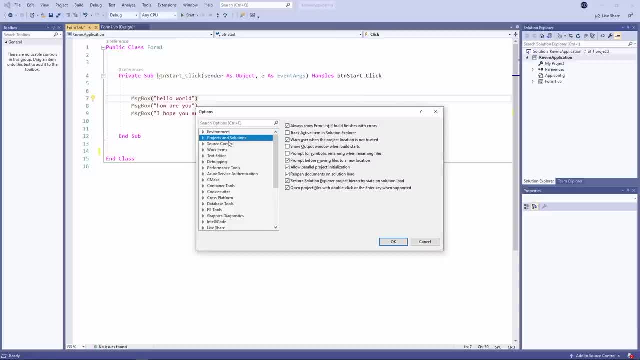 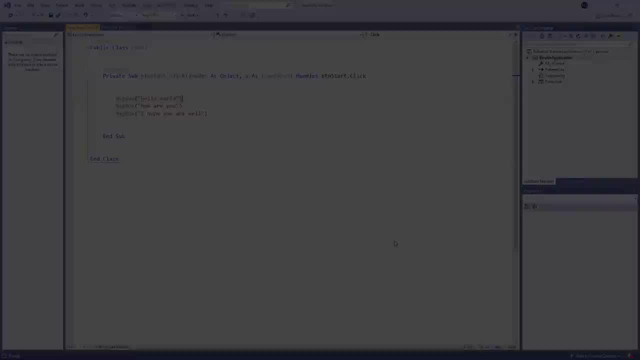 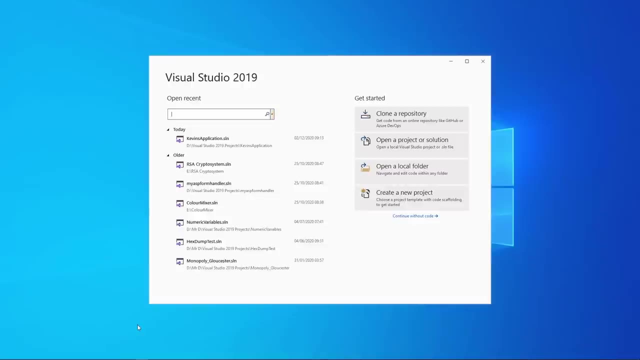 And I'll be honest, I don't know what half of them are, But when I need them, I'll find them. I'll find them. Click OK for your changes to take effect. In this video about VisualBasicnet, I want to say more about output and I'm going. 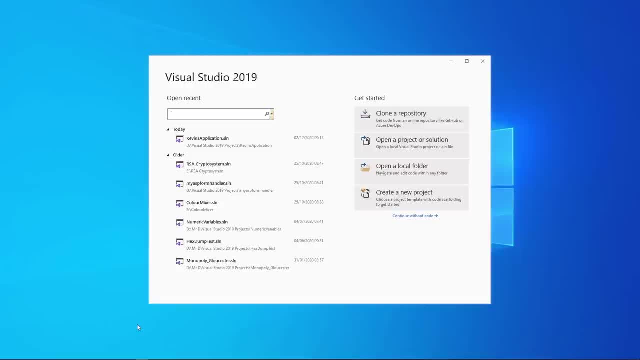 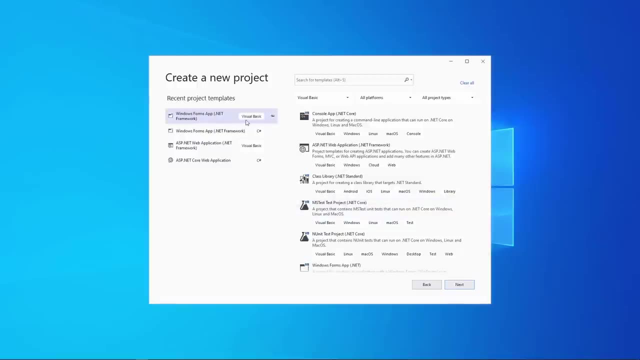 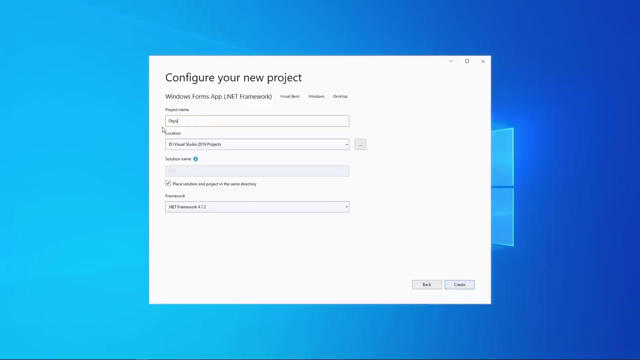 to introduce you to variables, I'll start by creating a new project. As before, it'll be a Windows Forms application in Visual Basic. Give the project a meaningful name and think about where it's going to be saved. You can change this if necessary. 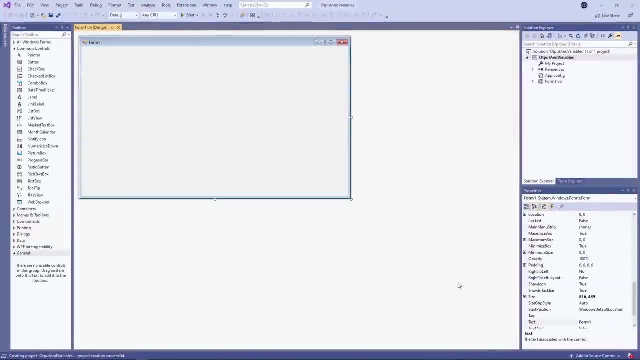 Let's start with a button on the form and I'm going to rename the button. Get in the habit of renaming things that you place on the form as you go along. btn, That's my convention. And then go. This is called camel notation because of the capital G. It looks like a camel with a hump. 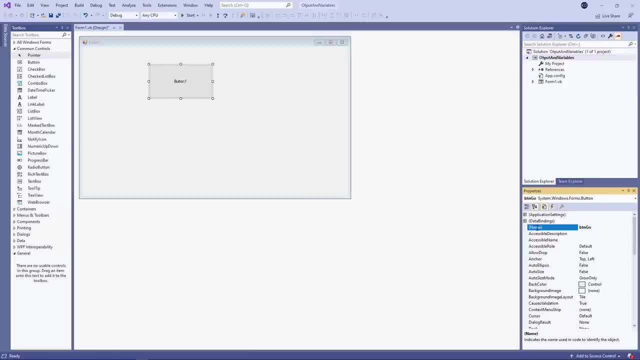 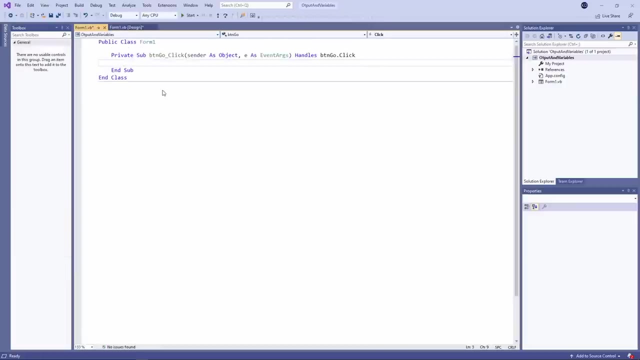 on its back. I'm also going to change the text property of the button And let's write some code that will run when the user clicks on the button. To get to the code behind the form, I double click the button And let me just remind you. 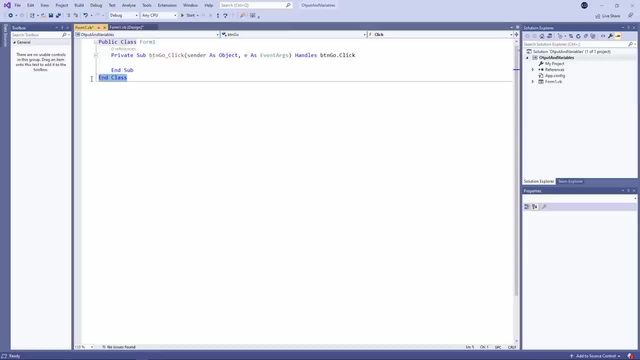 You mustn't change Or delete this. If you do, you'll start seeing errors on the screen. Watch Straight away. I've got a syntax error up here. Class statement must end with matching end class. I'll just use the undo button to put it back again. 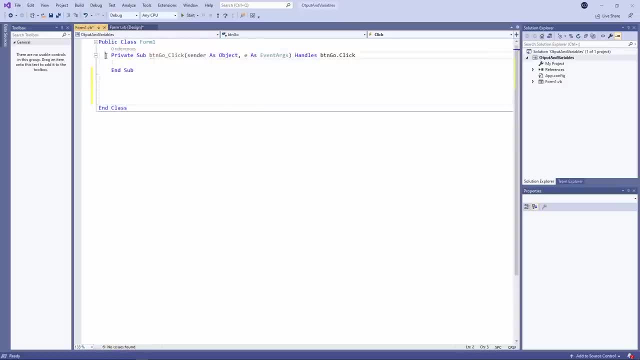 And I'm going to give myself some white space. Just give myself a bit more room on the screen here. And we've already seen that we can display a message on the screen using the message box command, So let's do this. To test it, I simply press the start button. 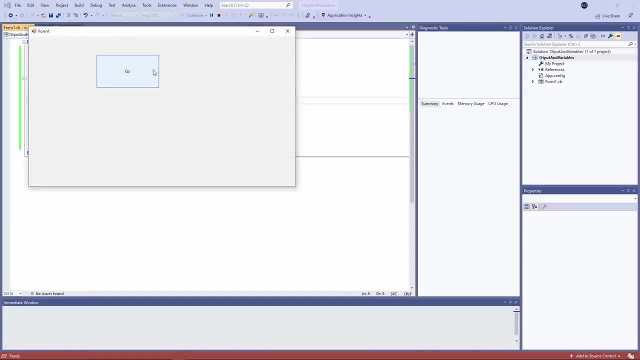 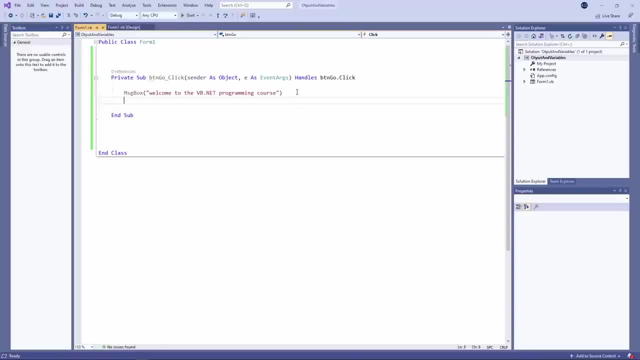 That will run the form up, And then I can run my code by clicking on the button itself. Now there are three fundamental constructs when it comes to programming that I'd like to mention now. The first of these is sequence, The second is function. 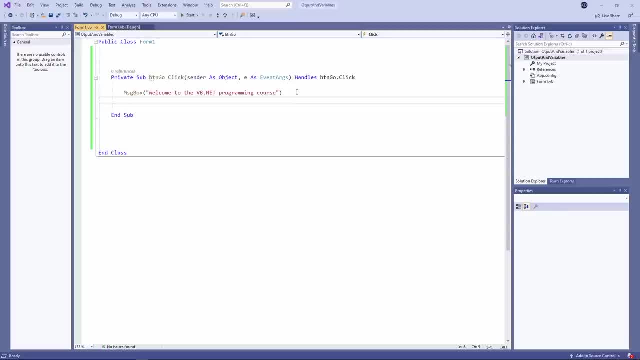 And the third is function. The third is selection, which you'll see in a later video, And the third is iteration, which you'll also see in a later video. For now, let's just say a little bit about sequence. Sequence simply means that each statement in a program or a block of code will run one. 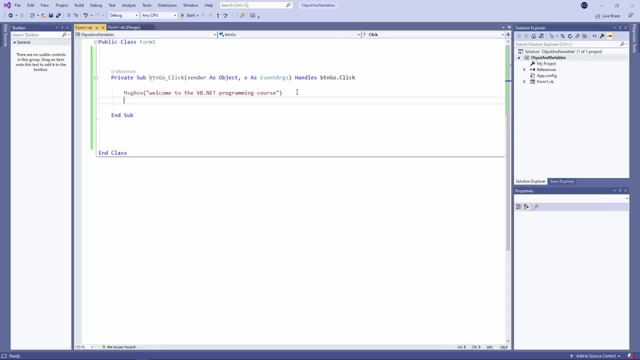 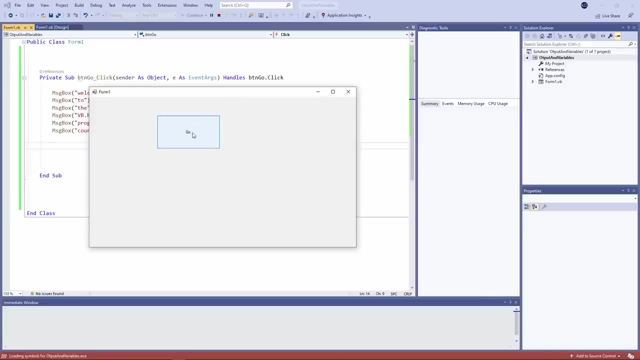 after another in sequence. So, for example, I could display each of these words separately. Run the program, Press the button and one message after another And I'll stop my application with this red square. If I want to display these words in reverse order, I can simply change the order. 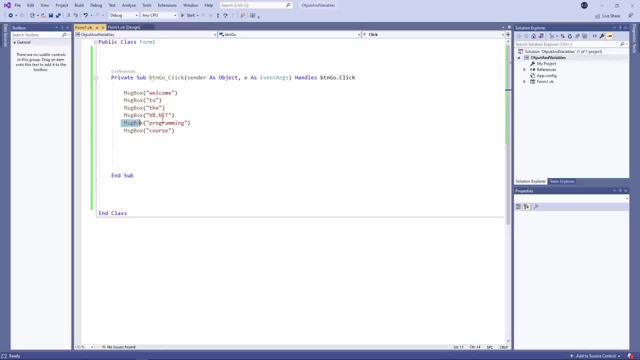 I can call this word a order and the other one a sequence. I can also give it a name. I can go to the other side. order of the commands. I'm just dragging and dropping and tidy up some of the white space. You can have as much or as little white space as you like, whatever. 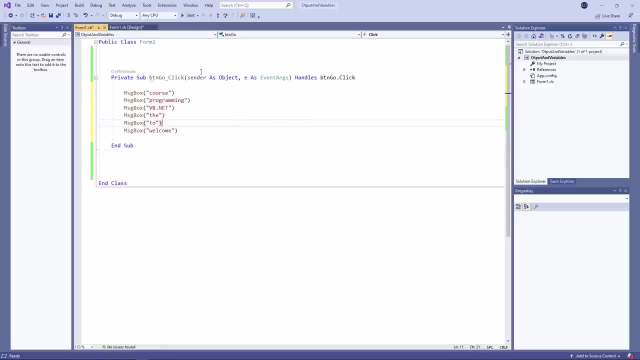 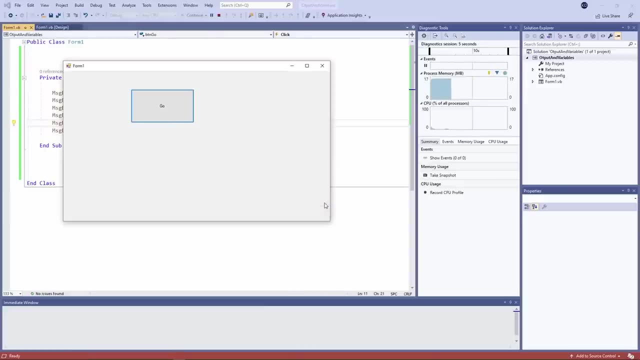 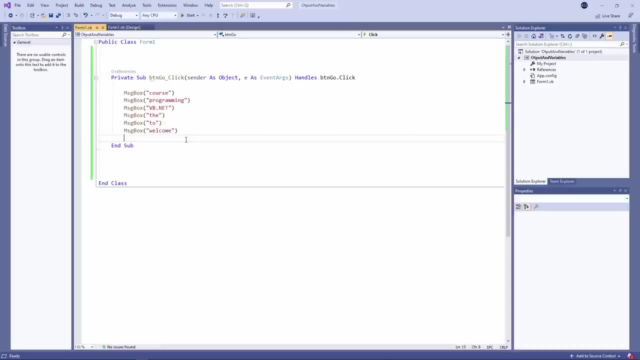 makes it easy for you to read the program. Let's give this a try. Before I continue and talk about variables, I just want to show you another command I can use to display a message on the screen- MessageBoxshow. Let's take a look This. 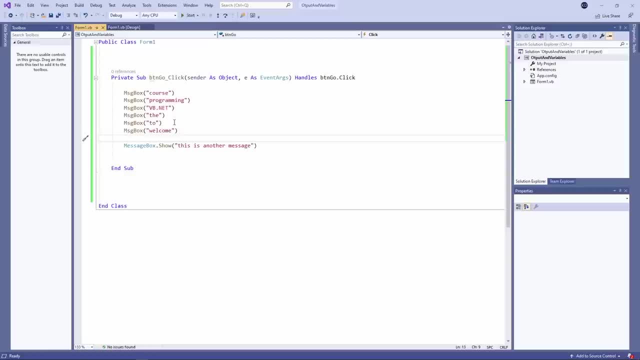 is another message. It does exactly the same thing. To be honest, this is a bit of an old style command which has existed from very early versions of Visual Basic. This is a more modern way of doing things. This is an object-oriented approach And it'll. 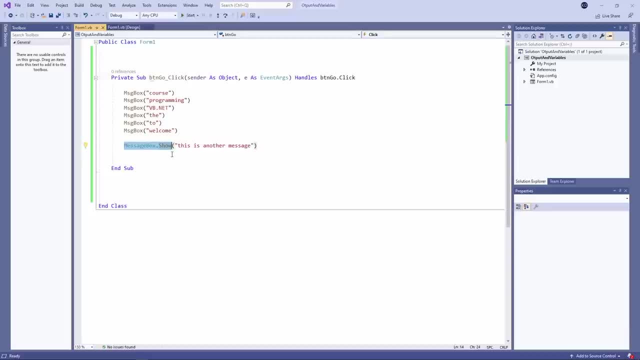 make more sense why you might do it this way later, when you find out more about object-oriented programming. For now, you can either use MSGBox or MessageBoxshow. I'm going to continue with MSGBox, So now let's talk about variables. I'll start by placing another button on the form. 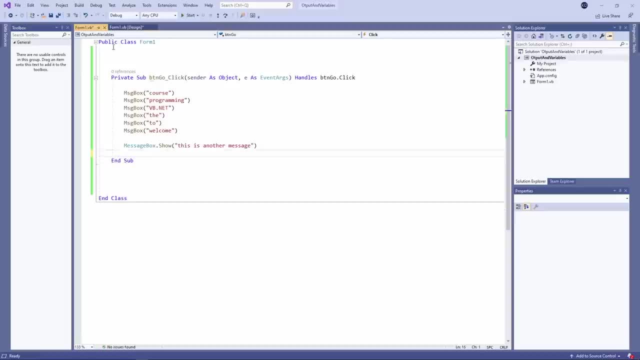 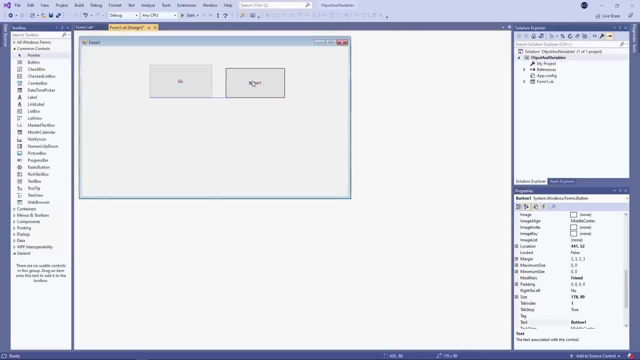 because I want to write a separate procedure. Switch to the form and drop another button on there. Notice I'm getting some guidelines as I drag the button around and resize it. This helps me to create a nice layout for my form. Okay, let's get in the good habits of naming objects as we go along. So I'm going to call. 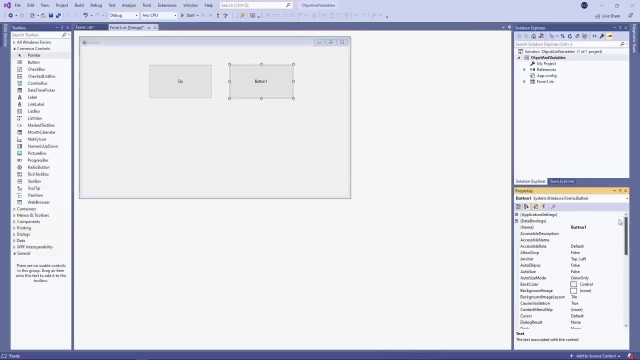 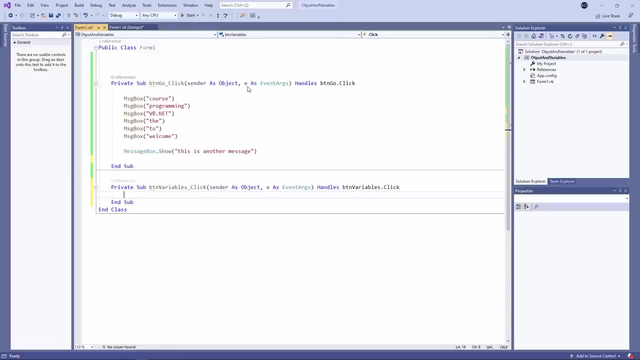 this btnVariables And I'll change the text property as well. To write the code as before. double-click And you can see I now have a new procedure stub. I can start writing my code here. Let's give myself a little bit of time. 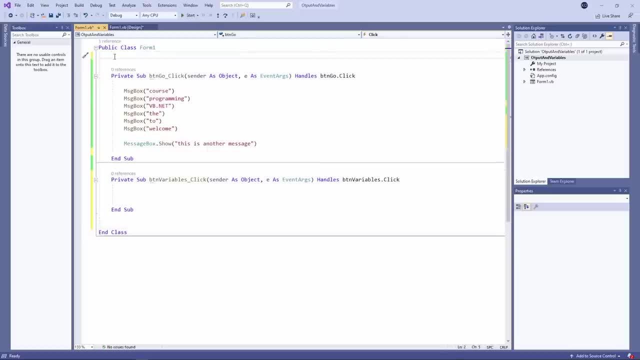 So I'm going to go back to my form and I'm going to call this btnVariables, And I'll have a little bit more white space below and a little bit less at the top here. So what is a variable? Well, a variable is actually a location in the computer's memory. 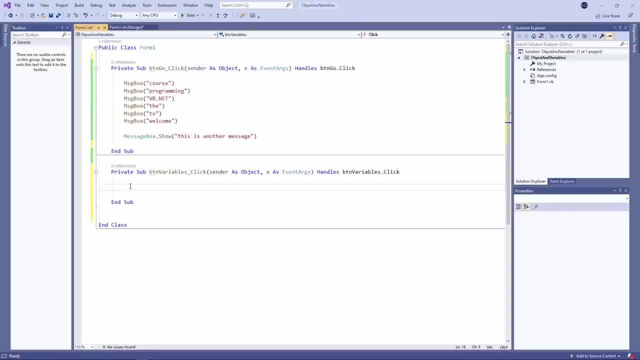 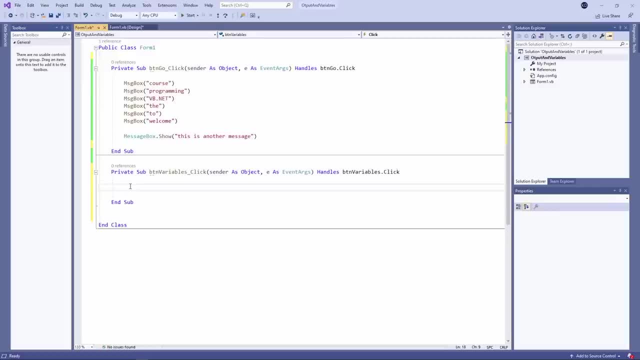 The first thing I need to do is declare it. I need to announce that I want to use a new variable, And I do this using the dim statement like this: Now, there are a number of things going on in this command. First of all, the word dim. 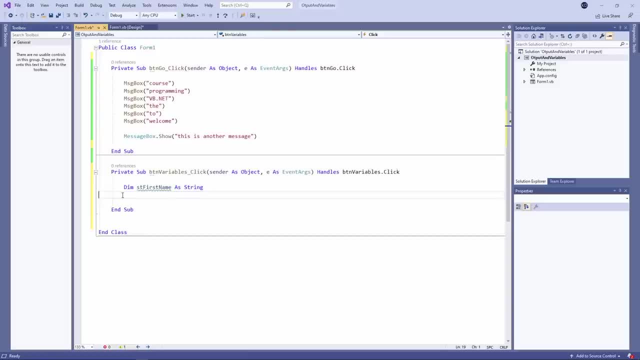 is short for dimension, because I'm actually setting aside a certain amount of memory. I'm specifying the size or the dimension of the variable. The amount of memory being set aside depends on this, which is the data type of the variable. When it comes to string variables, one byte of memory will be needed for each character. 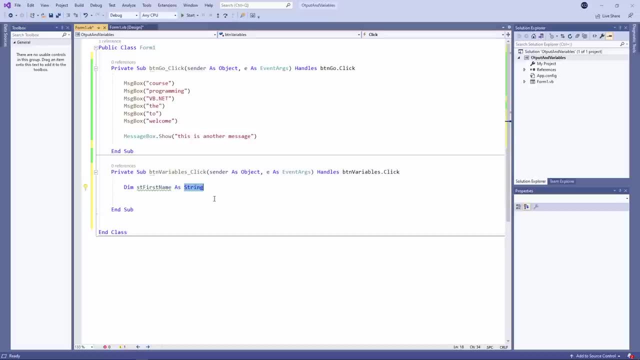 in the string. But, to be honest, I don't need to worry too much about that. Visual Basic will look after the memory for me. Or, to be more precise, the runtime engine that Visual Basic depends on will take care of the memory for me. 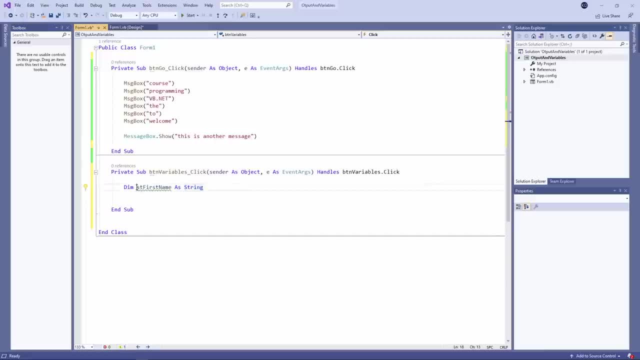 The other thing I'm doing is I'm giving my variable a name And again, notice that I'm using camel notation and I've prefixed it with st because it's a string variable. That's just a convention which I'm going to encourage you to use. You might want to. 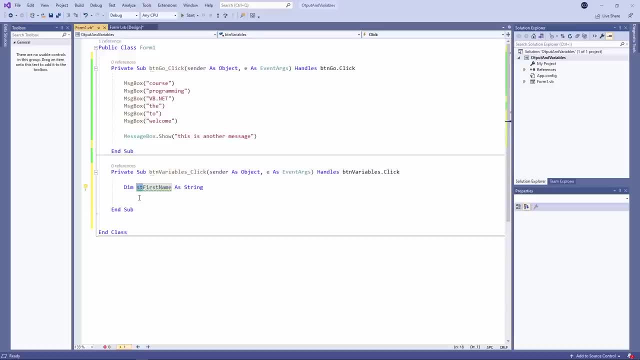 know what datatype a variable is just by glancing at its name. So that's my variable declaration. I've got a green wavy line underneath it to tell me that I haven't done anything wrong with it yet. unused local variable. so let's now assign a value to it. notice. 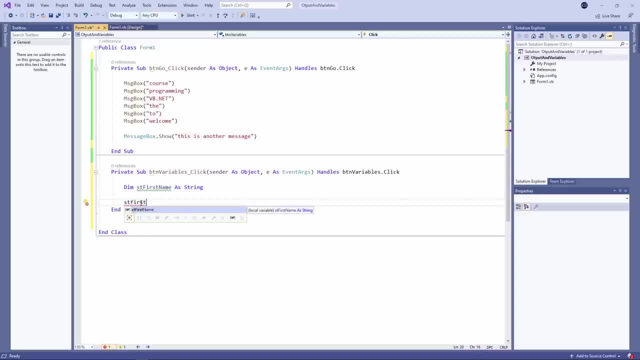 I'm typing in lowercase. I'm being offered the name of the variable in a list, so I'll just press the tab key to select it and I'll say ST. first name is equal to my first name. notice that the green wavy line has disappeared now. 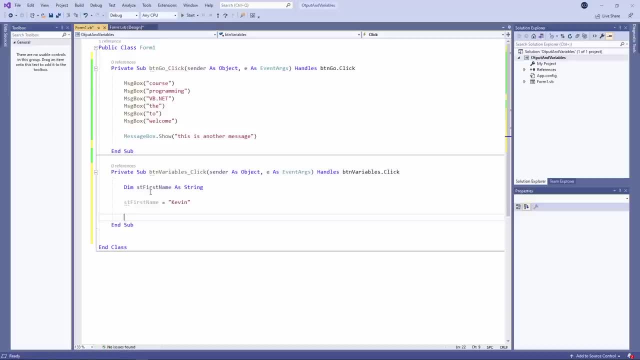 because I'm using the variable. in earlier versions of Visual Basic you would have to use the let command in front of this. you'd say: let ST first name equal Kevin, let it become Kevin. in this version of Visual Basic we don't use let at all. but what you need to appreciate here is I'm putting the 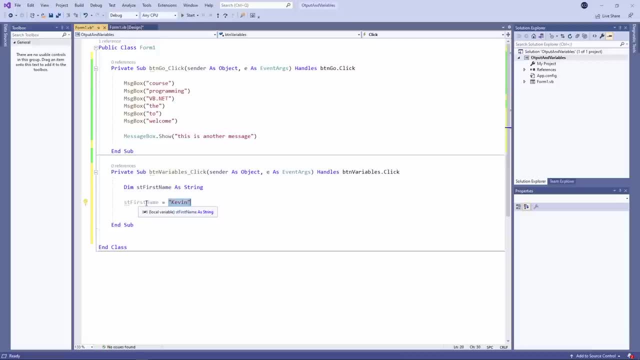 string Kevin into that piece of memory which I set aside, because the string is one, two, three, four, five, four characters long. it's going to take up five bytes of memory, as I said before, though you don't really need to worry too much about that. okay, now I'm going. 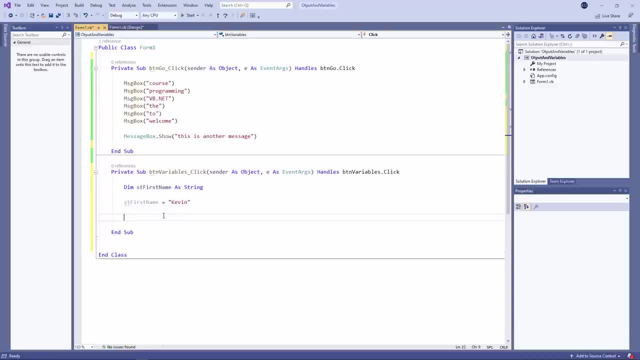 to output the contents of that variable and I'll do that using message box. notice that I haven't put double quotes around the name of the variable because I want to output its contents. I'm going to put the name of the variable because I want to output its contents. 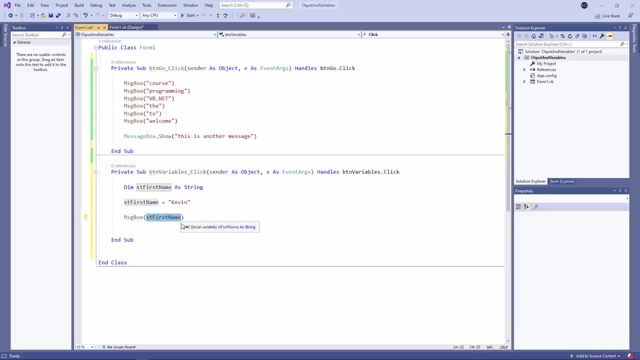 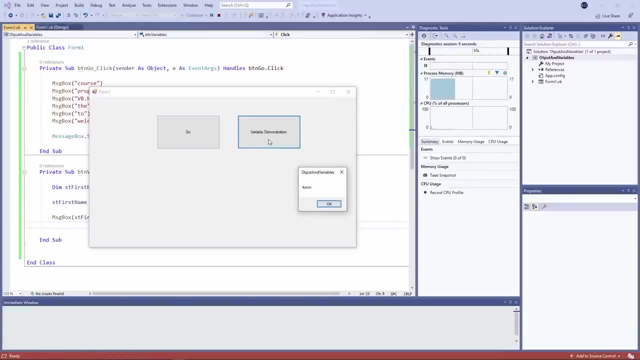 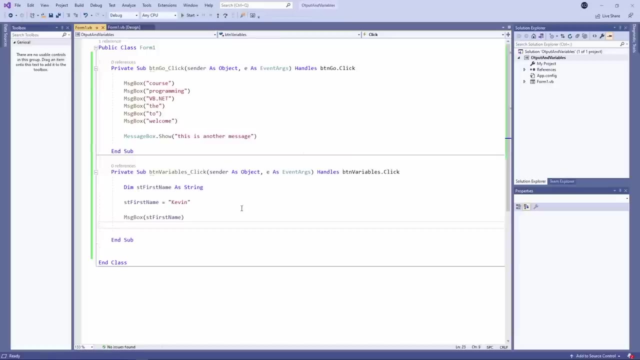 I don't literally want to output the string ST first name. let's see what happens. I'm outputting the contents of the variable. I want to make the message a little bit more friendly, so I'm going to join the contents of the variable with some literal text like this: 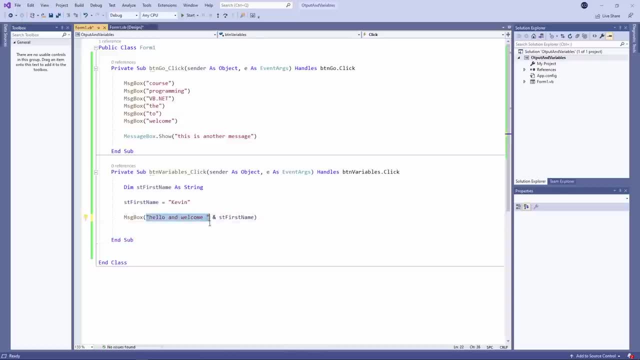 you can see that this is a literal string because it's inside double quotes and this is the contents of my variable and i'm using the concatenation operator, which is an ampersand, to join the two together. we call this string concatenation. i can concatenate something onto the end of it as well. 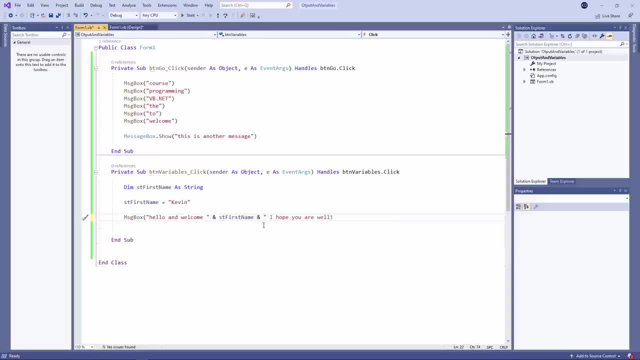 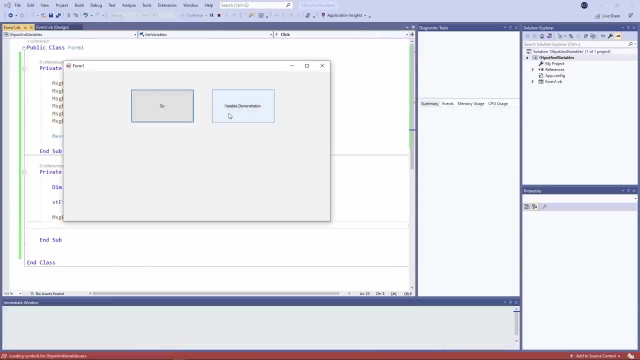 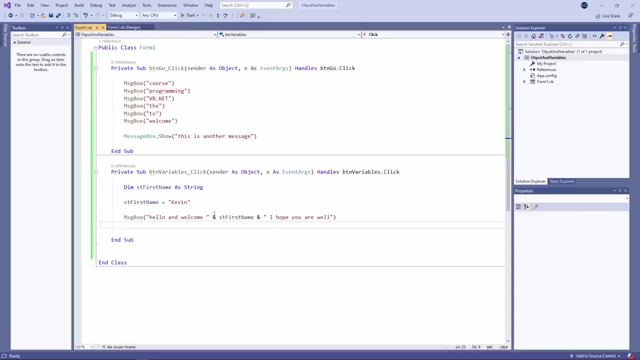 again another concatenation operator. let's see the effect. Hello and welcome, Kevin. I hope you are well. I want you to notice that I put spaces inside these text strings. Notice there's a space after the letter E. Let's just remove it for a second and see. 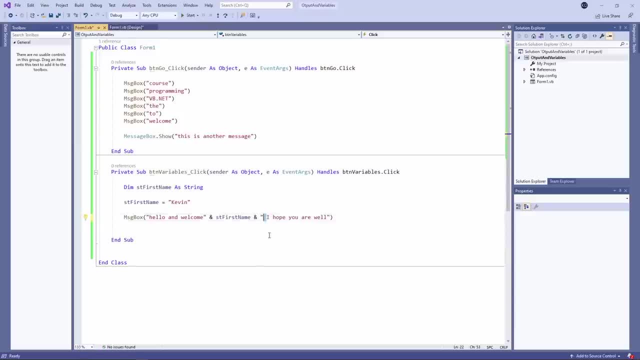 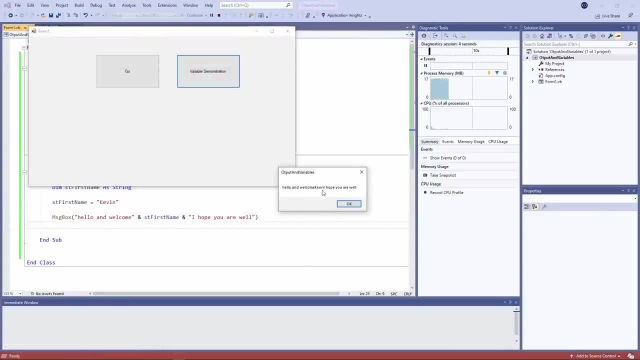 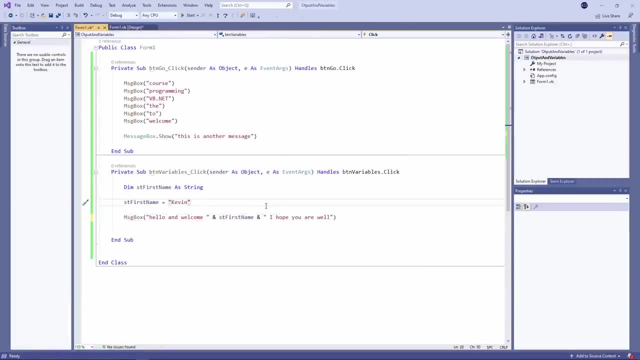 what happens. I've also got a space there inside the string immediately before the I. I'll just take that out as well. look what happens. You can see the message is a little bit messy. Let's tidy it up. Okay, I'm going to declare another variable to hold my last name. 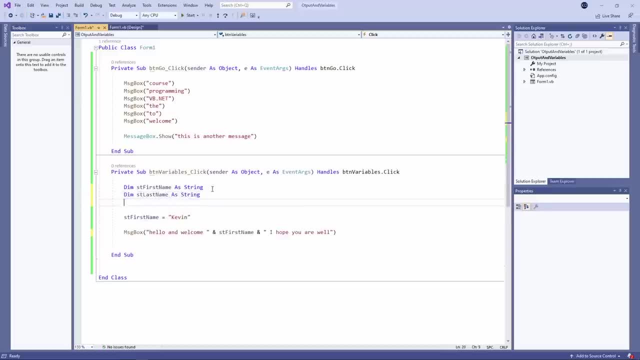 So another dim statement, And I'll assign a value to this variable as well, And I'll include the last name as part of the message. A common mistake is to not use enough ampersands. Watch what happens if I get rid of this one. 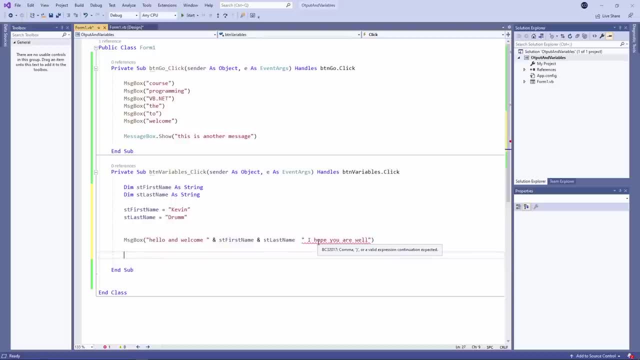 You can see I have a syntax error. The message isn't particularly helpful, but I know that there's something wrong with the way I've concatenated this string together, So let's put the concatenation operator back in place. Another common mistake is not to use enough double quotes. 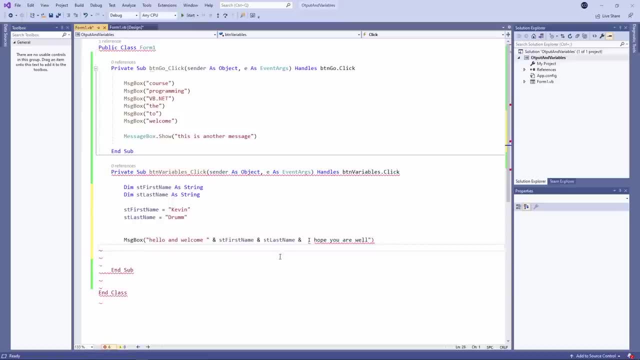 So again, I'll take out one of those double quotes And you can see that the whole thing seems to be a problem. One little error and I've got red wavy lines all over the place. This is not particularly helpful. Just remember: double quotes and brackets come in pairs. 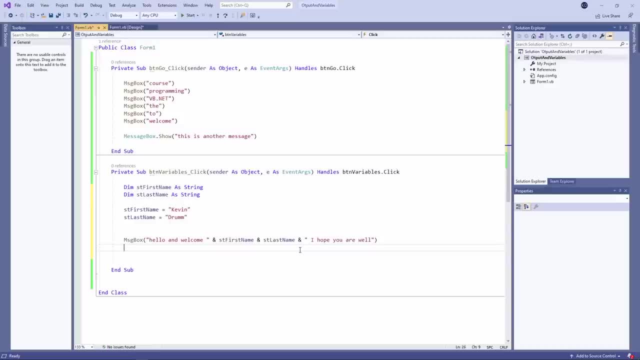 If you have an opening double quote, there has to be a matching closing double quote. If you have an opening bracket, there has to be a matching closing bracket. Let's try this Now. you can see. Kevin drum has come out as one word. 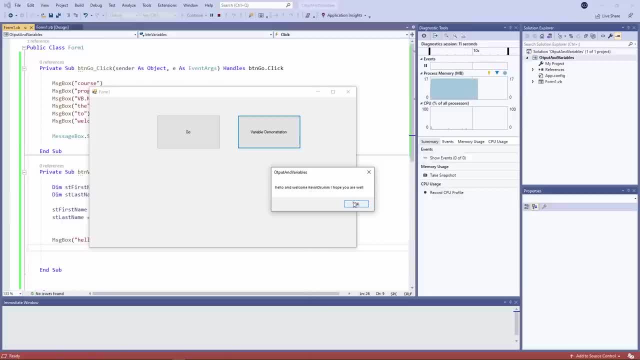 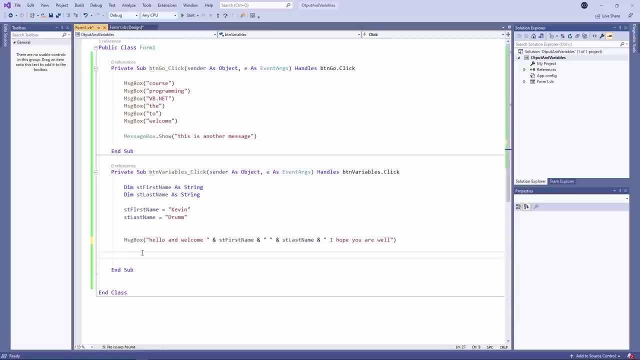 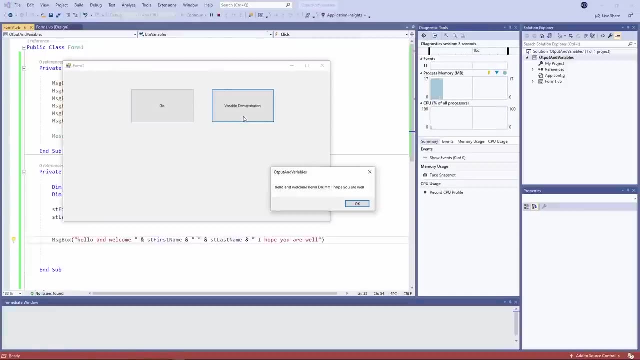 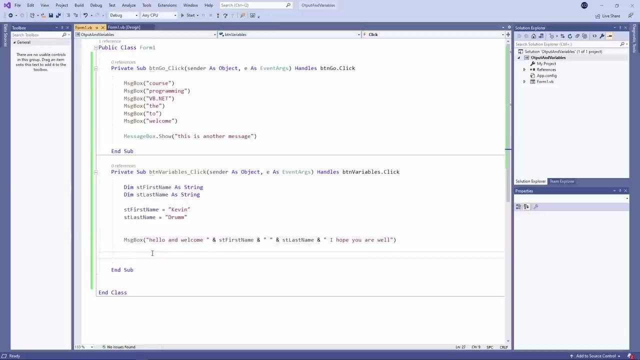 There's no space in between the two. I can fix this easily. I need to concatenate a space in between those two variables. A space is just another character. Let's take a look Much better. Notice that I've put my DIMM statements, my variable declarations, at the top of the 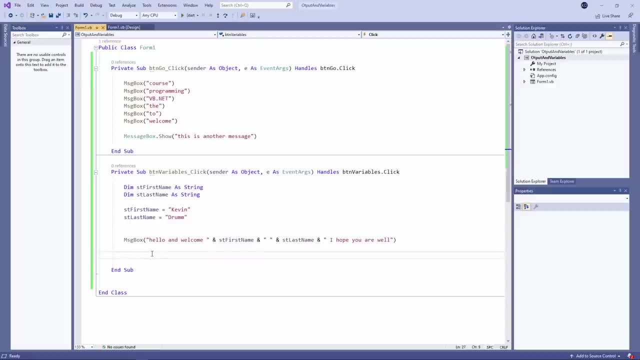 procedure. I didn't have to do this. As long as I declare a variable before I try to assign a value to it, I can put my DIMM statement wherever I like, So, for example, I could declare the last name here and then assign a value to it. 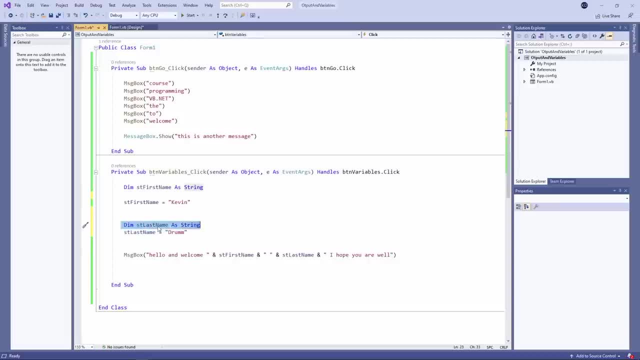 That's absolutely fine. What I mustn't do is try to assign a value to it before I declare it. You can see I have a syntax error. Local variable STLastName cannot be declared. It cannot be used before it has been declared. 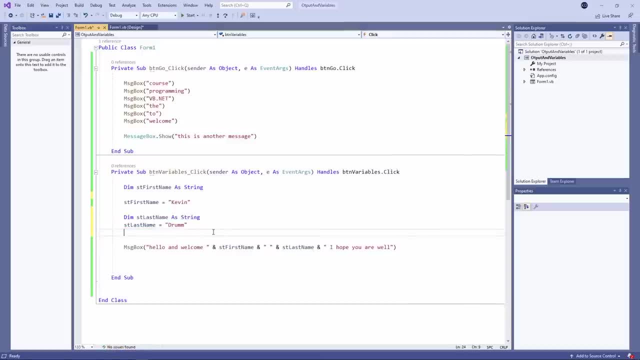 The sequence of operations is important. Although what you can see here is perfectly okay, I like to put all of my declarations at the top of the procedure. Keep them all together. It actually makes the code easier to manage, particularly when you have a lot of code. 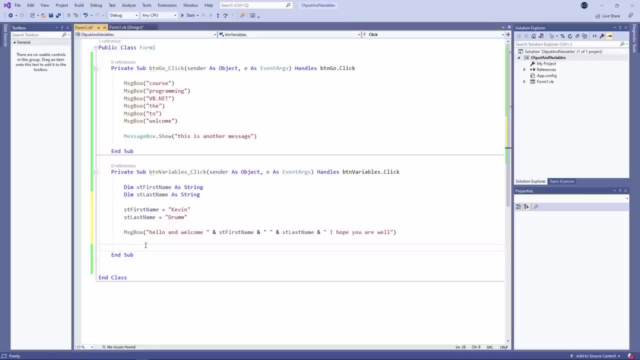 I told you that a variable was a temporary storage location. It can be used while it's running. When this program has done its job and it comes to an end, the memory being used by the variables will be released. It will be freed up for something else to use. 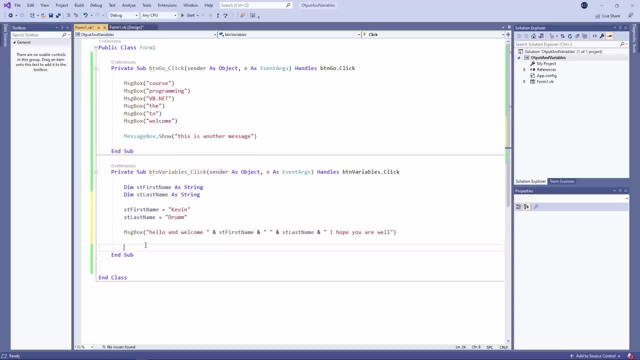 But I can change the contents of the variable while the program is running. That's why it's called a variable. Its contents can vary. So, for example, I can do this. I'm just going to copy these two lines of code, Paste them underneath. 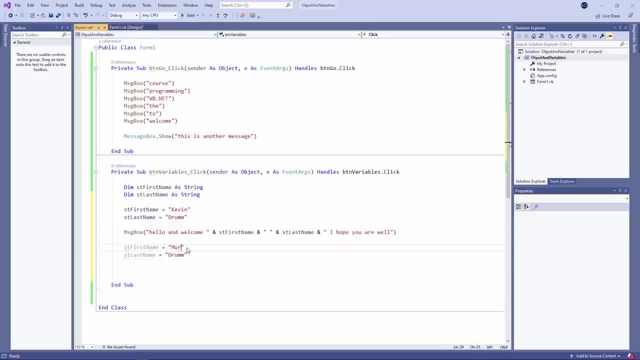 They're still part of the procedure And I'm assigning new values to those variables, which I'll output in the same way as I did before. I can just borrow this line of code and copy it, So watch what happens when I run the program. 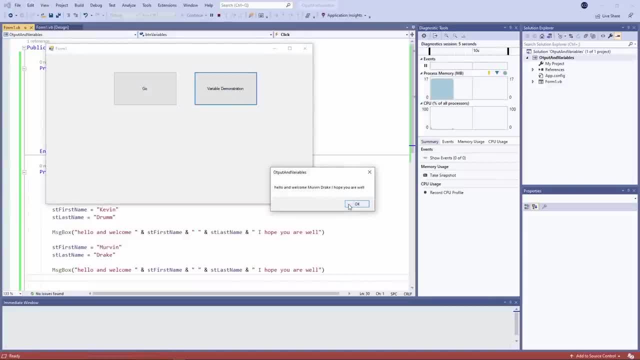 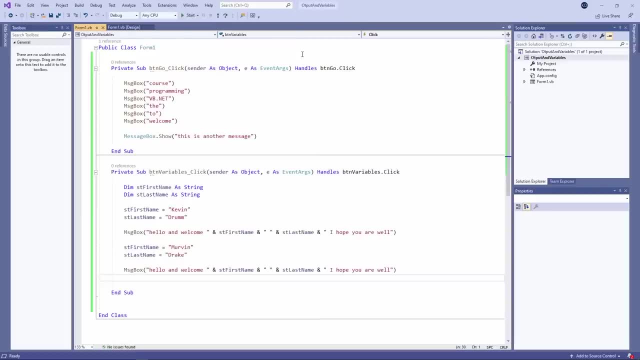 Hello and welcome Kevin Drum. I hope you are well. Hello and welcome Mervyn Drake. I hope you are well. This makes the point that the contents of a variable can change while the program is running. I can assign different values to those variables at runtime. 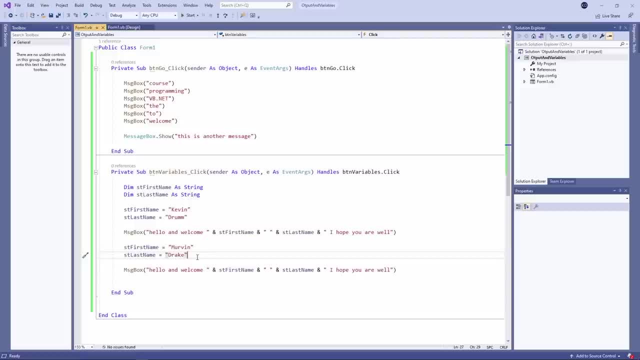 In the next video I'll say more about the different data types that you can use when you declare a variable and what implications this has for your code. Thank you. If you'd like, you can click the link in the description and see the video posted. 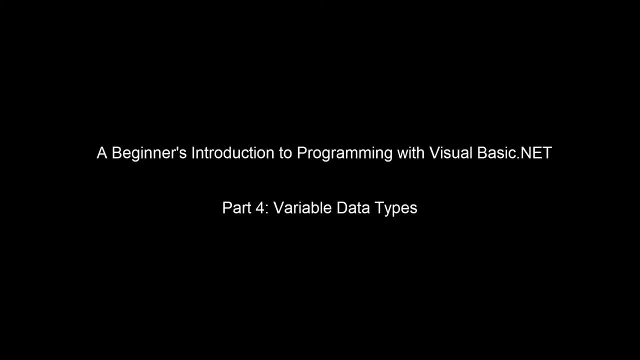 in the next video. In this video, I want to show you how you can convert a variable into a data type with the help of the various types of code you can use. I'm going to store some details about a car. Let's start with a new button on the form. 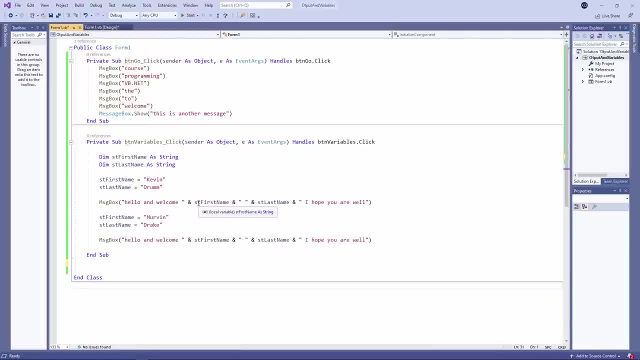 Give it a name and change the text property. Here's the new button On the form. just drag and drop into the ask box. It's in the Swap menu. You can see that this means that you've assigned the car. You can create a new button on the form with the help of the select field. 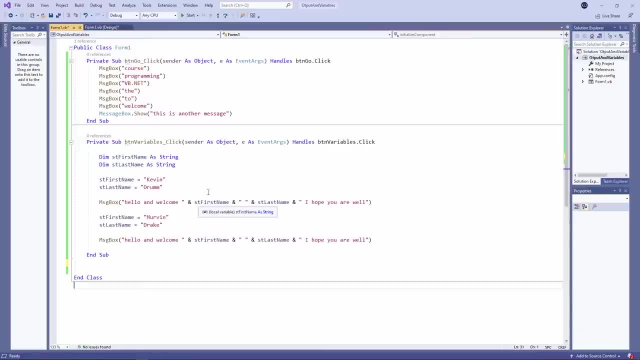 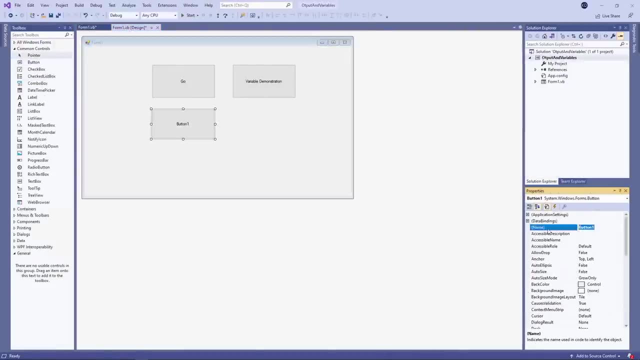 Now I just change this as, apart from the name, I'm going to ask you a question. What's up, Kevin? It's great to have us here, So what do I do? give it a name and change the text property. Double-clicking will allow me. 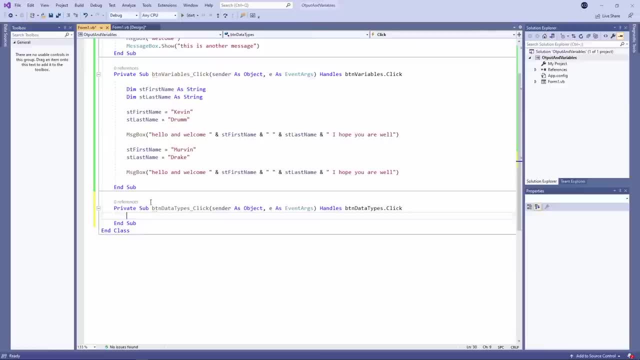 to write the code. Okay, so I'm going to start with a couple of string variables to store the make and the model. We've come across string variables already. Let's assign some values. A Ford Escort, a classic car? I also want to store the. 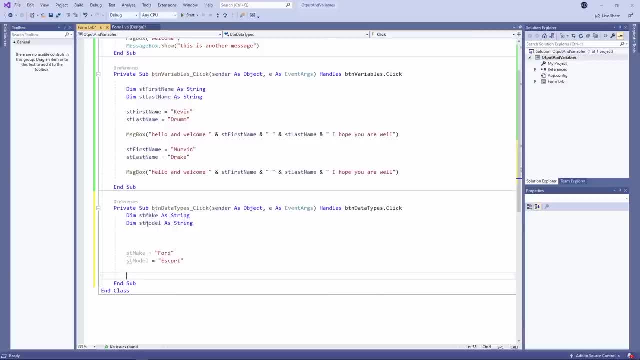 number of doors that this car has. This time I'm using a data type of integer. An integer is just another name for a whole number. Notice the naming convention I'm using: I doors. I for integer. I want to store the color of the car. This is going to be another string. 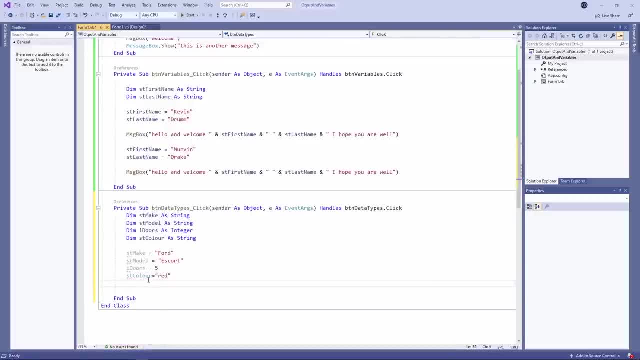 variable, I want to store some information about whether or not this car has been taxed. This time, I'm using a data type of Boolean named after the computer scientist George Boole. A Boolean variable can have one of two values, True or false. This car has been taxed. Boolean variables are good when 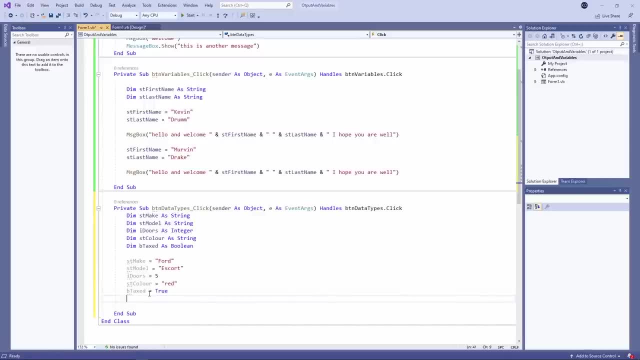 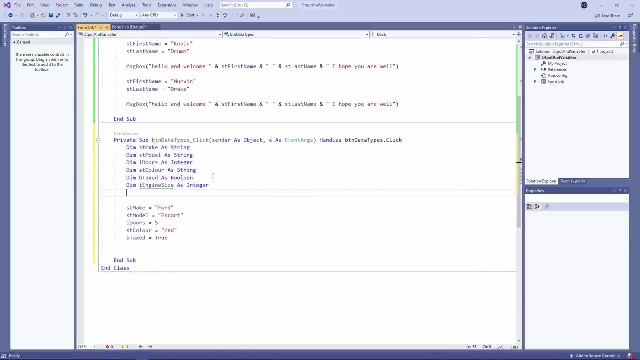 you have yes-no type data, For example, whether somebody is a vegetarian or not, Whether something is switched on or something is switched off. I also want to store the engine size. Another integer: 1,200 CC. I'd like to store the price of this car. I'm using a data type of. 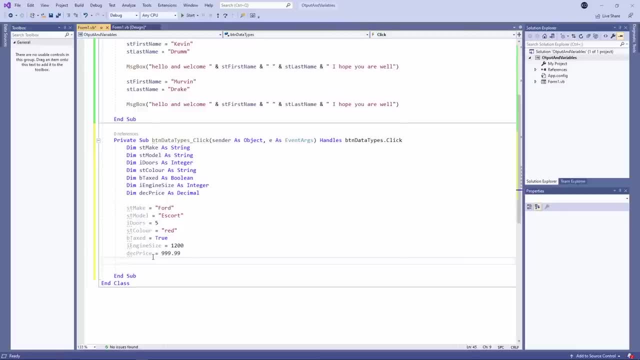 decimal. Decimal is the most suitable data type when you want to store money values. I could have used double and I could have used single, because all three data types Decimal double single. I could have used double and I could have used single, because all three data types Decimal double single. 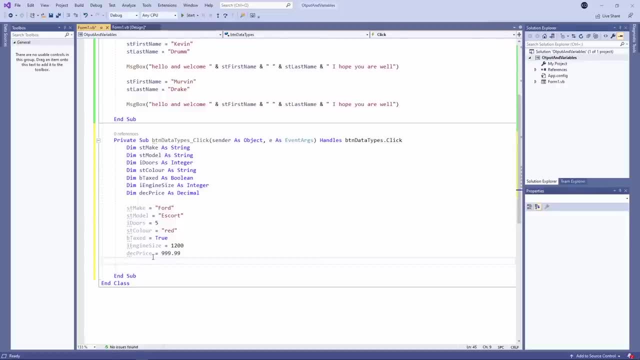 allow me to have a decimal point with decimal places after it, But double is twice as accurate as single. I can have more decimal places And the data type decimal is the most accurate of them all, Which makes sense when you're doing calculations with money. The final thing I want to store is the date that the car 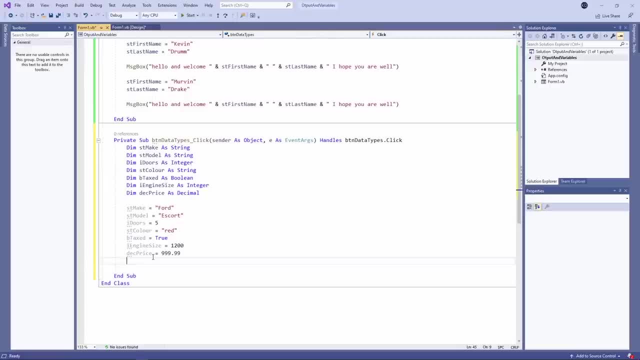 was registered, So I'm going to use a data type of date. There's a special way that I have to assign a value to a date variable. Notice I'm using the hash symbols to enclose the date. I should also point out that this is not the 11th of February, but the 2nd of November. When you type a. 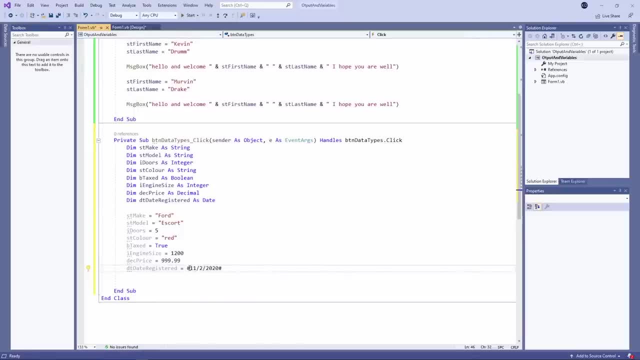 date, you need to type it in American format, which is the month following that date. When you type a date, you need to type it in American format, which is the month following that date, which is the month following that date, by the day followed by the year. 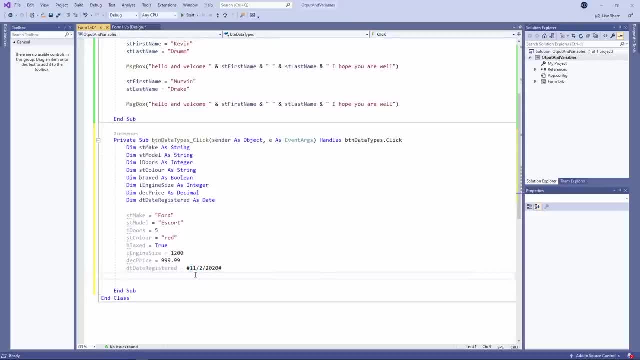 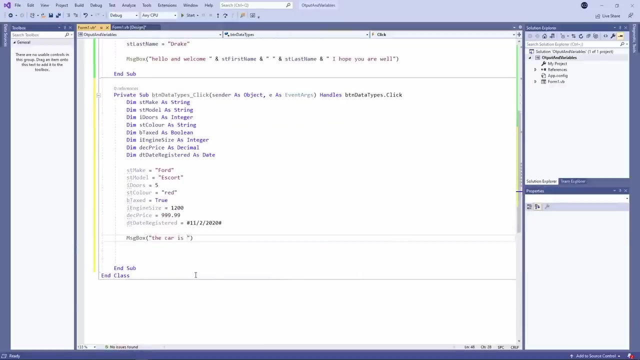 When I display this on the screen, for example in a message box, it'll be displayed according to the settings in my computer's control panel. You'll see in a moment that my computer is set up to display dates in British format. Now let's build a message box command to display all of this data. 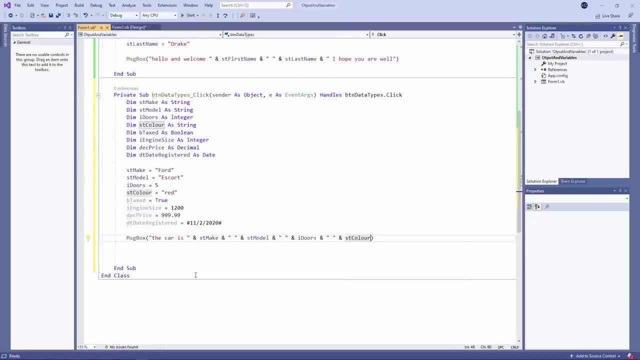 Notice the concatenation operators between the variable names and notice also that I'm concatenating spaces between these data items. OK, Now you can see I have a bit of a problem here with reading the code I've written on the screen. Nevertheless, let's test it and see if it runs. 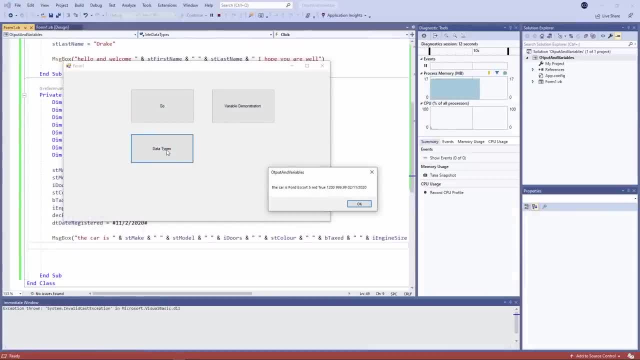 There's my message and it looks OK. Notice that the day and the month of the date are the other way around from the way I coded it. I've written the date in American format, but it's being displayed in British format. What I'd really like to be able to do is display each data item on a separate line. 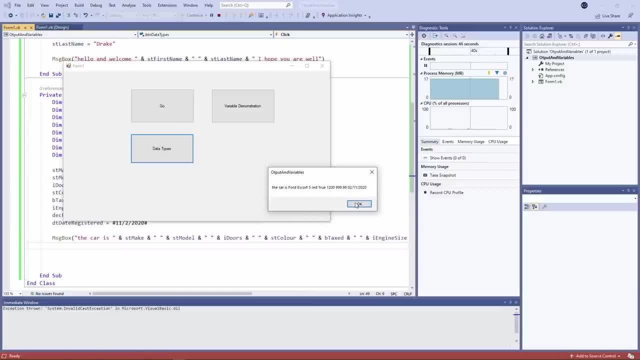 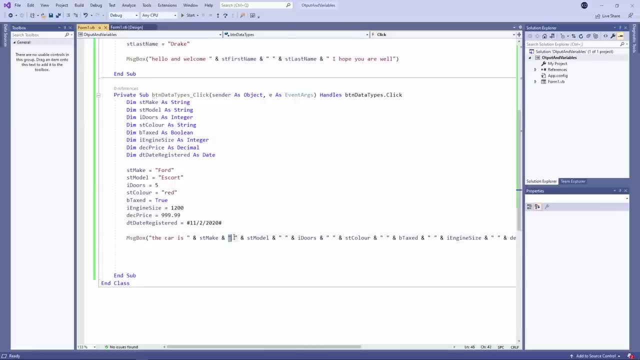 within the same message box. Let's see how to do that. Instead of concatenating spaces in between each data item, I'm going to type a special constant. I'll say more about constants later. Suffice to say, I'm just going to type VBC. 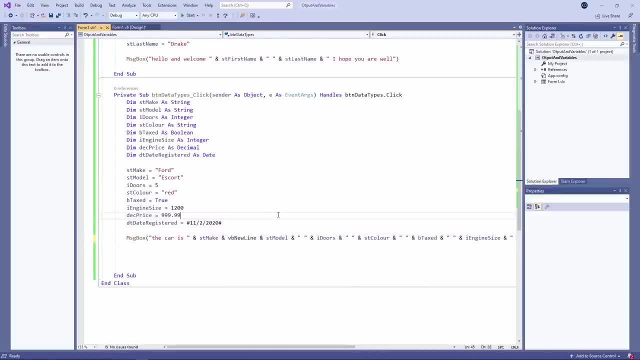 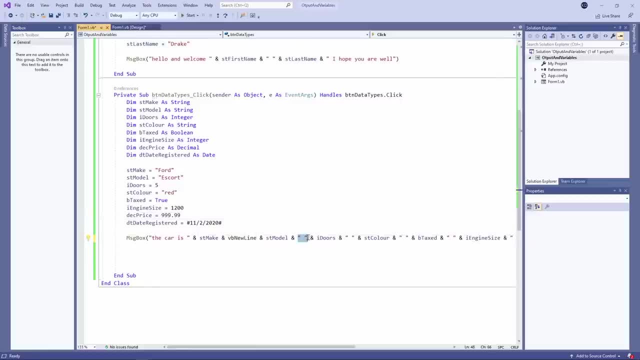 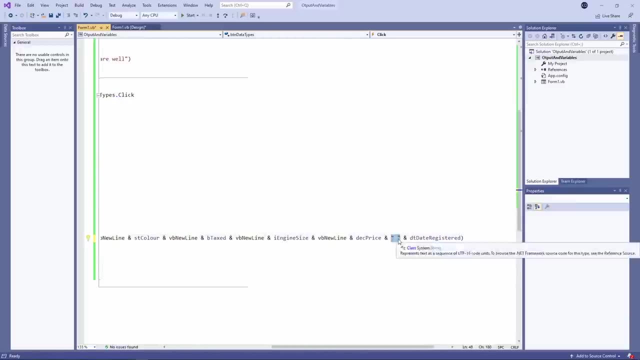 I'm going to type VBC And I'll replace each space with this. Let's just copy and paste it. Control C to copy. Control V to paste. I still need the same number of concatenation operators to join all these different bits. 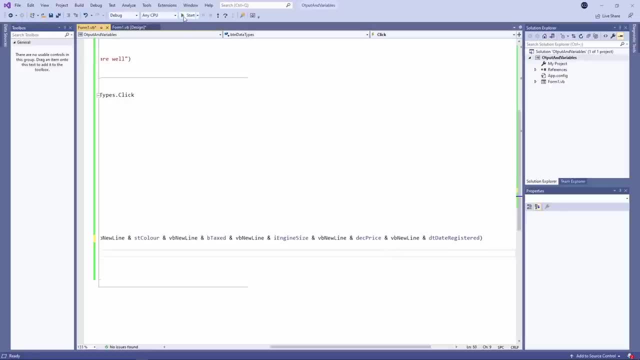 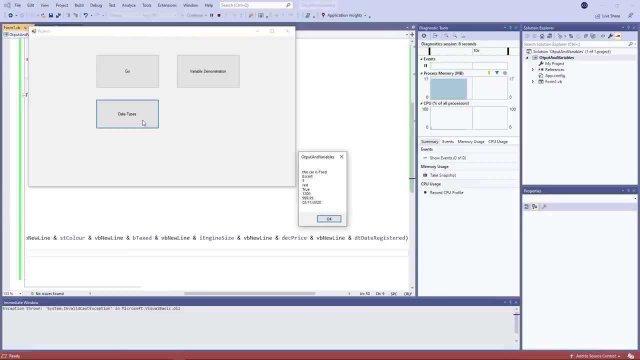 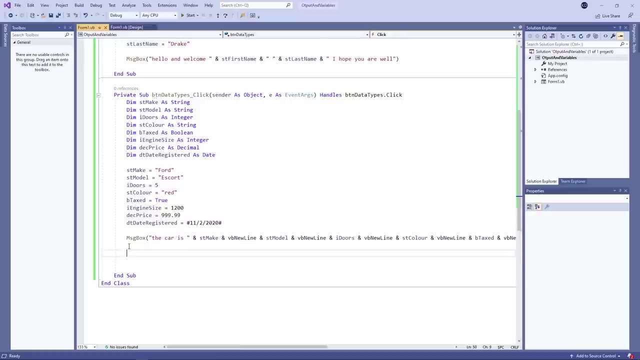 and pieces together. Let's see how it looks now. Well, that is certainly a nicer message, But now I want to do something about the problem that I can't actually read the whole line of code. I could give myself some more space on the screen by just dragging this bar across a. 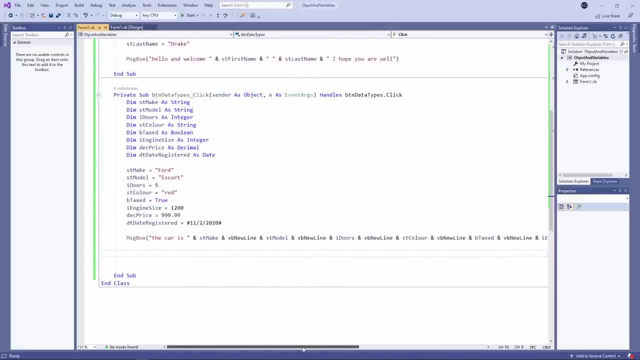 little bit, but even then I can't read the whole line of code. I essentially want to wrap this text on the screen. Well, I can do this Under the ampersand here. in fact, I can put this pretty much anywhere. I'm just going. 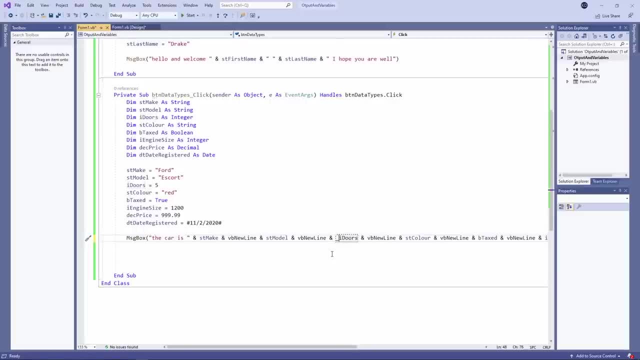 to leave a space and then type an underscore character. When I press enter I've moved the rest of the line onto the next line down. I can do that again here. Notice the underscore characters have actually disappeared, but this is still just one line. 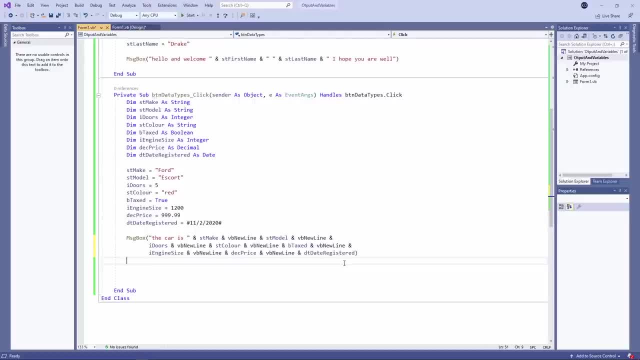 of code. It won't change the appearance of the message box, But it just allows me to read the whole line of code. Let's make sure it still works. Yep, that's absolutely fine. In the next video, I'll show you how we can capture input from the user of an application. 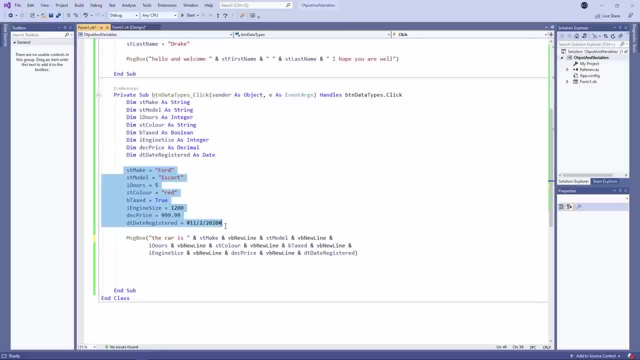 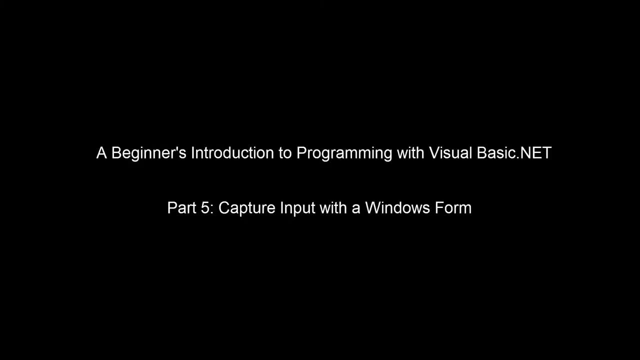 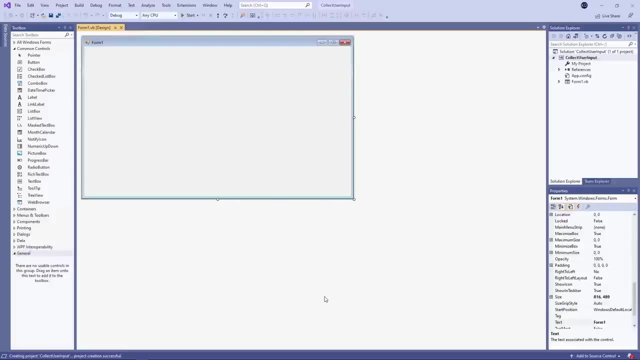 so we can assign the contents of these variables at run time, rather than hard coding the data, like we've done here. I want to show you how to capture input from the user of your application, And I'll be doing it by means of this form. 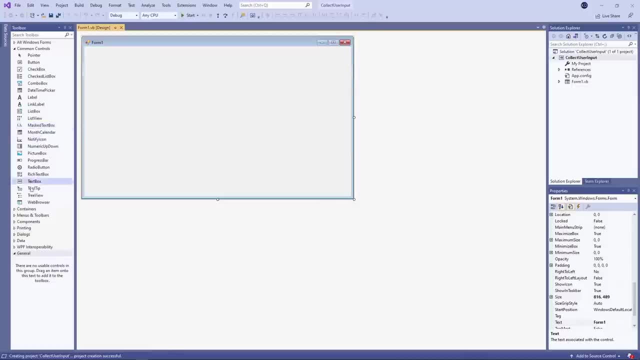 And you'll also see how to use some of these extra controls that we can place onto a form. Before I do, let me just show you a quick and easy way we can capture input from the user by means of the input box function. I'll drop a button on the form first. 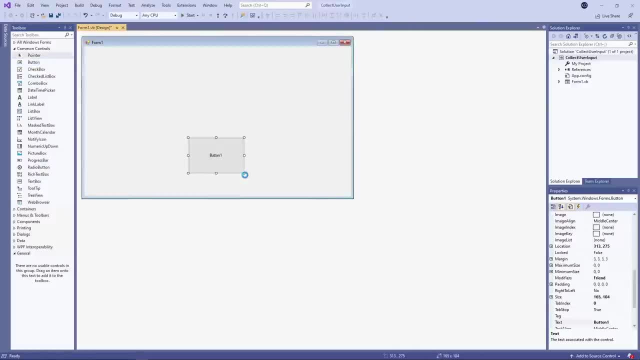 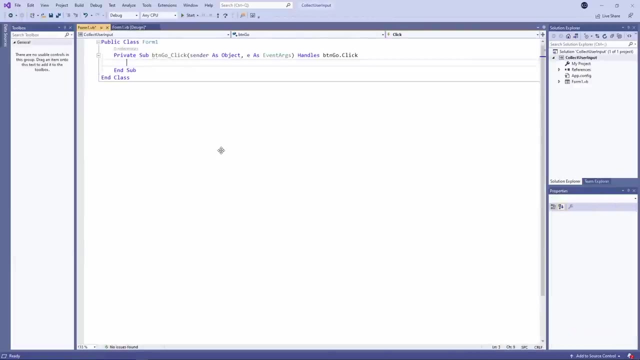 I'll press enter. That's it. Give it a name and a text property. Double click to write the code. The input box function will capture one piece of data. Specifically, it'll capture a string. I'll need a variable to put that piece of data into. 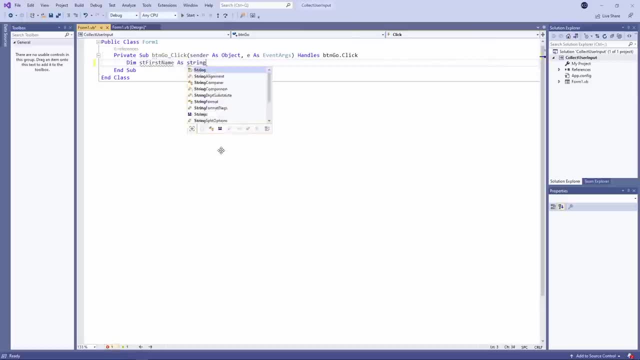 So let's declare a string variable first of all, And then I can assign a value to it by means of the input box function, just like this. And to prove it works, I'll output the contents of that variable. I'm concatenating the word hello in front of it. 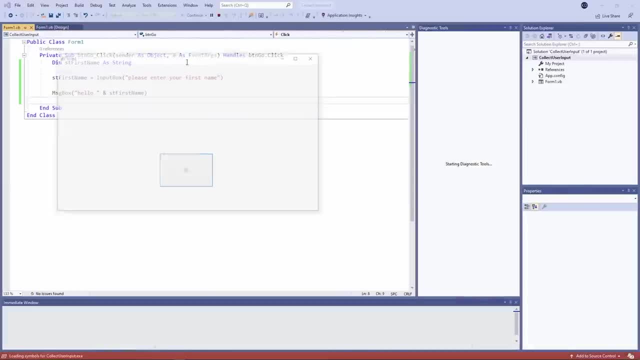 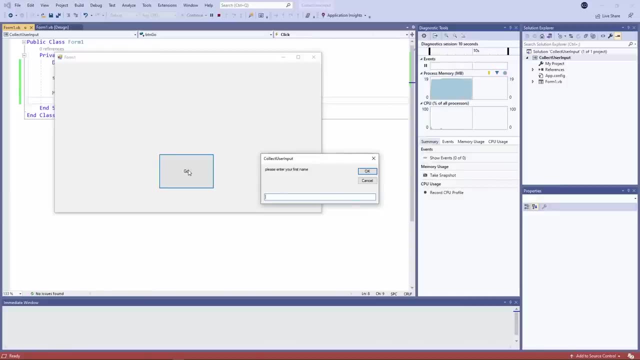 Let's give it a try. Press the button to launch the procedure And there's the input box prompt- Please enter your first name. And that's working fine. So it's a very simple procedure. It's just a few simple steps. 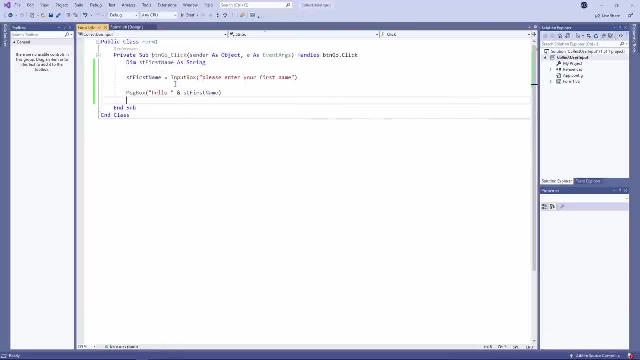 It's a quick and easy way to prompt the user for some input, But what I really want to talk about in this video is how we can use controls on the form to capture input. So I'm going to delete the code you can see here and do something else instead. 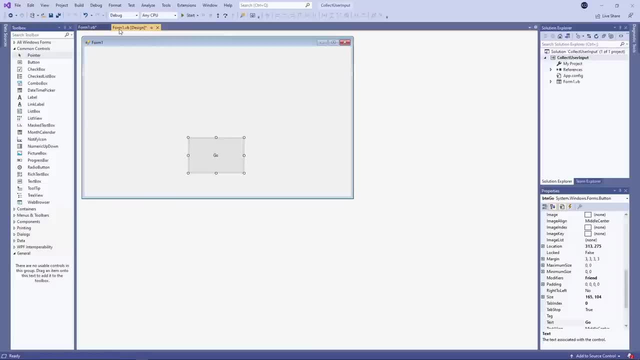 Let's go back to the form. I'm going to place a text box on the form. Here it is in the control toolbox. I'll give the text box a name. Notice. at the moment it's called text box 1.. I've prefixed the new name with txt to indicate that it's a text box. 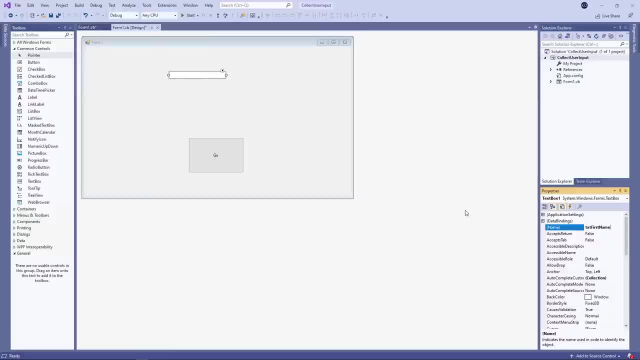 And then I'm calling it first name because that's the data I want to capture. I'm trying to keep the name meaningful. Notice the camel notation as well. You'll see the benefit of doing it this way. in a few moments I'm also going to put a label on the form so that the user of the form knows what the 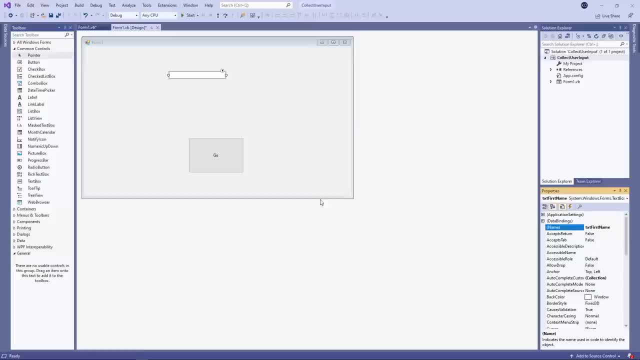 name is Notice what to type into the text box. Here's the label control, And again I'm going to change its name to keep it meaningful: LBL for a label, and then something to indicate its purpose. A label also has a text property, which I'm going to change. 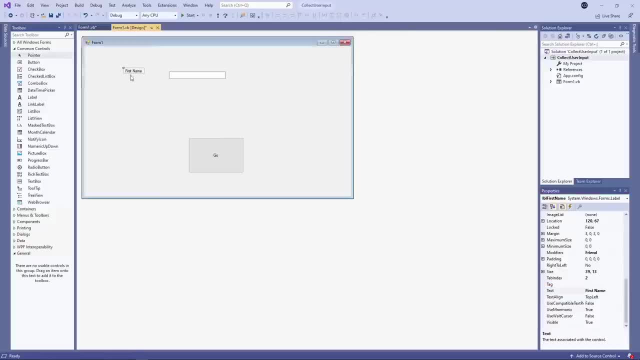 And you can see. that is what appears on the form. While I'm at it, I'm going to change the text. Once I'm at it, I'm going to add another text box to capture the user's last name And a matching label. 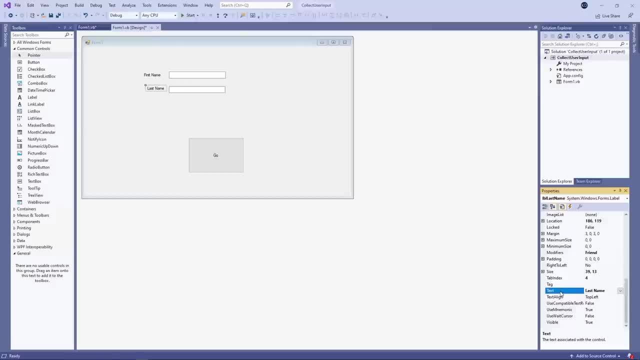 And one more text box to capture the user's gender. Notice that a text box also has a text property, But anything I type in here will actually appear in the text box. It will become the default data if a user doesn't type something into the text box. 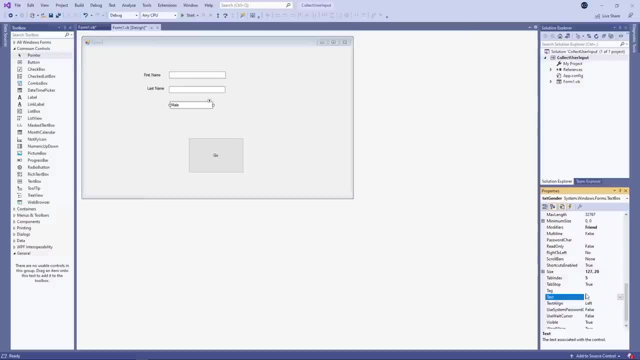 I'm going to leave it blank And we'll have another matching label to go with this text box. There are a couple of things you need to be aware of when you're placing controls on the form. Each control must have a unique name. 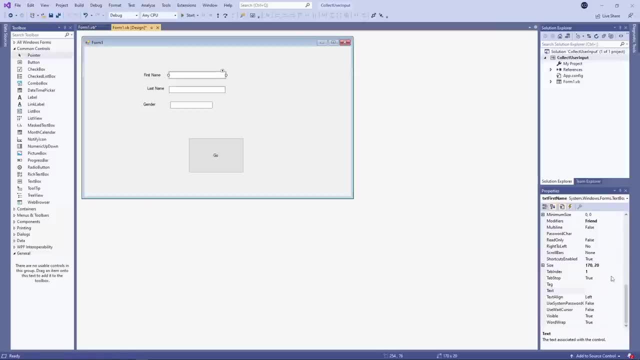 So this one, you can see, I called it TXT, first name. There's the name property, And this one I called TXT, last name. Let me just make the mistake of giving this text box the same name as the other one, and see what happens. 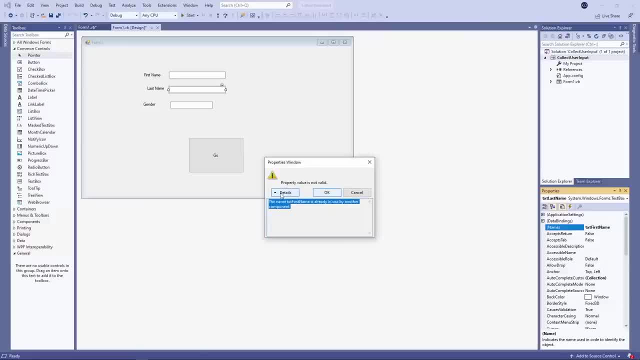 Property value is not valid, So I'm going to change the name. Take a look at the details And it's telling me that the name is already in use by another component. Something else on the form has already been called TXT first name. 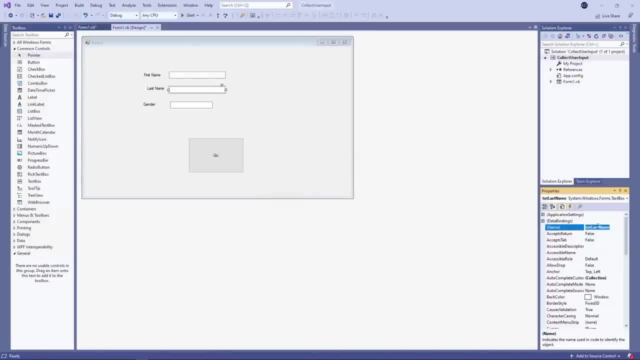 If this happens, just cancel And find out which one is the offending control. Something else I should mention is you can't have spaces in a control name, So let's put a space in this text box name. Again, an error message, And maybe I'll even try to change it. 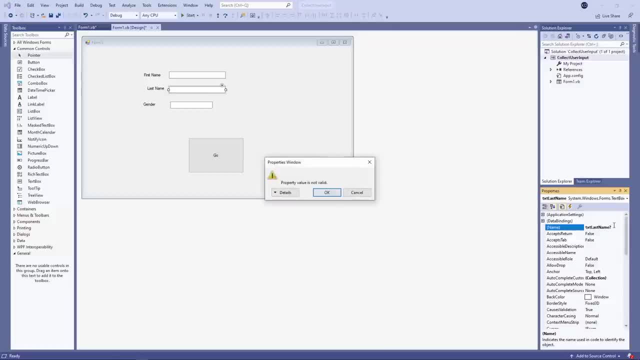 Maybe I'll even try putting a question mark on the end of the name. Another error message. So there are some limitations as to what you can call a text box or indeed any other control on the form. The text property, on the other hand, of a label or a button can be pretty much anything you. 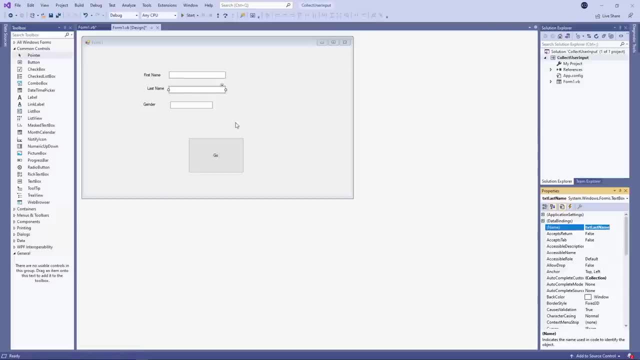 like: OK, Let's just tidy up the layout a little bit. I'm watching the guidelines for assistance And you can also use the format menu To help you control the layout of a form. See, I have options for alignment, horizontal and vertical spacing. 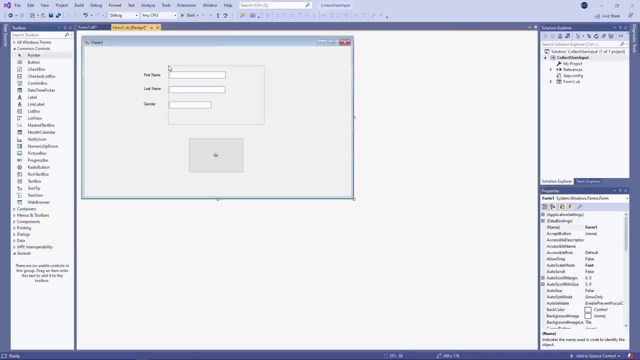 This one is particularly handy. If I select all of these text boxes, I can say I want to make them all the same width, for example, And I can make them all the same height. If I want to move things around as a group, I just draw a box around them to highlight. 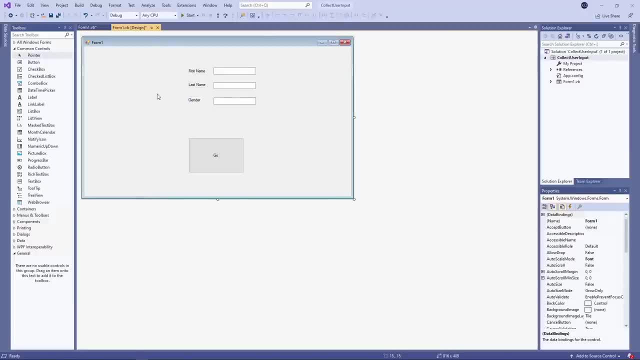 them, Or I can drag them to a new position. You can play around with the various tools available to improve the cosmetic appearance of your form when you have time, But for now I just want to show you how we can capture some data. So let's write the code for the button. 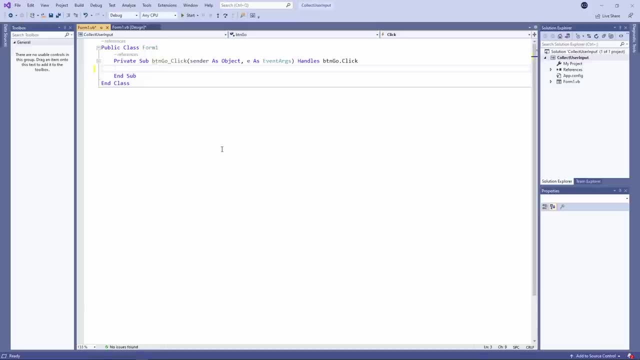 I'm going to start by declaring three variables into which I'm going to load the data that I capture. I'm using a standard naming convention, again st, because these are string variables. and then, of course, something meaningful in camel notation. I've just spotted a spelling mistake as well. let's fix this. 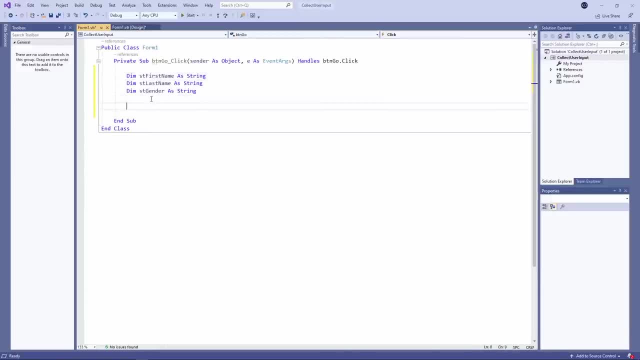 Now I'm going to take the information that the user types onto the form and load it into these variables, Starting with the first name. stFirstName equals. a single equal sign means I'm about to assign something to this variable And the information I want is on the form, in a text box called txtFirstName. 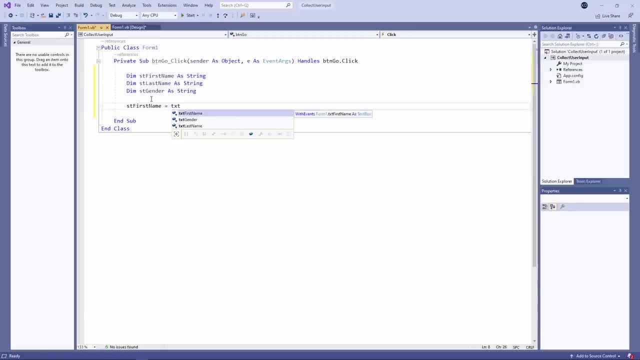 I've just typed the first three characters of the text box name, txt, and I'm being presented with a list of the text boxes on the form. You can see why I use this naming convention. As long as I make sure that all of my text boxes begin with txt, I'll get a nice little. 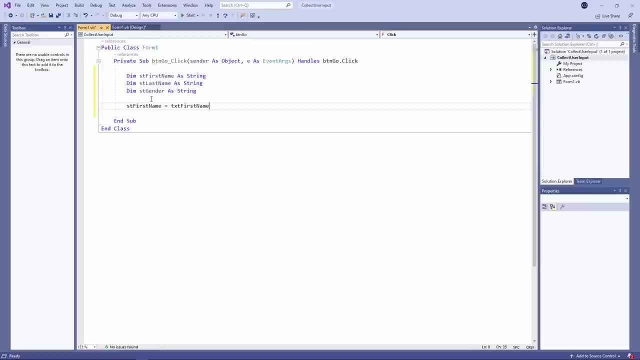 list of them. So I'll select txtFirstName and I want to take the text property, in other words the text that the user typed into that text box, and I'm going to load that into my variable. So this reads as: take the text from the text box called txtFirstName and assign it to that. 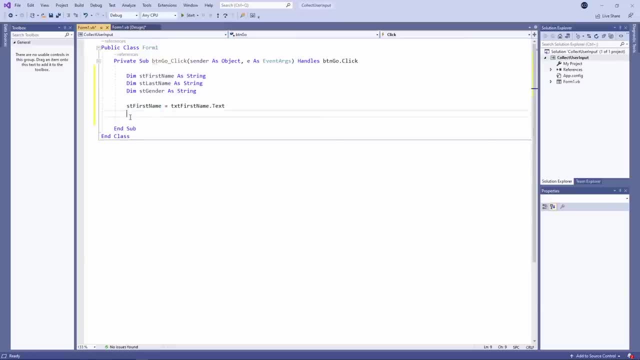 variable. So that's it. Let's do the same with the other variables And, finally, I'm going to output the data in a message box. just to make sure it worked, I've included a space between the first name and the last name. 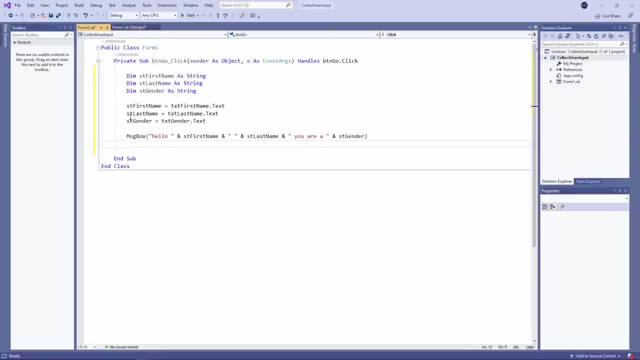 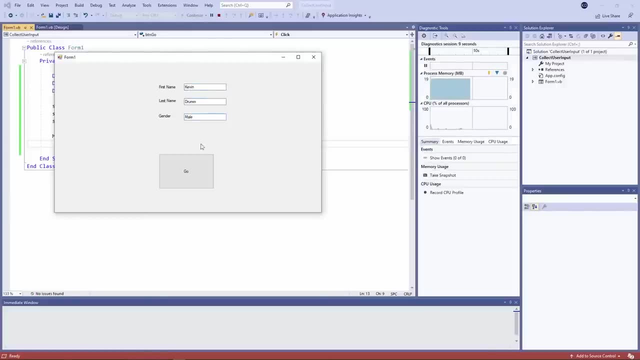 And I've concatenated some extra text in my message as well. Let's see what happens. Type in some information And there's the output from my procedure. If I dismiss the message box, the application is still running, So I can change the data here. 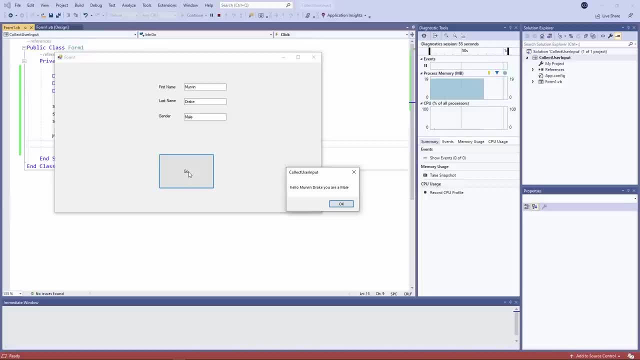 The program is assigning new values to those variables, overwriting the existing ones One more time. And there's the output from my procedure. If I dismiss the message box, the application is still running, So I can change the data here, Type in some information. 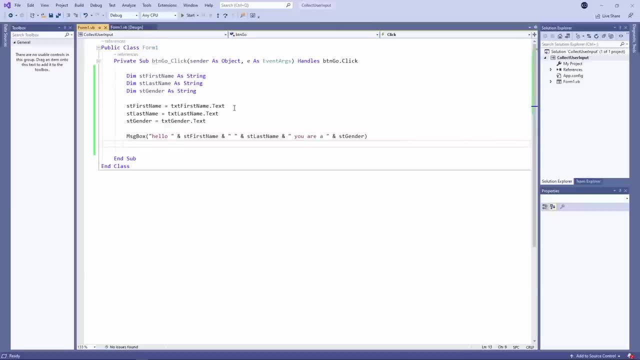 And there's the output from my procedure. And there's the output from my procedure. So there you have it: Capturing data from a user by means of text boxes on a form. Let's quickly take a look at another control which I can use on a form. 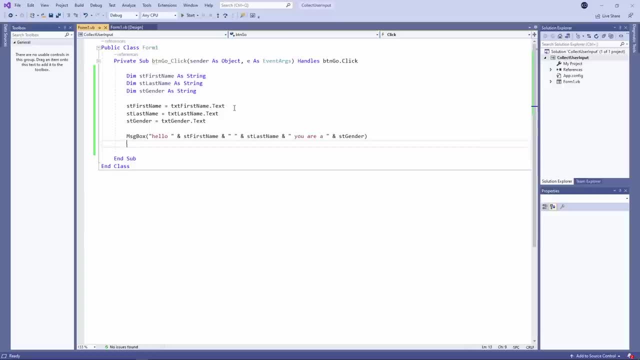 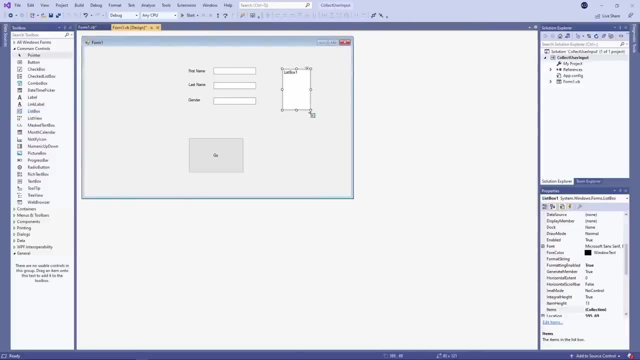 I want to show you a list box And I'm going to use this to capture the user's occupation. So let's give it a name LST, Occupation LST, because it's a list box. I'll put a label on the form to go with it so that the user knows what the list box. 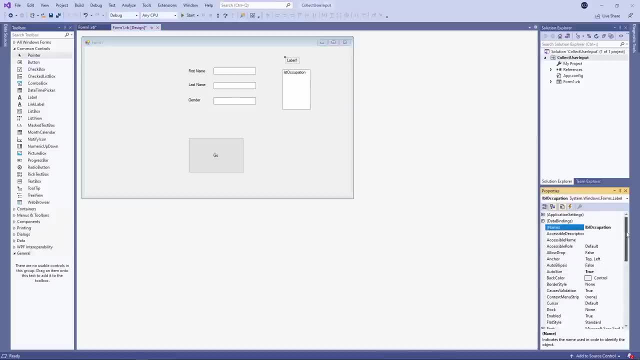 is for, And I'm going to include some occupations in the list box that the user can choose from. First of all, make sure that the list box is actually selected, And then use the items property. There's a little button here which will allow me to add a collection of items. 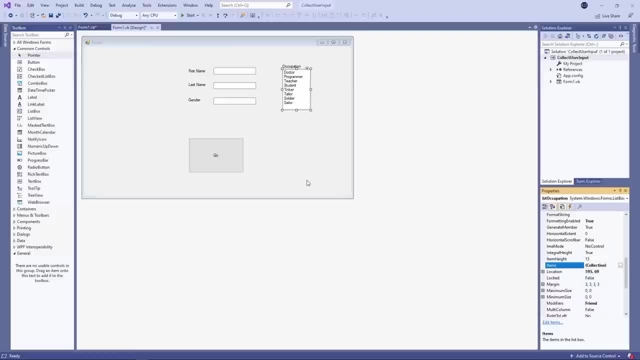 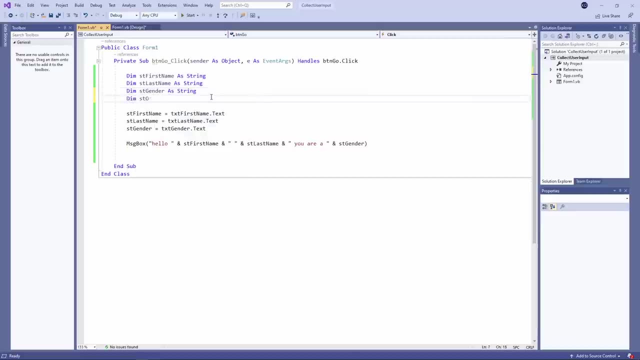 Click OK and I now have a populated list box. Let's capture the user's selection. I need a variable To store it in And I can capture the user's selection in a slightly different way. I'm using the selected item property. 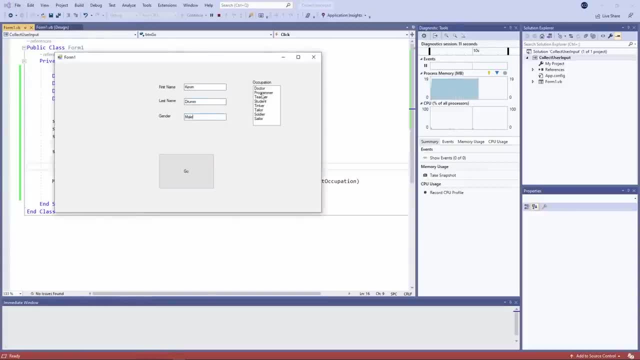 Let's try it out. Hello, Kevin Drum, you are a male teacher. I can also add items. I can also add items to the list box programmatically, In other words, in my code. I'll quickly show you this and then you can experiment with it yourself. 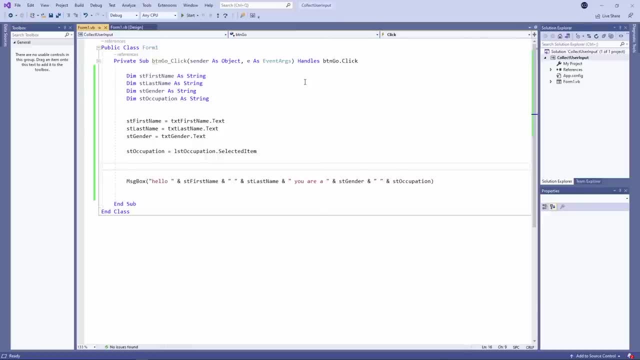 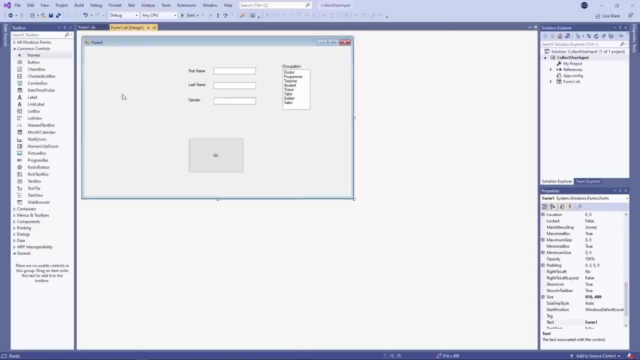 You might remember, in an earlier video I showed you how you could write code when the form loads. I'm going into the form design environment and I'll double click the form itself. I now have a procedure called form one load. I'm going to create a new form. 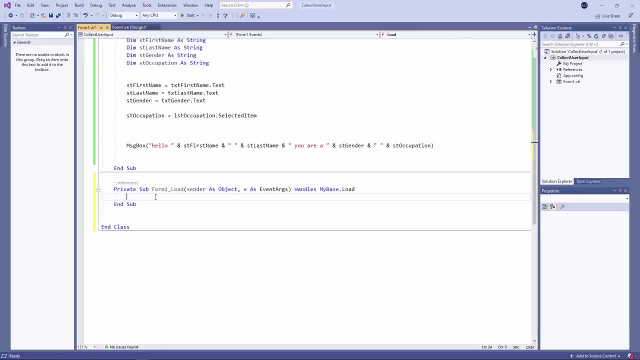 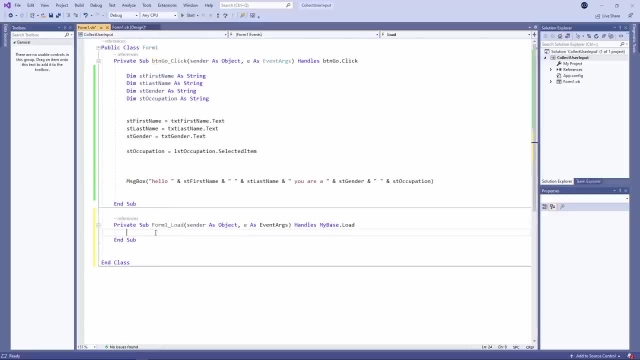 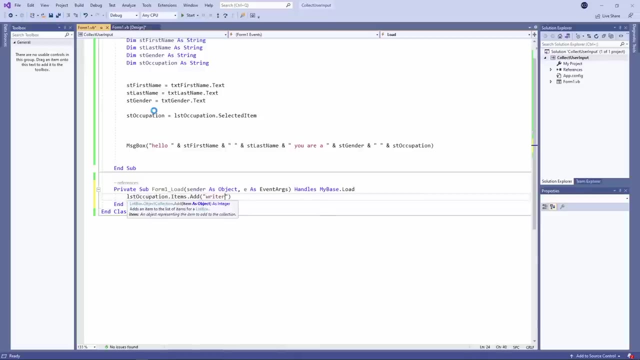 I'm going to create a new form. I'm going to create a new form. The form right here will run immediately after I start the application, but before the form appears on the screen, And I'm going to add some extra code to put a few more items into my list box. 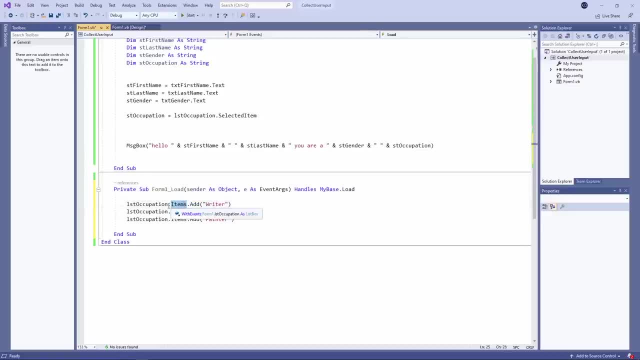 I am adding something to the collection of items. I'm going to add something to the collection of items. I'm going to add something to the collection of items. I'm going to add something to the collection of items. I'm just going to make sure that the listbox is big enough to display everything. 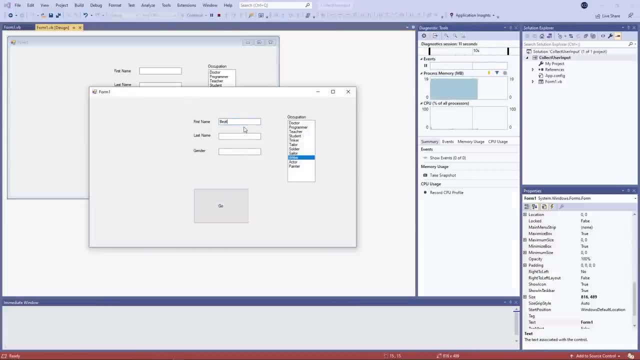 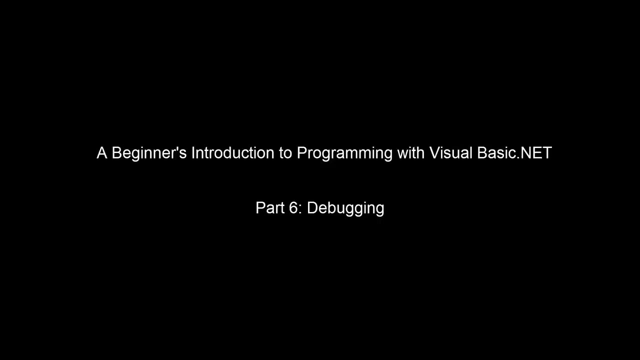 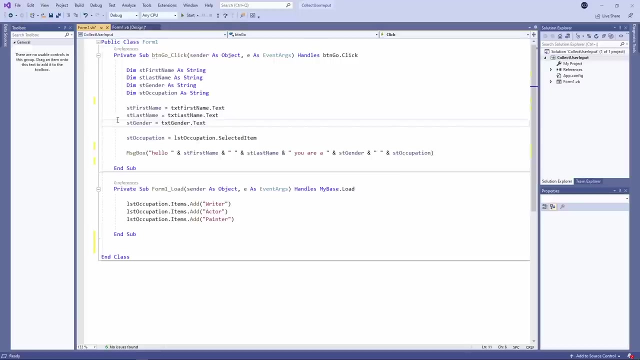 Let's give it a try. Hello, Beatrix Potter, you are a female writer. I'm going to add something to the collection of items. Before we look at some more code, I want to introduce you to some of the facilities that come with Visual Studio for debugging your code. 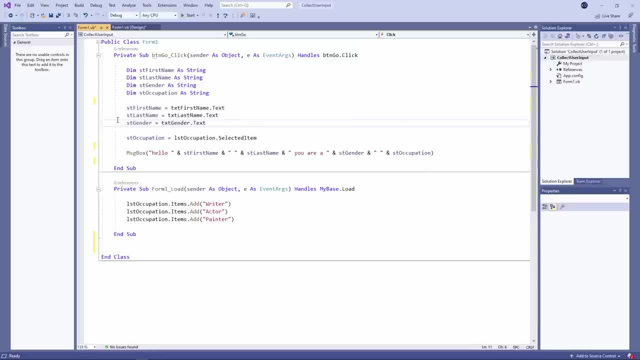 In other words, tracking down errors in the code. The first and probably most useful one that I want to talk about is being able to set a breakpoint and then step through the code. I can set a breakpoint by clicking on the grey bar here. 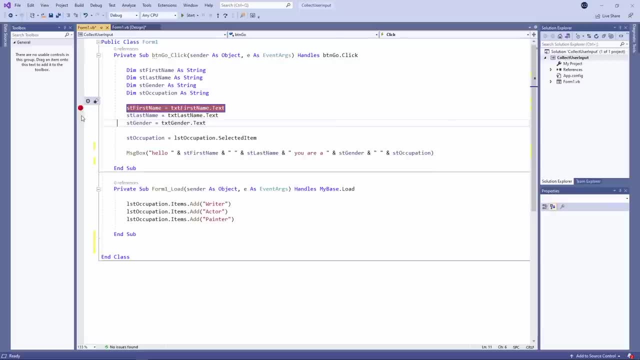 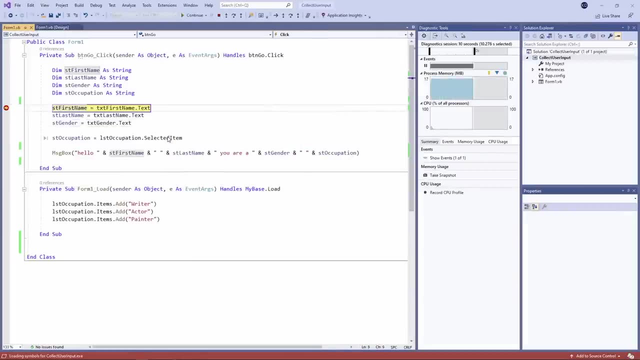 That's a breakpoint. Now I'm going to run the program, watch what happens. I'm now in what's called break mode or debugging mode. My application ran at full speed until it came to the breakpoint, and now it's suspended and I can step through the code once. 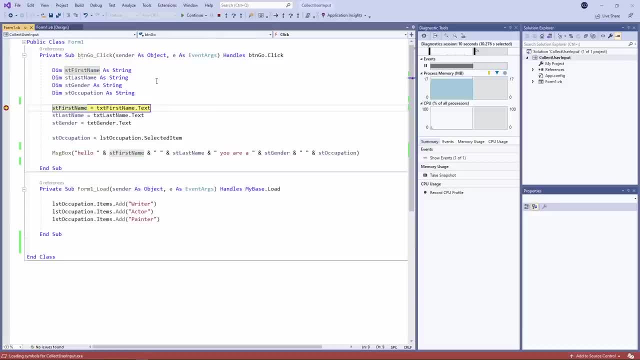 One line at a time. There are a number of buttons I can use to do this Up here: Step into, step over, step out. I'll say more about these two later. The most useful one is step into Notice. I can also use the function key F8 to do the same thing. 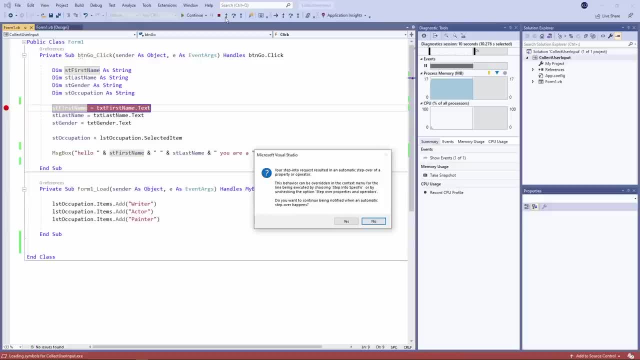 So when I click the button, I'm getting a message about how the stepping facility will behave. I'm not too worried about this for now. I'm just going to say I don't want to see these messages again. It's highlighting the line of code that it's about to execute. next, 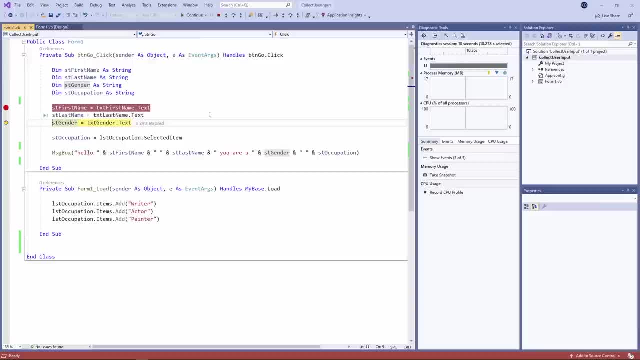 And now it's about to execute this line of code. And again it's about to execute this line of code. When I'm in debug mode, I can hover over the name of a variable to see its contents, So I can see that the string mail has been executed. 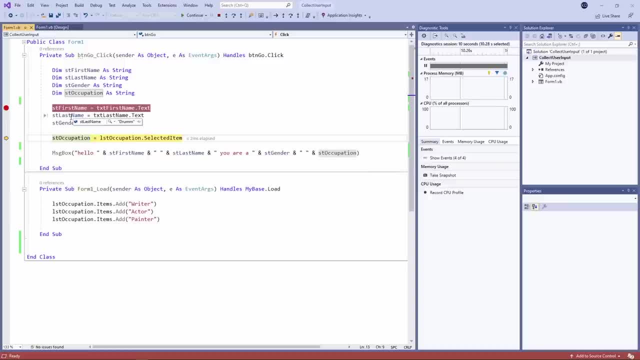 And I can see that it's been assigned to this variable. Drum has gone into this one And Kevin has gone into that one. If I take a look at this variable, it hasn't been assigned a value yet because this line hasn't executed yet. 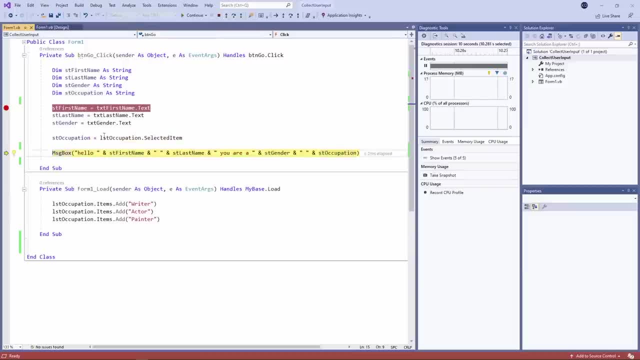 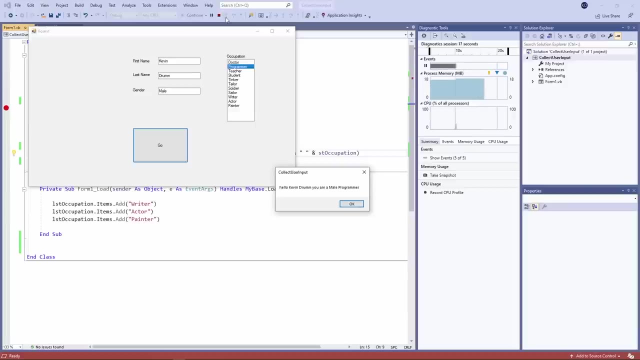 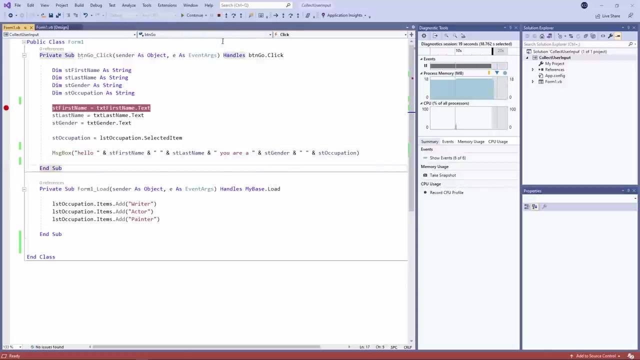 Let's continue stepping, And I can see there's something inside that variable. now The final line of code in this procedure will do some output, So I've been switched back to the user interface And finally the procedure will come to an end. 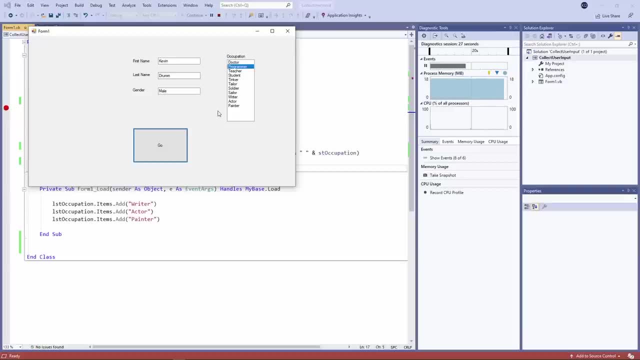 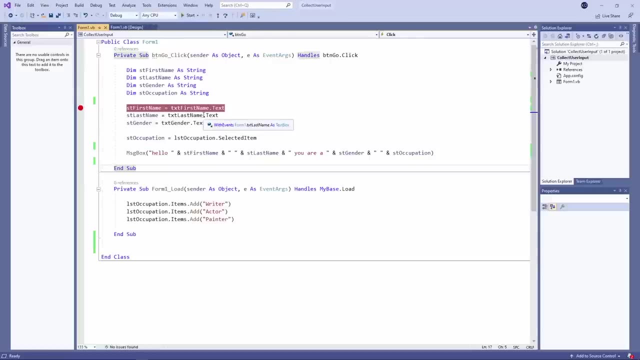 My application is still running. The form is still on the screen, But the procedure which I launched when I clicked on the button has now finished. I can use as few or as many breakpoints as I like. I'm going to remove this breakpoint just by clicking on it. 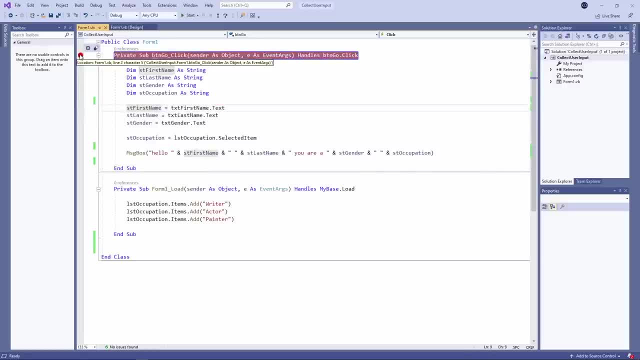 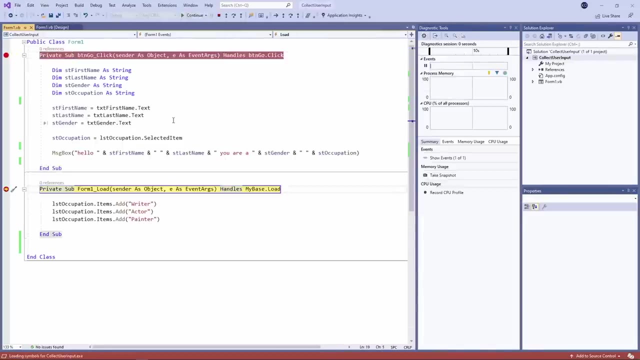 And I'll place a breakpoint here instead. I'm also going to place a breakpoint on the form's load event handler. Let's run it again. As I told you in the previous video, when you launch a Windows Forms application, the form is loaded into memory before it hits the screen. 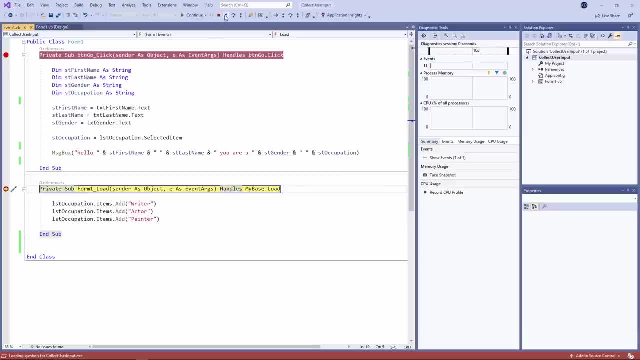 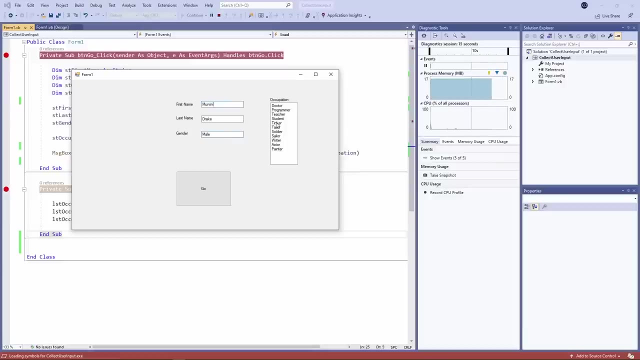 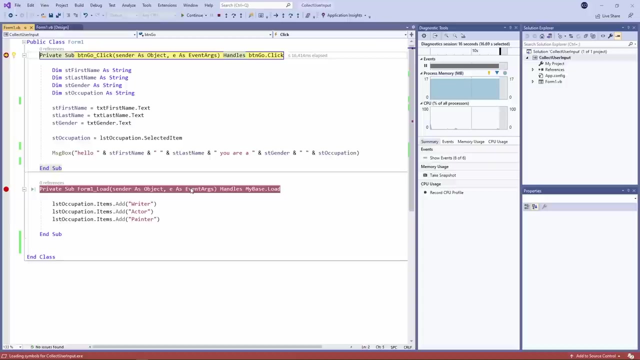 So the form's load event handler is running first- I'll step through that- And it's populating the list box. When that's complete, the form can hit the screen And clicking the button causes the button's click event handler to start running. 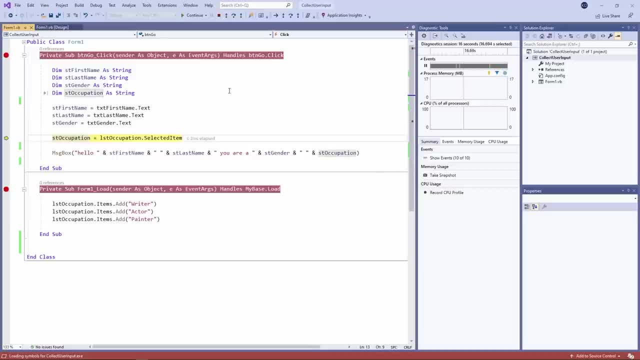 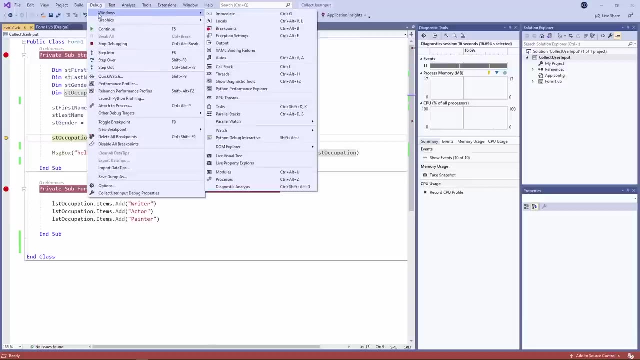 And we've seen this before. When we're in debug mode, there's some extra windows that you might want to switch on. A particularly useful one is called the Locals window. You can find it here on the Debug menu: Debug Windows- Locals. 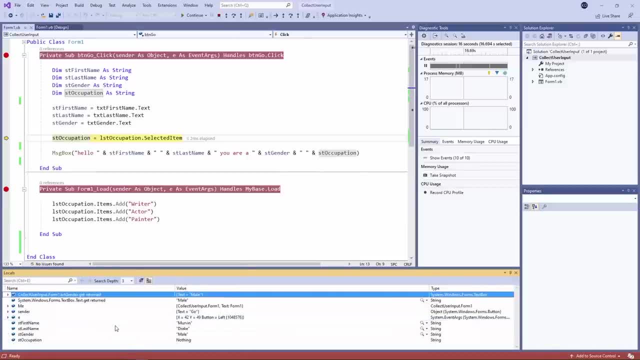 What it's showing me is the contents of any local variables, In other words variables which have been declared within this procedure. I'll say more about the difference between local and global variables later on. Suffice to say, for now, this is an alternative way of finding out what's inside a variable. 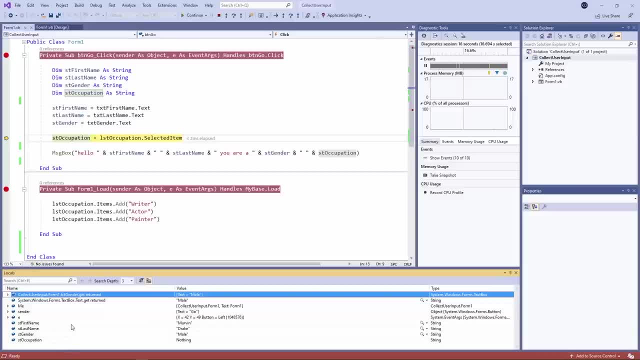 I can see a nice summary down here. There's additional information in this window as well which pertains to these parameters which I mentioned in another video. We'll say more about these later. With the Locals window, I can actually change the contents of a variable on the fly, as. 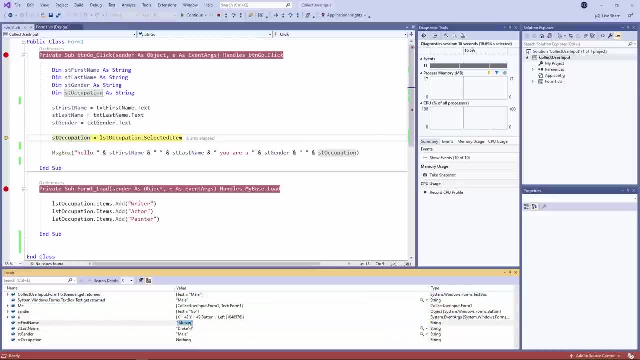 it were. I just double-click it here and re-type it. I've overwritten the existing value of that variable. If you've finished stepping through your program, you can stop the execution just by clicking on this red square, Or you can press Continue and it will jump you straight to the next breakpoint, if there 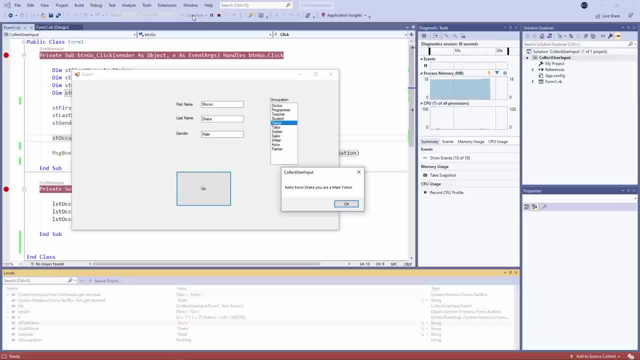 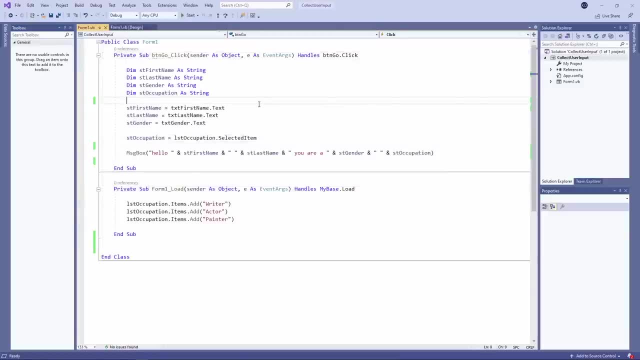 is one. At this point, I just want to return to a type of error that you've seen already, And that's the so-called syntax error. For example, if I misspell the word Text, I type Text on the end, I've got a red wavy line. 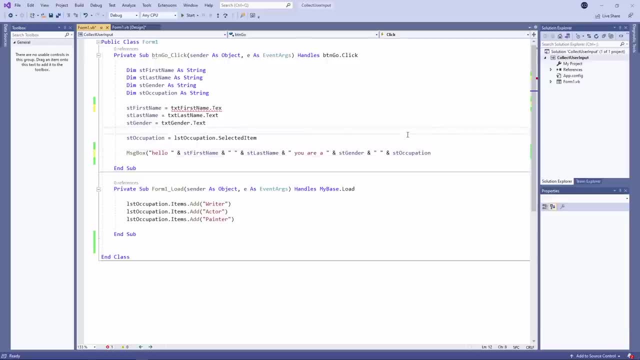 If I open a bracket but forget to close it again, that's a syntax error. I can see a red wavy line on the end of this. Keep an eye out for these, because your program won't run properly If you don't fix them. 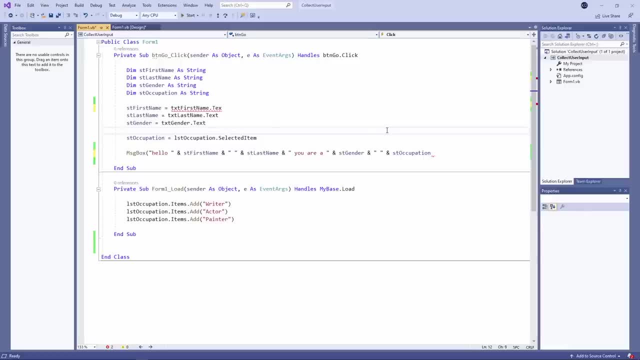 I like to fix them as I go along, But let's see what happens when I try to run a program which has got syntax errors like this in it: There were build errors. Would you like to continue and run the last successful build? Well, that begs the question: what does it mean by build? 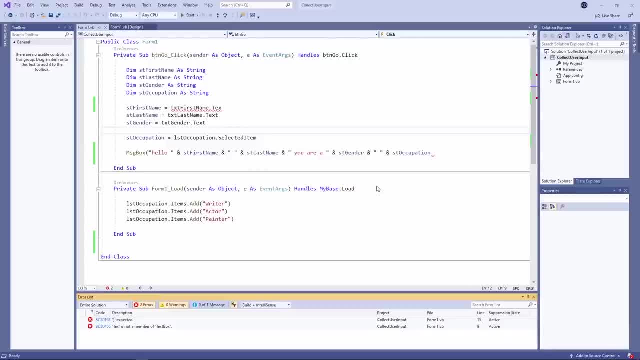 So let's say no And I'm going to switch on something called the Output window. Let's see what happens when I try to run the program again. Watch what happens when I try to run the program again. Build- 0 succeeded- 1 failed. 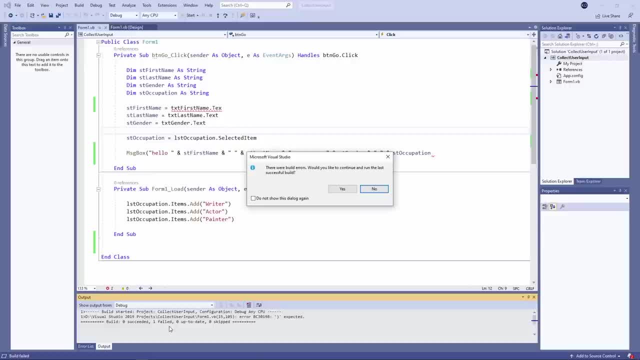 This tells us something very important about VBNET programs. When you write a program, you're writing source code, Code that a human being can understand. But before you can run a program, it has to be compiled. What that means is it has to be turned into machine code- binary 1s and 0s- that the computer 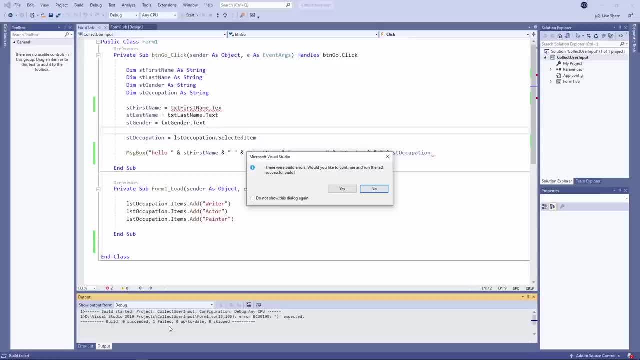 can understand, When you press the start button, Visual Studio will automatically try to compile the program first. Another name for compiling a program or compilation is to build the program. So you can see here: The program has failed to compile, The build failed. 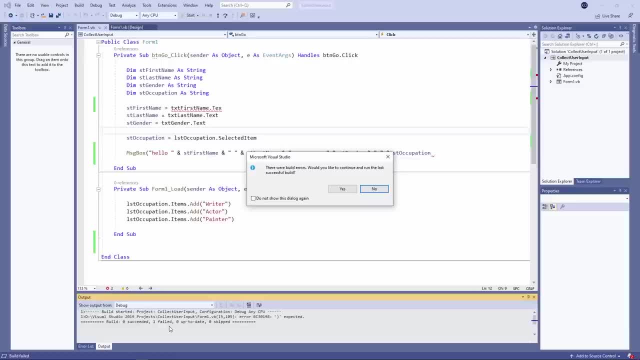 And I'm very kindly being asked: would I like to use the last successful build? Would I like to run the version of the program that compiled successfully previously? Well, in this case, the answer is no. I want to fix this version of the program. 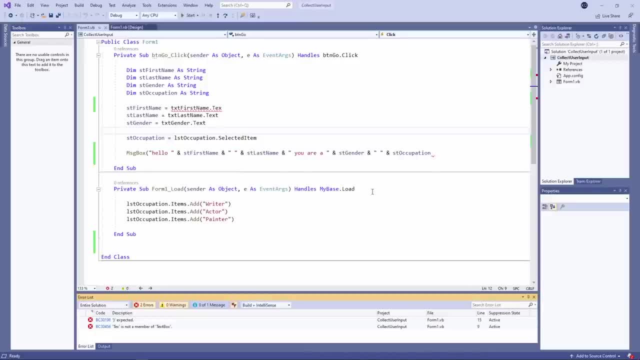 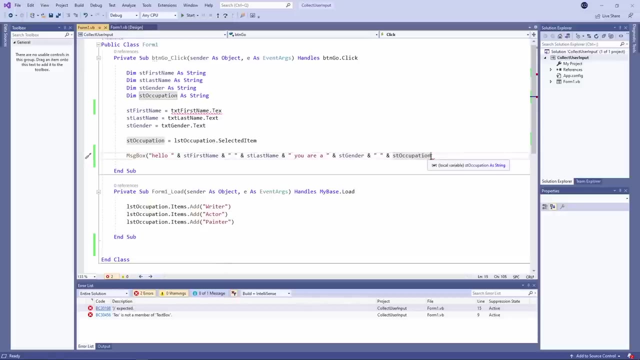 So I'm going to click on no, And now I have a list of errors. This is really just a summary of the same information that I saw with the red wavy lines. I'm being told that it's expecting a closing bracket. A double click on there and it jumps me to where I need to do the fix. 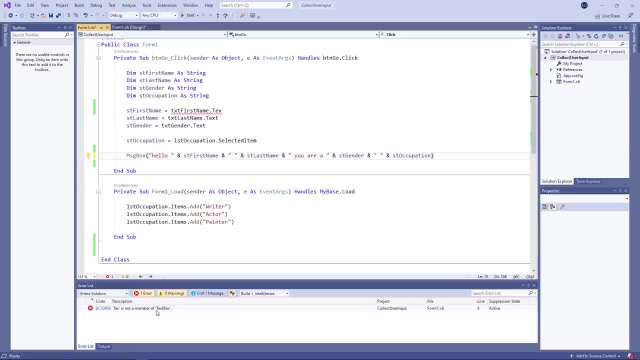 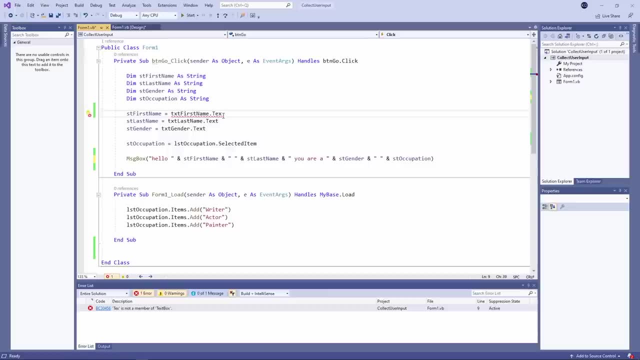 And I'm being told that text is not a member of text box. In other words, text is not a property of a text box. A double click and it will jump me straight to that line. I can fix it here now. As I said before, though, I like to watch out for the red wavy lines while I'm coding. 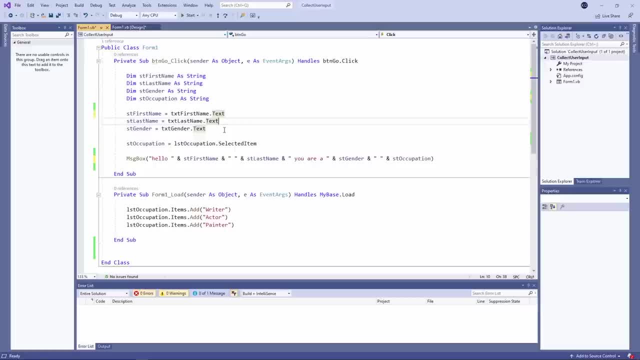 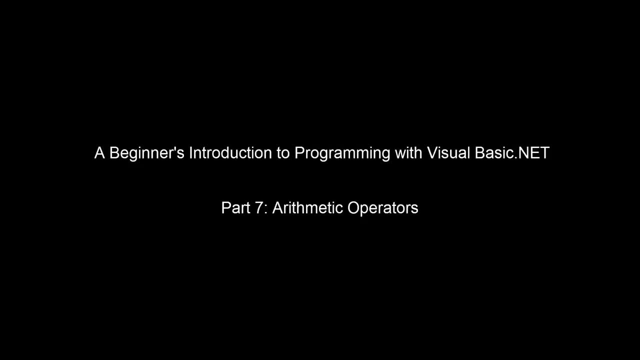 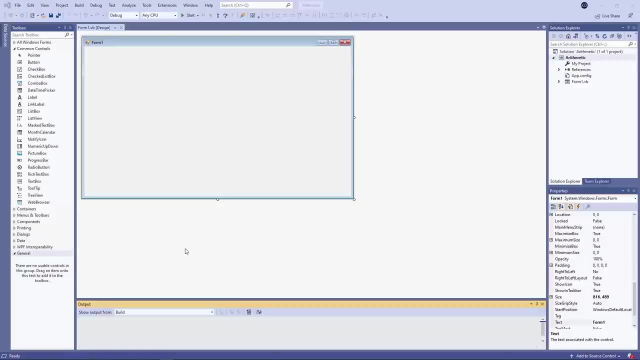 and fix them as I go along. OK, Show you some more debugging facilities as and when I need them in later videos. In this video, I'm going to talk about how we can work with numeric input from the user, In other words, how we can do calculations with number data. 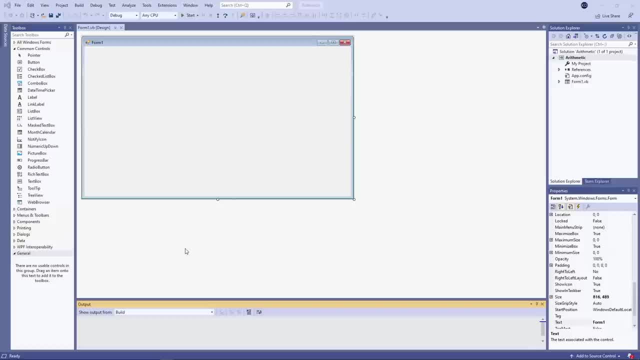 Before I do, I'm going to build myself a simple little interface with a couple of text boxes and a button. So I'm going to build a simple little interface with an image as a name, and then I'm going to add a new reference in the name of the reference. 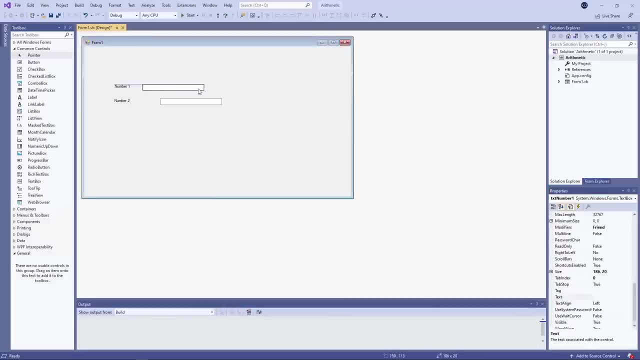 I'm going to add a name for that reference and then I'm going to add a new reference in the name of the reference. Now I would like to record the data that's resulting from those numbers. Let's do that, Hi. Notice how I've been naming the controls as I go along. 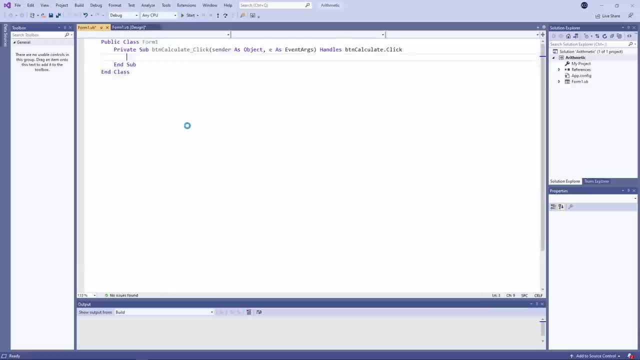 This will make the code easier to understand. The first thing I'd like to do is add together two numbers that the user types onto the form, So I'll start by declaring a couple of variables. Remember the data type: integer means a whole number. 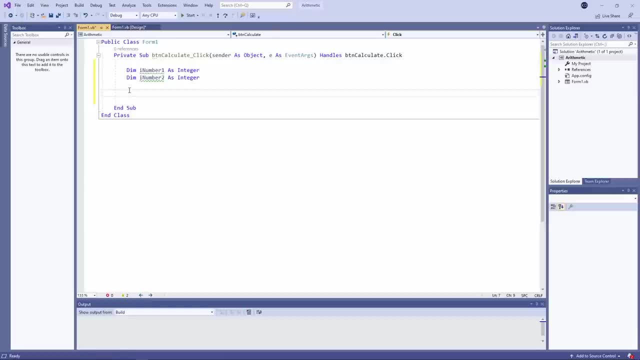 I'm going to declare another variable to store the result of the calculation, And now I'm going to capture the data that the user types into those text boxes. Adding these together couldn't be simpler. I result equals I number one plus I number two. 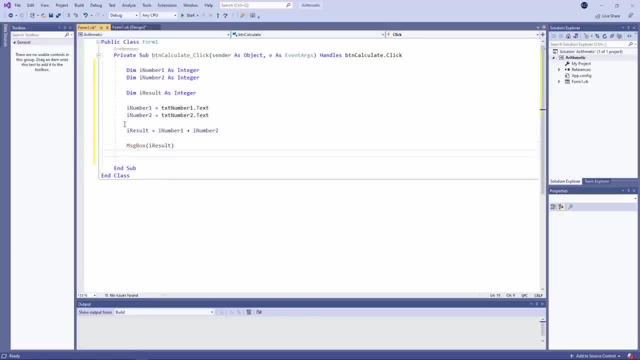 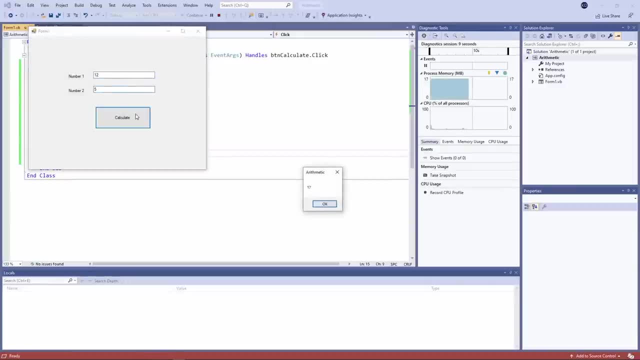 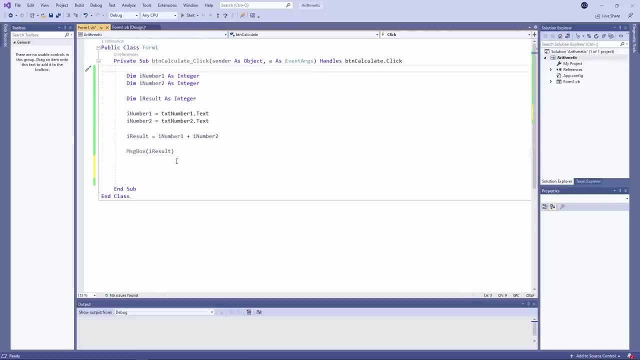 Let's output the result and see if it works. Twelve plus five is seventeen. Let's try something else. Let's subtract one number from the other. I result equals I number one minus I number two. I'll just borrow that message box statement. 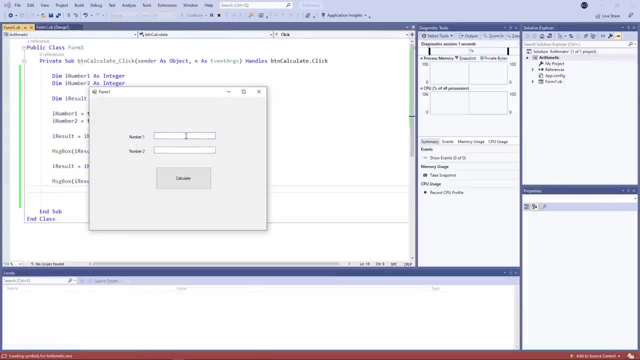 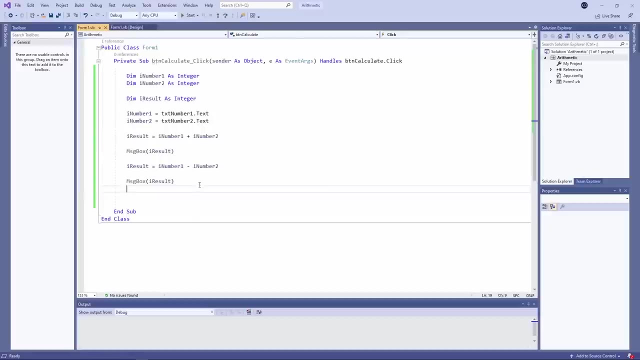 And we'll run the program again. So that's the two numbers added together and that's what we get when we subtract five from twelve. What about multiplication? To multiply two numbers together, we use an asterisk. That's the multiplication symbol. when you're programming, 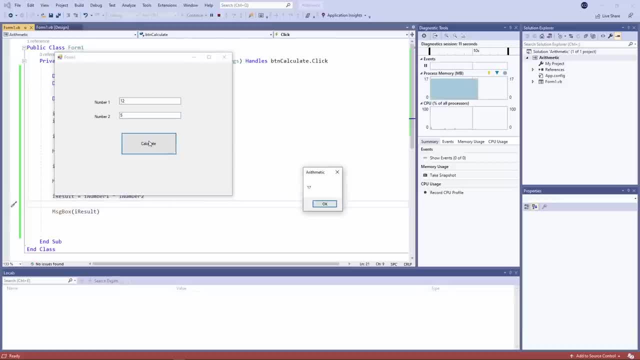 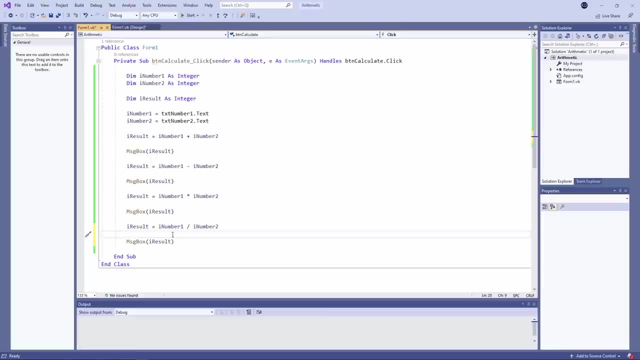 Twelve plus five, It's seventeen. Twelve minus five is seven, And twelve times five is sixty. Bit of copying and pasting. to speed things up: To divide one number by another, use a forward slash. So this reads as I number one divided by I number two. 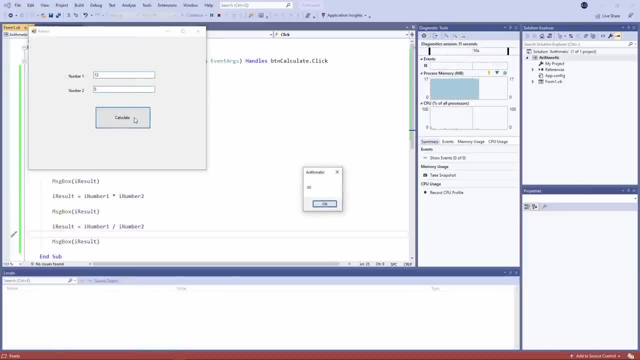 Twelve plus five is seventeen. Twelve minus five is seven. Twelve times five is sixty, And twelve divided by five is two. Well, not quite, but remember we're working with integers here, We're working with whole numbers. When I divide one integer by another and store the result in an integer variable, VB is automatically. 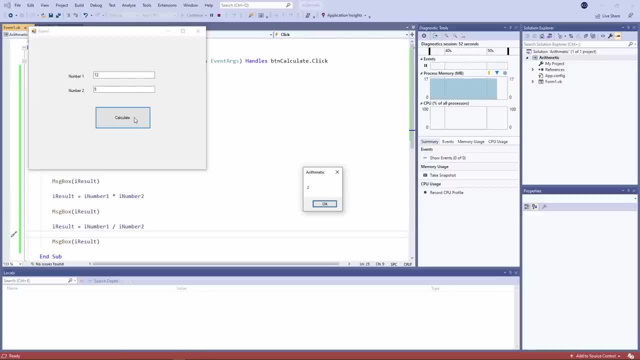 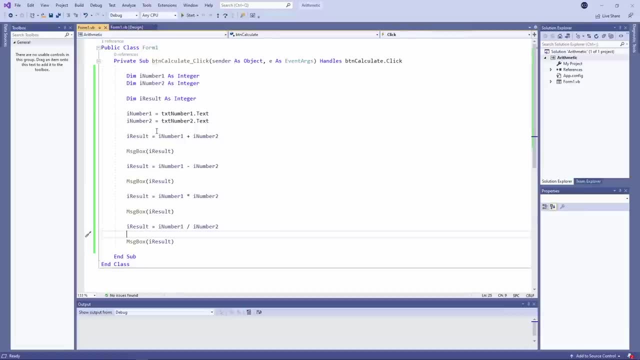 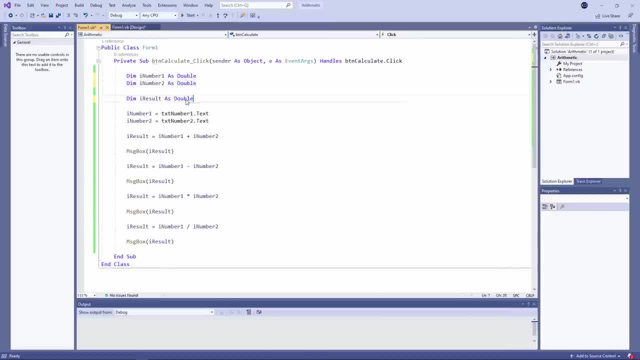 I'm going to use a real number type. Let's use a double. I'm also going to change the naming I've used here: DBL for a double. Strictly speaking, it doesn't matter what I call these variables, but I want the names. 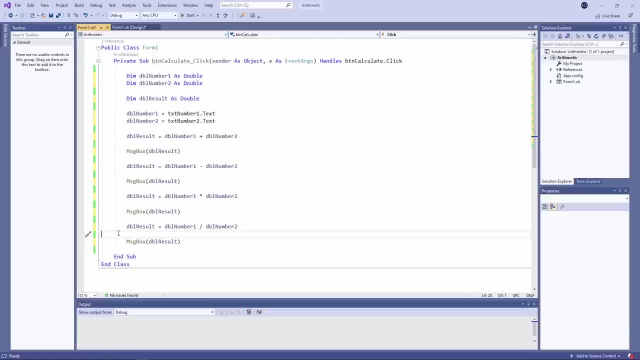 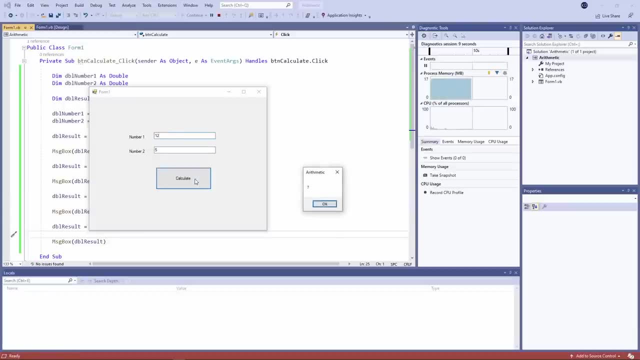 to be meaningful And I want the names to reflect the variables, reflect the data type. let's see what we get this time. same as before: 12 plus 5 is 17, 12 minus 5 is 7, 12 times 5 is 60. but 12 divided by 5 is 2.4. that makes 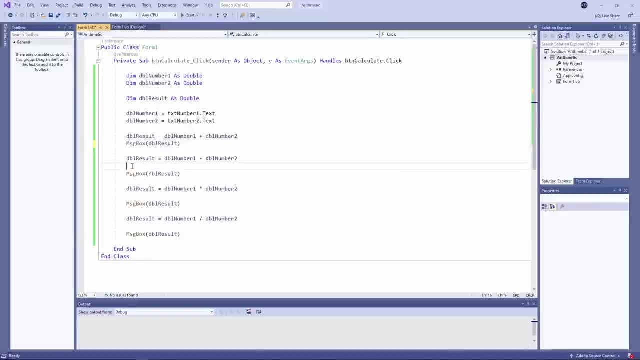 more sense. just to be clear about the way a variable works: I'm multiplying two numbers together here and I'm storing the result in this variable called DBL result. when I perform a second calculation, I'm storing the result in the same variable. what's happening is I'm overwriting the existing value in 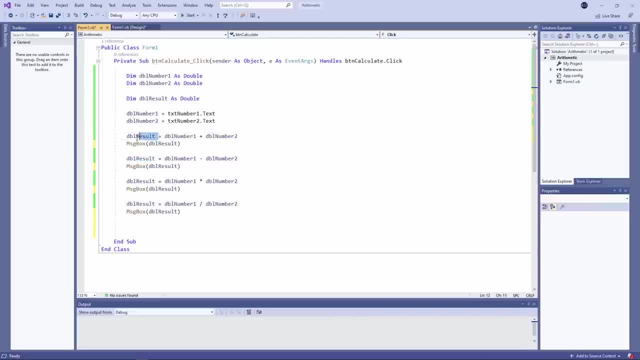 DBL result, I lose the value which was generated by the first calculation. when I do the third calculation, I overwrite the value inside DBL result again, so I lose the result of the second calculation. by the time my program comes to an end, this contains the result of the first. 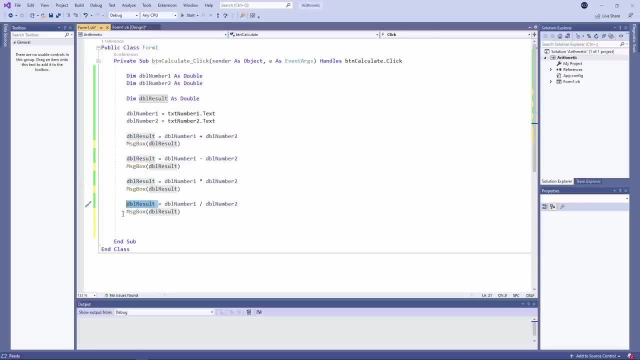 number divided by the second number. if I wanted to keep the result of each of these calculations, then I should have declared four separate variables. these are called arithmetic operators. these are the basic operations that we might want to perform with numbers. there are a couple more. let me show you them. 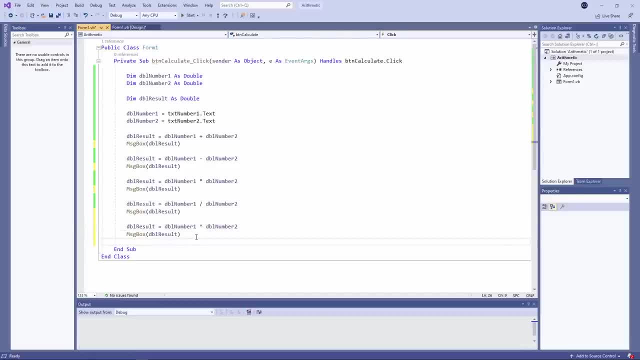 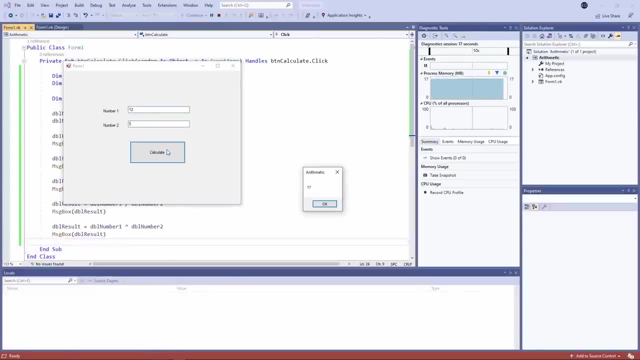 that's the Carre symbol, which is normally above the number six on your keyboard, and what it means is raised to the power of. so it's going to raise number one to the power of number two. twelve plus 5, 12 minus five. twelve times 5, 12 divided by 5 and 12 to the power of. 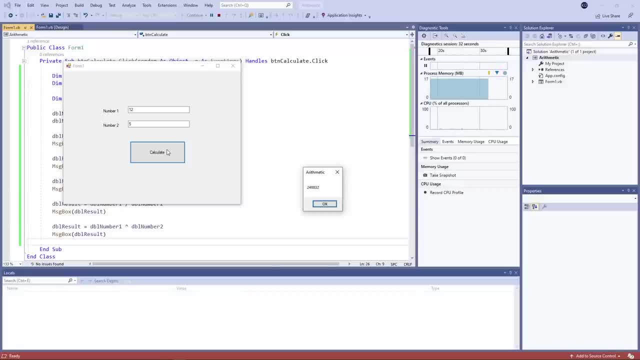 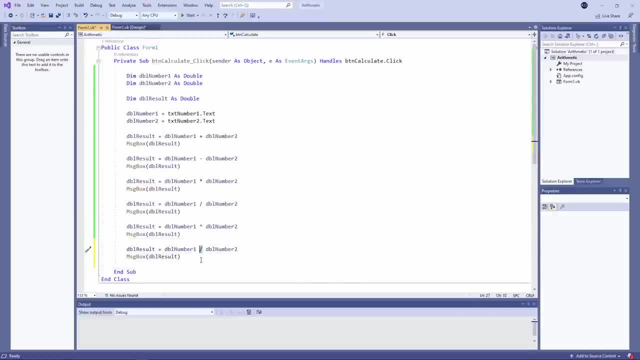 Another useful operator is integer division. I'm going to use a backslash instead of a forward slash. In some programming languages you would use the word div. In fact, the pseudocode that you see on most exam papers will use the word div. 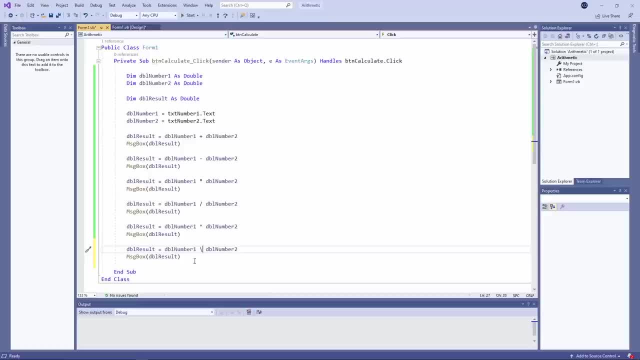 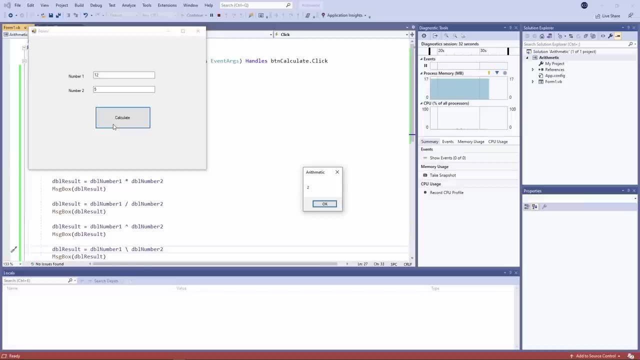 In Visual Basic we use a backslash. Let's take a look. That's the effect of using a backslash instead of a forward slash. Twelve is being divided by five, but only the whole number. part of the result is being kept. 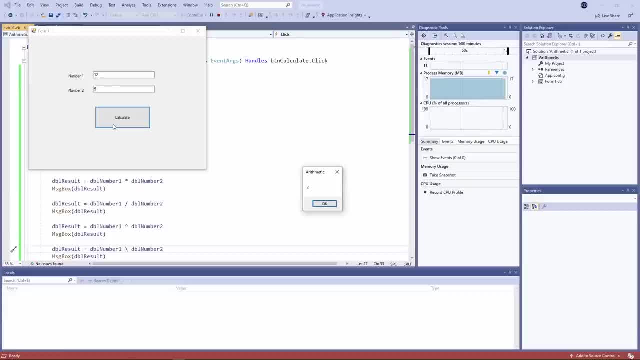 Twelve divided by five is two, with two remainder. We're ignoring the remainder. Let's try fifteen and four. Fifteen plus four is nineteen. Fifteen minus four is eleven. Fifteen times four is fifteen. Fifteen divided by four is sixty. 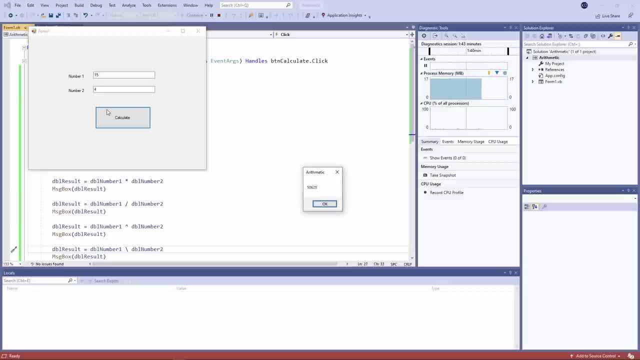 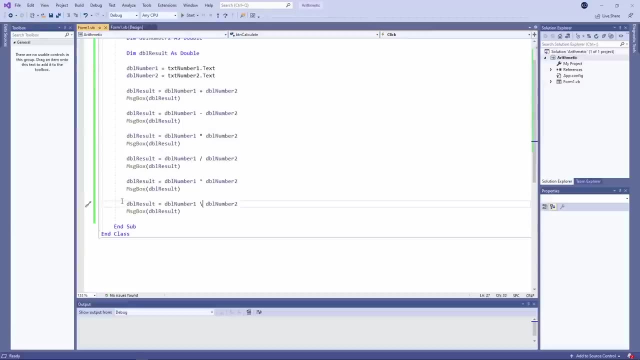 Fifteen divided by four is 3.75.. That's fifteen raised to the power of four, And that's fifteen divided by four. ignoring the remainder Four, goes into fifteen three times. The last arithmetic operator that I'd like to show you now is mod. 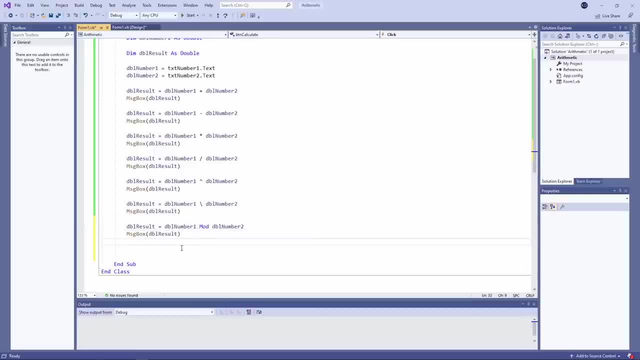 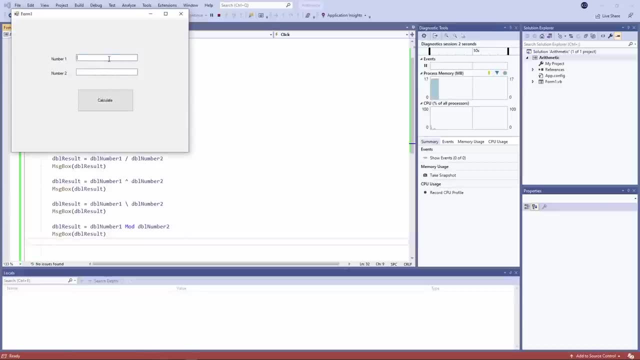 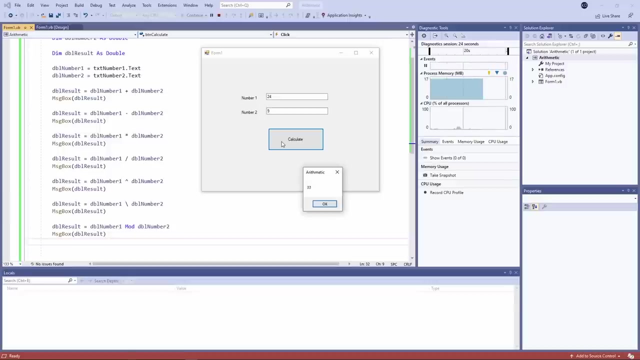 Number one mod. number two Mod is the remainder after whole number division. Let's see what this does. Let's go with twenty-four and nine this time. I'll just move the form across so you can see the code as well. Twenty-four plus nine is thirty-three. 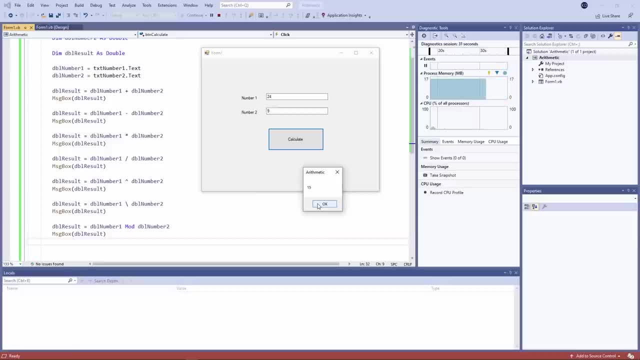 Twenty-four minus nine is fifteen. Twenty-four multiplied by nine is fifteen. Twenty-four minus nine is fifteen. Twenty-four multiplied by nine is fifteen. Twenty-four minus nine is fifteen. Twenty-four divided by nine is 216.. Twenty-four divided by nine is 2.6. recurring. 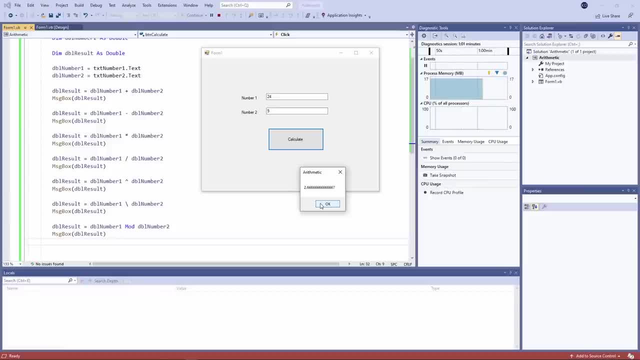 The number of decimal places you can see there is governed by the data type. Twenty-four raised to the power of nine is this rather large number. Twenty-four divided by nine, using integer division, is two. Nine goes into twenty-four twice And nine goes into twenty-four twice, with six remaining. 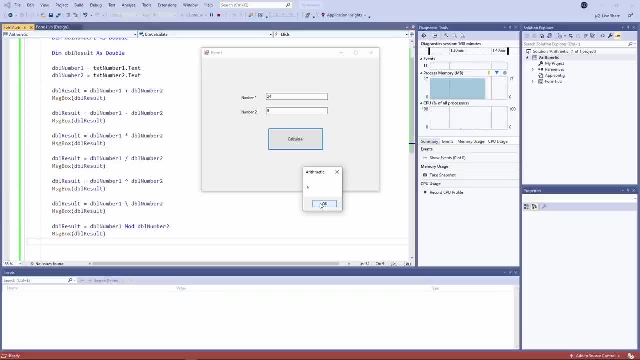 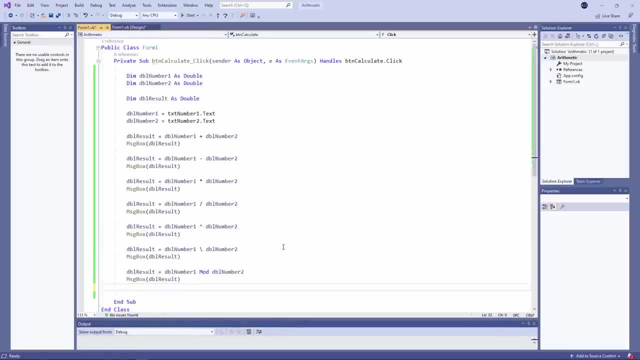 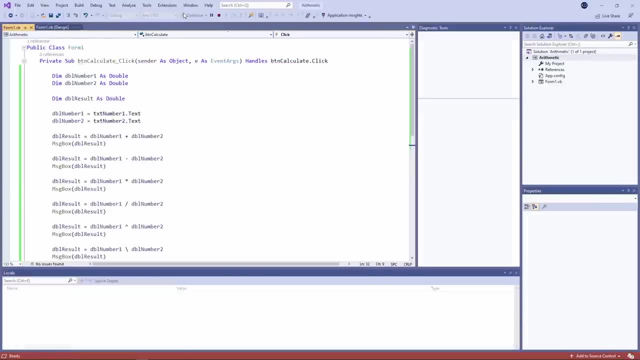 That's what mod is giving me. It's the remainder after whole number division. Let me finish with a word of warning. I'm going to run this program again, but I'm not going to enter any data. I'm going to leave these two text boxes empty. 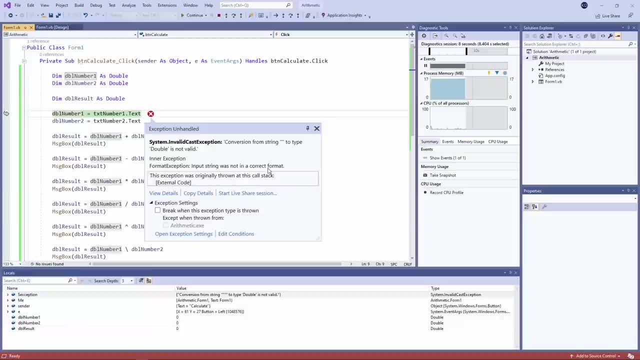 I'm going to run this program again. Straight away, I have an error message. Conversion from string to type double is not valid. This tells me something about what's going on behind the scenes. Let's stop the program and put a breakpoint on this line. 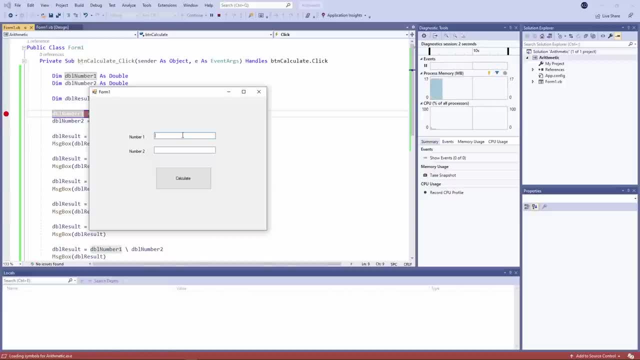 When you type something into a text box, it's actually a string. Notice here: text equals five seven in double quotes. When this line of code executes, VB will automatically convert the string five seven into a number. You can see DBL number one has got a zero in it at the moment. 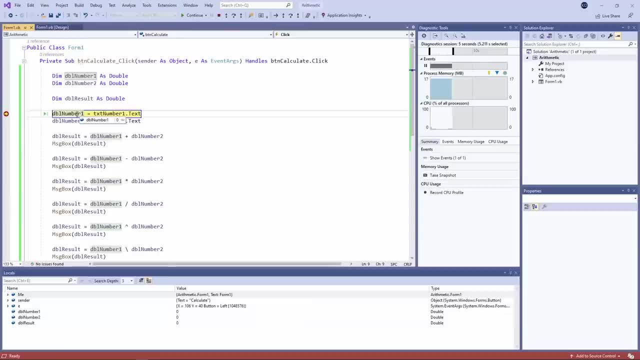 That's the initial value of any numeric variable until you assign something else to it. Step through the code. The text box contained five, seven, but the variable contains fifty seven. Behind the scenes, Visual Basic is automatically converting the string into a double because 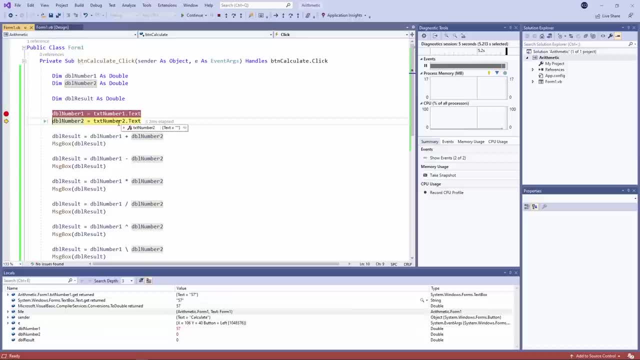 it can But notice that my second text box contains a zero length string, A pair of double quotes with nothing in between them. It's a string, but it just doesn't have any length, And when this line of code executes, VB will attempt to convert that zero length string. 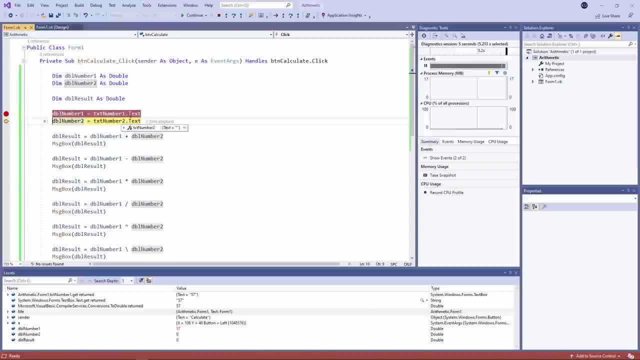 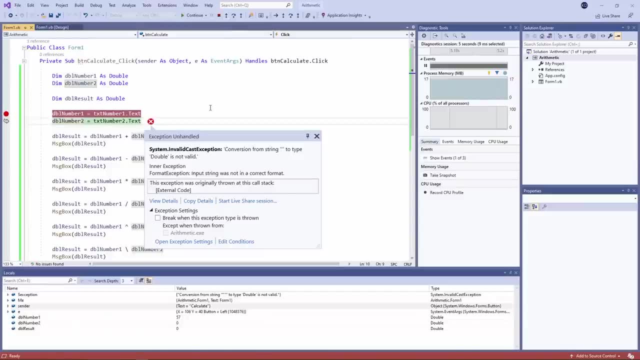 into a number. but of course it can't And my program has crashed. This is what we call a runtime error. The program crashed while it was running. It crashed at runtime. Another name for a runtime error is an exception. So you can see here I have an unhandled exception. 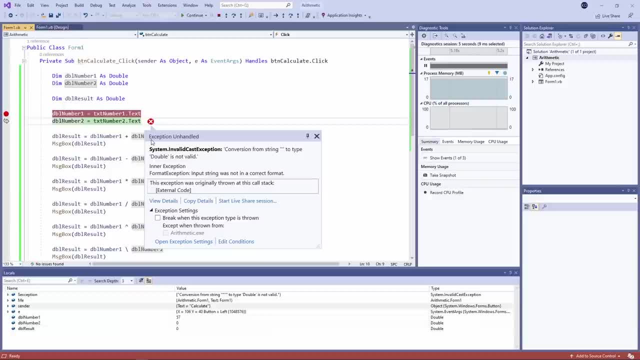 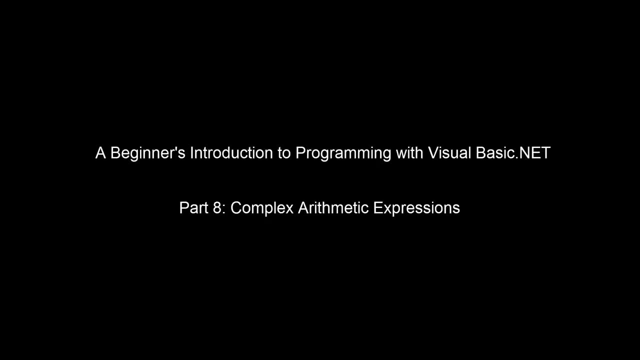 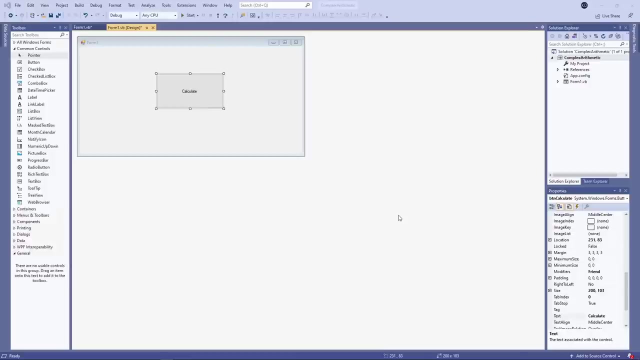 I'll talk more about runtime error handling or exception handling in a later video, But for now, with this program, we just have to expect the user to do the right thing: not to leave any of the text boxes blank. In this video I'll say something about complex arithmetic, that is, arithmetic expressions. 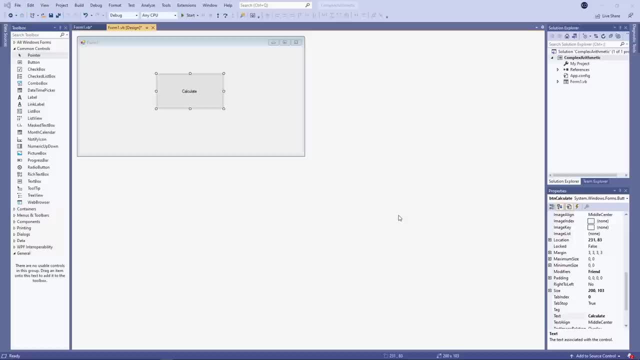 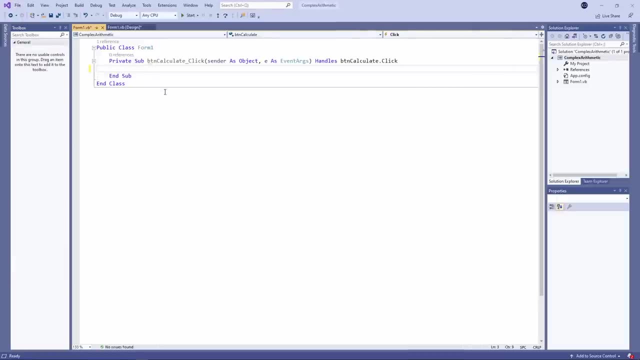 that contain more than one arithmetic operator. Let's write some code. Let's imagine we're building an application for a cake shop and the application will calculate the total cost of a number of cakes. I'm not going to capture any input, I'm just going to hard code the data to keep things. 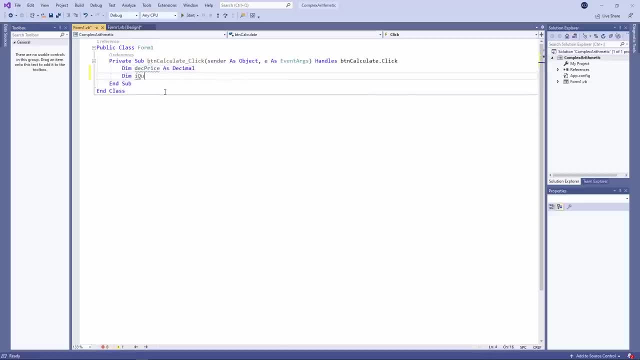 simple. So I've declared three variables: one for the price of a cake, one for the quantity of cakes and one to store the total cost of however many cakes are being bought. Let's initialize these variables with some data. As I said, I'm hard coding the data, so I can focus on the calculation. 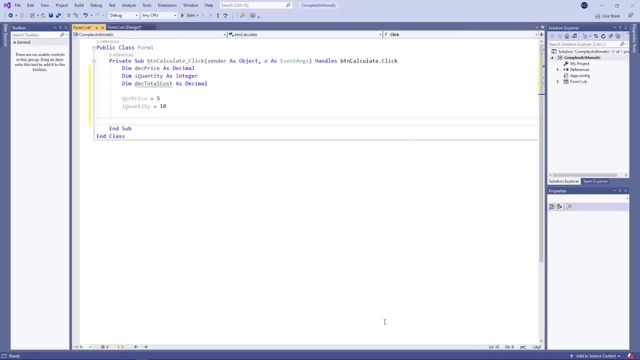 But of course I would probably want to capture this data from text boxes on the form. So to calculate the total cost of ten cakes at a price of five pounds per cake- these are good cakes, by the way- I'll use the multiplication operator. 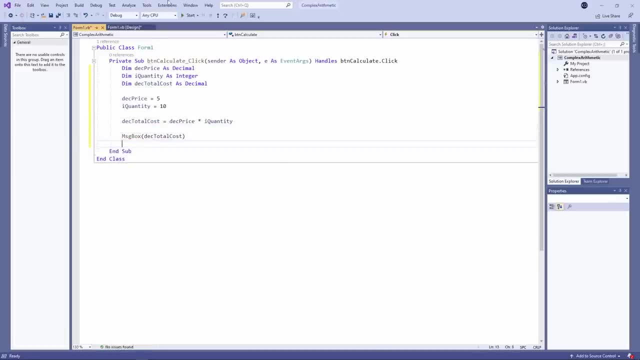 And let's output the result: Fifty pounds worth of cakes. No surprises there, Let's see. OK, Now suppose for a moment we want to calculate a discount of, let's say, two pounds per cake. You might be tempted to try this. 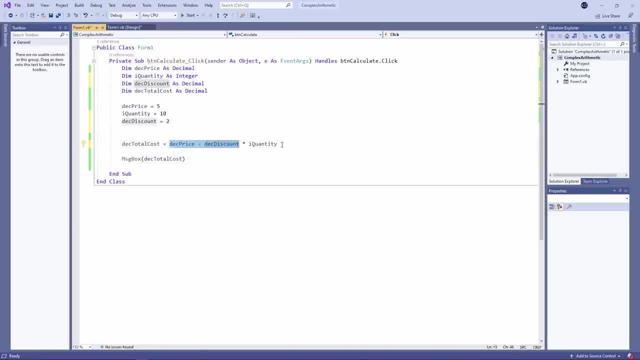 Take the original price, subtract the discount and multiply it by the quantity. Five pounds per cake minus two pounds per cake, that's three pounds per cake multiplied by ten, I might expect a result of thirty pounds. Let's take a look. 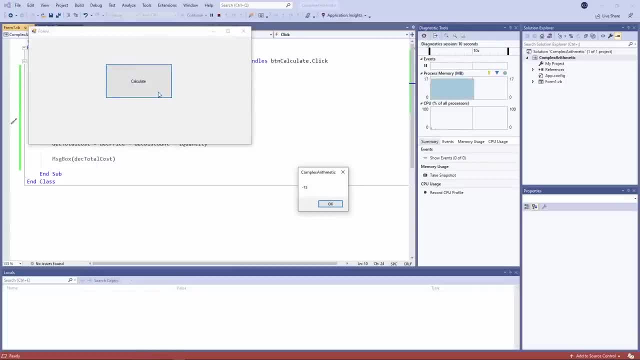 Minus fifteen pounds. Not only are we giving the cakes away, we're giving money to the customers as well. That's totally unsatisfactory. What's going on? Well, there's an order of operations that applies when it comes to complex arithmetic. 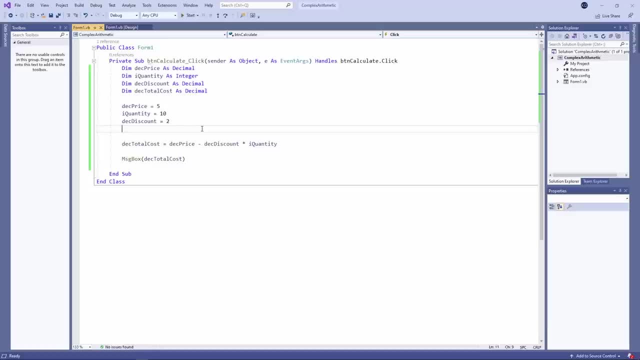 expressions. By a complex arithmetic expression I simply mean an expression, An expression with more than one operator. This expression includes a minus sign and a multiply sign. The order of priority is that multiplication is done first. So in this case the discount is being multiplied by the quantity, which is twenty, and then 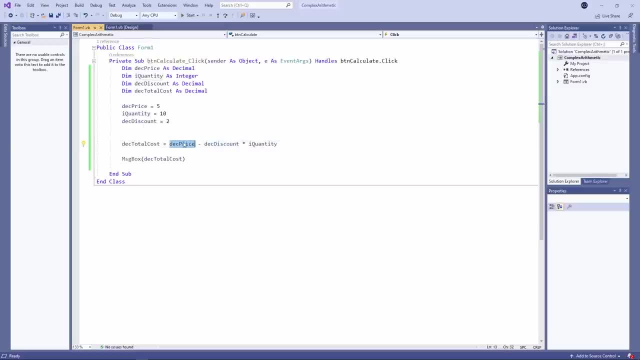 that is being subtracted from the price. Five minus twenty is indeed minus fifteen. OK, If I want the discount to be applied first- in other words, I want the subtraction to happen first- I can control it using brackets or parentheses, as they're otherwise known. 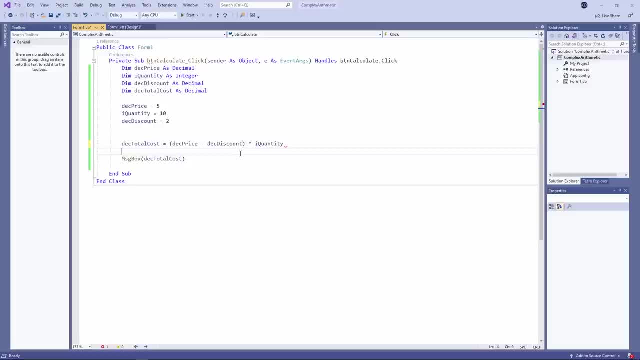 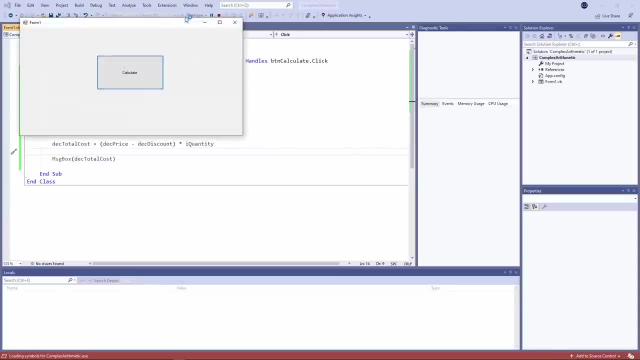 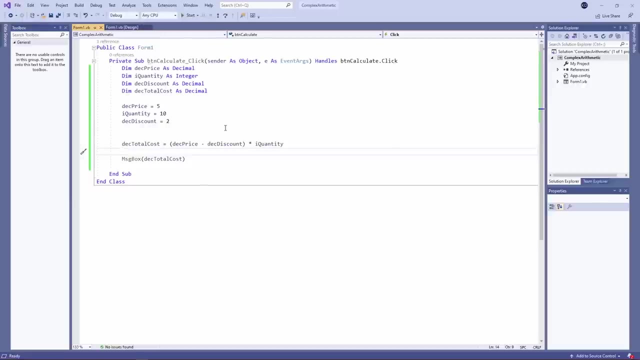 Like this. So now anything inside the brackets will happen first, And there's the thirty pounds I was expecting. You may well have come across this already. You might have heard of BODMAS. BODMAS stands for brackets. order, division, multiplication, addition and subtraction. 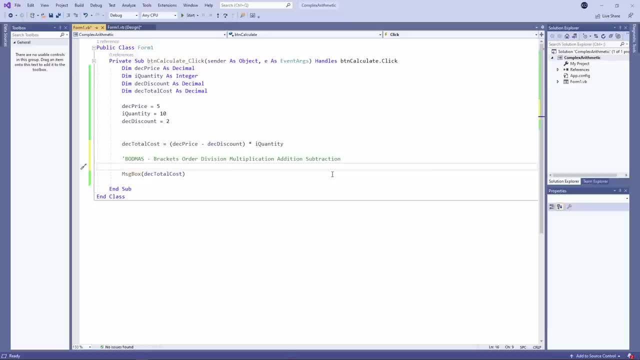 That's the order of priority of the arithmetic operators. Order, by the way, means exponentiation. It means raising something to the power of something else. So what we're saying is: anything inside brackets will be done first. If there's an exponentiation operator in the expression, that will happen next. 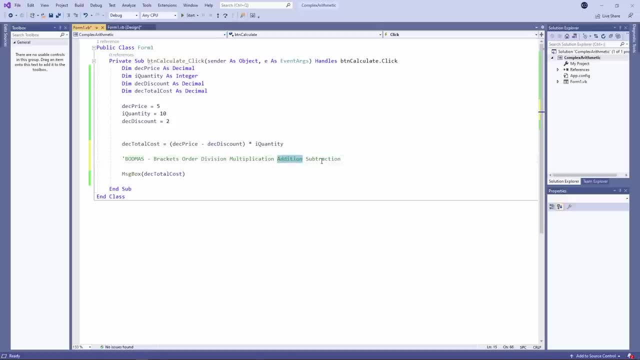 Followed by division, multiplication, addition and subtraction. The truth is, division and multiplication have the same priority. Also, addition and subtraction have the same priority. So perhaps we should say to indicate the fact- By the way, I typed a single apostrophe before I wrote this: 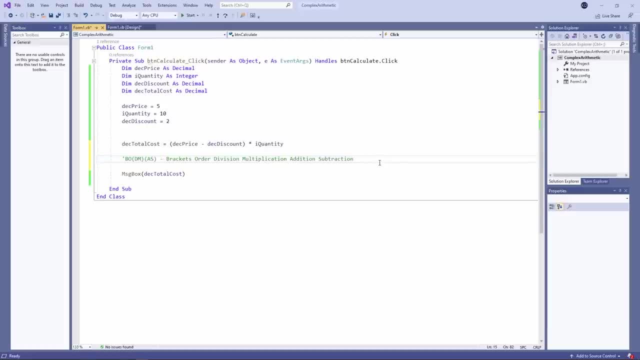 This is not code. This is simply a comment which I've added to my code. Comments aren't executed. They're not part of the program. A comment is just something that I can put in my code to help me to understand it. Now let's suppose for a moment. I want to add a charge for postage and packaging. 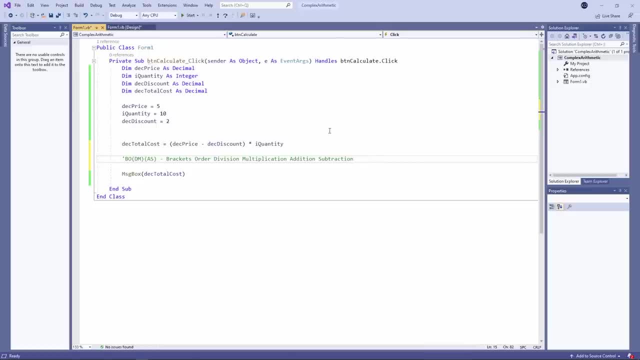 To the total cost of this order. We'll have a flat charge of three pounds, And I'm just going to add it to the end of this calculation. Thinking about the order of operations, whatever's in brackets will happen first. Then that will be multiplied by the quantity. 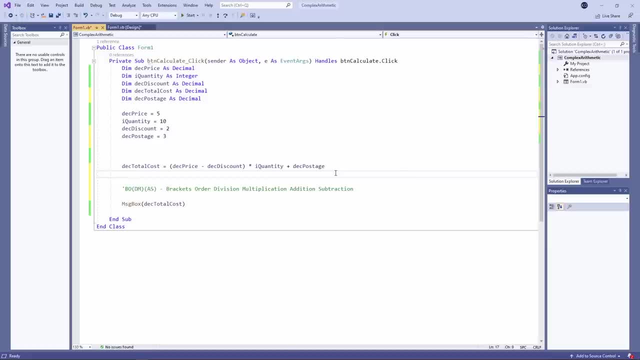 And then, finally, the postage will be added on, So I don't actually need to include any brackets here. Thirty-three pounds, as expected, But there's nothing to stop you from adding brackets if it helps you to understand the code. So, for example, I might do this: 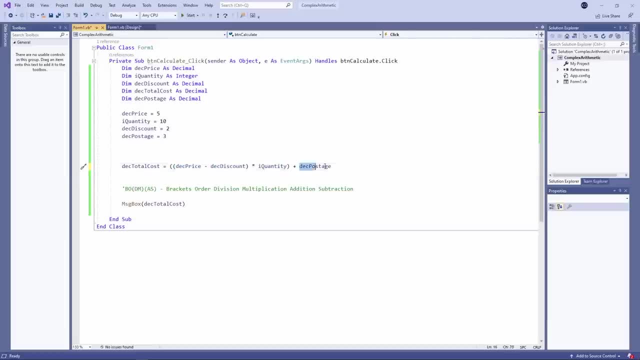 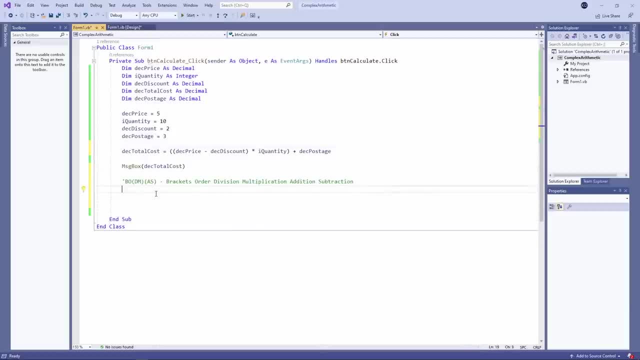 I'm going to add brackets. I'm going to add brackets. Now, this is the standard one that you may have come across. is this PEMDAS? This stands for PEMDAS. It's essentially the same thing as BODMAS. 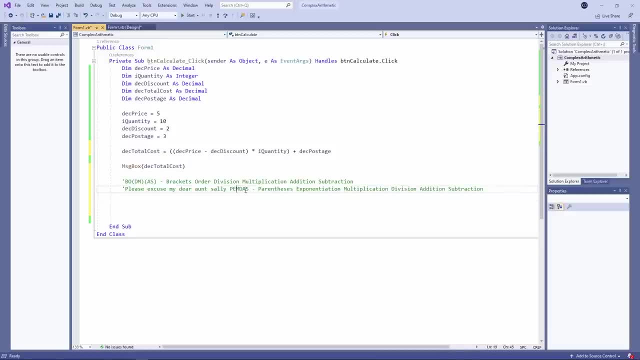 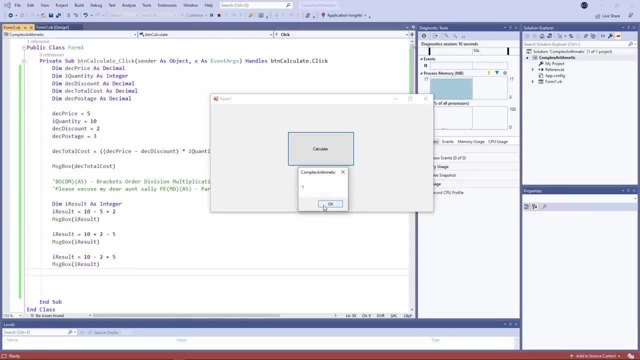 You might have noticed that the M and the D are the other way around, But that just makes the point that the order of operations when it comes to division and multiplication is irrelevant. Now beware, you might come across this: That's the cost of my cakes. 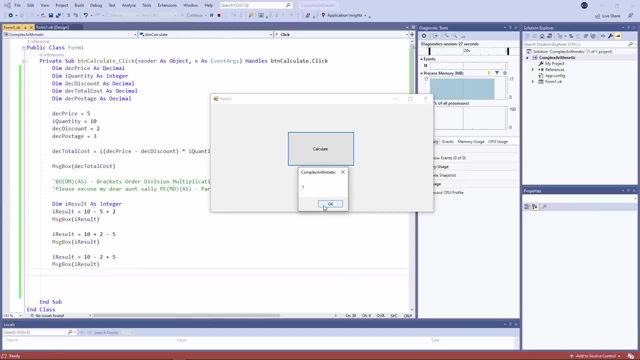 That's 10 minus 5 plus 2.. Of course, 10 minus 5 is 5, plus 2 is 7.. That is 10 plus 2 minus 5.. 10 plus 2 is 12, minus 5 is also 7.. 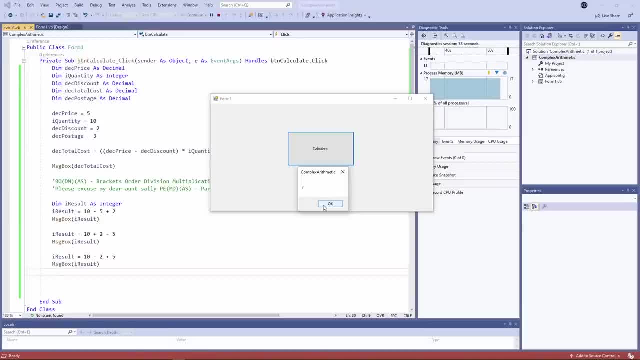 All I've actually done is swap around the order of the operations. But 10 minus 2 plus 5 is 13.. Let's be clear. I haven't just swapped around the order of the operations. I'm changing the number which I'm subtracting from 10.. 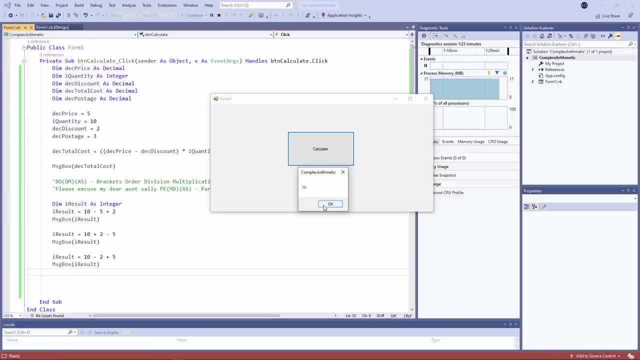 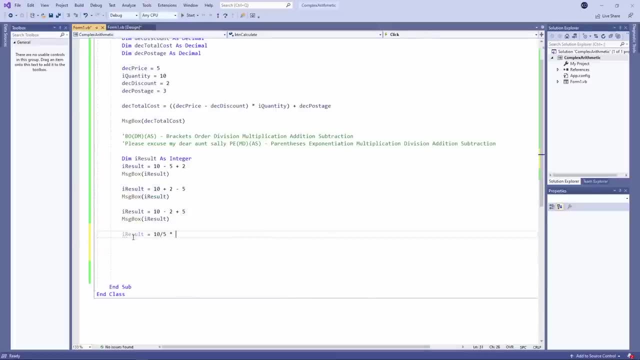 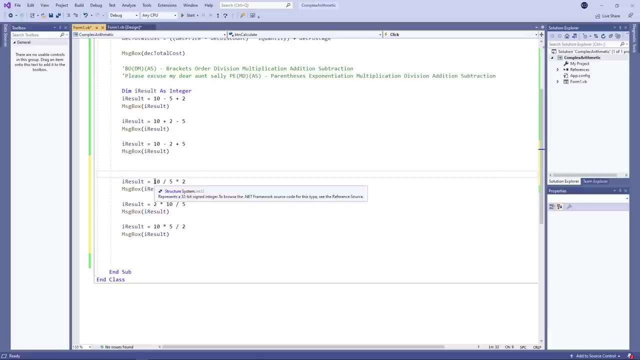 10 minus 2 is 8, plus 5 is 13.. It's a different calculation. The same applies here. In the first two examples, all I've done is change the order of operations. I've got 10 divided by 5.. 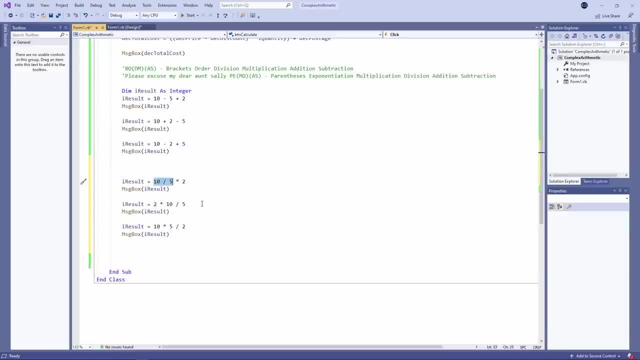 Times 2. Or 2 times 10 divided by 5.. But in the third example it's a different calculation: It's 5 divided by 2, multiplied by 10.. So beware, BODMAS and PEMDAS, both apply. 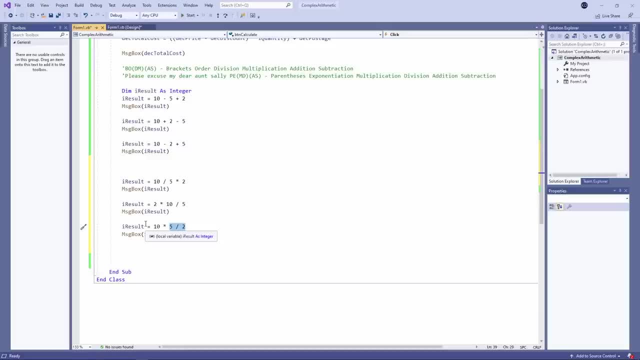 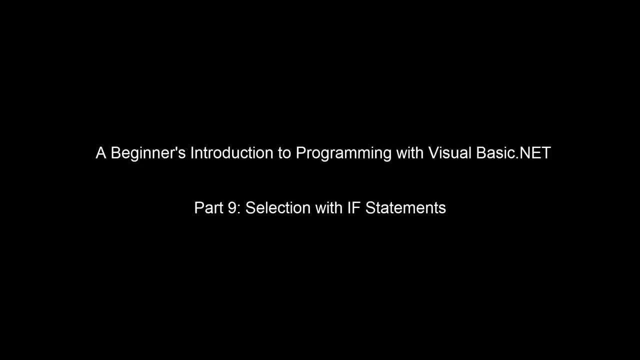 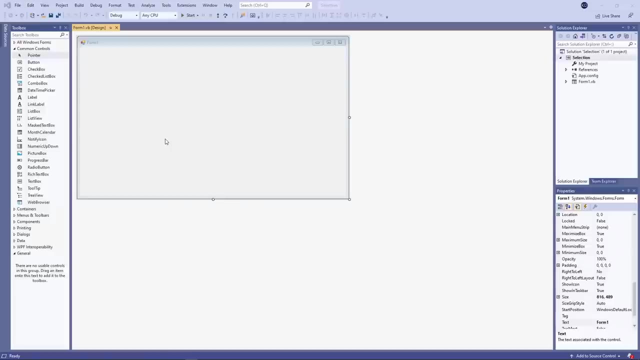 They do tell us the order of operations when it comes to complex calculations, But complex calculations can also be quite deceptive. There are three fundamental constructs in most high-level procedural programming languages, such as VBnet, And they are: sequence, selection and iteration. 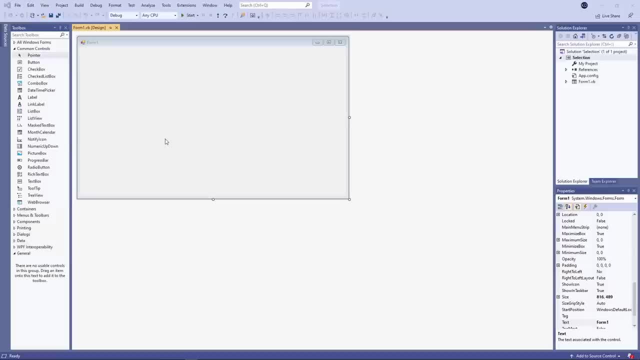 In this video I'm going to introduce selection. That means executing one block of code or another depending on the outcome of a test. One way we can do this is using the IF statement. Let's start with a simple user interface. I've said it before and I'll say it again: 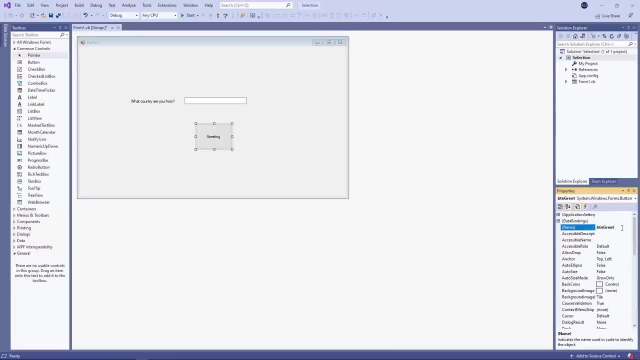 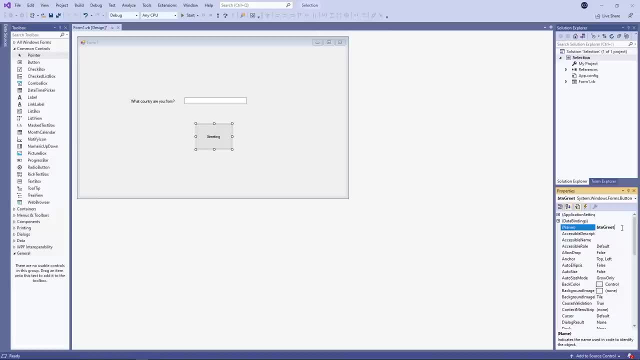 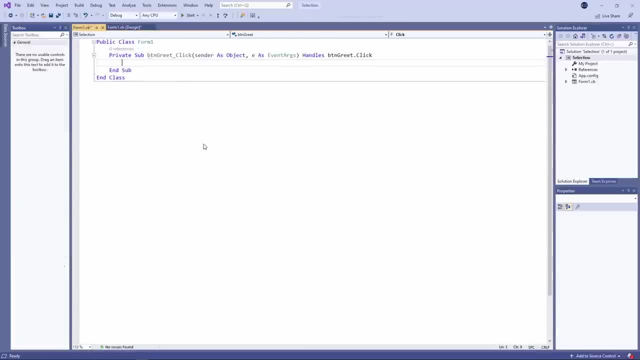 I'm going to do that in a minute. I'm going to do that in a minute. I'm going to ask the user what country they come from and then give them an appropriate greeting. I'll capture the input from the form by assigning it to a variable. 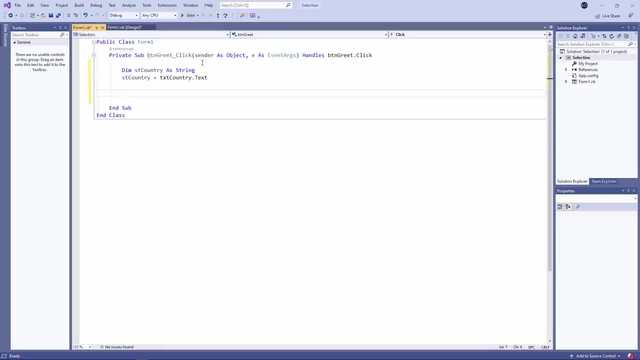 And now I'm going to use an IF statement to test the contents of that variable. On the right side I've made it clear that this is a variable. If the country is equal to Australia, then I'm going to output the message. G'day mate. 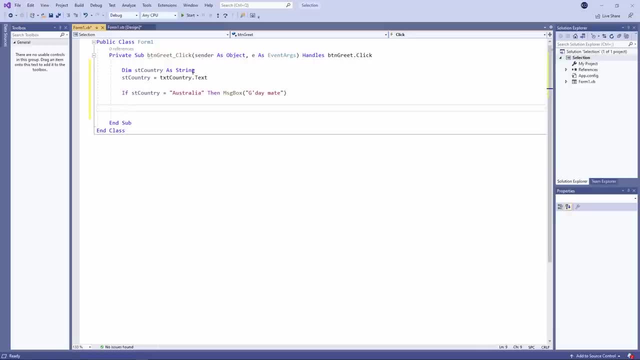 I want you to notice that I'm using the equal sign to check if two things are equal, Whereas here I'm using the equal sign to assign something to a variable. In some programming languages you'll use a slightly different approach. For example, in Python, if you were checking for equality, you would use two equal signs. 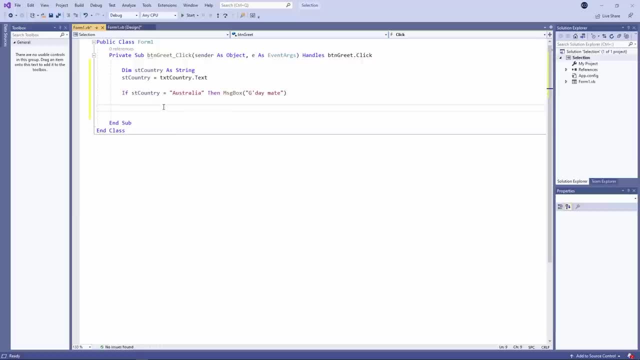 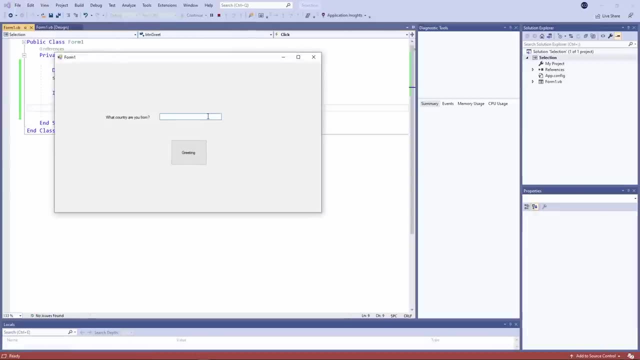 In VB, a single equal sign can be used either for checking or for assignment. So let's try it out. If I input Australia, I get the Australian greeting. If I input something else, nothing at all. That doesn't mean my code isn't working. 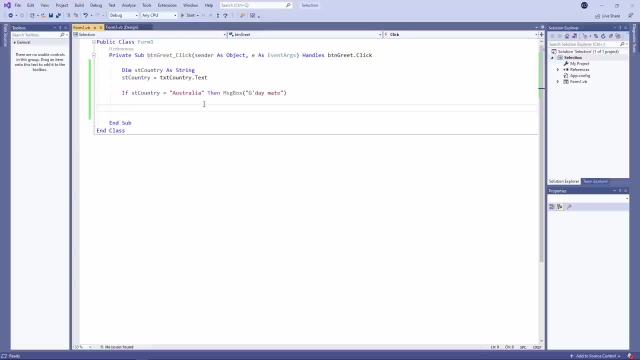 It's doing exactly what it's supposed to do. This is what we call a one-line if statement. I can execute one command depending on the outcome of the test, But if I want to execute multiple commands depending on the outcome of a test, I'm going. 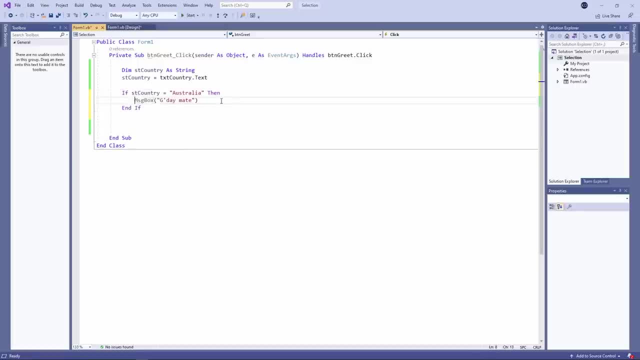 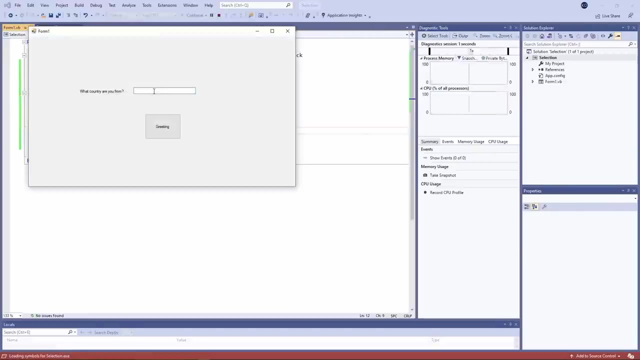 to use a block if statement. I've moved that command to the next line down. Visual Studio has automatically added an end if. And now between the if and the end, if I can have as many commands as I like, So watch what happens now. 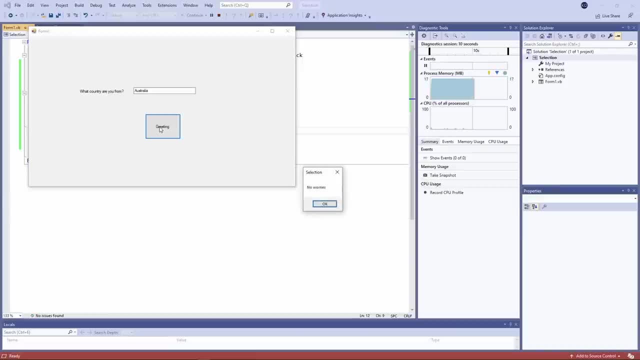 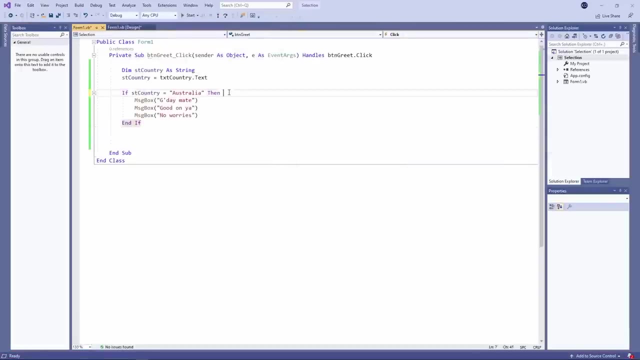 G'day mate. Good on ya. No worries If I don't type Australia. if I type something else, nothing happens at all. Now a word of warning: If I put something else After the word, then that's a syntax error. 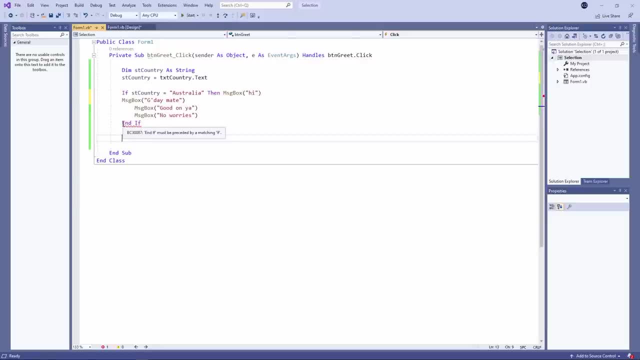 End if must be preceded by a matching. if This line of code is complete, It's syntactically correct. However, you can't have an end if on its own. If you're going to use a block, if there should be nothing after the word, then 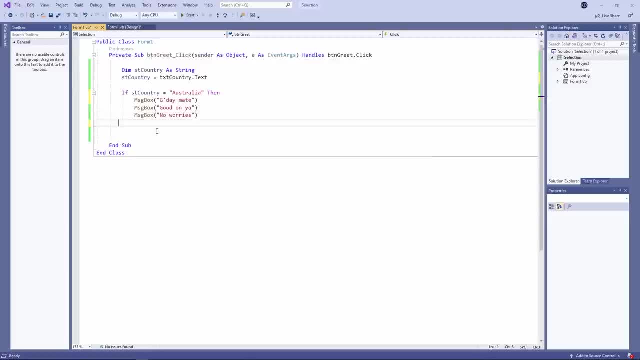 If there's nothing after the word, then- And I forget to use end if- Again, I've got a syntax error- If must end with a matching end if. So you have a choice. You can either use a block if Or a one line if. 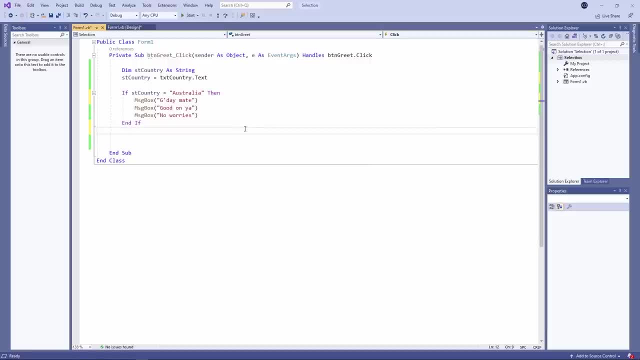 But whichever one you use, you have to use it correctly. When it comes to a block, if I can have multiple else, if clauses as part of it Like this: There we go, There it is else. if country equals France: bonjour, comment, allez-vous? let's try it out. 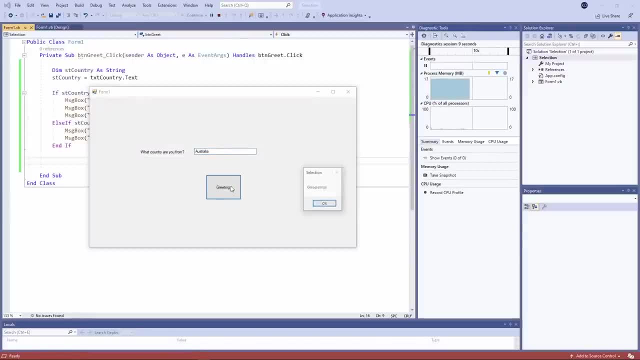 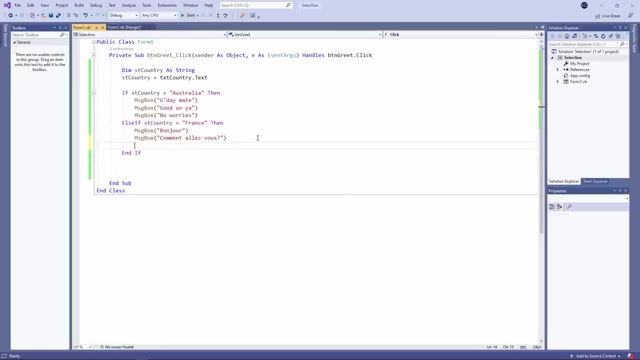 those are my three Australian greetings, and if the country is France, bonjour, comment allez-vous? however, if I enter something which isn't France and isn't Australia, nothing, let's include another else. if else, if country equals Japan, konichiwa chelsea wadu desuka. 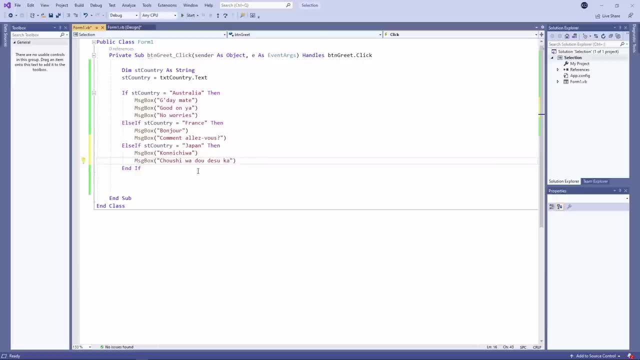 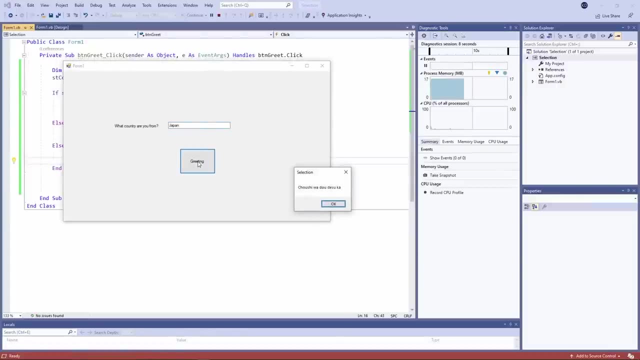 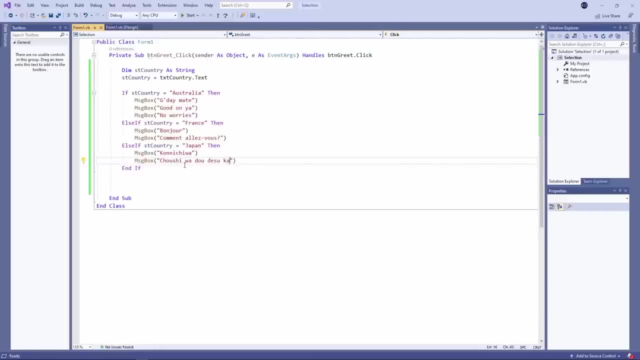 I think I pronounced that correctly. let's try it out now. and there are my Japanese messages. I can have as many else if clauses as I like in a block if statement and I can finish with a single else clause. if I don't type Australia, France or Japan, then it will say: hello there. I hope you. 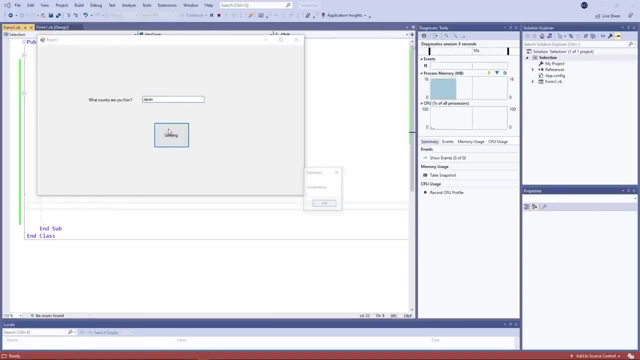 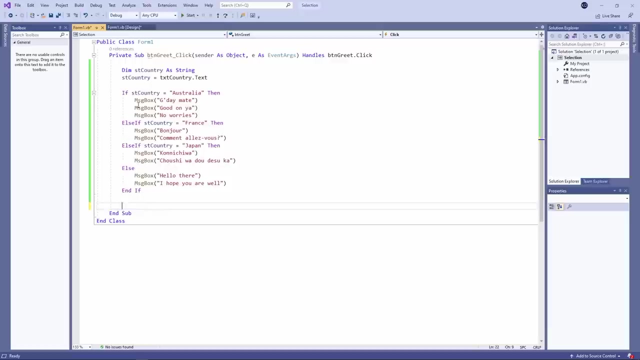 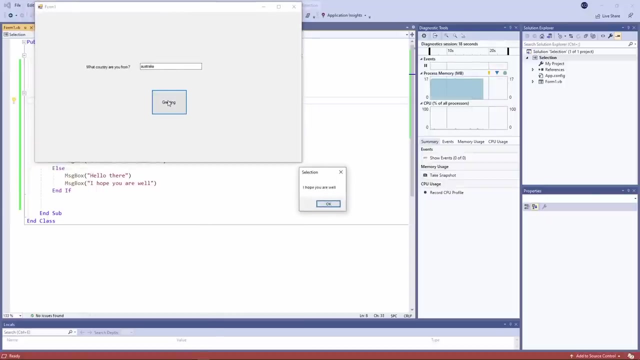 are well, so everybody gets something. now just a small word of warning. the tests that you perform with an if statement are case-sensitive. watch what happens. if I type Australia in lowercase, you, The block of code in the ELSE clause is executing because I didn't use a capital A. 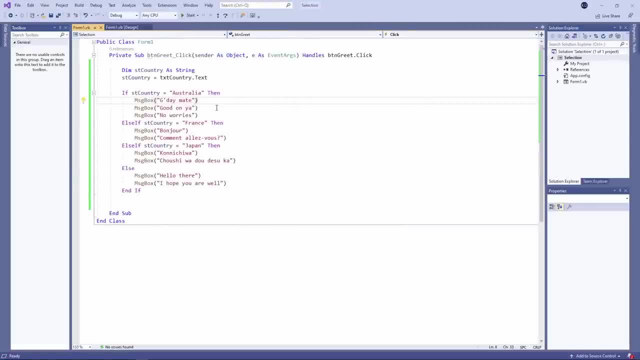 I can remove the case sensitivity of this test by converting the contents of the variable STCountry into uppercase. like this I'm saying: take the content of STCountry, convert it to uppercase and then put the uppercase version of it back into the variable, overwriting the original contents of that. 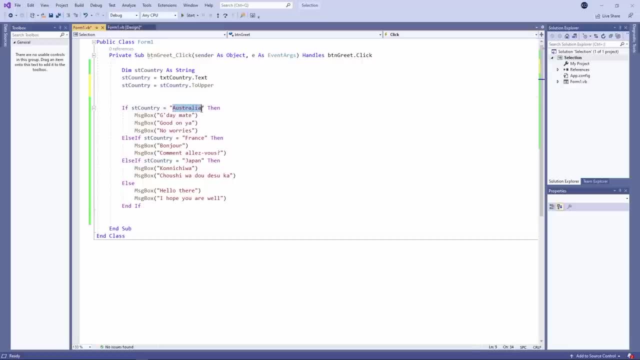 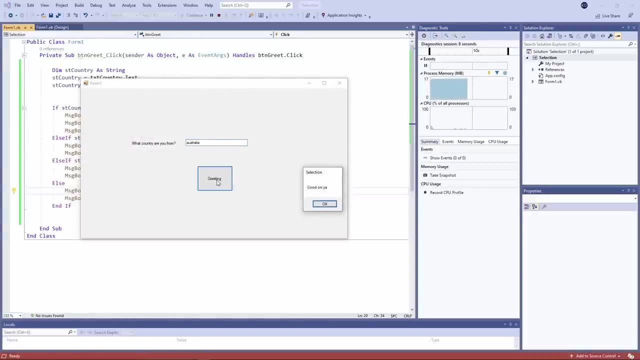 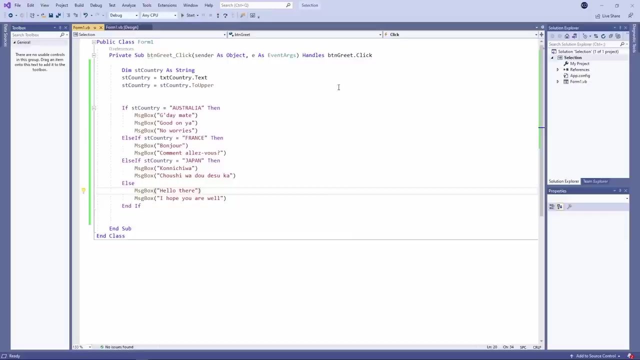 variable, And now I'm going to check to see if that is equal to this. It doesn't matter what type of case I use when I'm typing in the country. I've removed the case sensitivity from the test. Let's just step through this to be sure what's going on. 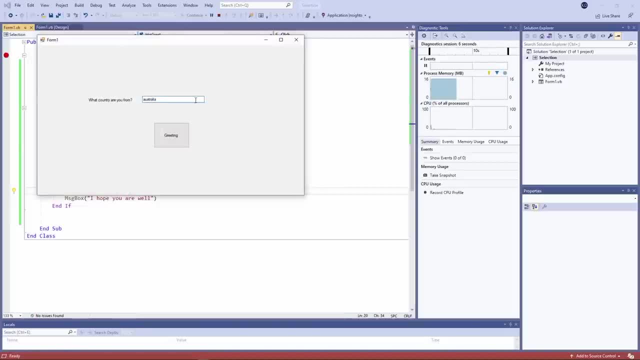 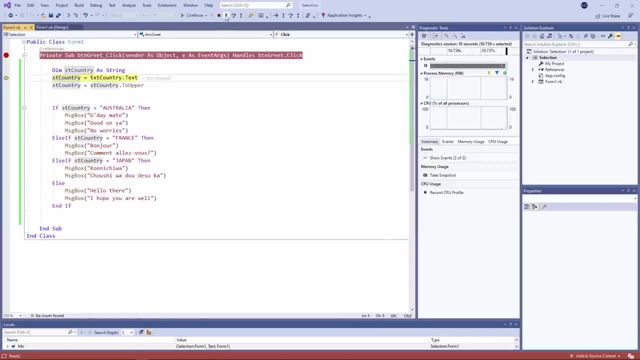 I'll put a breakpoint on the procedure. So I've typed in lowercase Australia, That's what I've captured into this variable, And then I've converted it to uppercase Australia. So I'm asking if uppercase Australia is equal to uppercase Australia. OK, 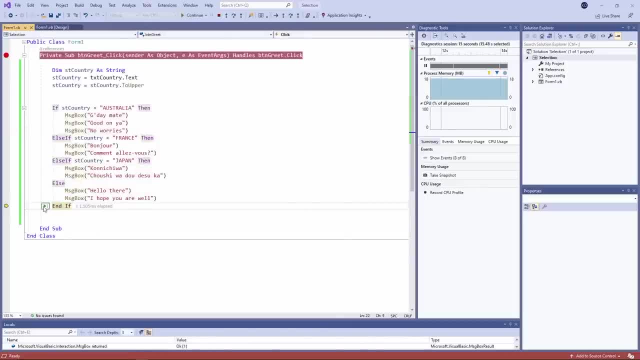 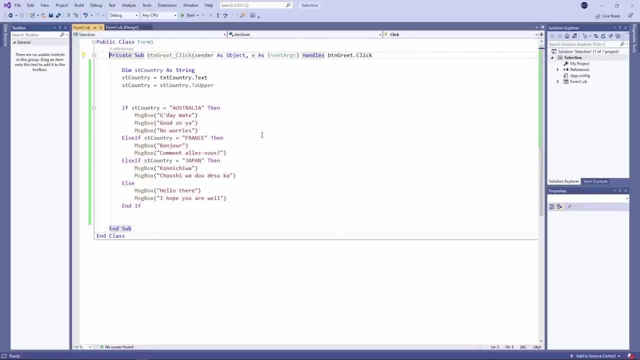 And notice how execution has passed to the end of the if block. Because the Australian greetings have been displayed, there's no need to perform these other tests. One final thing to say: I've converted the user's input into uppercase and I might not. 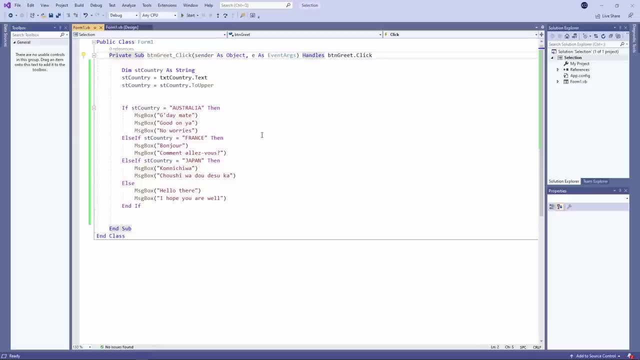 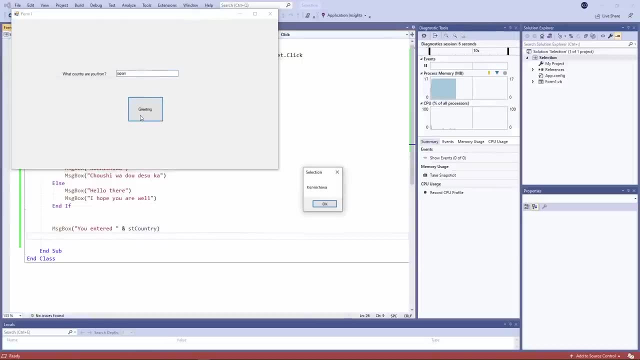 want to leave it in uppercase. Notice this: Once the if block has completed any code which comes after, it then executes, For example, this message box statement: But notice that ST country now contains uppercase Japan. I might want to leave it the way it was when it was input by the user. 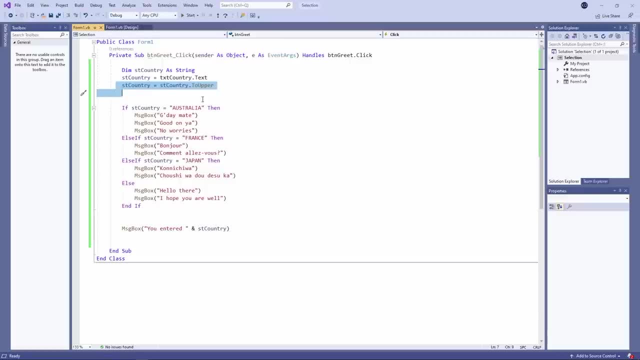 So, rather than doing this, Which replaces the existing contents of the variable, I'm going to do this. The content of the variable is only being converted to uppercase for the purpose of the test, But I'm not reassigning the uppercase text back into the variable. 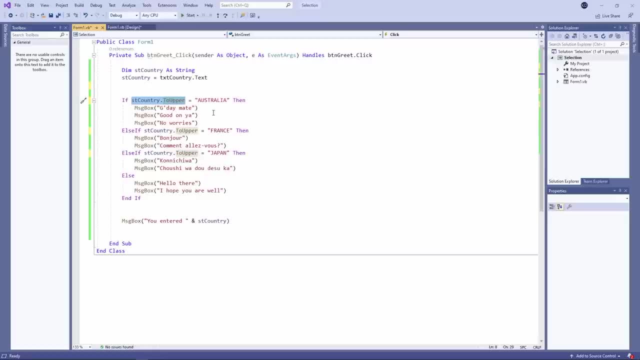 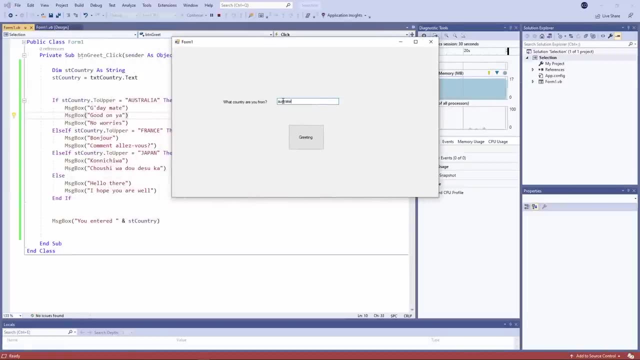 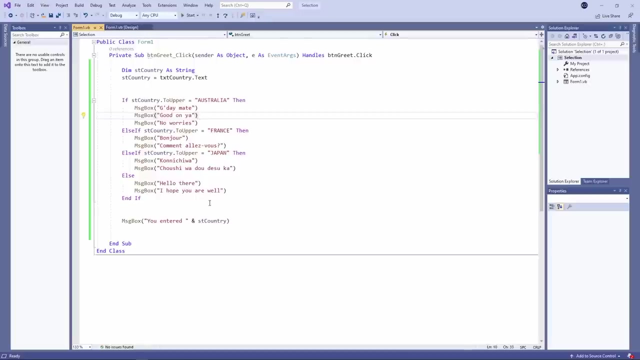 I'm converting the text to uppercase on the fly, as it were. Watch what happens now. By the time we get to the end of the program, the contents of the variable are still in their original state. You might like to try writing a similar program yourself. 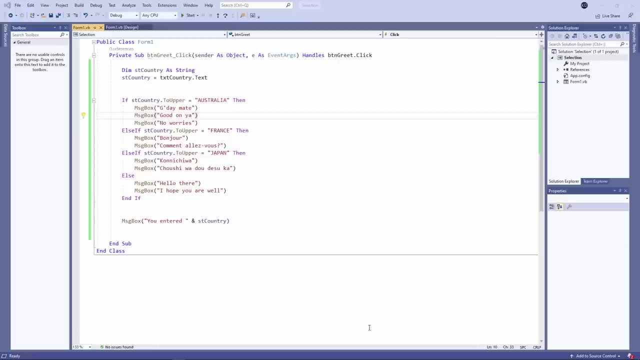 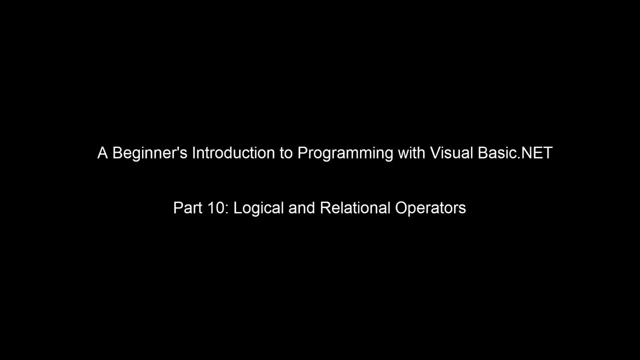 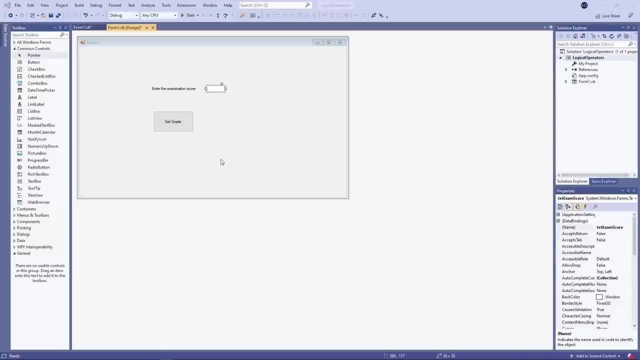 Have a single if block with lots of else: if clauses to greet people from different countries. In the previous video of this series, I showed you how to use an if block to execute a block of code conditionally, In other words, to decide whether or not to execute a block of code. 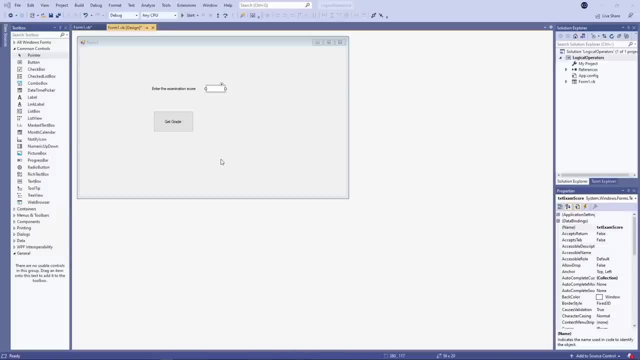 The if block allows you to use one of the three constructs of high level programming languages, namely selection. In this video, I want to say more about the if block And the kind of tests that we can perform with an if block. I've already created a new Windows Forms application. 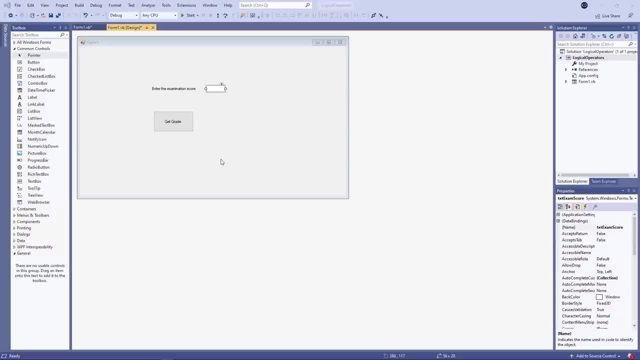 And I've put three controls on the form. I have a label, a text box and a button. Notice that I've named the text box TXT- Exam Score And I've named the button BTN Get Grade. The idea is that the user of this application will type in an exam score. 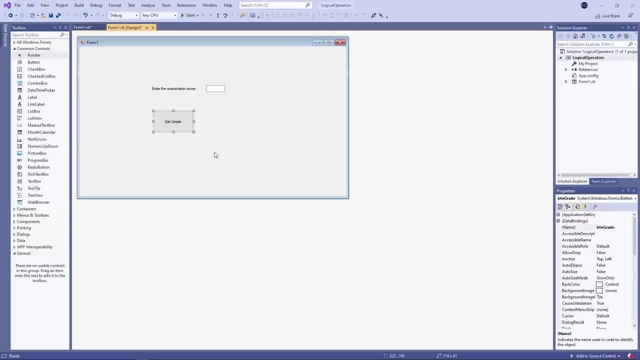 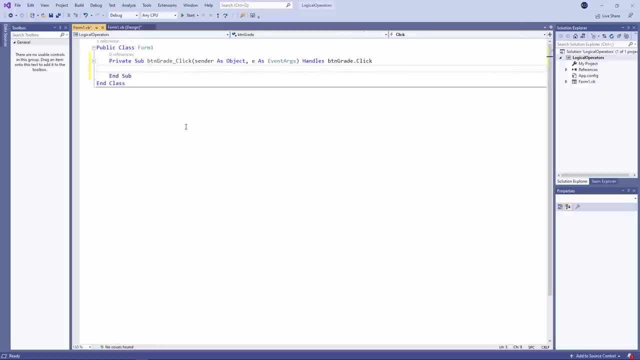 And then the program will calculate the grade. And then the program will calculate the grade. Let's write the code and see how we can use logical operators to build complex conditions. I'll start by capturing the score into a variable. I'm assigning the contents of the text box to an integer variable called iscore. 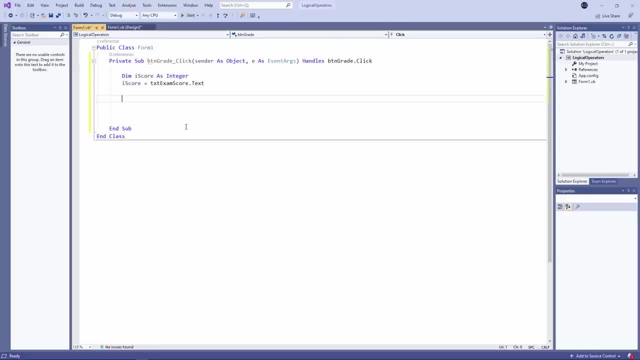 Now the first thing I want to do is check whether it's a valid score. Let's suppose that you can only score between 0 and 100 on this test. There's a few things to notice here. I'm asking if the score is less than zero. This: 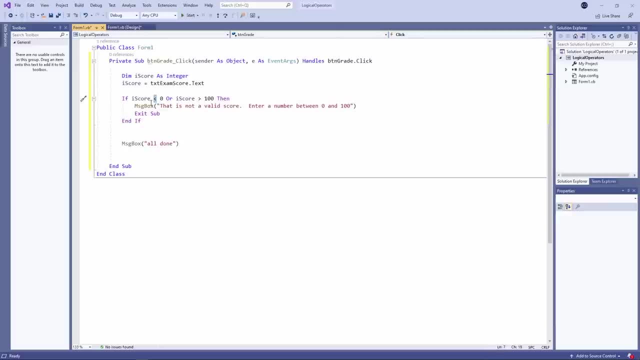 is the less than symbol. And let me be clear: less than zero means minus one, minus two, minus three. Zero is not actually less than zero. Zero is equal to zero. I'm also checking to see if the score is bigger than 100.. Given that you can't score more than 100 on this, 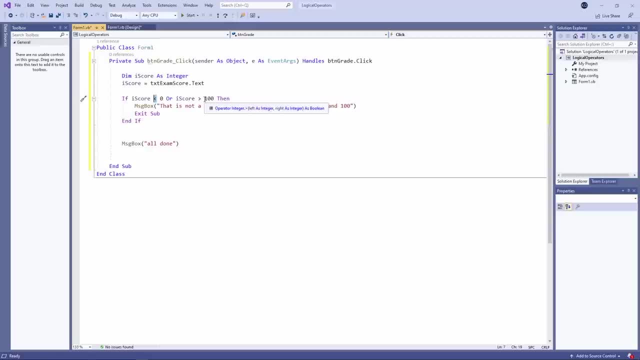 particular exam, anything bigger than 100 would be invalid. If the score is less than zero or the score is greater than 100, then we'll display a message saying this is not a valid score. I'm also giving the user of my application some guidance, I'm not just telling them. 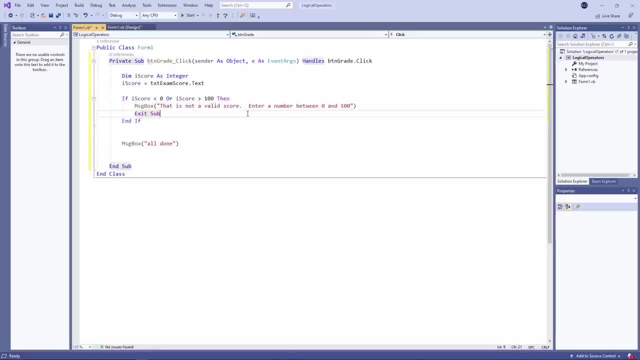 what they did was wrong. I'm telling them what they should do instead, which is good practice for an error message. Then notice I'm exiting the program. I've put another line of code here just to prove the point. When we drop out of the if block, normally this line of code would be executed. 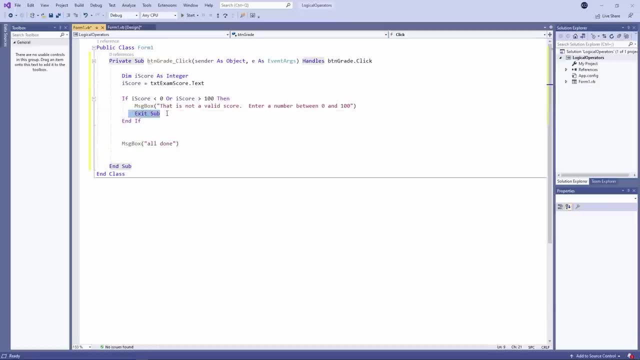 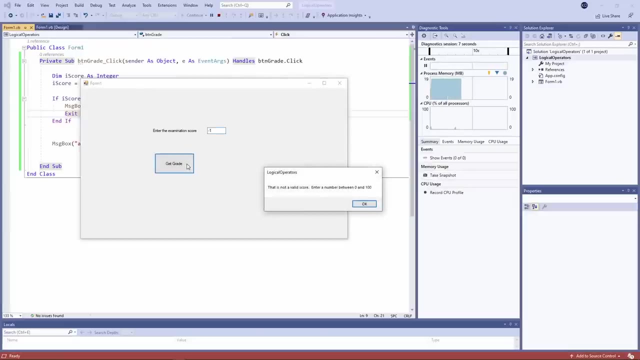 But because I've said exit sub, this will force the program to stop there, and then Let's give it a try. If I type a score of, let's say, minus one, this is not a valid score. I'm getting the. 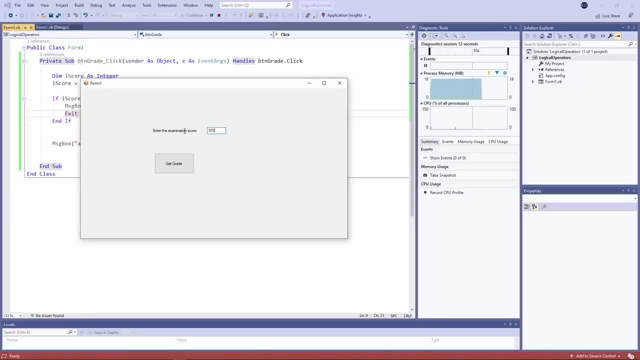 error message. Let's try a score of 101.. Again, not a valid score. Let's try a score of 99.. And I want you to notice that we've dropped out of the if block and we're going to have to start getting that message at the end of the program saying all done, It hasn't actually. 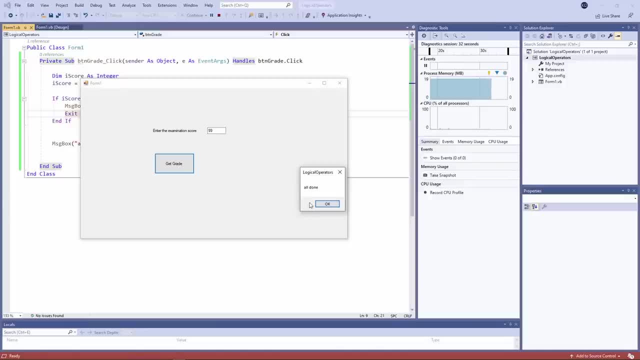 done anything yet. We'll deal with that in a moment. Just to be sure, I should really test the value zero. Zero is valid, Zero is a perfectly good value, And I should also test the value 100.. And that's fine as well. 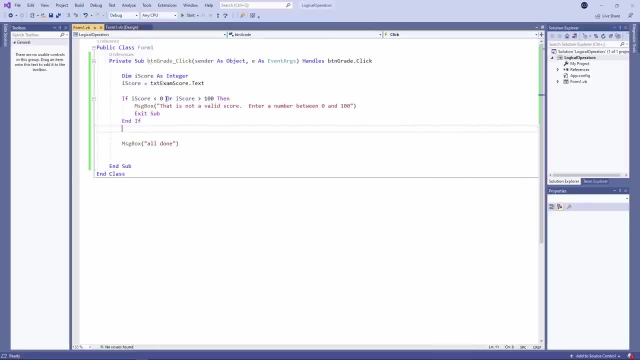 So that's the beginning of my exam checker program And I'm using something called the test checker. I'm using something called a logical operator. The word or is one of three logical operators which you'll come across. The less than symbol and the greater than symbol are called relational. 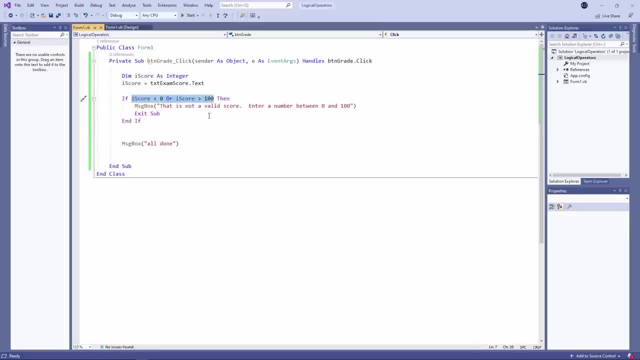 operators. That is the condition clause of my if statement, And because it's effectively performing more than one test, we call it a complex condition. Now, before I try and work out what the grade for a particular score is, I'm going to keep 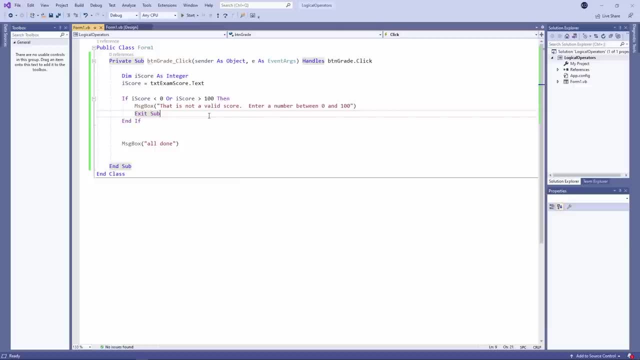 it really simple and just test to see whether somebody has passed or failed. So if the score is bigger than or equal to 50, it's a pass. If the score is less than 50, it's a fail. Notice the greater than or equal to symbol. 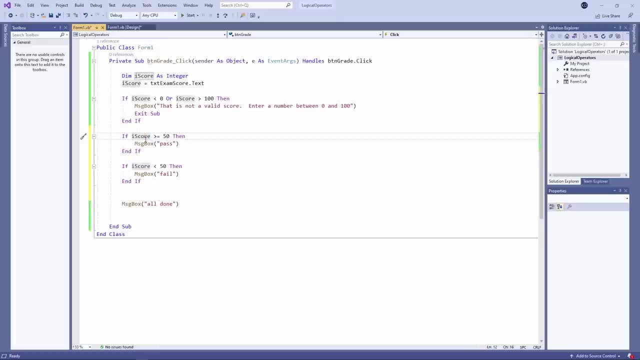 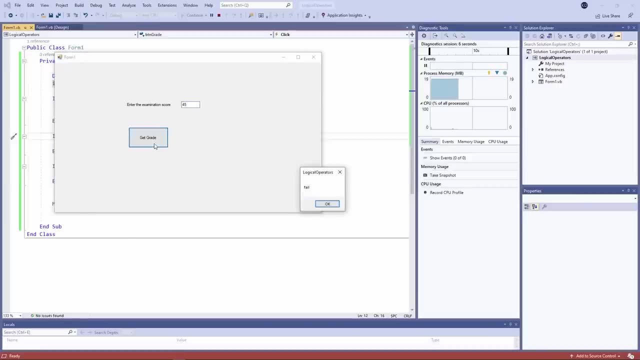 That's another relational operator. Let's give it a whirl. A score of 45 is a fail. And notice: all done is being displayed unconditionally. That's going to happen one way or the other. A score of 55 is a pass. 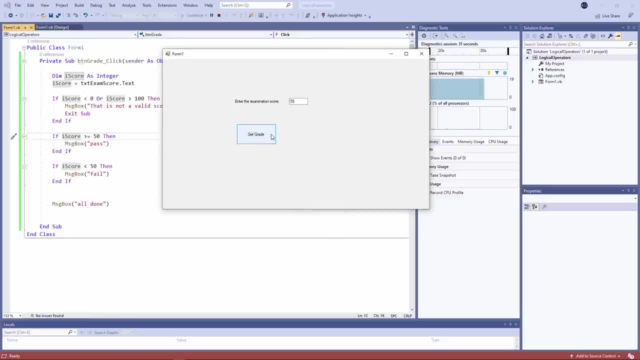 Now it's good practice, when you're testing a program like this, to try all of the boundary values, And by boundary values I mean: 50 is a boundary, 100 is a boundary, Zero is a boundary, So let's try a score of 50.. 50 is a pass. 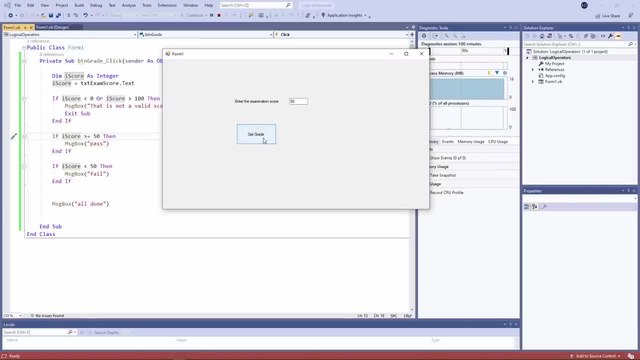 It's also a good idea to test parts of the program that we've already tested, Because when you add new code you might introduce bugs. I'm going to test less than zero again. Minus five is not valid, And neither is 105. It. 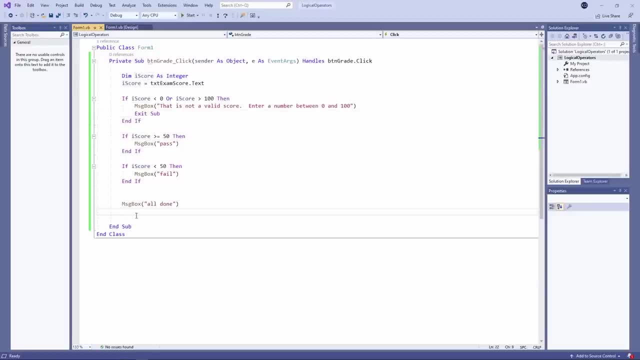 seems to be working. Now. you might have already noticed that I've used three separate if blocks. In the previous video, I showed you one if block with multiple else if clauses, And I'd like to point out the difference between the two. I'm going to set up a new block. I'm going to set up a new block And I'm going to set. 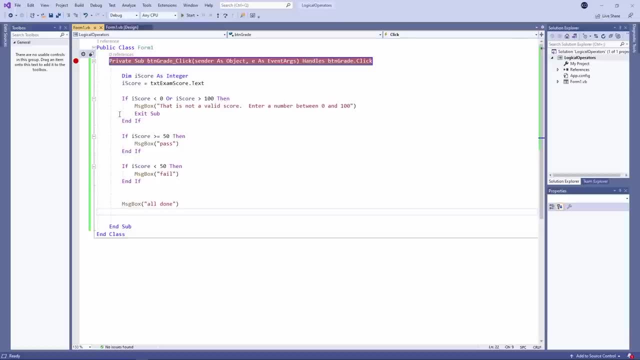 up a new block And I'm going to set up a new block And I'm going to set up a new block. I'm going to set a breakpoint on this program. I'm going to run it up again. I'm going to. 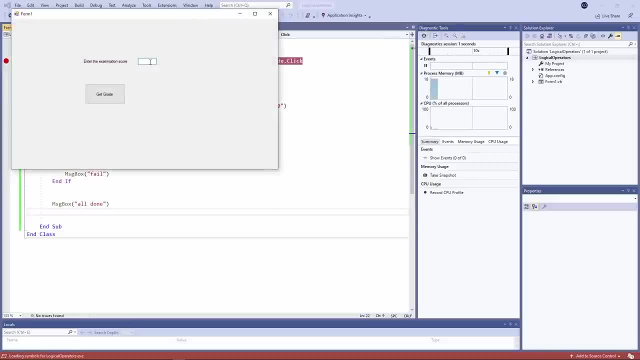 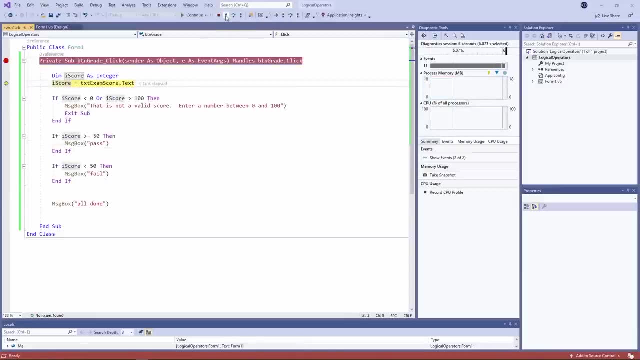 put in a failing score, Let's say 30. And then I'll step through the code. So we assign the contents of the text box to the variable. We check to see if the contents of the variable are within range. In this case they are. 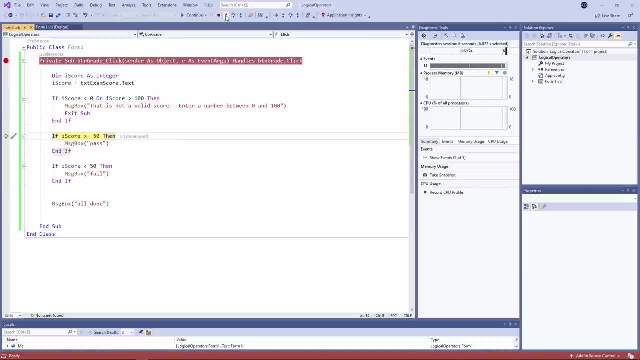 so we jump to the end of this if block. Then we check to see if the score is greater than or equal to 50, which it isn't. so we jump to the end of this if block. and then, finally, we check to see if the score is less than 50, which it is. 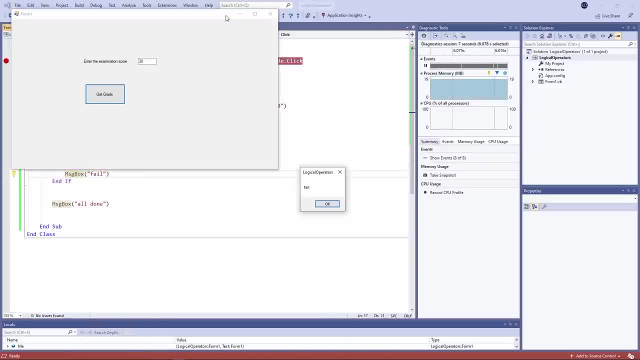 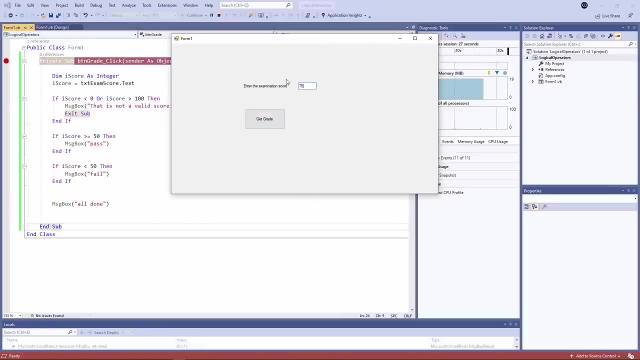 and we report that it's a fail. all done, let's do that again, but this time I'm going to put in a passing score, let's say 75. assign the content of the text box to the variable. check that it's in range, which of course it is. so we jump to the end of the first if block. 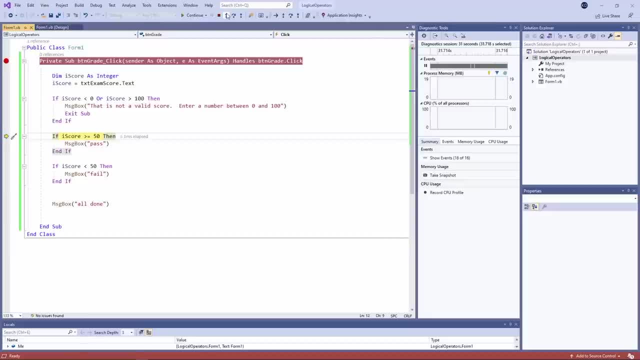 check to see if the score is bigger than or equal to 50, which it is report that it's a pass. and now we're checking to see if the score is less than 50, which of course is unnecessary. we're doing a test that's a fail. and now we're checking to see if the score is less than 50, which of course is unnecessary. we're doing a test that. 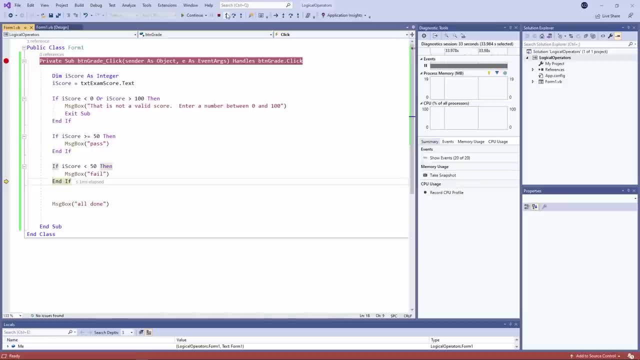 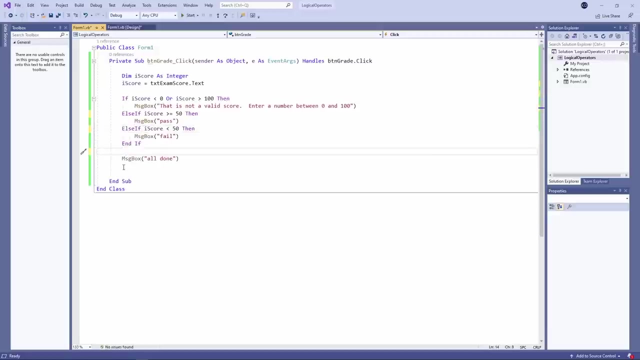 we don't need to do. we've already established that it's a pass. to make my program more efficient, I'm going to use a single if block with multiple else ifs. my validation test, where I check to see that the score was actually within range. my validation test, where I check to see that the score was actually within range. 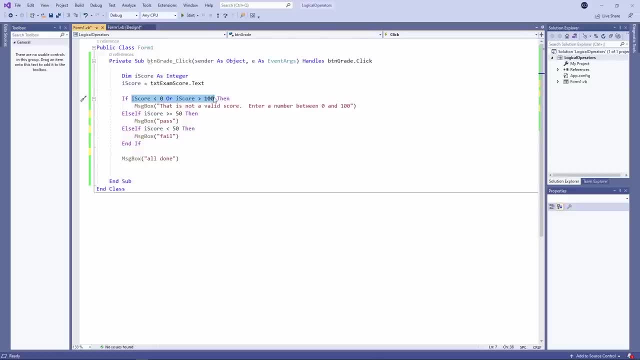 could have left as a completely separate if block, but don't forget there could have left as a completely separate if block, but don't forget there was an exit sub in there and it may well be that there's some code I want to was an exit sub in there and it may well be that there's some code I want to. 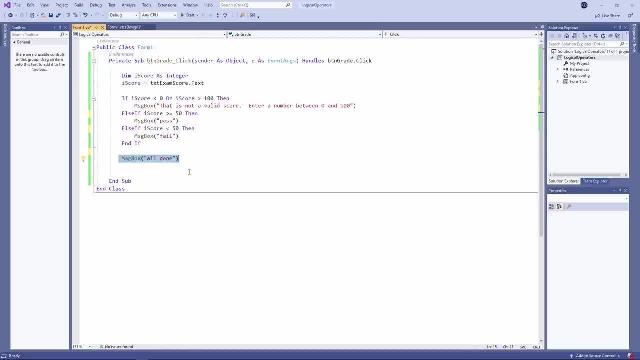 execute unconditionally at the bottom of the program if you use exit sub early on. execute unconditionally at the bottom of the program if you use exit sub early on. that won't happen, so I've included this as well inside the if block with. that won't happen, so I've included this as well inside the if block with. 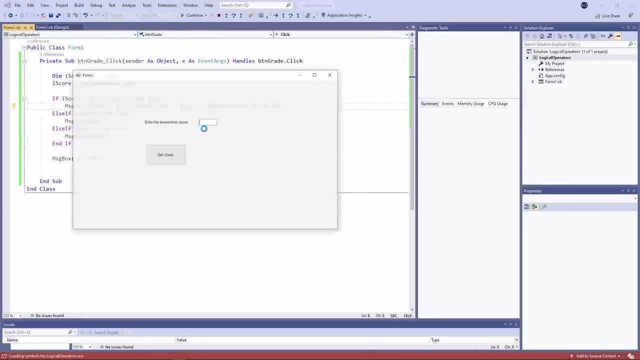 multiple. else, ifs, let's give it a go. multiple, else, ifs, let's give it a go. multiple, else ifs, let's give it a go. a score of 67 is a pass, all done, let's. a score of 67 is a pass, all done, let's. 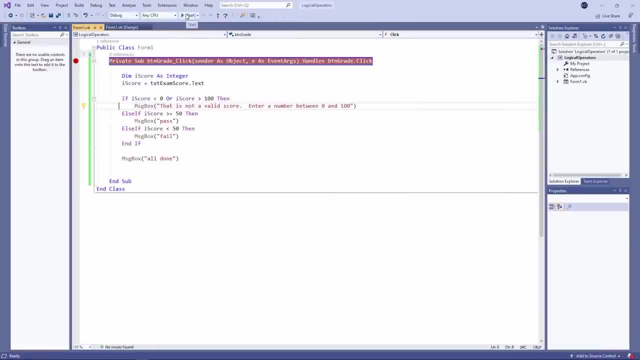 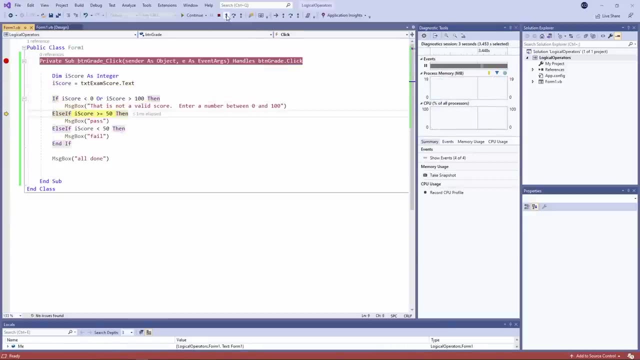 a score of 67 is a pass. all done. let's step through it and watch what's step through it and watch what's step through it and watch what's happening. the score is in range, the score is bigger. the score is in range, the score is bigger. 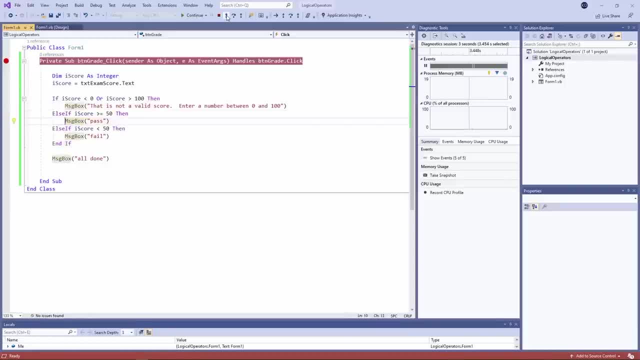 the score is in range. the score is bigger than or equal to 50, so we report a pass than or equal to 50, so we report a pass than or equal to 50, so we report a pass and then we drop out of the if block. we. 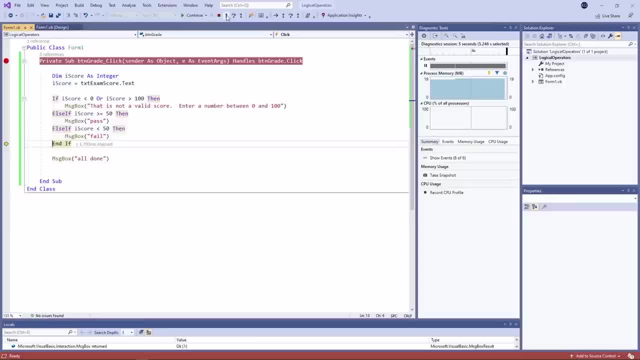 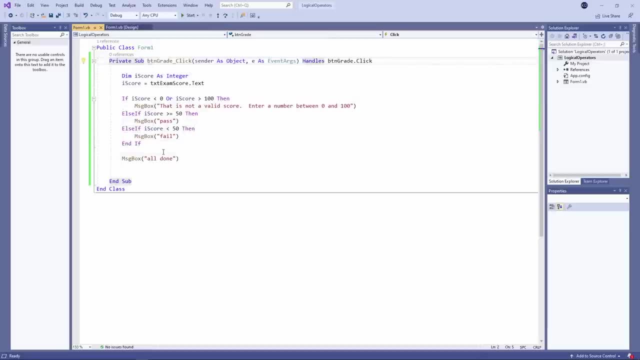 and then we drop out of the if block. we, and then we drop out of the if block. we don't need to do any more tests. so, although it's perfectly reasonable to so, although it's perfectly reasonable to so, although it's perfectly reasonable to have multiple if blocks, each performing a 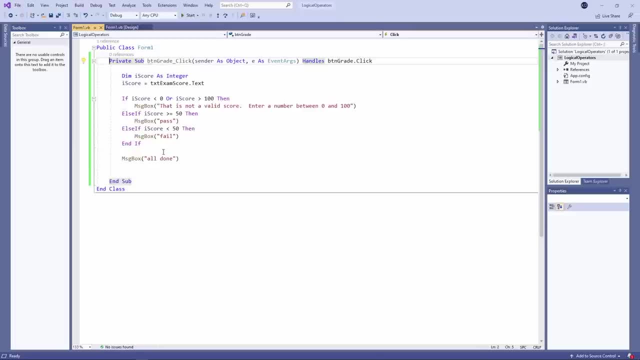 have multiple. if blocks each performing a have multiple. if blocks each performing a separate test, it may be better to use a separate test. it may be better to use a separate test. it may be better to use a single if block with multiple, else ifs. single if block with multiple, else ifs. 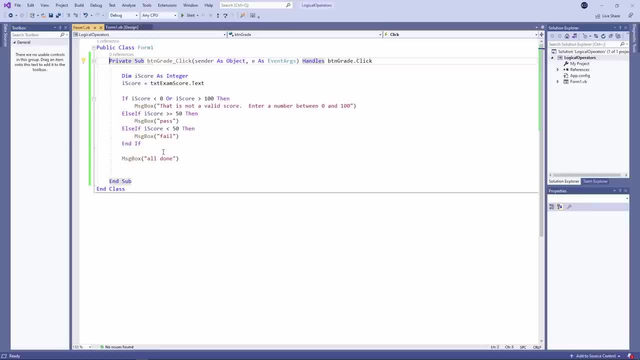 single if block with multiple else ifs, and then the program doesn't have to, and then the program doesn't have to, and then the program doesn't have to work as hard now, admittedly, with a work as hard now, admittedly, with a work as hard now, admittedly, with a little program like this, I'm not going to. 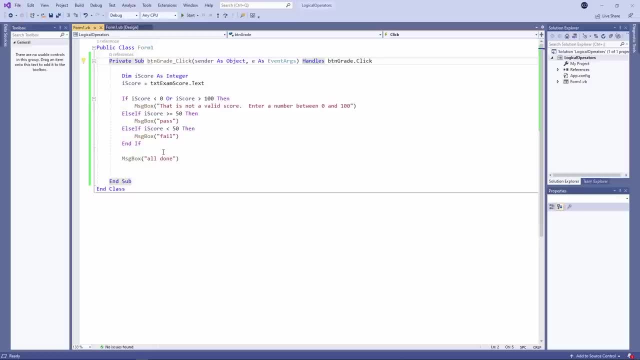 little program like this, I'm not going to little program like this. I'm not going to notice a lot of difference. but as you notice a lot of difference. but as you notice a lot of difference. but as you start writing longer, more complex, start writing longer, more complex. 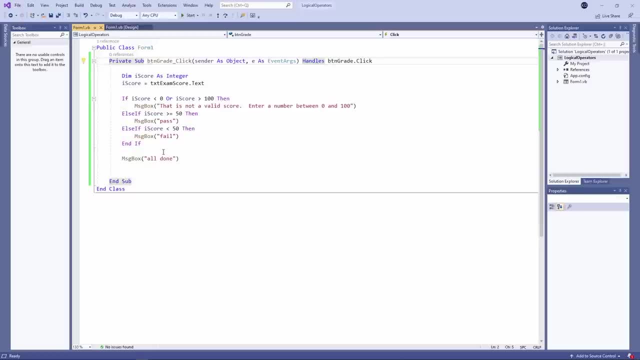 start writing longer, more complex programs, then small adjustments will add programs, then small adjustments will add programs. then small adjustments will add up and your program will run faster- okay, up and your program will run faster- okay, up and your program will run faster- okay, it's one thing writing a program. that 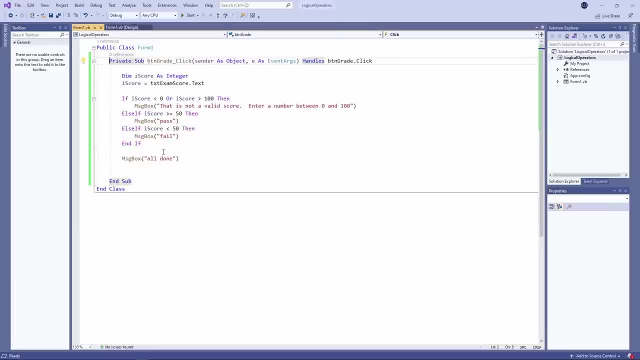 it's one thing writing a program that. it's one thing writing a program that works efficiently, but it also has to be works efficiently. but it also has to be works efficiently, but it also has to be robust. we want a program that you can't robust. we want a program that you can't. 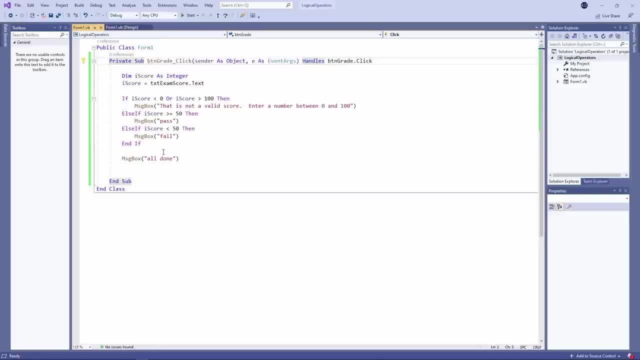 robust. we want a program that you can't crash and I can crash this one easily. crash and I can crash this one easily. crash and I can crash this one easily. watch, watch, watch. I'm typing text into the text box. I'm typing text into the text box. 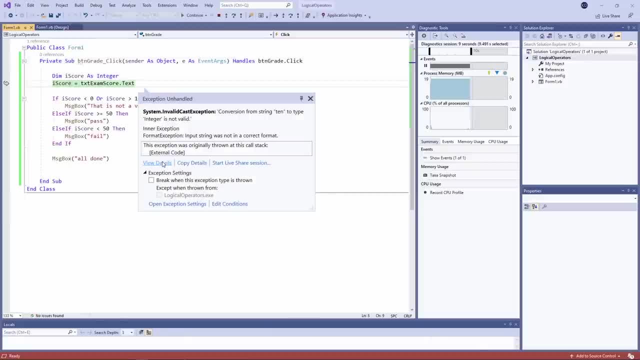 I'm typing text into the text box rather than a number, rather than a number, rather than a number. invalid cast exception. conversion from invalid cast exception. conversion from invalid cast exception. conversion from string 10 to type integer is not valid. string 10 to type integer is not valid. 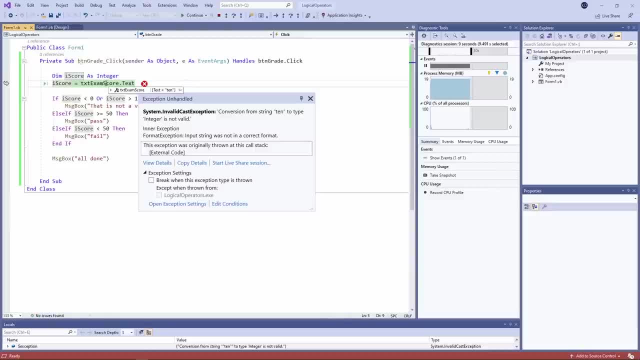 string 10 to type integer is not valid. this makes the point that when you type this makes the point that when you type this makes the point that when you type something into a text box, it's a string, something into a text box, it's a string. 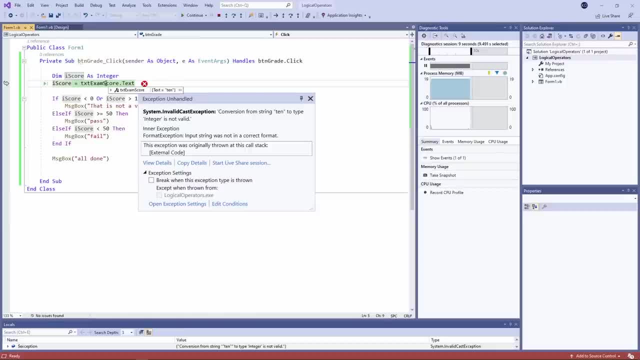 something into a text box. it's a string. there's the word 10 with double quotes. there's the word 10 with double quotes. there's the word 10 with double quotes around it, and I'm trying to put that around it, and I'm trying to put that. 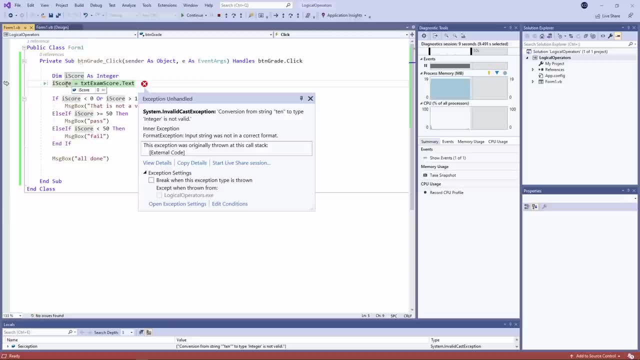 around it and I'm trying to put that string into a variable that's designed string into a variable that's designed string into a variable that's designed to hold integers, whole numbers. I'll run to hold integers, whole numbers. I'll run to hold integers, whole numbers. I'll run the program again with a breakpoint, but 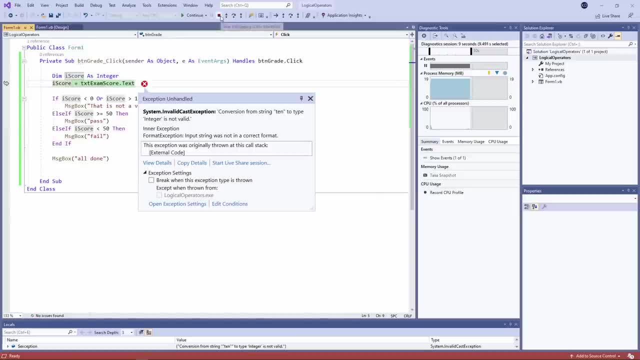 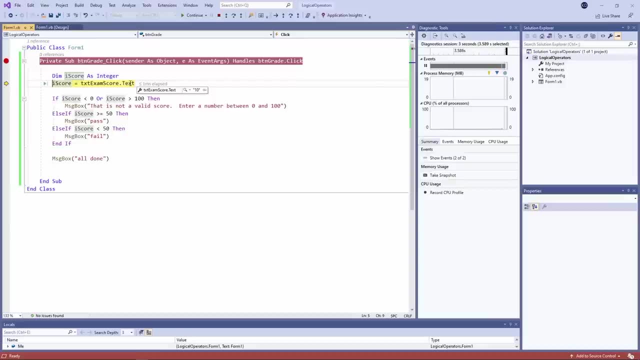 the program again with a breakpoint. but the program, again with a breakpoint. but this time I'll be a well-behaved user. this time I'll be a well-behaved user. this time, I'll be a well-behaved user. notice that the text box contains the 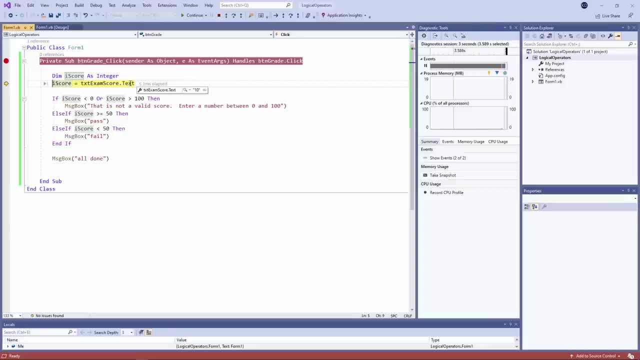 notice that the text box contains the notice that the text box contains the string 10. the text box does not contain string 10. the text box does not contain string 10. the text box does not contain a number. it's a string of characters but a number. it's a string of characters, but. 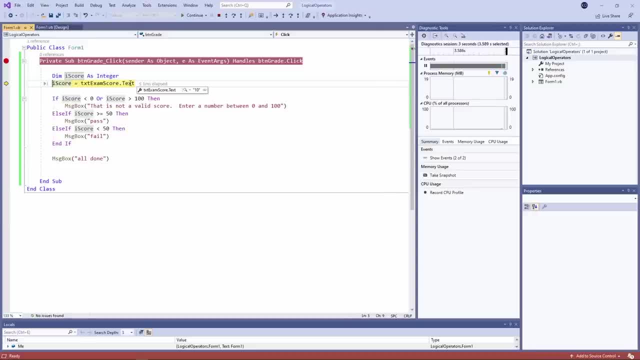 a number. it's a string of characters, but because I'm trying to assign it to an, because I'm trying to assign it to an, because I'm trying to assign it to an integer variable VB will attempt to integer variable. VB will attempt to integer variable. VB will attempt to convert it into an integer. and the 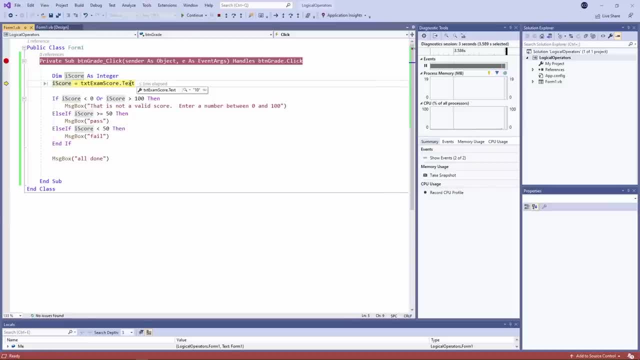 convert it into an integer and the convert it into an integer and the string 1: 0 can be converted into the string 1: 0 can be converted into the string 1: 0 can be converted into the number 10, so everything is fine. the. 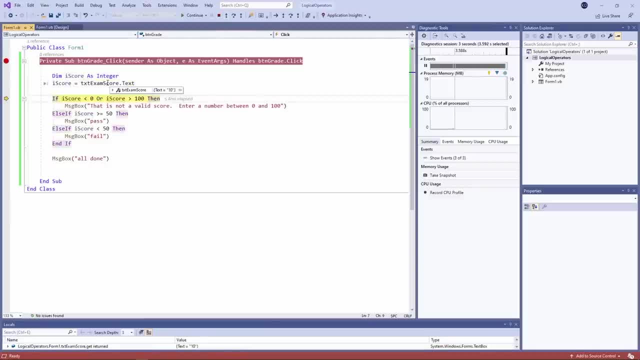 number 10, so everything is fine. the number 10, so everything is fine. the program does not crash. the text 1: 0 in program does not crash. the text 1: 0 in program does not crash. the text 1: 0 in double quotes has been converted into: 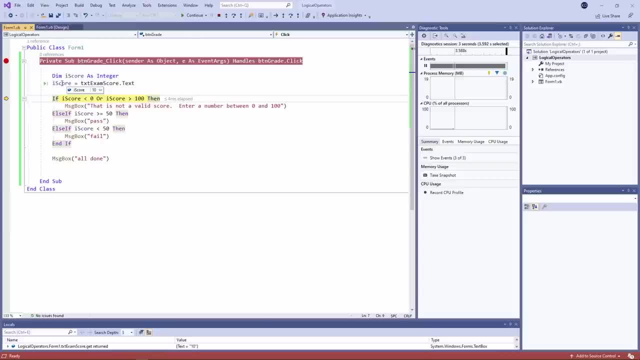 double quotes has been converted into double quotes has been converted into the number 10 converting data from one. the number 10 converting data from one. the number 10 converting data from one type to another is called casting and type to another is called casting and type to another is called casting. and VB was able to do the cast. let's run it. 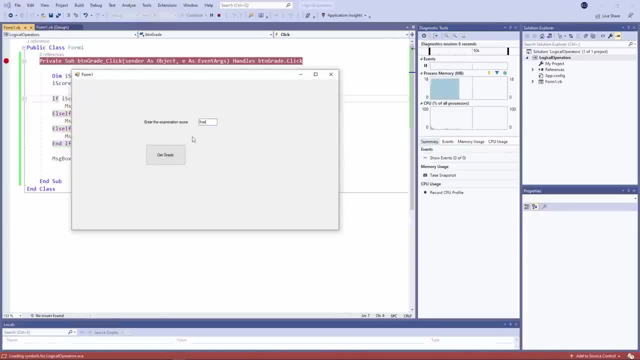 VB was able to do the cast, let's run it. VB was able to do the cast. let's run it again with something it can't handle. VB again with something it can't handle. VB again with something it can't handle. VB will attempt to convert the string F IV. 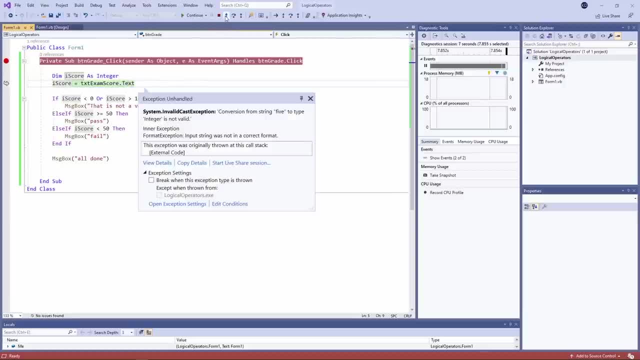 will attempt to convert the string F IV. will attempt to convert the string F IV e into a number, and of course that is an e into a number, and of course that is an e into a number, and of course that is an invalid cast. it can't do it the last. 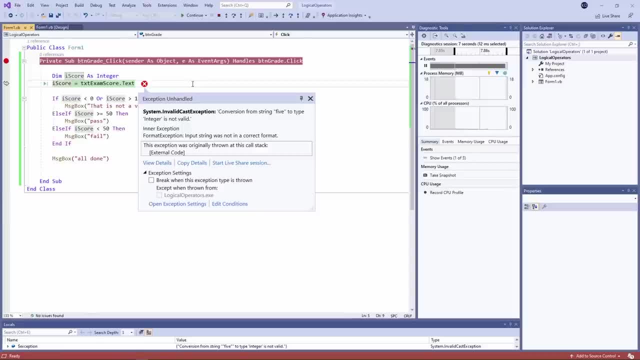 invalid cast: it can't do it. the last invalid cast: it can't do it. the last thing I want to do is give my program to. thing I want to do is give my program to. thing I want to do is give my program to a user who can inadvertently crash it. so 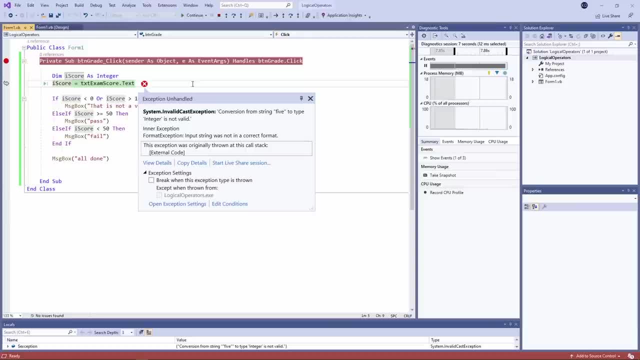 a user who can inadvertently crash it. so a user who can inadvertently crash it. so let's add some extra code to get around. let's add some extra code to get around. let's add some extra code to get around this problem. before I attempt to this problem, before I attempt to 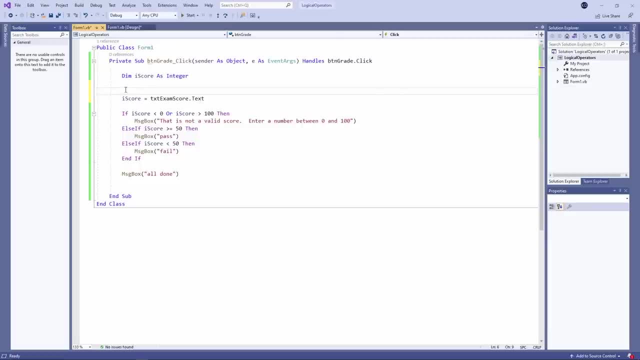 this problem. before I attempt to initialize the variable, I score with the. initialize the variable. I score with the. initialize the variable. I score with the contents of the text box. I'm going to contents of the text box. I'm going to contents of the text box. I'm going to test to see whether or not VB will be. 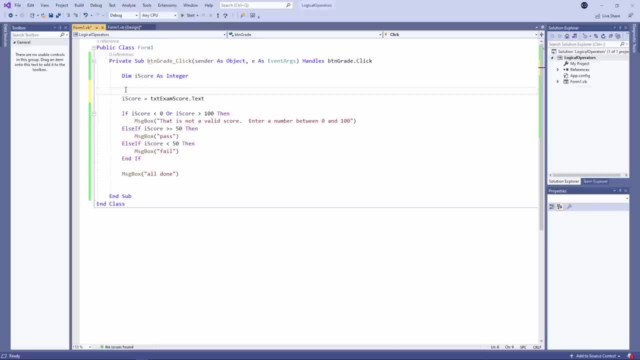 test to see whether or not VB will be. test to see whether or not VB will be able to convert it into a number. like able to convert it into a number. like able to convert it into a number like this is numeric, is a special built-in. this is numeric, is a special built-in. 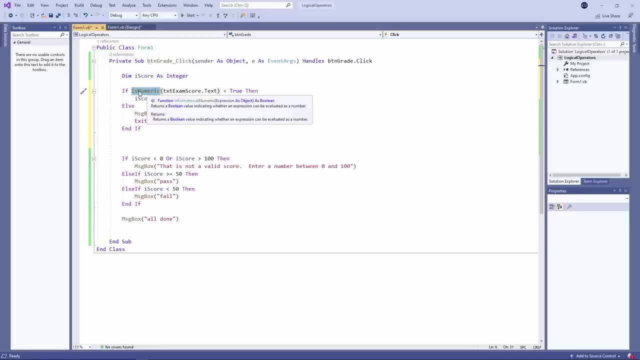 this is numeric, is a special built-in function which will allow me to test function, which will allow me to test function which will allow me to test whether or not something can be converted, whether or not something can be converted, whether or not something can be converted into a number. in this case, I'm testing. 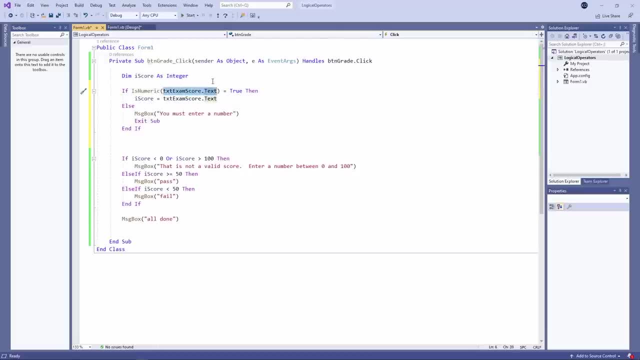 into a number. in this case, I'm testing into a number. in this case, I'm testing the contents of the text box. let me be the contents of the text box. let me be the contents of the text box. let me be clear: it doesn't convert it into a. 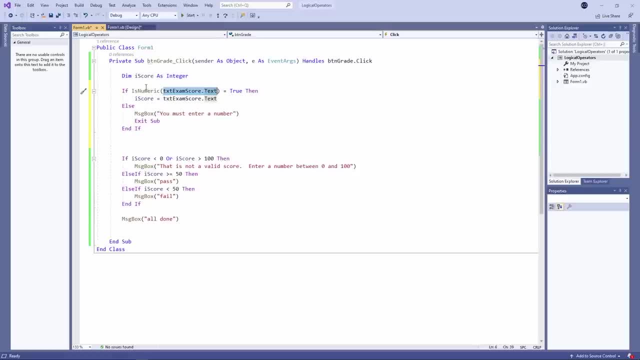 clear. it doesn't convert it into a clear. it doesn't convert it into a number. it simply asks the question: can number? it simply asks the question: can number? it simply asks the question: can it be converted into a number when I? it be converted into a number when I? 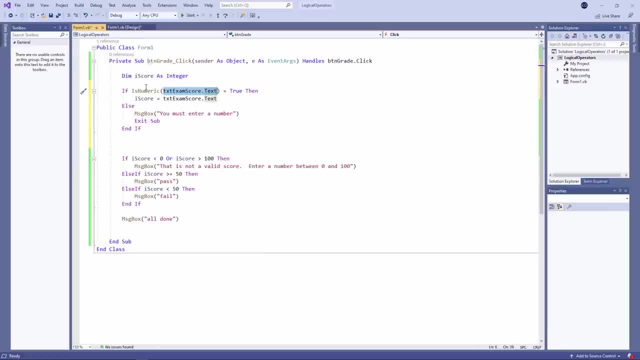 it be converted into a number when I perform this test. the outcome will perform this test. the outcome will perform this test. the outcome will either be true if it can be converted, or either be true if it can be converted, or either be true if it can be converted or false if it can't. so I'm saying if is. 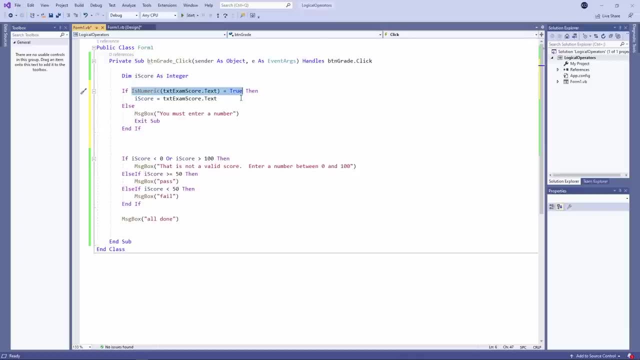 false. if it can't, so I'm saying: if is false, if it can't, so I'm saying: if is numeric equals true, if it can be numeric equals true, if it can be numeric equals true, if it can be converted into a number, then I will do. 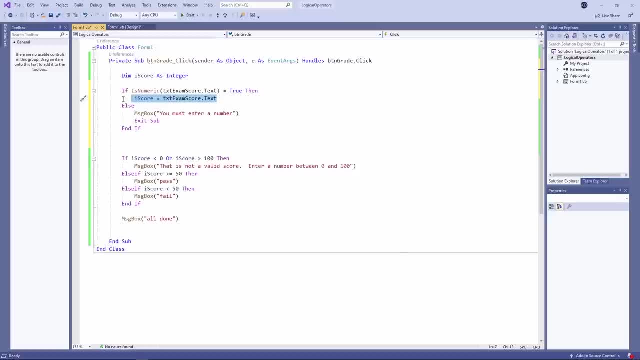 converted into a number, then I will do converted into a number, then I will do this line of code. I'm initializing the this line of code. I'm initializing the this line of code. I'm initializing the variable conditionally if it can't be variable conditionally. if it can't be. 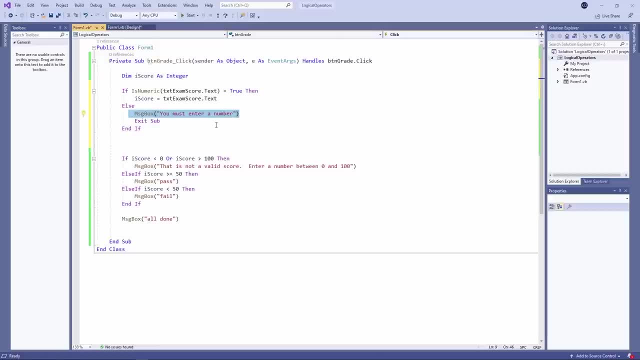 variable conditionally. if it can't be converted, then I give an appropriate converted, then I give an appropriate converted, then I give an appropriate error message and I am exiting the error message. and I am exiting the error message. and I am exiting the program this time because there isn't. 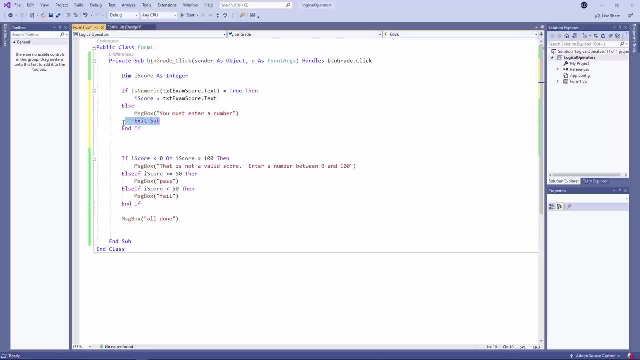 program this time. because there isn't program this time? because there isn't much I can do with that data. unless it is much, I can do with that data. unless it is much, I can do with that data, unless it is actually a number. so there's my little. 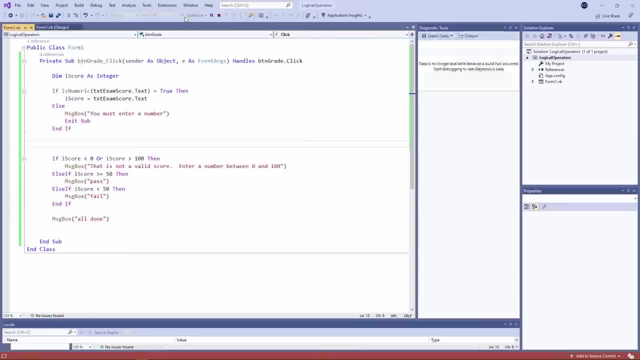 actually a number. so there's my little, actually a number. so there's my little validation routine. let's give it a go. validation routine. let's give it a go. validation routine. let's give it a go. type in some text. you must enter a type. in some text, you must enter a. 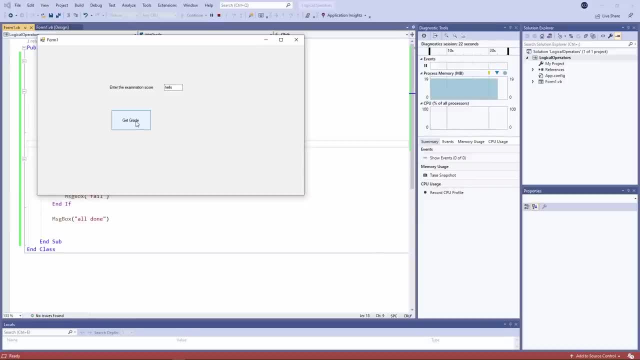 type in some text. you must enter a number and I'm not getting the all done number. and I'm not getting the all done number. and I'm not getting the all done message because I've forced an exit from message because I've forced an exit from. 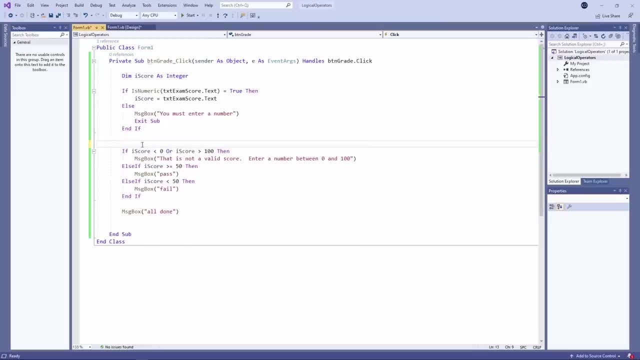 message because I've forced an exit from the program. now there's one more thing: I the program. now. there's one more thing: I the program. now there's one more thing I can do just to improve the efficiency of, can do just to improve the efficiency of. 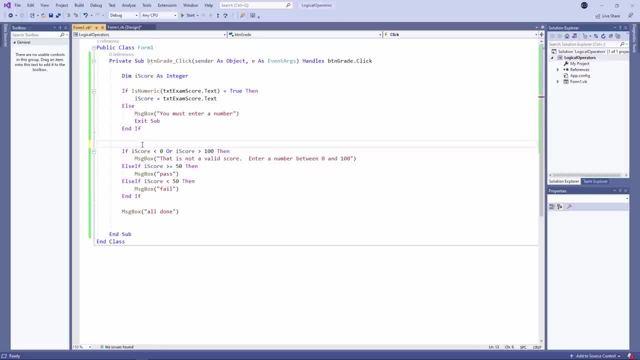 can do just to improve the efficiency of the program a little bit. and that's to the program a little bit, and that's to the program a little bit. and that's to tell VB that I want to convert the. tell VB that I want to convert the. 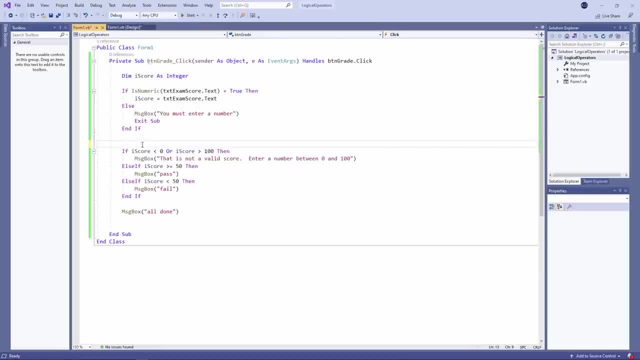 tell VB that I want to convert the contents of the text box into an integer. contents of the text box into an integer. contents of the text box into an integer. rather than allowing VB to make the, rather than allowing VB to make the, rather than allowing VB to make the decision for me, and I can do it like. 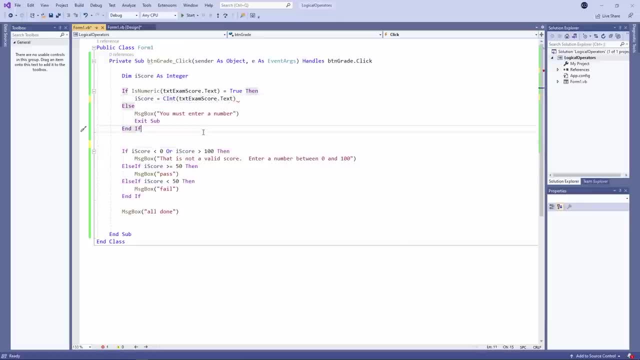 decision for me and I can do it like decision for me and I can do it like this: see int is short for convert to this, see int is short for convert to this, see int is short for convert to integer, and of course my program is only integer and of course my program is only 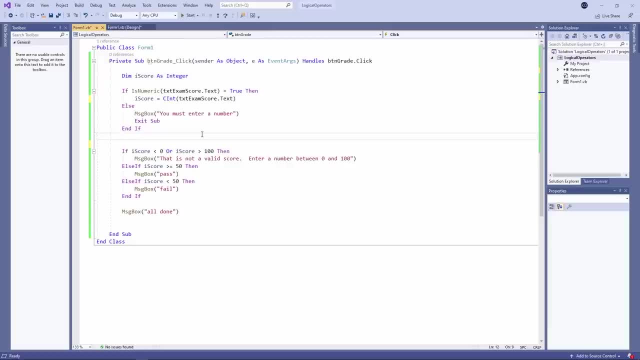 integer. and of course, my program is only going to do this. if it can, I've already going to do this. if it can, I've already going to do this. if it can, I've already made sure of that with my is numeric. made sure of that with my is numeric. 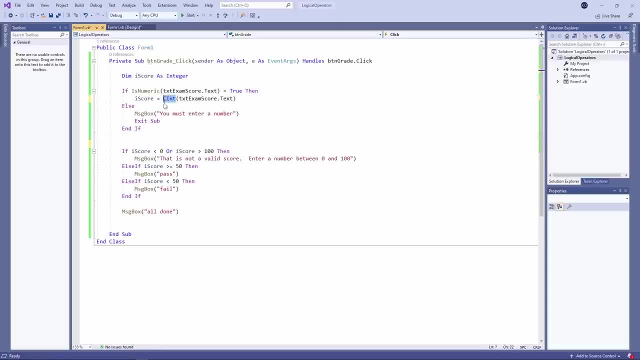 made sure of that with my is numeric test. if I left this out, it would still test. if I left this out, it would still test. if I left this out, it would still work. but I'm leaving it up to VB to work. but I'm leaving it up to VB to. 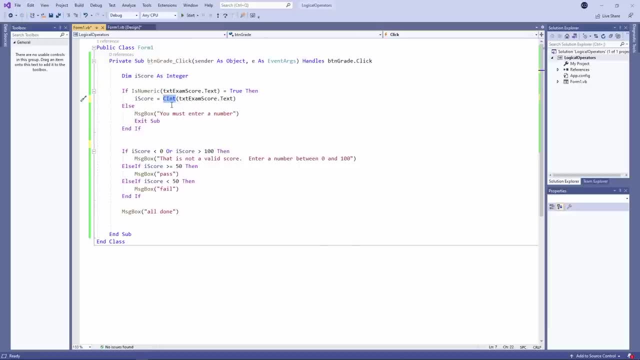 work, but I'm leaving it up to VB to decide what to convert the contents of. decide what to convert the contents of. decide what to convert the contents of the text box into an integer- a double a. the text box into an integer- a double a. the text box into an integer- a double, a single. and it will make that decision. 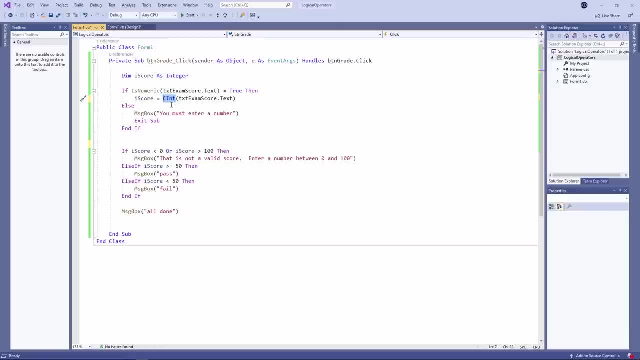 single and it will make that decision single. and it will make that decision based on the variables data type. I'm based on the variables data type. I'm based on the variables data type. I'm just taking the decision out of VB's. just taking the decision out of VB's. 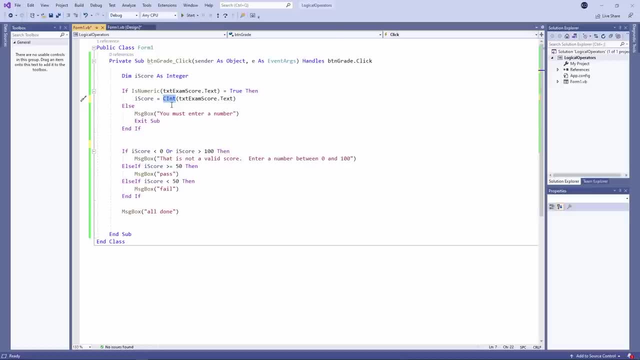 just taking the decision out of VB's hands and it will result in a very hands and it will result in a very hands and it will result in a very slight improvement in performance. I'll slight improvement in performance. I'll slight improvement in performance. I'll talk more about special inbuilt. 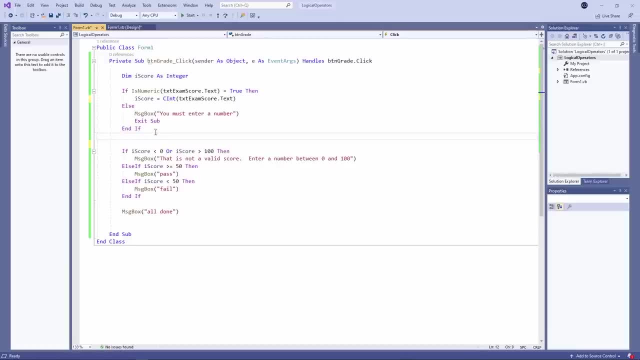 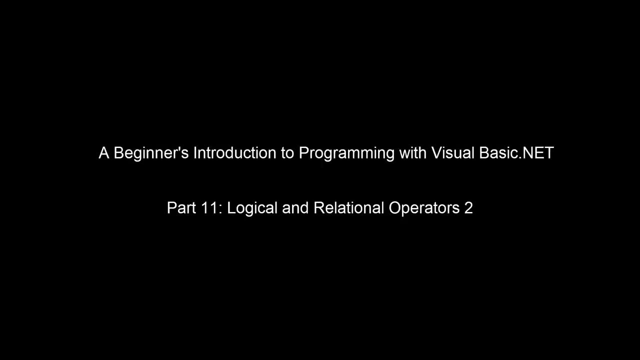 talk more about special inbuilt. talk more about special inbuilt functions in another video. but you've functions in another video. but you've functions in another video. but you've seen two already is numeric and see int. seen two already is numeric and see int. seen two already is numeric and see int. in the previous video I showed you how 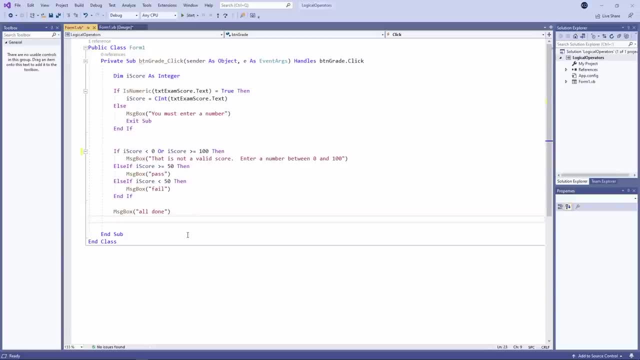 in the previous video I showed you how. in the previous video, I showed you how to write this little routine to check if to write this little routine, to check if to write this little routine to check if an exam score was a passing score or a- an exam score was a passing score or a. 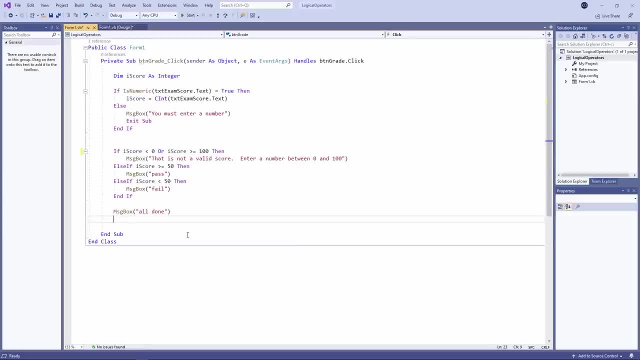 an exam score was a passing score or a failing score. I made use of one of three failing score. I made use of one of three failing score. I made use of one of three logical operators. I used the or operator logical operators. I used the or operator logical operators. I used the or operator. in this video I want to say a little bit. 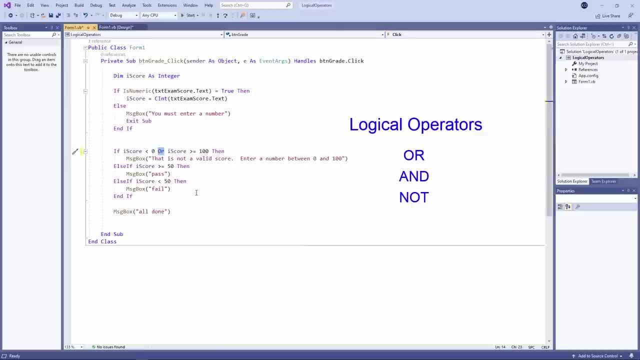 in this video. I want to say a little bit in this video. I want to say a little bit about the other two logical operators. about the other two logical operators. about the other two logical operators, namely and, and not. I'll be adding more. namely, and and not I'll be adding more. 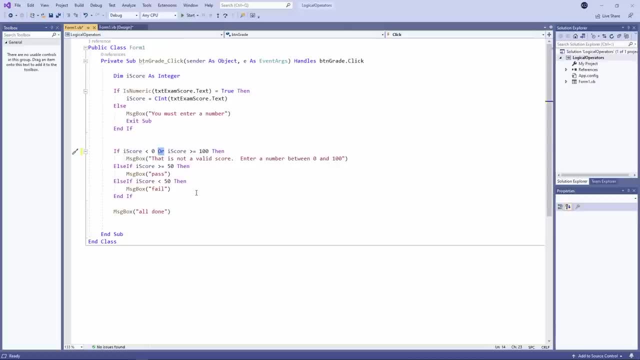 namely and and not. I'll be adding more else. if clauses to my if block to come, else if clauses to my if block to come, else if clauses to my if block to come up with a grade for a particular score. up with a grade for a particular score. 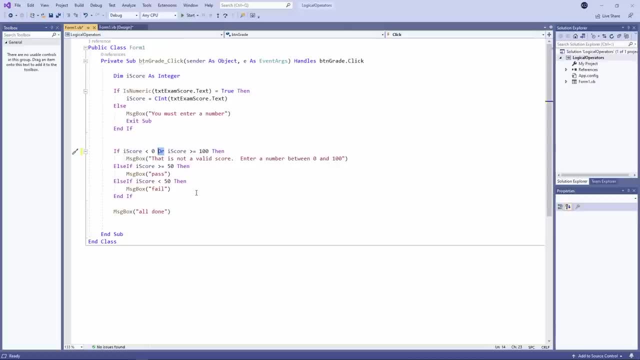 up with a grade for a particular score rather than just pass or fail in the, rather than just pass or fail in the, rather than just pass or fail. in the previous video, I also paid particular previous video. I also paid particular previous video. I also paid particular attention to validating the users input. 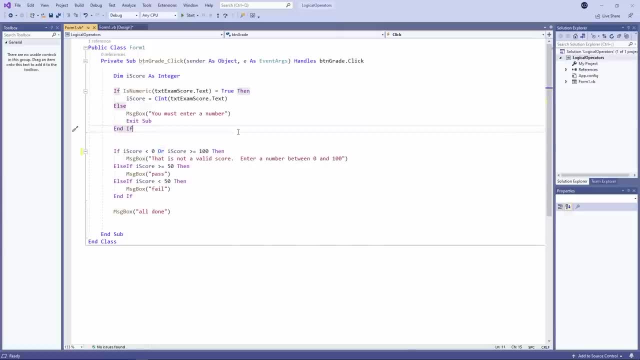 attention to validating the users input. attention to validating the users input. you can see my program has an if block. you can see my program has an if block. you can see my program has an if block right at the start to check if the right at the start to check if the 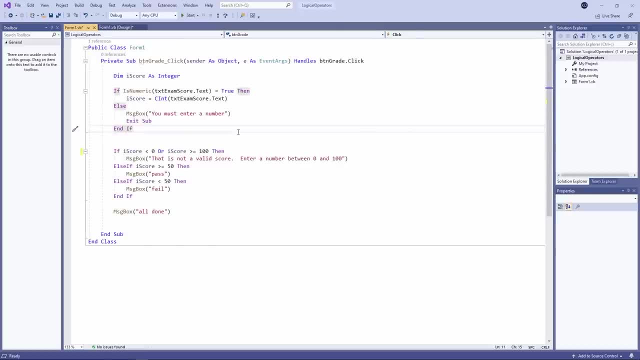 right at the start to check if the users input can be converted into a. users input can be converted into a. users input can be converted into a number, and if it can, then it does it number, and if it can, then it does it number, and if it can, then it does it converts it into an integer. I've 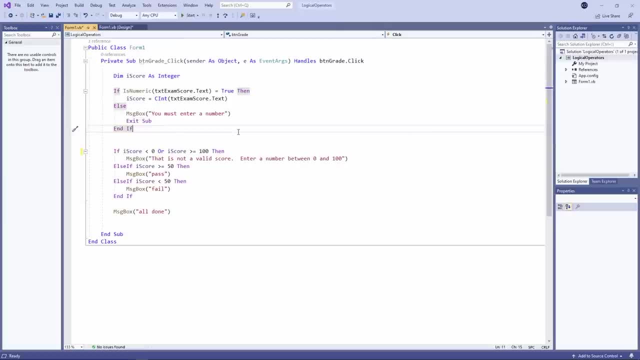 converts it into an integer. I've converts it into an integer. I've explicitly performed the type conversion. explicitly performed the type conversion. explicitly performed the type conversion. also known as a cast using the C into, also known as a cast using the C into, also known as a cast using the C into function. if I hadn't used C int, then VB. 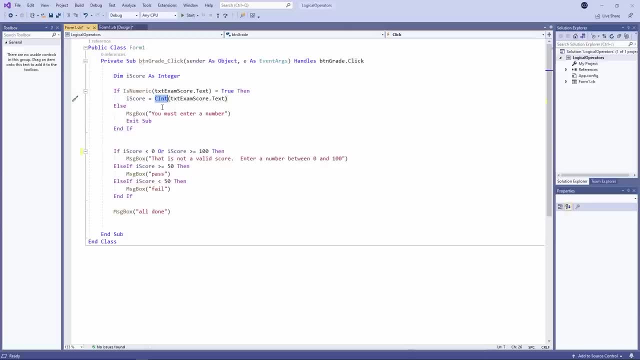 function. if I hadn't used C int, then VB function. if I hadn't used C int, then VB would have done the cast for me. if it would have done the cast for me. if it would have done the cast for me if it could. if VB does it, it's known as 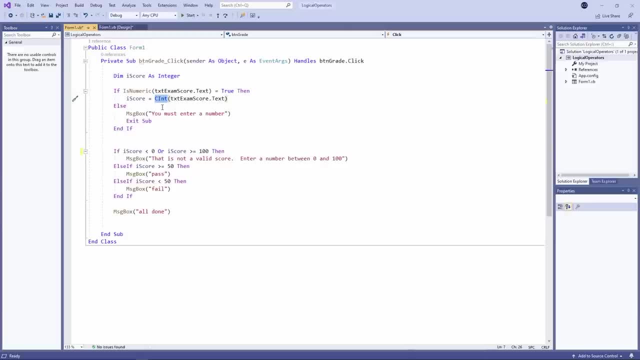 could. if VB does it, it's known as could. if VB does it, it's known as implicit type conversion. explicit type, implicit type conversion. explicit type, implicit type conversion. explicit type conversion is more efficient before we conversion is more efficient before we conversion is more efficient. before we add some more logic to this program, I 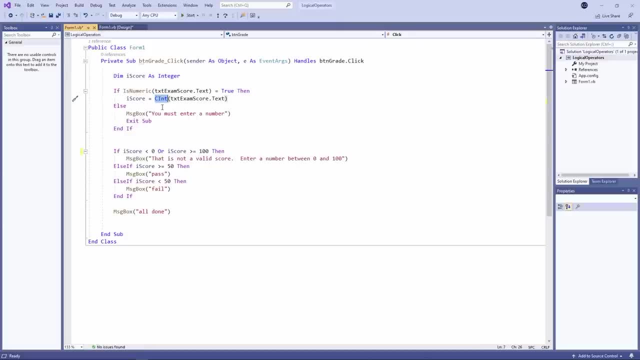 add some more logic to this program. I add some more logic to this program. I just want to point out that it's not just want to point out that it's not just want to point out that it's not perfectly robust, yet I can still crash. perfectly robust, yet I can still crash. 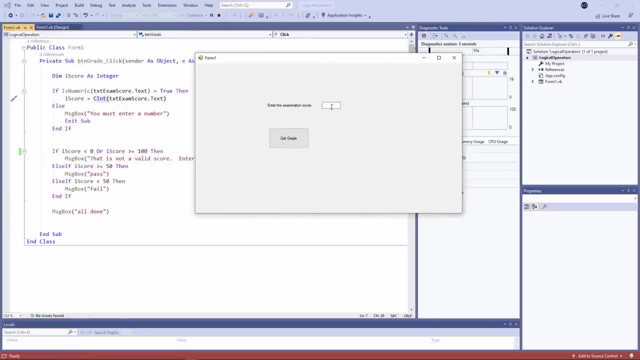 perfectly robust, yet I can still crash this. let me show you how this. let me show you how this. let me show you how. you've seen that, if I type text, I've. you've seen that, if I type text, I've. you've seen that, if I type text, I've essentially trapped the error. but what? 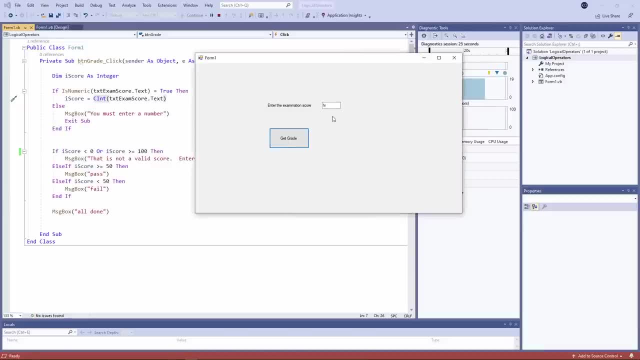 essentially trapped the error. but what essentially trapped the error? but what if I put in a number which is too big? if I put in a number which is too big? if I put in a number which is too big, that is an extremely large number and that is an extremely large number. and 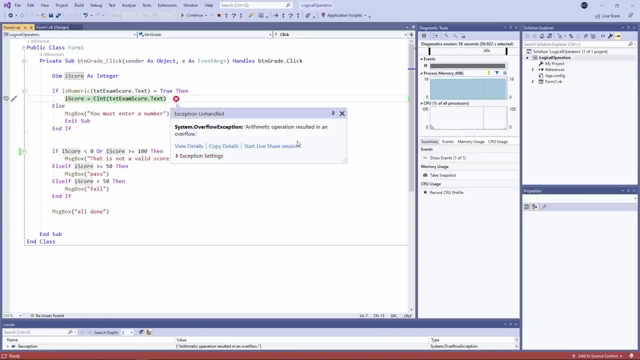 that is an extremely large number and it's crashed my program, an integer. it's crashed my program, an integer. it's crashed my program. an integer variable occupies four bytes of memory variable occupies four bytes of memory variable occupies four bytes of memory. that is, 32 bits. so the maximum number of 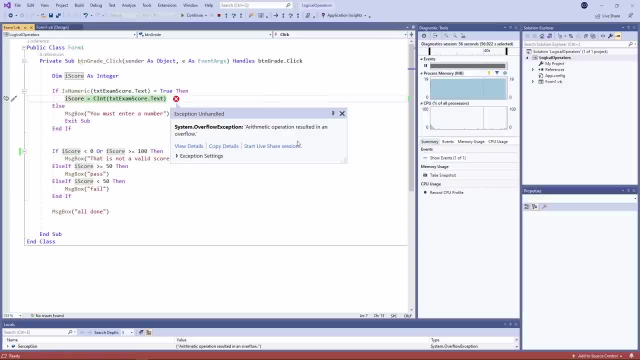 that is 32 bits. so the maximum number of that is 32 bits. so the maximum number of values that you can store in an integer values that you can store in an integer values that you can store in an integer variable is 2 to the power 32. 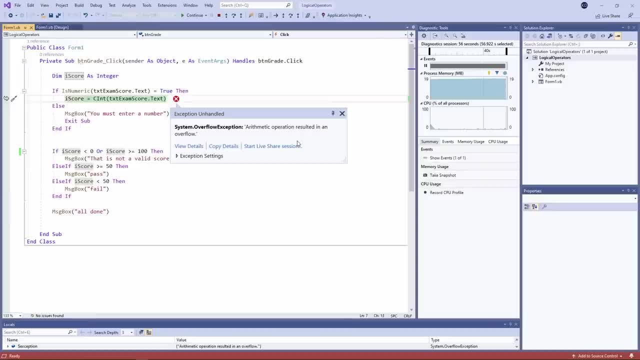 variable is 2 to the power 32. variable is 2 to the power 32, it works out to about 4 billion now. since it works out to about 4 billion now, since it works out to about 4 billion now, since we also need to store negative integers. 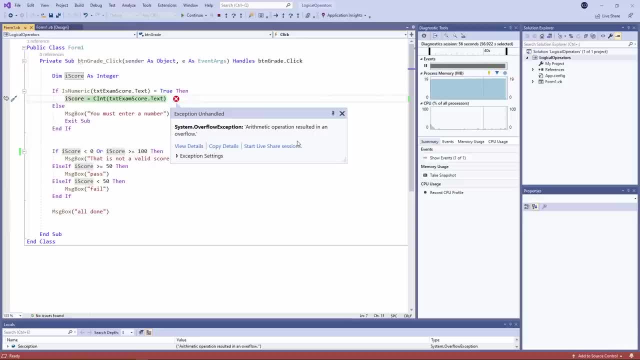 we also need to store negative integers. we also need to store negative integers. that means we can go from about minus 2. that means we can go from about minus 2. that means we can go from about minus 2 billion to positive 2 billion. the number: 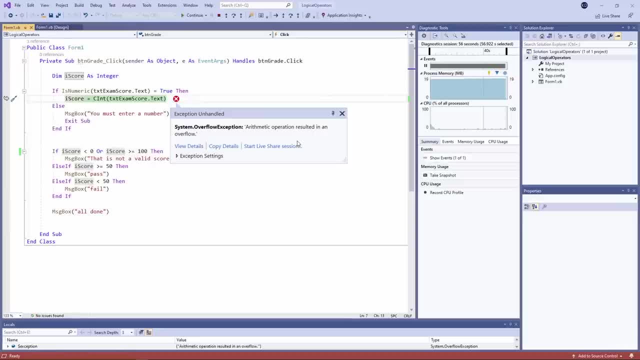 billion to positive 2 billion. the number billion to positive 2 billion. the number I entered was bigger than 2 billion and I entered was bigger than 2 billion and I entered was bigger than 2 billion and I've got what's known as an overflow. 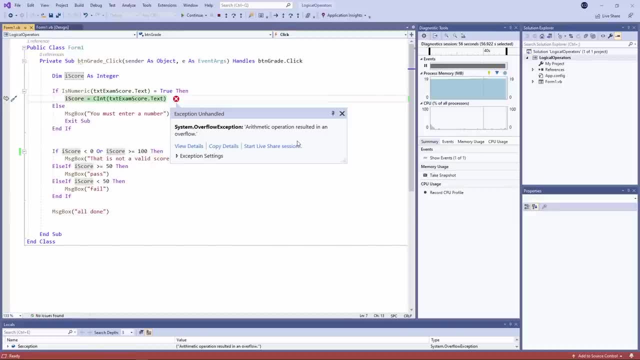 I've got what's known as an overflow. I've got what's known as an overflow exception. there's a possibility that the exception. there's a possibility that the exception. there's a possibility that the person who's using my program might type. person who's using my program might type. 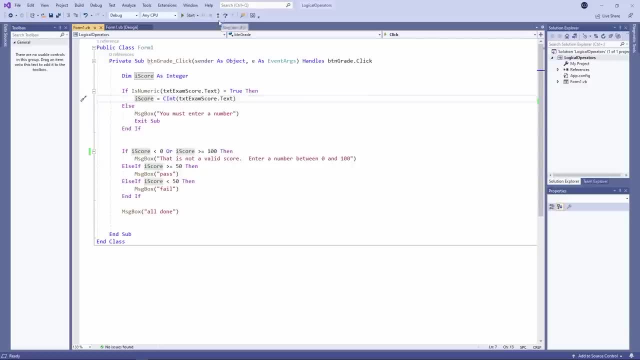 person who's using my program might type: I'm just going to change the user. I'm just going to change the user. I'm just going to change the user interface. notice that my text box has a max length. notice that my text box has a max length. 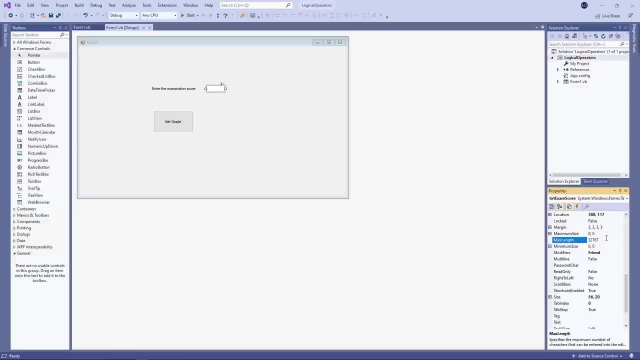 notice that my text box has a max length property. that's the maximum number of property. that's the maximum number of property. that's the maximum number of characters I can type into the text box characters. I can type into the text box characters I can type into the text box. you can see it's over 32,000. I can type: 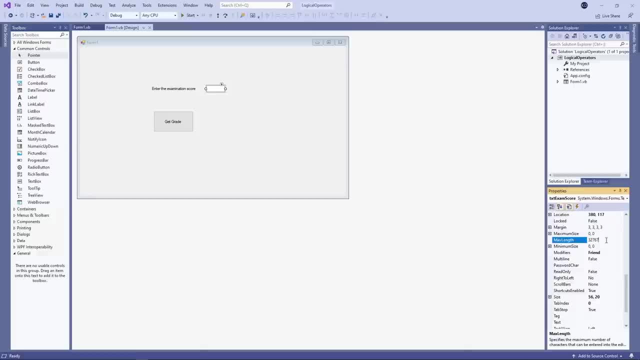 you can see, it's over 32,000. I can type: you can see, it's over 32,000. I can type 32,000 767 characters into this text box. 32,000 767 characters into this text box. 32,000 767 characters into this text box. well, my exam score is never going to be. 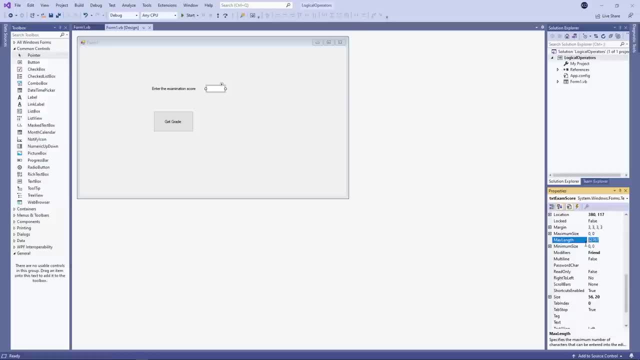 well, my exam score is never going to be well. my exam score is never going to be bigger than, let's say, a hundred. so if I bigger than let's say a hundred, so if I bigger than, let's say a hundred, so if I limit the number of characters that you 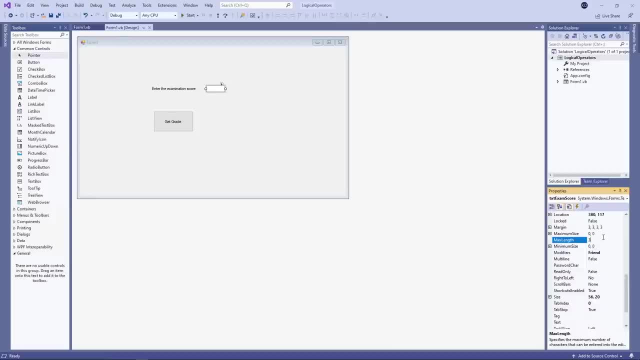 limit the number of characters, that you limit the number of characters that you can type into the text box to, let's say, can type into the text box to, let's say, can type into the text box to, let's say, three, then the maximum value you can put. 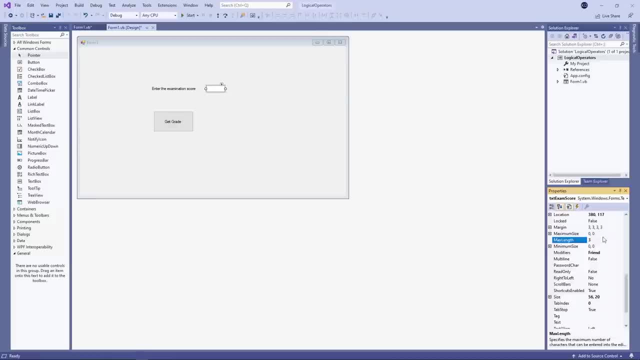 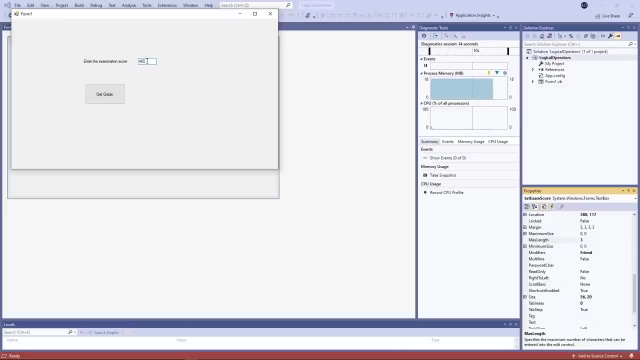 three, then the maximum value you can put. three, then the maximum value you can put in there is 999, a simple fix. I can't enter a number bigger than three. I can't enter a number bigger than three. I can't enter a number bigger than three characters long. 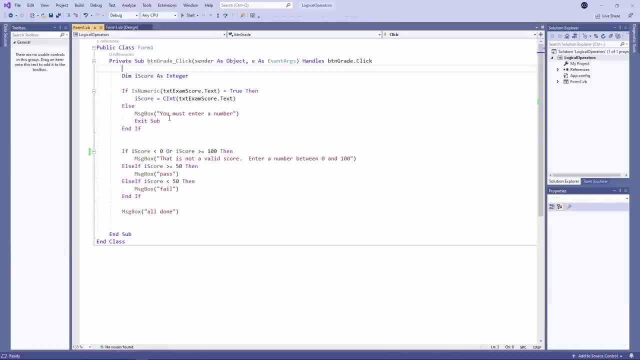 now, let's add some more logic to the if. now, let's add some more logic to the if. now, let's add some more logic to the if block, depending on the score. I want to block, depending on the score. I want to block. depending on the score, I want to award a grade which is either a, B, C, D, E. 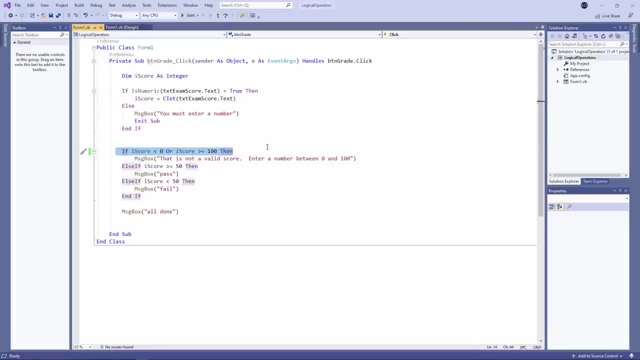 award a grade which is either a, B, C, D, E. award a grade which is either a, B, C, D, E or F. I'm going to keep the test which or F. I'm going to keep the test which or F. I'm going to keep the test which checks to see if the data is within. 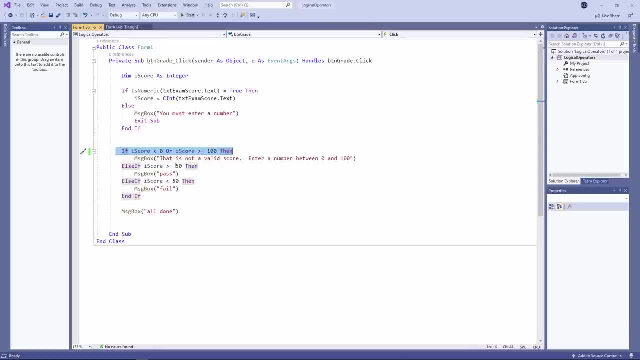 checks to see if the data is within. checks to see if the data is within range. but I'll add some more else if range. but I'll add some more else if range. but I'll add some more else if clauses, if you score less than or equal. 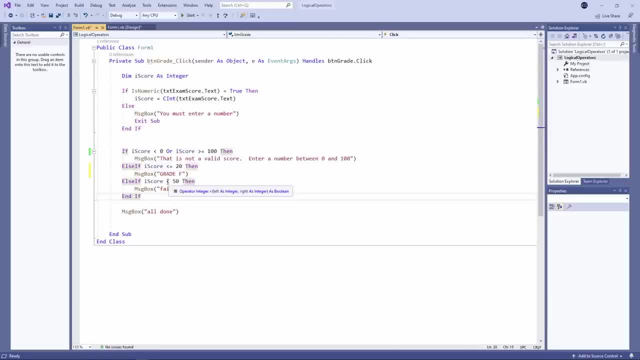 clauses if you score less than or equal clauses if you score less than or equal to 20. that is a grade F to 20. that is a grade F to 20. that is a grade F if you score more than 20 and less than. if you score more than 20 and less than. 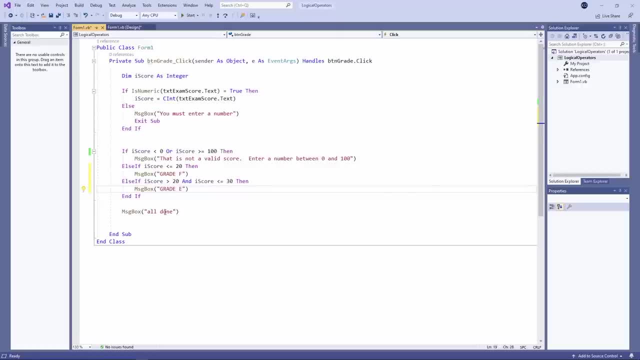 if you score more than 20 and less than or equal to 30, that is a grade E notice. or equal to 30, that is a grade E notice. or equal to 30, that is a grade E notice. the use of the logical operator and what. 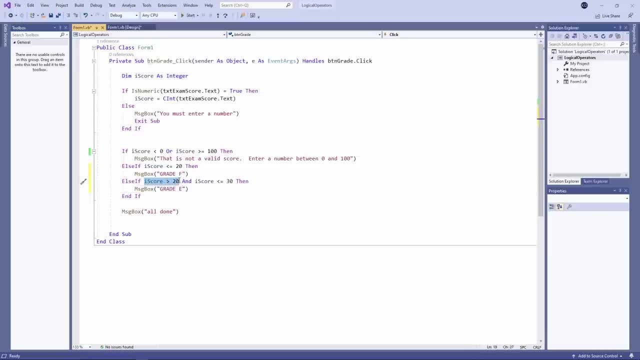 the use of the logical operator and what the use of the logical operator and what I'm saying is the score must be bigger. I'm saying is the score must be bigger. I'm saying is the score must be bigger than 20 and it must also be less than. 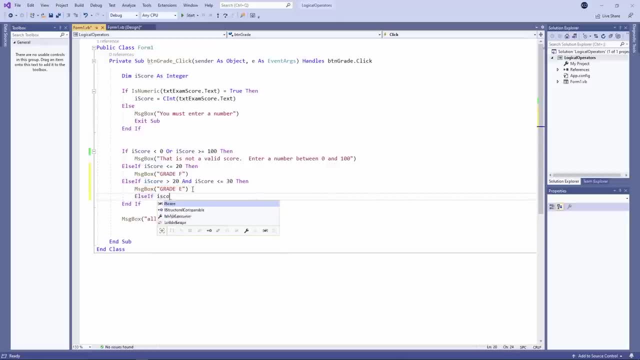 than 20, and it must also be less than than 20, and it must also be less than or equal to 30, or equal to 30 or equal to 30. a score between 31 and 40 will get you a. a score between 31 and 40 will get you a. 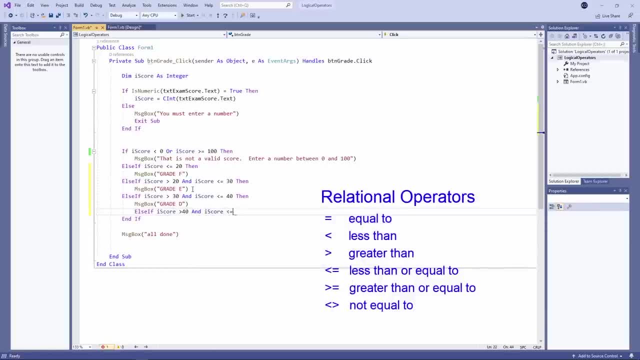 a score between 31 and 40 will get you a D, and anything between 41 and 50 will D, and anything between 41 and 50 will D, and anything between 41 and 50 will call that a C in this particular. call that a C in this particular. 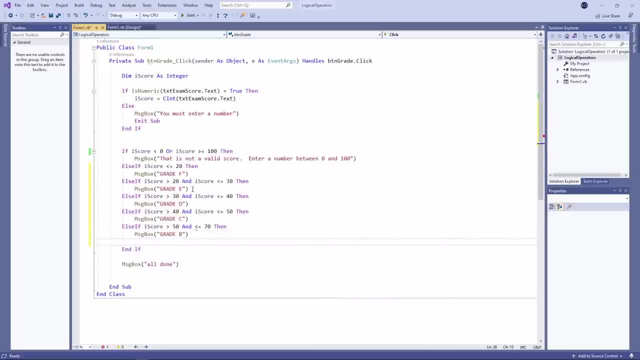 call that a C in this particular examination. anything between 51 and 70 examination, anything between 51 and 70 examination, anything between 51 and 70 will get you a B notice. I've got a. will get you a B notice. I've got a. 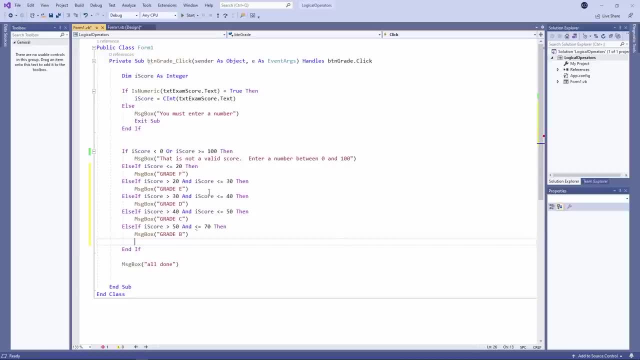 will get you a B notice. I've got a syntax error. there's a red wavy line- syntax error. there's a red wavy line- syntax error. there's a red wavy line. what's it telling me expression expected. what's it telling me expression expected? 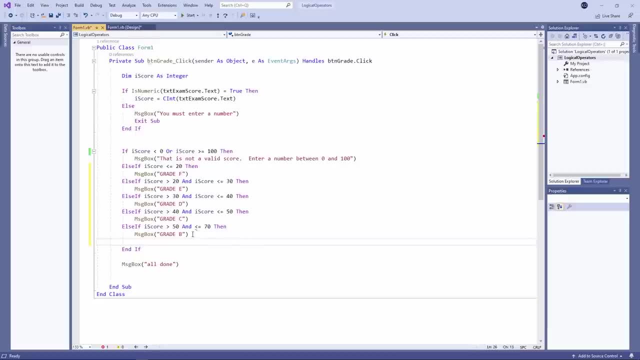 what's it telling me? expression expected, not particularly helpful, but this is not particularly helpful. but this is not particularly helpful, but this is actually quite a common mistake, when actually quite a common mistake, when actually quite a common mistake, when you're writing complex expressions which you're writing, complex expressions which 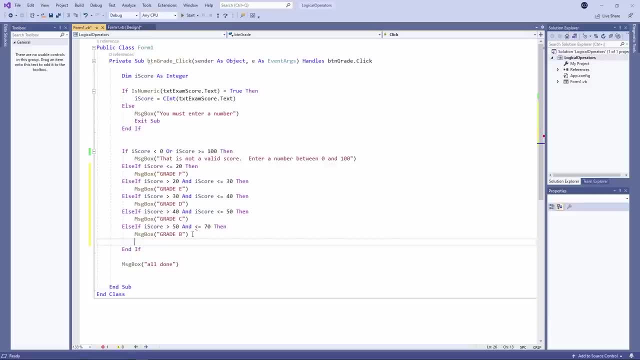 you're writing complex expressions which include logical and relational, include logical and relational. include logical and relational operators. I need to include I score operators. I need to include I score operators. I need to include I score again right here if I'm using a. again right here if I'm using a. 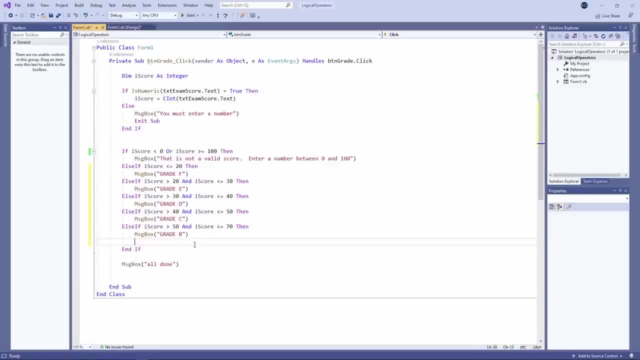 again right here. if I'm using a relational operator to compare two relational operator to compare two relational operator to compare two things such as a variable and a number, things such as a variable and a number, things such as a variable and a number, then I have to say what two things I am. 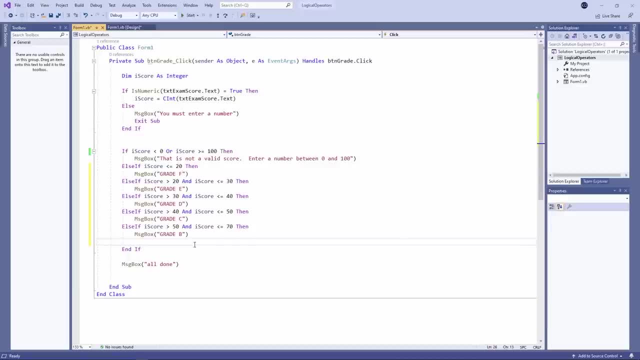 then I have to say what two things I am. then I have to say what two things I am comparing- I have to be explicit. okay. so comparing, I have to be explicit. okay. so comparing, I have to be explicit. okay, so every other score is going to get you a. 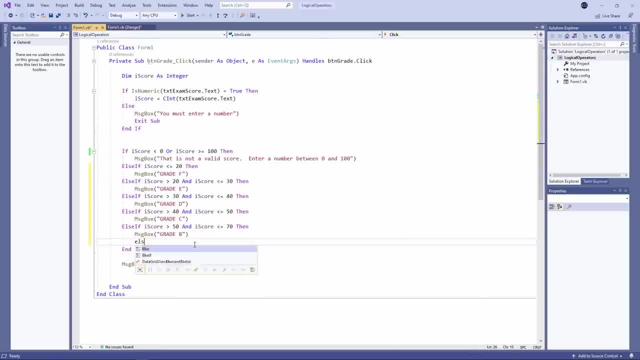 every other score is going to get you a. every other score is going to get you a grade a, so I can just use an else clause- grade a. so I can just use an else clause- grade a. so I can just use an else clause now, and that is all of the possibilities. 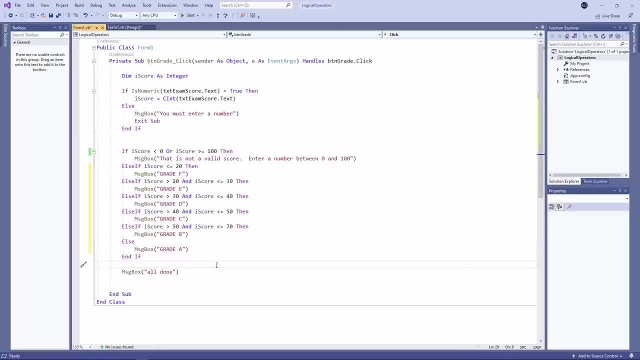 now and that is all of the possibilities now and that is all of the possibilities taken care of now. notice: I've been very taken care of now. notice I've been very taken care of now. notice I've been very, very careful not to overlap the ranges, very careful not to overlap the ranges. 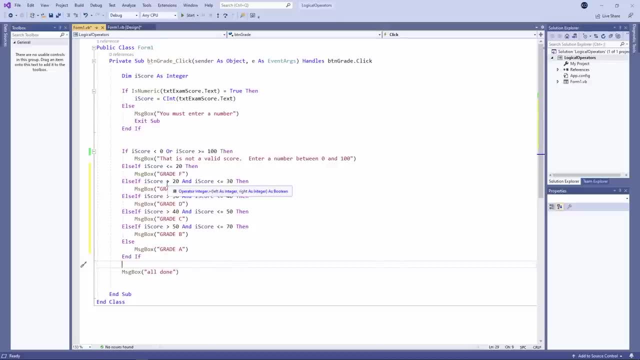 very careful not to overlap the ranges of scores. this range is between 21 and 30 of scores. this range is between 21 and 30 of scores. this range is between 21 and 30 inclusive. this range is between 31 and inclusive. this range is between 31 and. 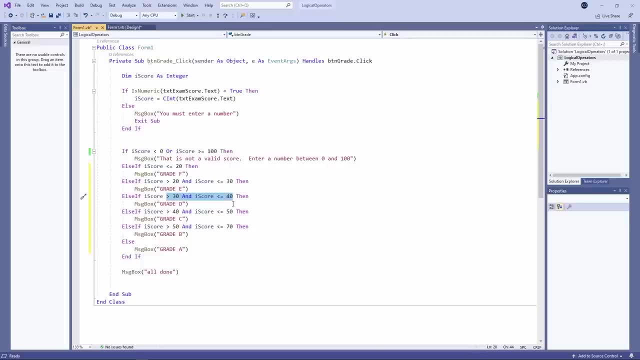 inclusive. this range is between 31 and 40 inclusive, there's no overlap. if for 40 inclusive, there's no overlap. if for 40 inclusive, there's no overlap. if, for example, I made this mistake and I said example, I made this mistake and I said: 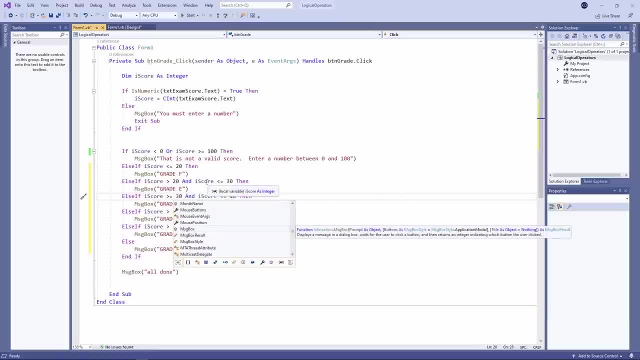 example, I made this mistake and I said greater than or equal to 30, then a score greater than or equal to 30, then a score greater than or equal to 30, then a score of 30 falls into this range and it falls of 30 falls into this range and it falls. 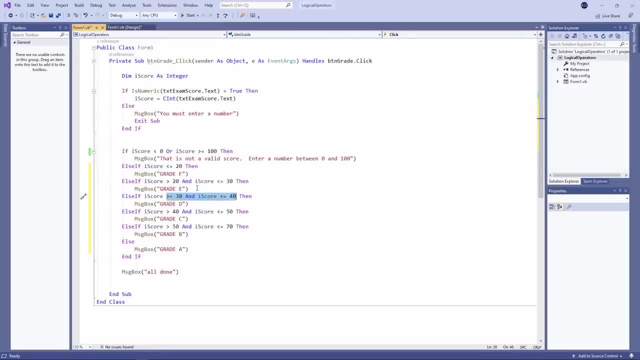 of 30 falls into this range, and it falls into this range, into this range, into this range, then my program might not work. I might, then my program might not work. I might, then my program might not work. I might get some peculiar results, so just be. get some peculiar results, so just be. 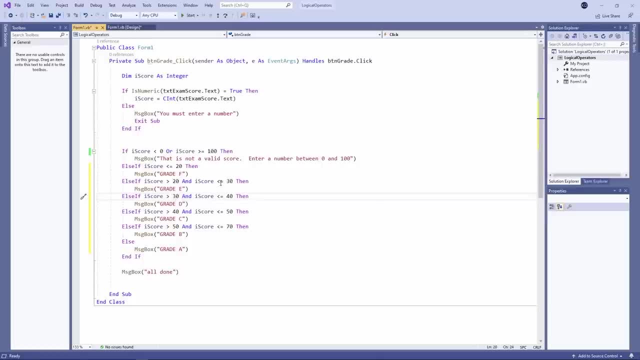 get some peculiar results. so just be very careful about that. if you think very careful about that, if you think very careful about that, if you think about what's going on here, a score of about what's going on here, a score of about what's going on here, a score of 30, is not covered either by this test or 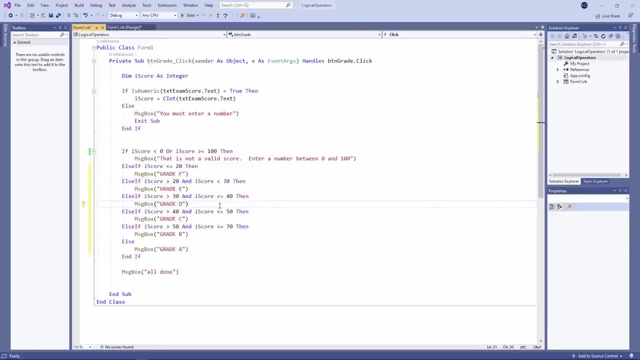 30 is not covered either by this test, or 30 is not covered either by this test or by this test. think it through and you'll by this test, think it through and you'll by this test, think it through and you'll see that a score of 30 will actually get. 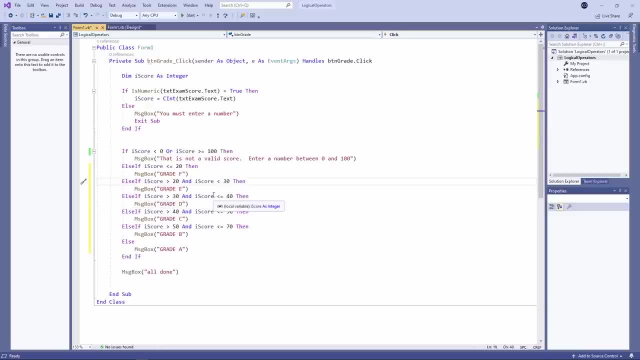 see that a score of 30 will actually get. see that a score of 30 will actually get you a grade a, but that should be fine. you a grade a, but that should be fine. you a grade a, but that should be fine. there's one more logical operator, which. 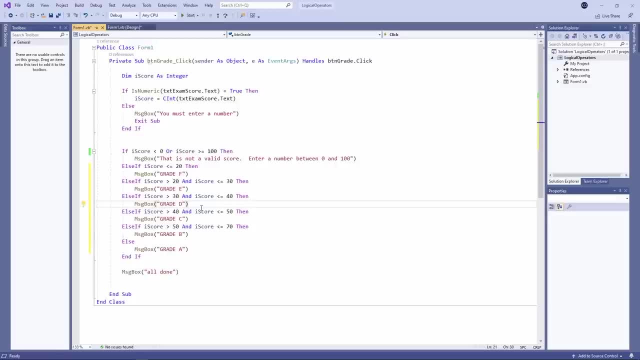 there's one more logical operator which. there's one more logical operator which I haven't mentioned and, to be honest, I I haven't mentioned and, to be honest, I I haven't mentioned and, to be honest, I don't really need it in this scenario, don't really need it in this scenario. 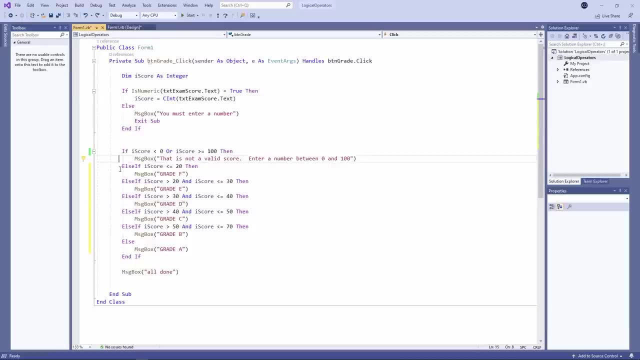 don't really need it in this scenario, but I can make use of it just to. but I can make use of it just to. but I can make use of it just to illustrate how it works. instead of illustrate how it works, instead of illustrate how it works, instead of asking if the score is out of range, I'm 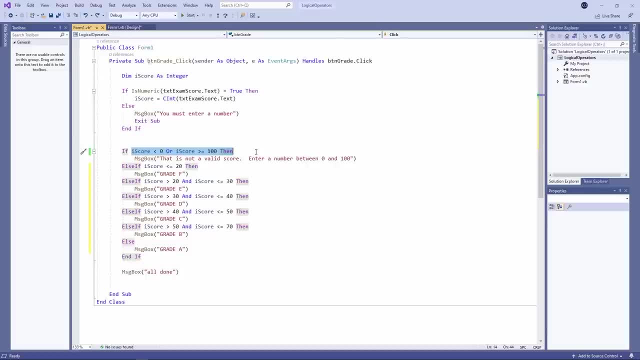 asking if the score is out of range. I'm asking if the score is out of range. I'm going to just turn the logic of that, going to just turn the logic of that, going to just turn the logic of that question around and ask if the score is. 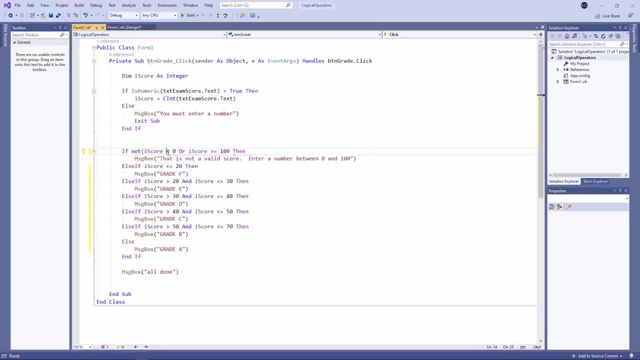 question around and ask if the score is. question around and ask if the score is not in range. in a sense it's the same question if the. in a sense it's the same question if the. in a sense it's the same question if the score is not in between one and a. 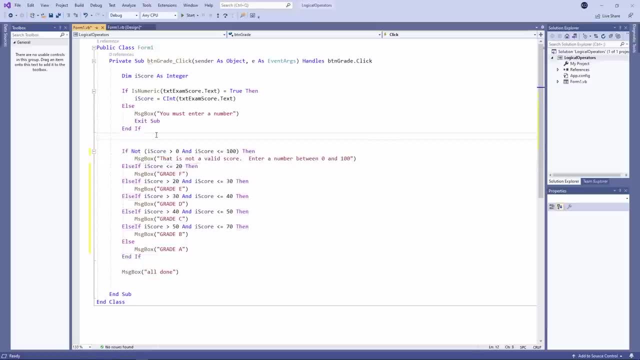 score is not in between one and a score is not in between one and a hundred, then it must be out of range now. hundred, then it must be out of range now. hundred, then it must be out of range now. all that remains is to test the program. 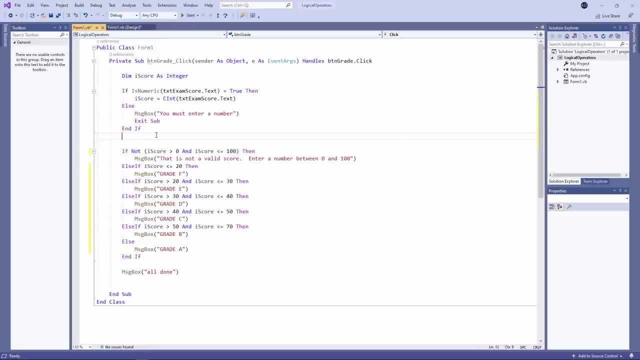 all that remains is to test the program. all that remains is to test the program thoroughly. there are several possible thoroughly. there are several possible thoroughly. there are several possible execution paths, and I should execution paths and I should execution paths and I should really test them all. I should also make a 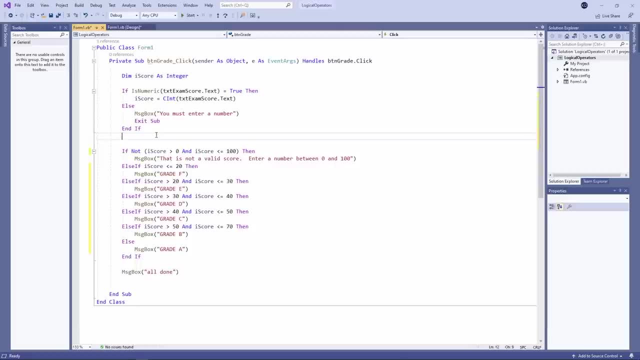 really test them all. I should also make a really test them all. I should also make a point of testing things which I've point of testing things which I've point of testing things which I've tested before, for example, my validation, tested before, for example, my validation. 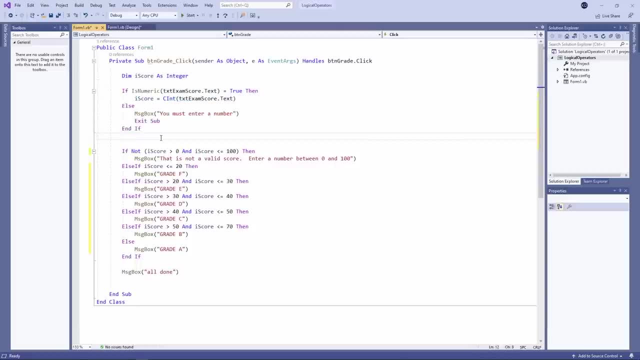 tested before, for example, my validation routine. here I need to make sure that I routine here. I need to make sure that I routine here I need to make sure that I haven't introduced any bugs when I added: haven't introduced any bugs when I added: haven't introduced any bugs when I added new functionality. this is called. 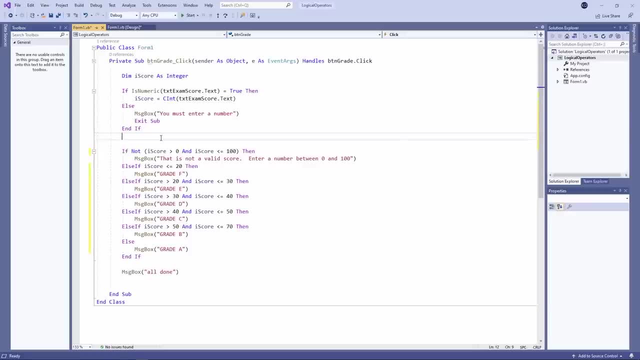 new functionality. this is called new functionality. this is called regression testing. I should also check regression testing. I should also check regression testing. I should also check all of the boundary values. I should try all of the boundary values. I should try all of the boundary values. I should try a value of 0, a value of 100, a value of 20. 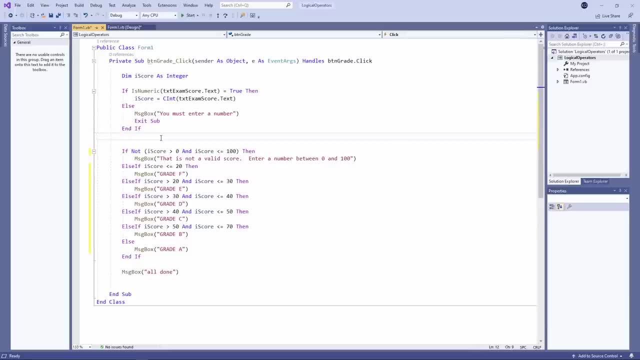 a value of 0, a value of 100, a value of 20, a value of 0, a value of 100, a value of 20, 30, 40, 70 and I should also try valid- 30, 40, 70 and I should also try valid. 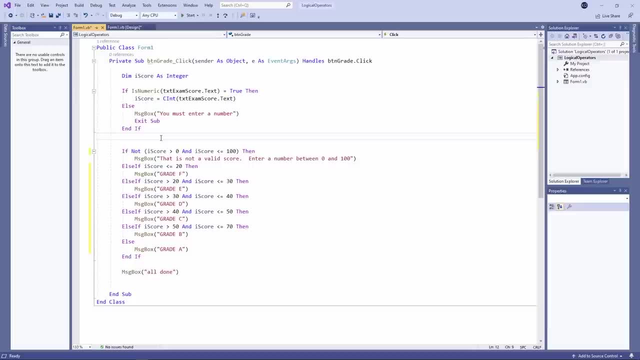 30, 40, 70 and I should also try valid values within the ranges which I've values within the ranges which I've values within the ranges which I've specified in my if statement, namely 25 specified in my if statement, namely 25 specified in my if statement, namely 25, 35, 45, 60, 75, if you don't test thoroughly. 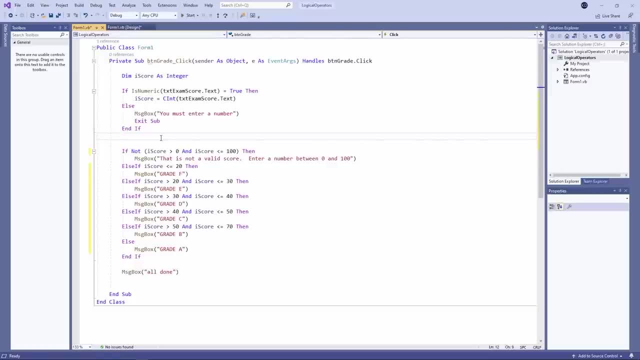 35, 45, 60, 75 if you don't test thoroughly, 35, 45, 60, 75, if you don't test thoroughly, and then you start adding more code to, and then you start adding more code to, and then you start adding more code to this, then you're building on shifting. 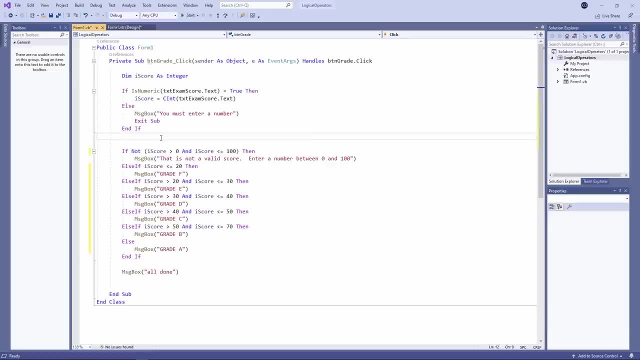 this, then you're building on shifting this, then you're building on shifting sand. do it carefully now and you'll save sand. do it carefully now and you'll save sand. do it carefully now and you'll save yourself a lot more work later on. yourself a lot more work later on. 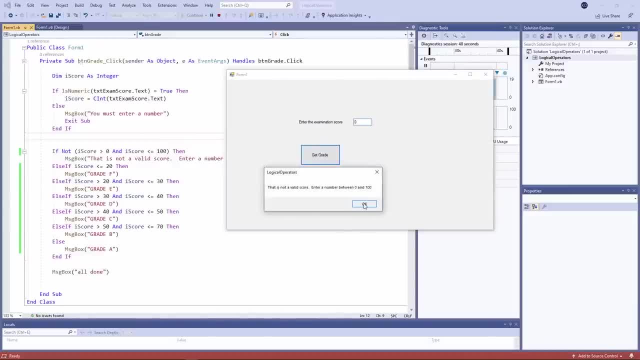 yourself a lot more work later on. and straight away I found a problem. it and straight away I found a problem. it and straight away I found a problem. it is possible to score 0 on an exam. that is possible to score 0 on an exam that. 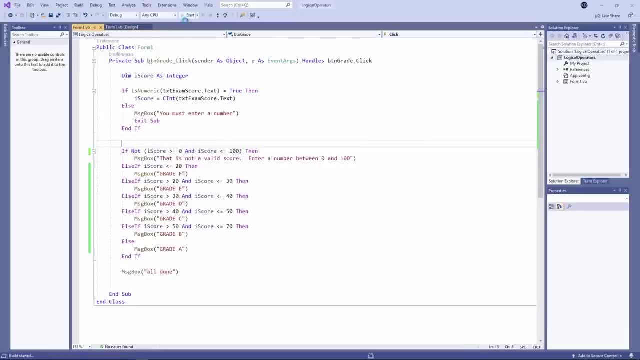 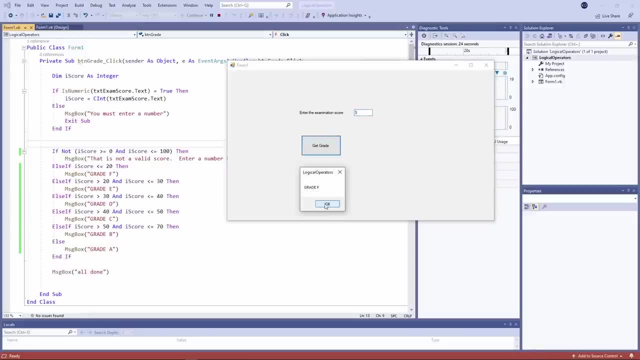 is possible to score 0 on an exam that should have been greater than or equal. should have been greater than or equal. should have been greater than or equal to zero. that's better to zero. that's better to zero. that's better. as I said, make sure that you test every. 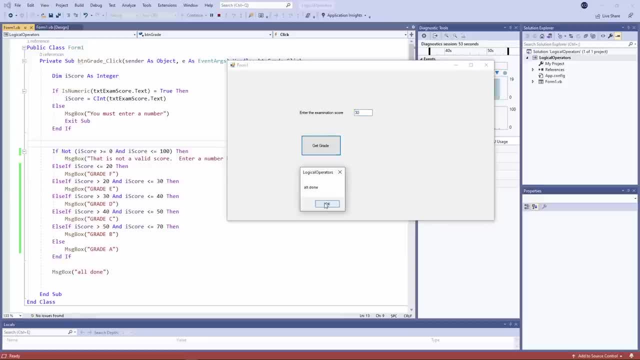 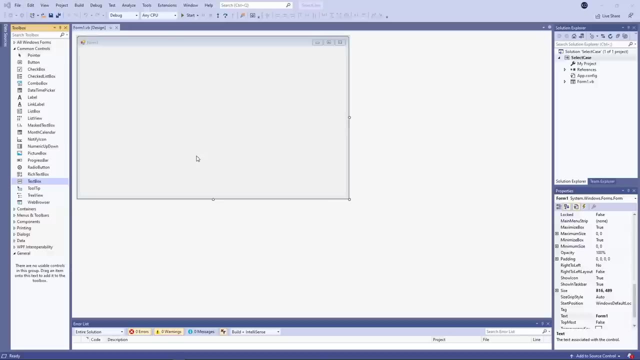 as I said, make sure that you test every. as I said, make sure that you test every possible pathway through the program. I'm going to show you an alternative to. I'm going to show you an alternative to. I'm going to show you an alternative to the if block: another way to perform. 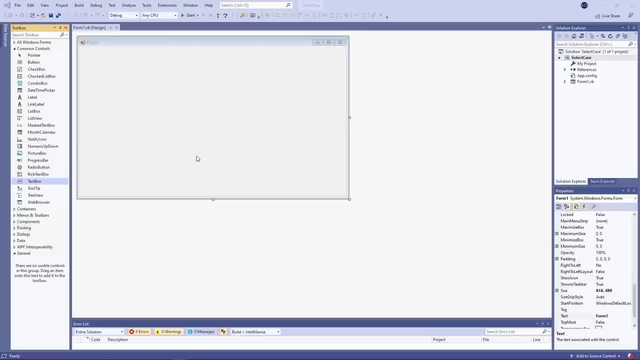 the if block. another way to perform the if block. another way to perform selection in your selection, in your selection, in your code. I've created a new project. let's pop code. I've created a new project. let's pop code. I've created a new project. let's pop a text box on there to capture some. 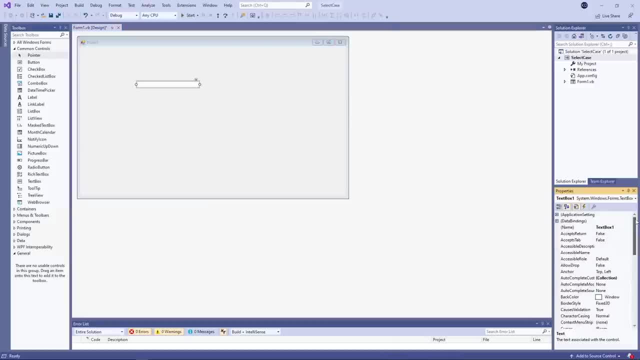 a text box on there to capture some, a text box on there to capture some input and a button to run my program. the idea is that the user types in a. the idea is that the user types in a. the idea is that the user types in a temperature, maybe 15 degrees and then. 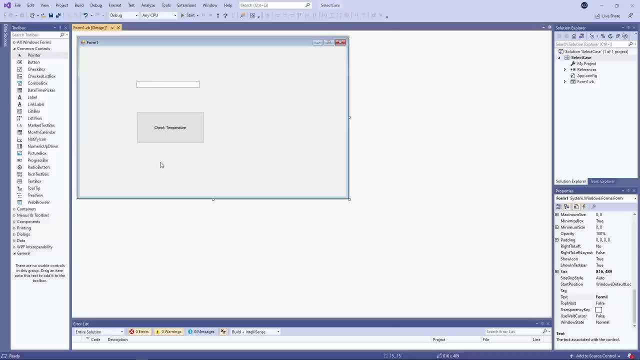 temperature maybe 15 degrees and then temperature maybe 15 degrees and then the check temperature button will tell the check temperature button will tell. the check temperature button will tell the user whether it's cold, freezing, warm the user whether it's cold, freezing, warm the user whether it's cold, freezing, warm, hot, that kind of thing. 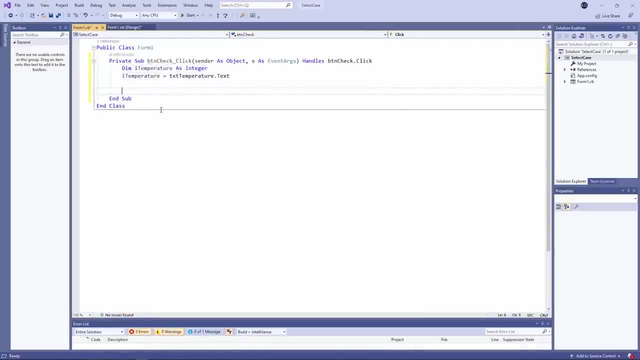 hot that kind of thing. hot that kind of thing. and although I could allow VB to do the and although I could allow VB to do the and although I could allow VB to do the implicit type conversion for me, I'm going. implicit type conversion for me, I'm going. 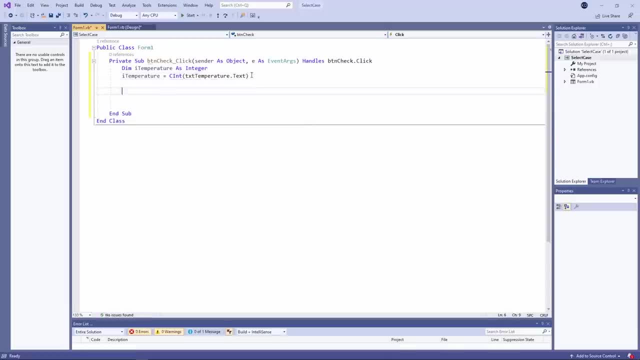 implicit type conversion for me. I'm going to do it explicitly. remember a text box. to do it explicitly. remember a text box. to do it explicitly. remember a text box captures text input. I'm converting it. captures text input. I'm converting it. captures text input. I'm converting it into an integer. I'm not going to worry. 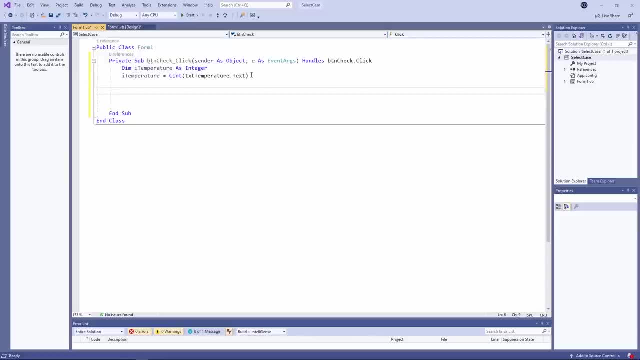 into an integer. I'm not going to worry into an integer. I'm not going to worry about my program crashing if the user about my program crashing, if the user about my program crashing, if the user doesn't behave themselves and type in a, doesn't behave themselves and type in a. 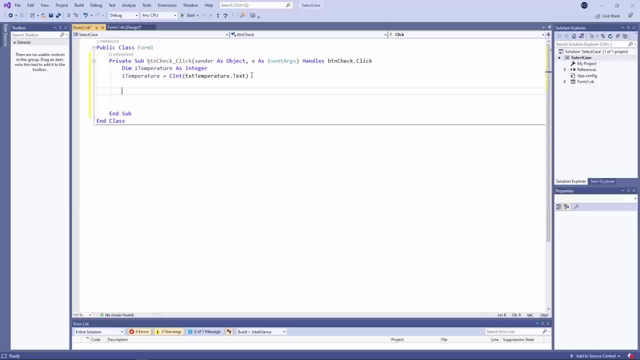 doesn't behave themselves and type in a number. now this is what the select case number. now. this is what the select case number. now this is what the select case construct looks like. it begins with the construct. looks like it begins with the construct. looks like it begins with the word select case and then the name of 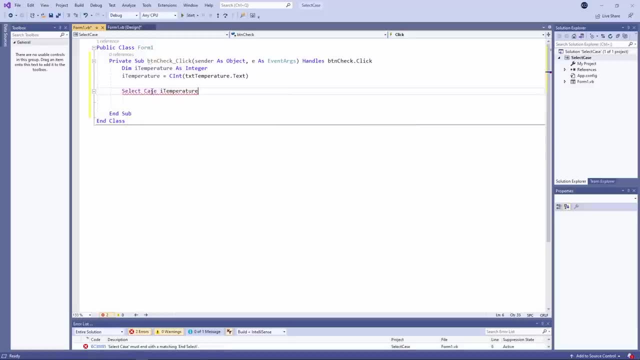 word select case and then the name of word select case and then the name of the variable which I want to test in the variable which I want to test, in the variable which I want to test in this case I temperature, and it finishes this case I temperature and it finishes. 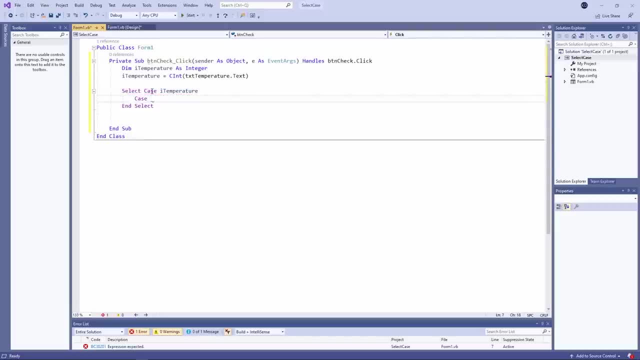 this case I temperature. and it finishes with end select. and now I'm going to say with end select, and now I'm going to say with end select, and now I'm going to say: in case I temperature is equal to zero, I, in case I temperature is equal to zero, I. 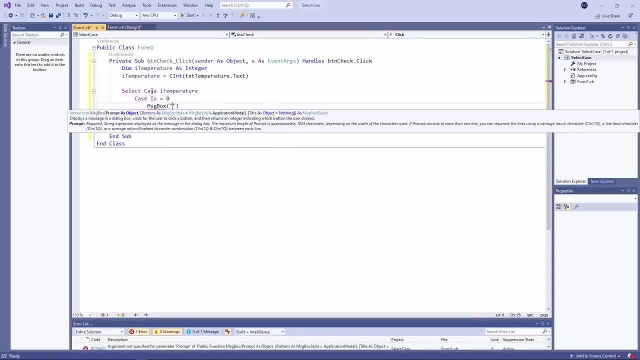 in case I temperature is equal to zero, I will output the message freezing. if the will output the message freezing. if the will output the message freezing. if the temperature is less than zero, I'm going. temperature is less than zero. I'm going. temperature is less than zero. I'm going to output an appropriate message for. 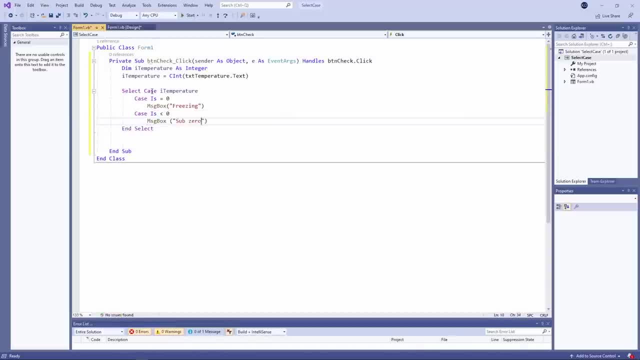 to output an appropriate message for. to output an appropriate message for that as well. if the temperature is that as well, if the temperature is that as well. if the temperature is between 1 and 10, that's cold notice. the between 1 and 10, that's cold notice. the. 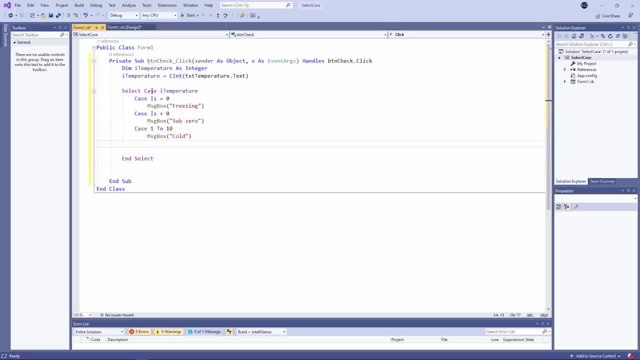 between 1 and 10. that's cold notice. the syntax case 1 to 10. that means syntax case 1 to 10. that means syntax case 1 to 10. that means everything between 1 and 10 inclusive. so everything between 1 and 10 inclusive. so 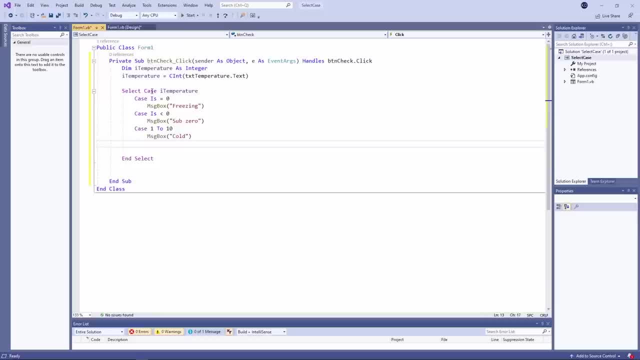 everything between 1 and 10 inclusive, so 1 and 10 are included as well. if it's 1 and 10 are included as well, if it's 1 and 10 are included as well, if it's between 11 and 20, it's warm. 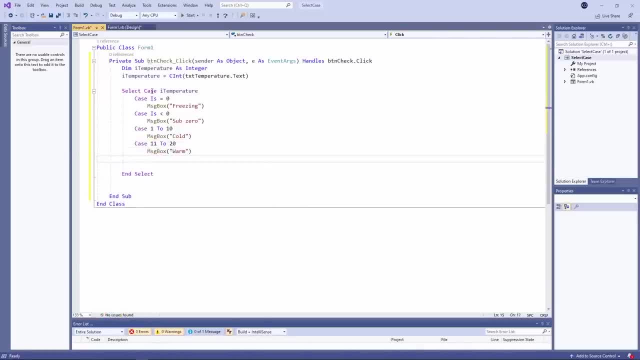 between 11 and 20 it's warm. between 11 and 20 it's warm. and let's say everything else is hot, and and let's say everything else is hot, and and let's say everything else is hot. and there it is, the select case construct. 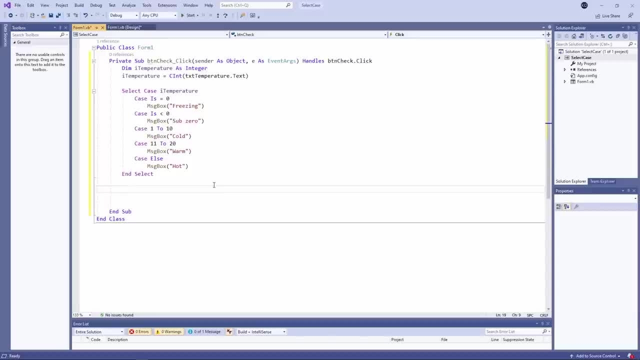 there it is the select case construct. there it is the select case construct. now I could have done exactly the same now. I could have done exactly the same now. I could have done exactly the same thing using an if block, but arguably. thing using an if block, but arguably. 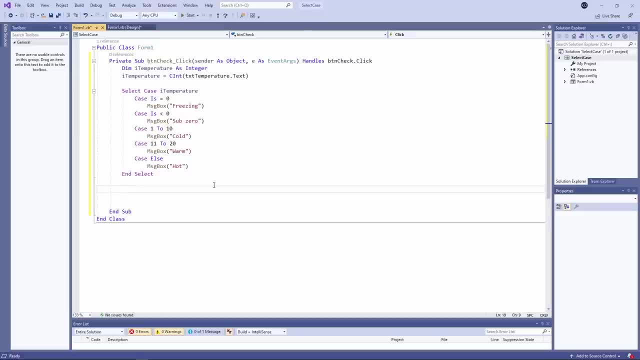 thing using an if block, but arguably, this is a little easier to read. it's this is a little easier to read. it's this is a little easier to read. it's somewhat easier to see what's going on. somewhat easier to see what's going on. somewhat easier to see what's going on. by the way, I could execute multiple. 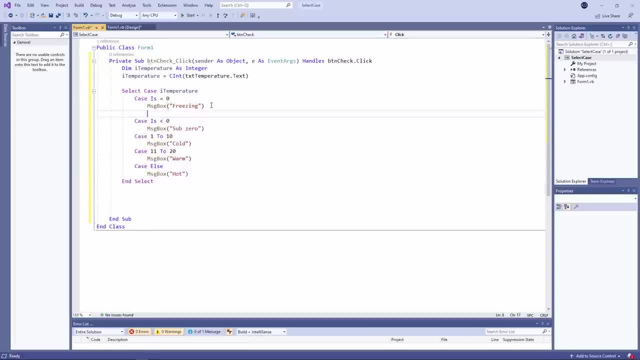 by the way I could execute multiple. by the way I could execute multiple lines of code as a result of each test. lines of code as a result of each test. lines of code as a result of each test. okay, it's a bit silly, but you get the. 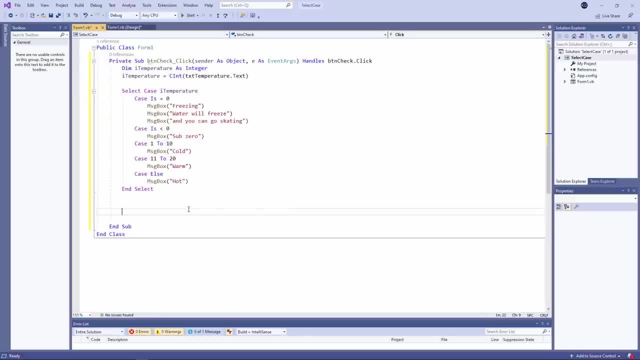 okay, it's a bit silly, but you get the. okay, it's a bit silly, but you get the point. I'm selecting one block of code or point. I'm selecting one block of code or point. I'm selecting one block of code or another, depending on the outcome of a 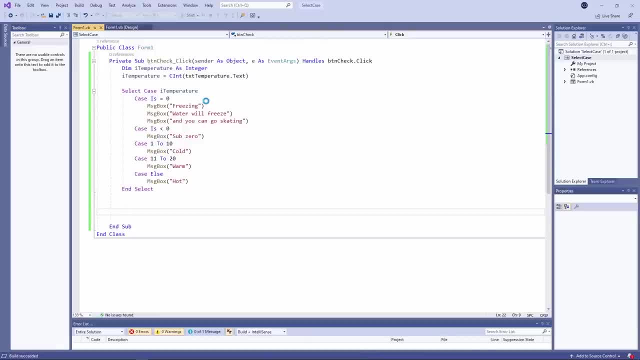 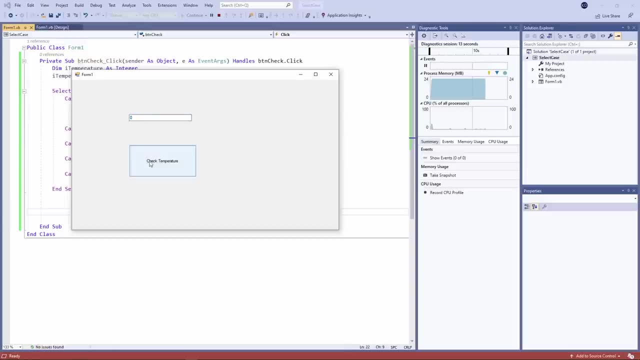 another depending on the outcome of a another. depending on the outcome of a test, let's give it a try test. let's give it a try test. let's give it a try. minus 5 is sub 0: 0 is freezing water will. minus 5 is sub 0: 0 is freezing water will. 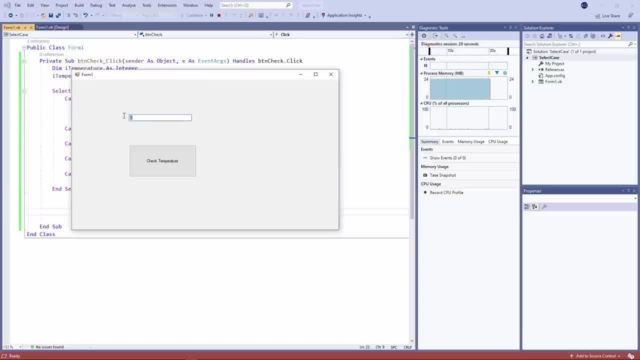 minus 5 is sub 0, 0 is freezing. water will freeze and you can go skating freeze and you can go skating freeze and you can go skating. hate is cold, 15 is warm and 200 is hot. hate is cold, 15 is warm and 200 is hot. 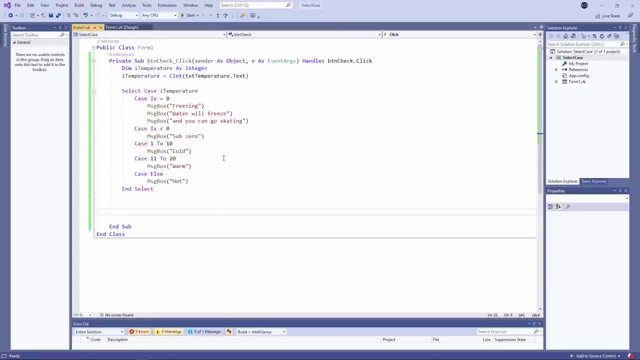 hate is cold, 15 is warm and 200 is hot. you should really test all of the. you should really test all of the. you should really test all of the boundaries as well. so you should see boundaries as well. so you should see boundaries as well. so you should see what happens if you enter a 1 or a 10 or 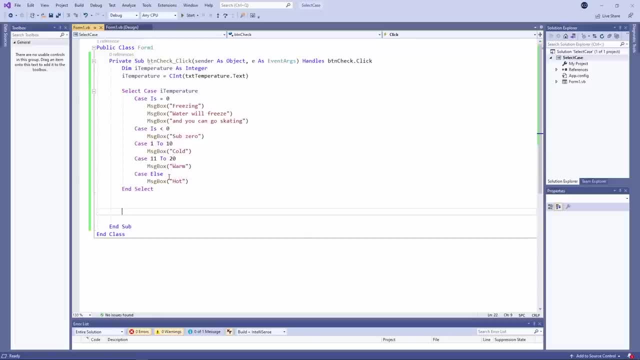 what happens if you enter a 1 or a 10? or what happens if you enter a 1 or a 10 or 11- 20, and then something incredibly big- 11- 20- and then something incredibly big- 11- 20- and then something incredibly big. this program can be crashed as well. 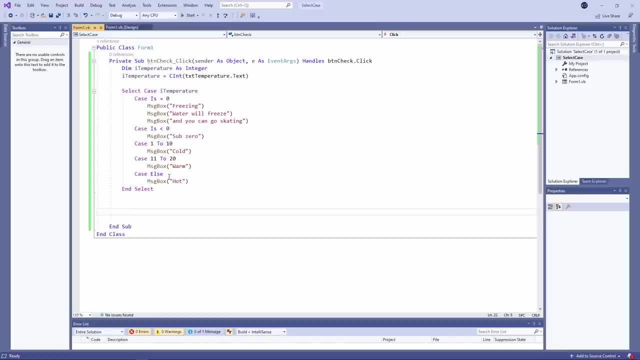 this program can be crashed as well. this program can be crashed as well, because we could type in some text, but because we could type in some text, but because we could type in some text, but of course we could add some additional. of course we could add some additional. 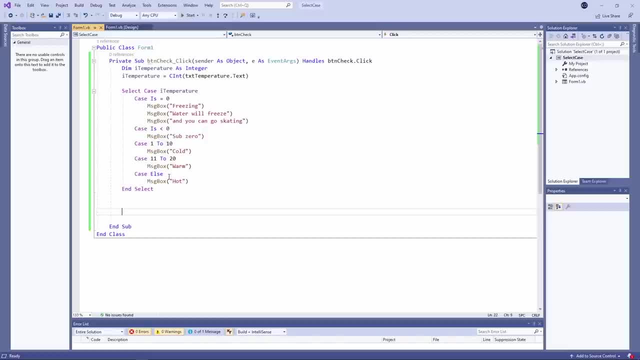 of course, we could add some additional logic to validate the data before the logic to validate the data before the logic to validate the data before the code gets into the select case, block by code gets into the select case, block by code gets into the select case block. by the way, there are some other things I 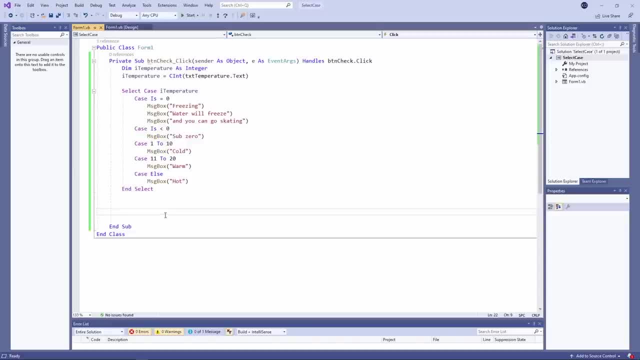 the way there are some other things I the way there are some other things I can use in a case statement, for example, can use in a case statement, for example, can use in a case statement. for example, I could say: case 1 comma, 2 comma, 3 comma. 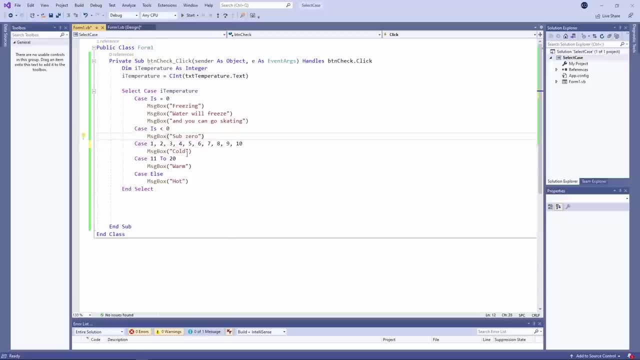 I could say case 1 comma, 2 comma, 3 comma. I could say case 1 comma, 2 comma, 3 comma, 4, 5, and that's an alternative to saying 4- 5, and that's an alternative to saying 4- 5 and that's an alternative to saying 1 to 10. so if it isn't a continuous range, 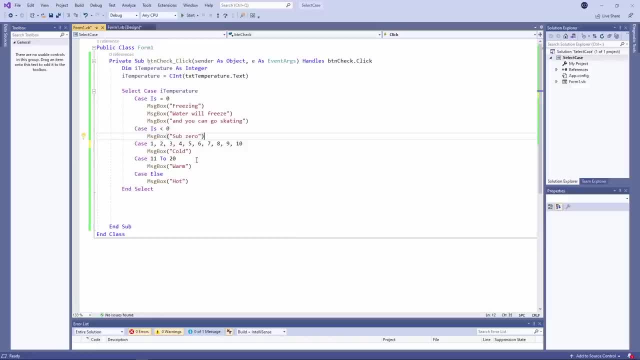 1 to 10. so if it isn't a continuous range- 1 to 10- so if it isn't a continuous range of values which I'm testing, that would be of values which I'm testing, that would be of values which I'm testing. that would be the way to go and I can use all of my 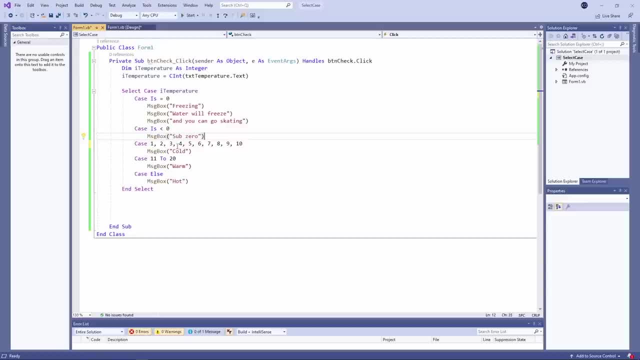 the way to go and I can use all of my the way to go and I can use all of my relational operators when I'm composing a relational operators, when I'm composing a relational operators when I'm composing a test as well. so, for example, here I've 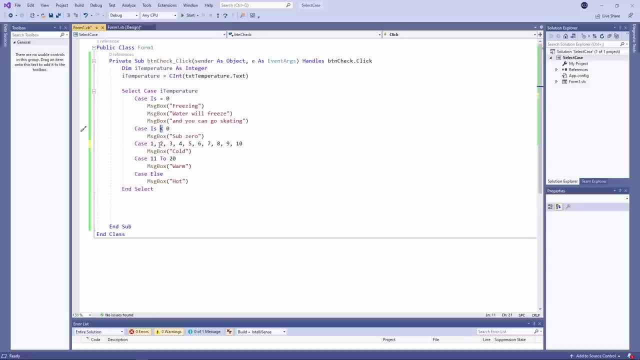 test as well. so, for example, here I've test as well. so, for example, here I've used a less than sign, but I could use used a less than sign, but I could use used a less than sign, but I could use greater than. I could use less than. or. 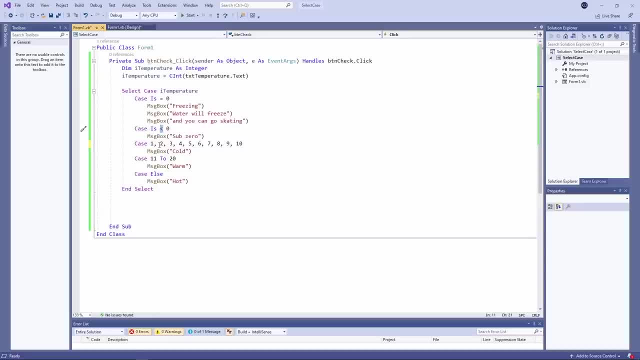 greater than I could use, less than, or greater than I could use, less than, or equal to greater than, or equal to not equal to greater than, or equal to not equal to greater than or equal to not equal to the same as if I was building a. equal to the same as if I was building a. 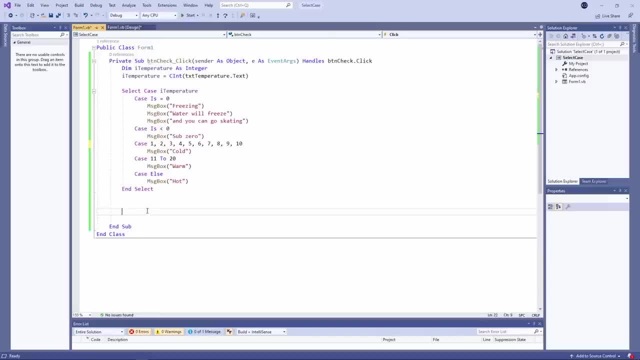 equal to the same as if I was building a test for an if block now. you might be test for an if block now. you might be test for an if block now. you might be wondering why bother with an if block at. wondering why bother with an if block at. 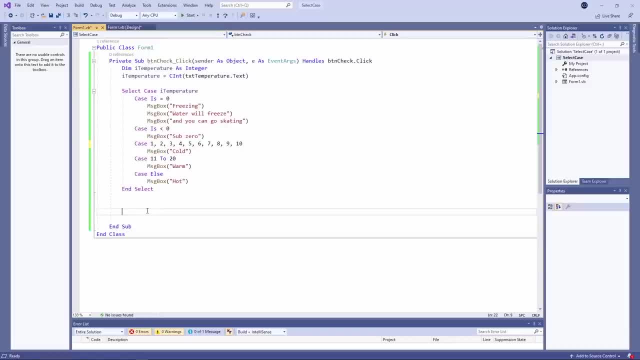 wondering: why bother with an if block at all? why not use select case every time all? why not use select case every time all? why not use select case every time? well, there is a particular limitation. well, there is a particular limitation. well, there is a particular limitation when it comes to select case. you can. 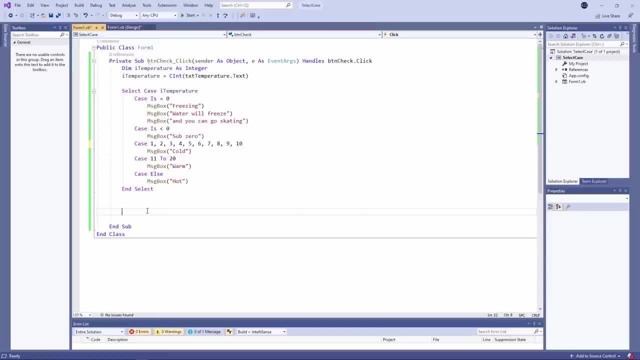 when it comes to select case, you can. when it comes to select case, you can only test one variable at a time. let's only test one variable at a time. let's only test one variable at a time. let's say, for example: we've also captured the. 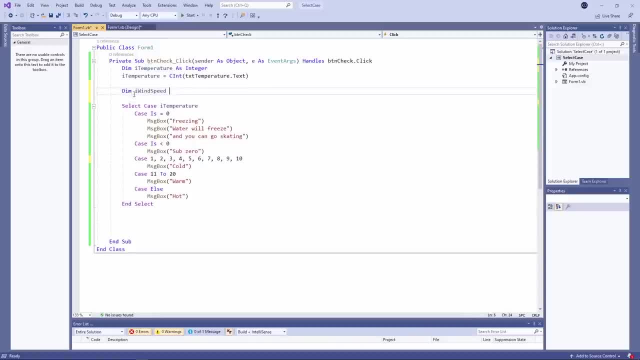 say, for example, we've also captured the say. for example, we've also captured the wind speed. I've just hard-coded a value- wind speed. I've just hard-coded a value- wind speed. I've just hard-coded a value for the purpose of demonstration. I can't. 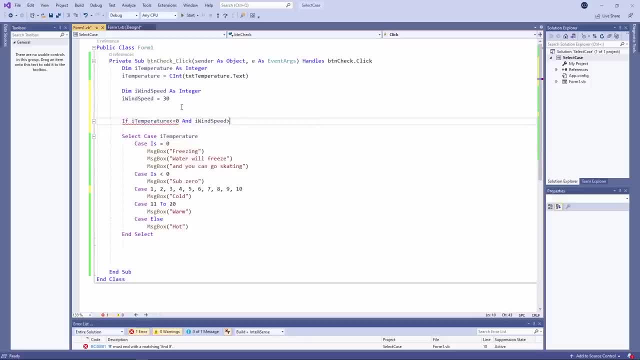 for the purpose of demonstration. I can't, for the purpose of demonstration. I can't do something like this with a select. do something like this with a select. do something like this with a select case construct. I'm testing the contents case construct. I'm testing the contents. 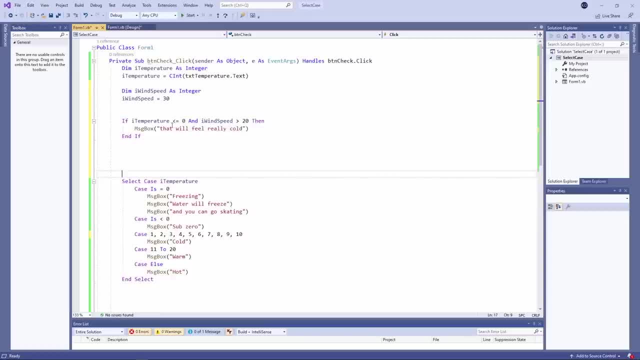 case construct. I'm testing the contents of two variables using a logical of two variables, using a logical of two variables, using a logical operator with a select case construct. I operator with a select case construct, I operator with a select case construct. I can only test, can only test. 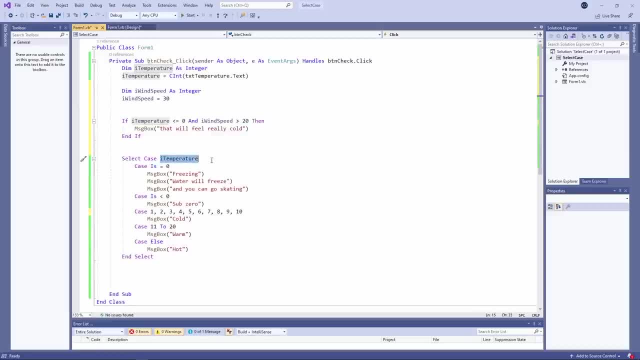 one variable at a time. I could, however, nest an if block inside the select case, construct something like this: so if the temperature is less than zero, will report that it is sub-zero, and then we'll check the wind speed, and if the wind speed is bigger than 20 will report. 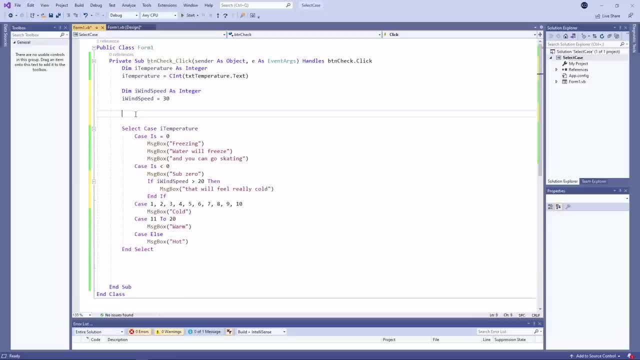 that it's going to feel really cold. perhaps you'd like to give it a try yourself. maybe rewrite the exam grading program to use a select case construct instead of an if block. by the way, different programming languages might well have their own equivalent to the select case construct. C sharp, for example, uses the switch construct, but it 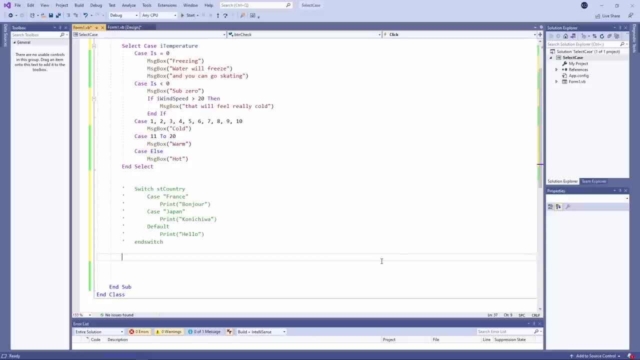 does pretty much the same thing. you might want to make sure that you have a. if you see pseudocode on an exam paper, it may well be written like this. I've commented it out because it won't work in Visual Basic, but you can see. the concept is pretty much the same. 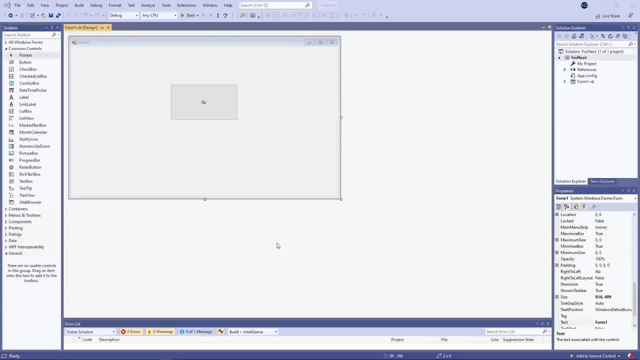 I'm going to show you the third of the three fundamental constructs of high level programming, namely iterations. Iteration means executing a block of code repeatedly. iteration is also known as looping, and there are two ways you can do this in VBnet. one of them is with a. 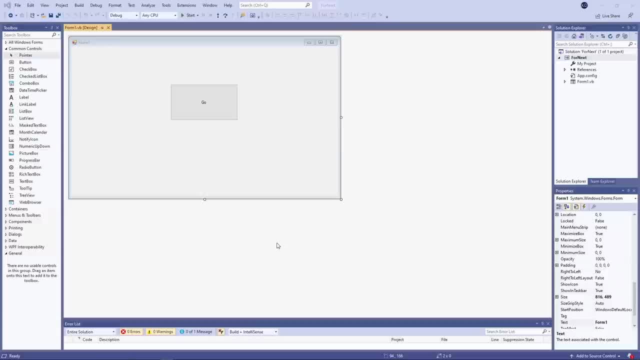 for loop and the other is with a do loop. in this video I'm going to focus on the for loop. I've already created a new Windows Forms application and I've placed a button on the form, so let's get right into the code to make something. 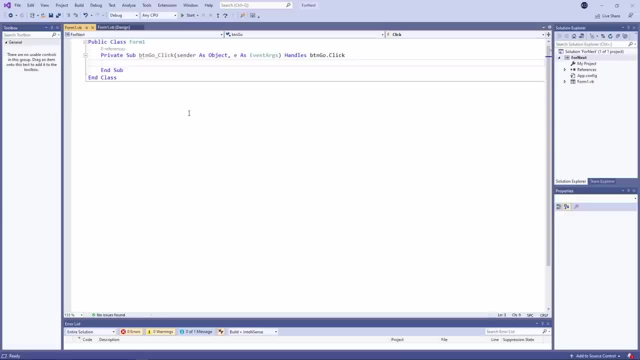 execute repeatedly. I need a way to count the number of repetitions. I need a way to count the number of iterations. so I'm going to declare a variable of type integer. it doesn't really matter what I call the variable. I've called it, I count because I'm going to counter my way through a loop. the for loop looks like: 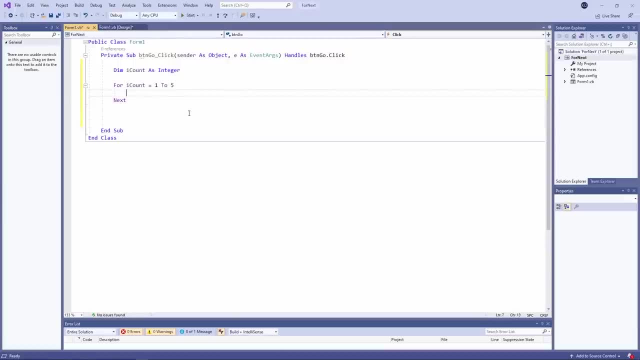 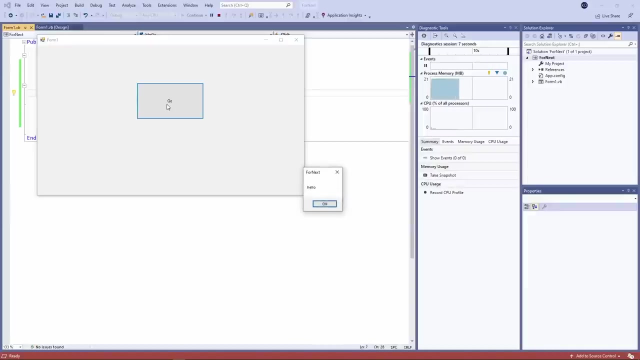 this: any code that I write between for and next will execute repeatedly, In this case five times, because I'm counting from one to five. Let's begin with a simple message. Give it a try. Hello, once, twice, three times, four times, five times. 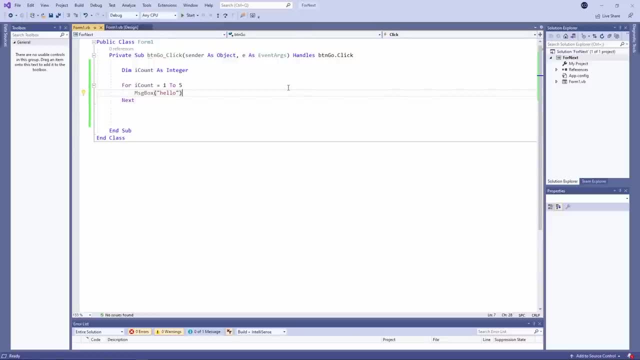 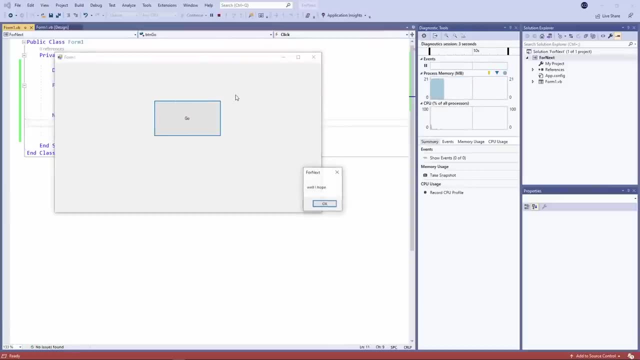 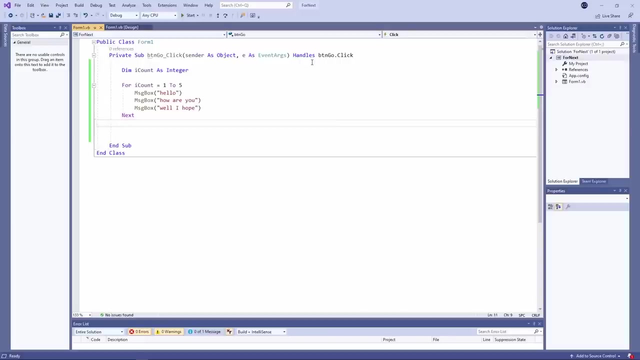 Now, that was a single line of code, but let's put a couple more inside the loop. Try it again. Hello, how are you well? I hope once. Hello, how are you well? I hope twice. So these three lines of code are executing in sequence five times. 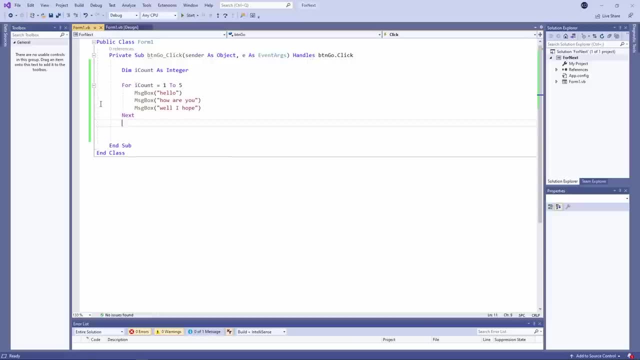 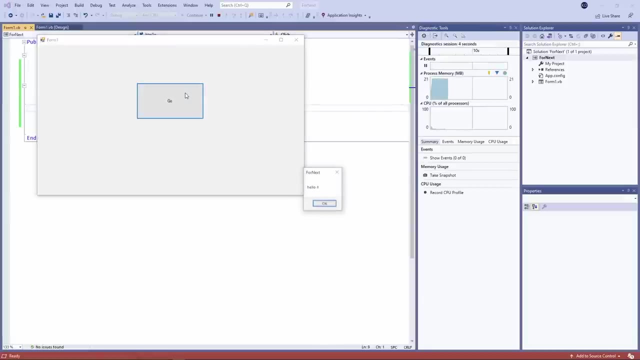 Let's take it back down to one line for now. I can display the value of iCount as part of the message like this: Hello one, hello two, three, four, five. Let's do something a little more interesting. 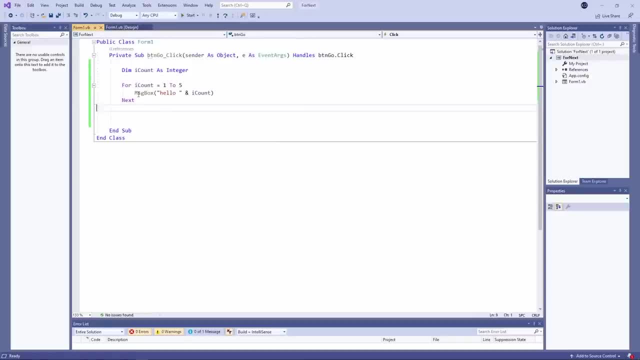 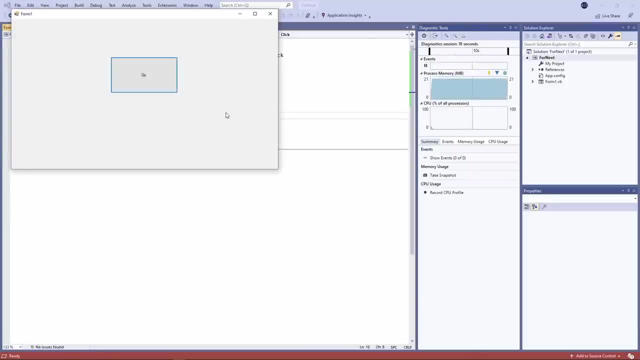 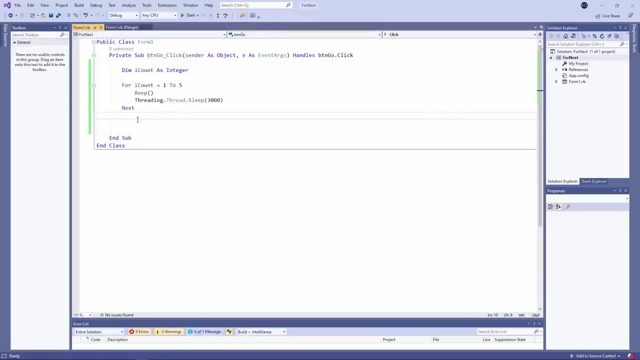 My program will beep every time we pass through the loop. The beep command is very straightforward: Threadingthreadsleep means pause for three seconds. Something nice about a looping construct such as the for loop is I can change the number of iterations as easily as this. 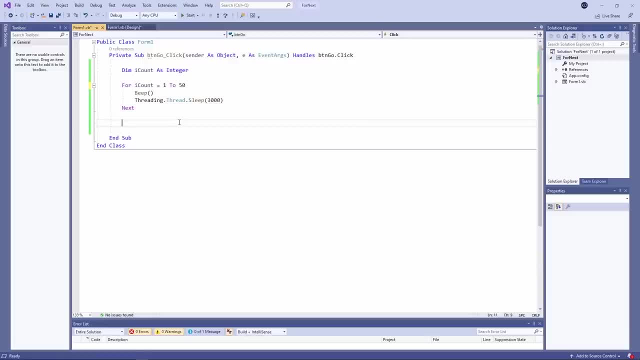 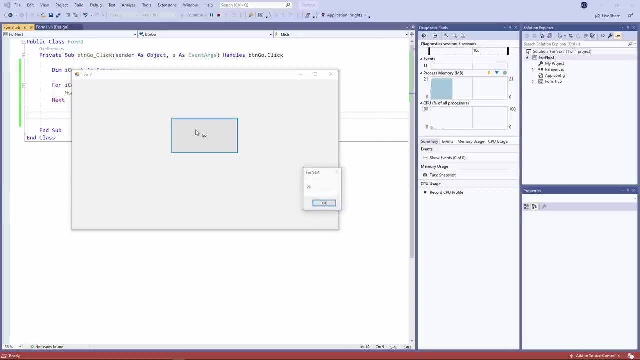 The code inside the loop will now execute fifty times. I can also change the step value like this: I'm going to count up from 1 to 50, five at a time. 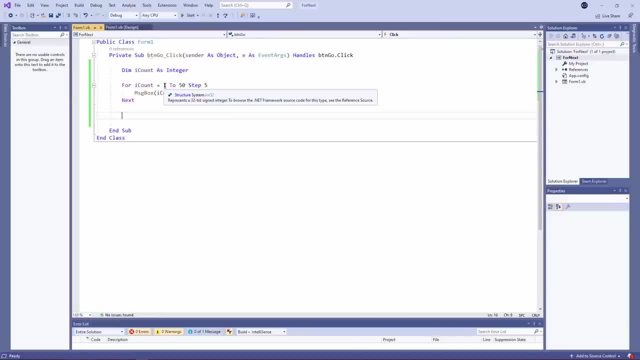 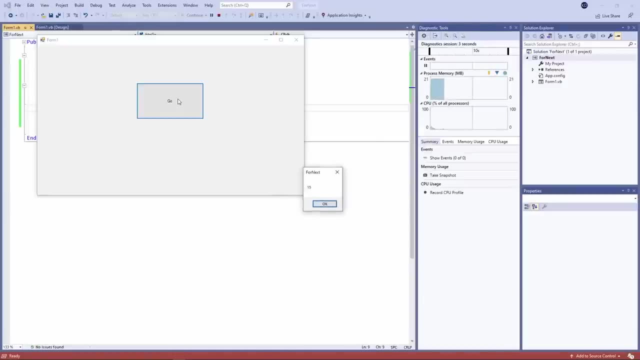 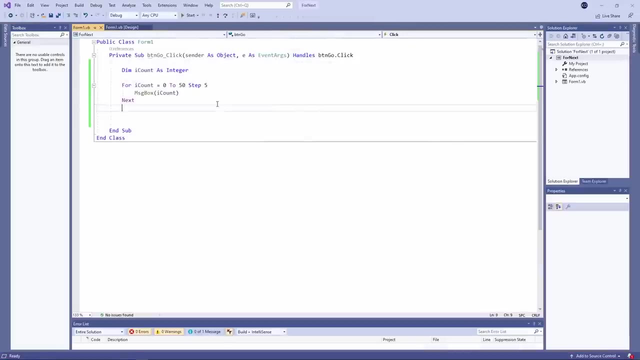 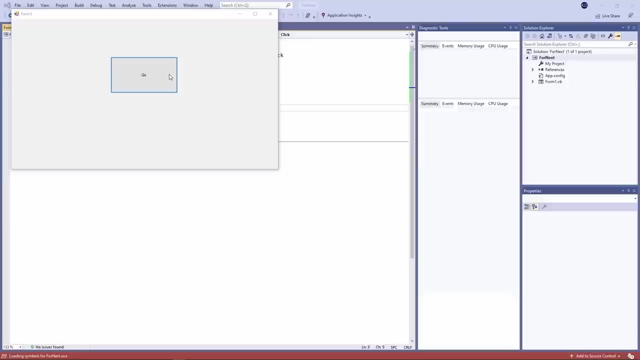 Perhaps it makes more sense to count from zero. I can also count backwards. In this case, I'm counting from 50 to zero and I'm stepping minus five at a time. 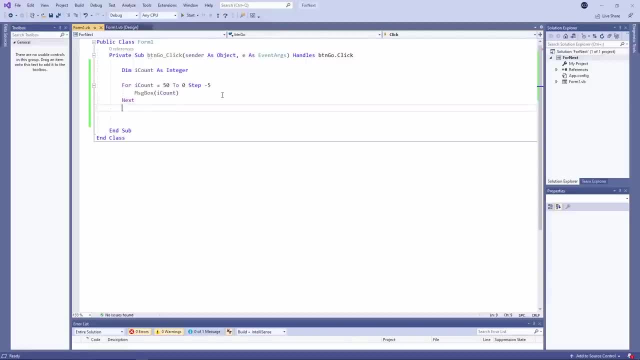 If I want to display the output in a single message box rather than separate message boxes, I could do something like this Inside the loop: I'm not doing any output, I'm simply building the output string. I'm saying: let stout equal, whatever it used to be, and then something else. 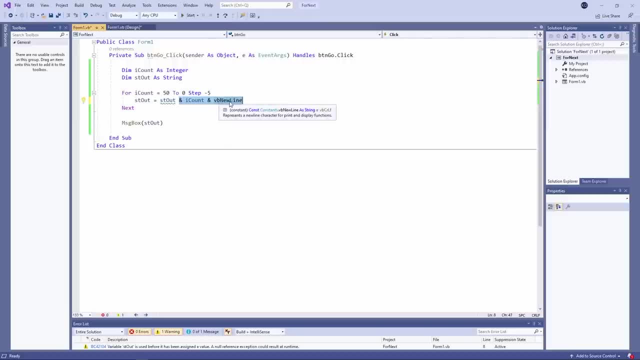 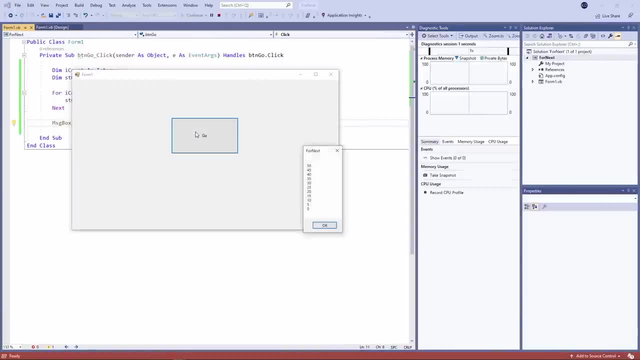 In this case the value of iCount, along with a new line operator. This time I only have one message box outside of the loop, And that's quite a common technique. So there it is, The for loop. In the next video we'll look at the do loop. 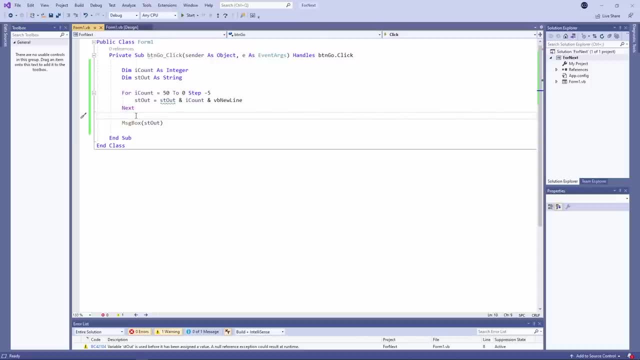 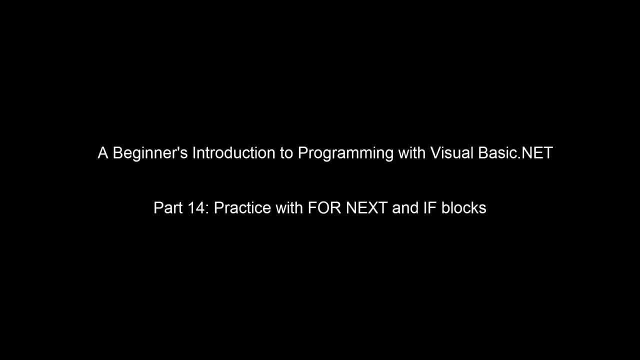 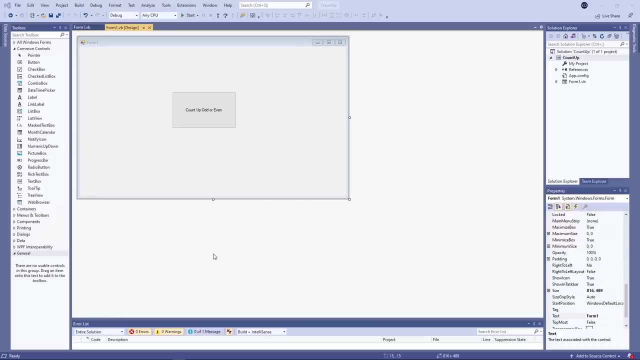 And then, following that, you'll see how the looping constructs really come into their own when working with array variables. Before we move on and look at another iteration construct, I thought it would be a good idea to get some practice in with what you've already learned. 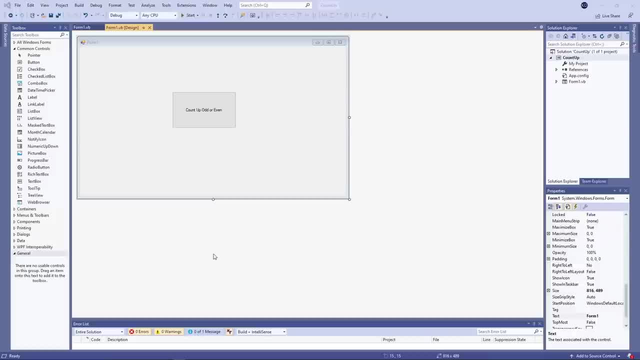 I've written a program here which makes use of an if block and a couple of for loops. I'll show you what it does first. then you can pause the video and try to write it yourself. When you're ready, you can look at my solution. 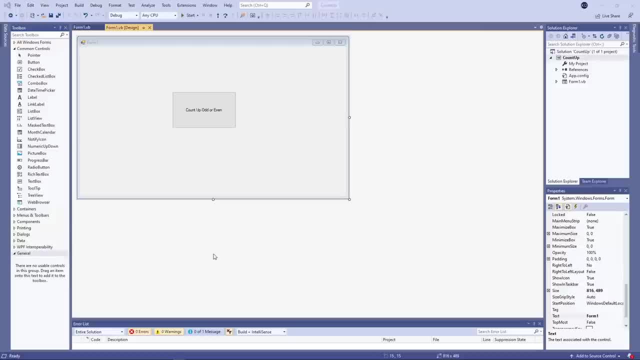 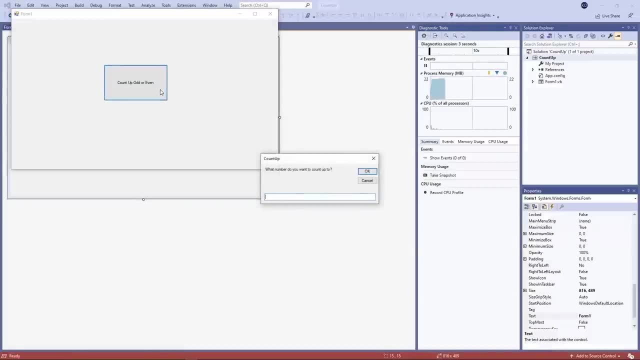 My button has the text count up odd or even, because that's what it does. Let's see. First I'm asked: what number do you want to count up to? I'd like to count up to 10.. Then I'm asked: do you want odd numbers or even numbers? 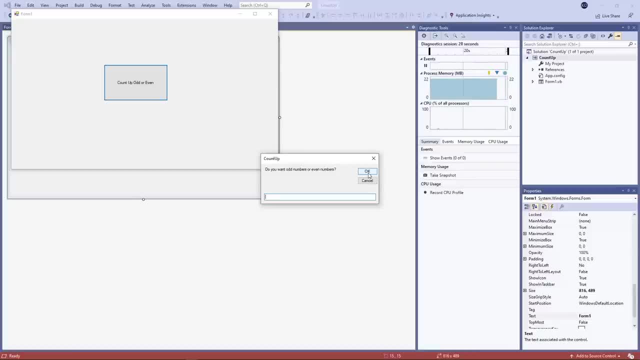 Notice: I'm using an input box here. You've seen this in an earlier video. I want the even numbers And my program comes back with 2,, 4,, 6,, 8, 10.. Let's run it again. 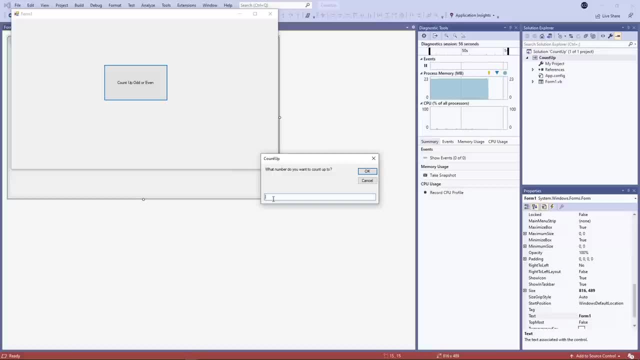 What number do you want to count up to? I can choose any number I like. I'll go with 10, again, Odd or even numbers. Let's try the odd numbers this time: 1, 3, 5, 7, 9.. 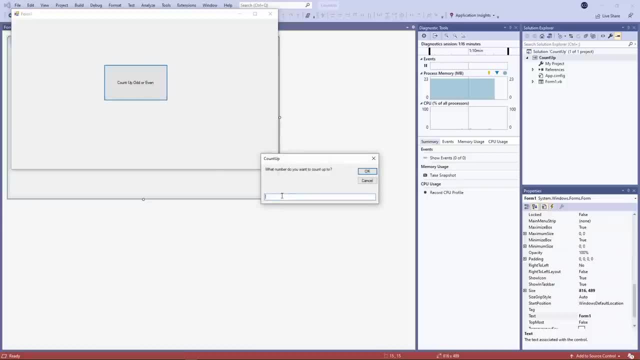 And that's it. Let's just give it one more try. Let's count up to 20.. Odd, or even Let's go with odd again. So that's the idea. If you want to try writing this program yourself, pause the video now and give it a go. 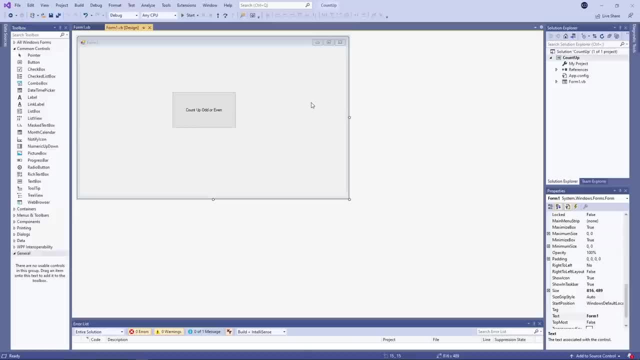 And then you can resume the video when you're ready to see my solution. I should say there's no one way to solve this problem, And that's it. I hope you enjoyed this video. I hope you found it useful And if you have any questions, feel free to ask them in the comments. 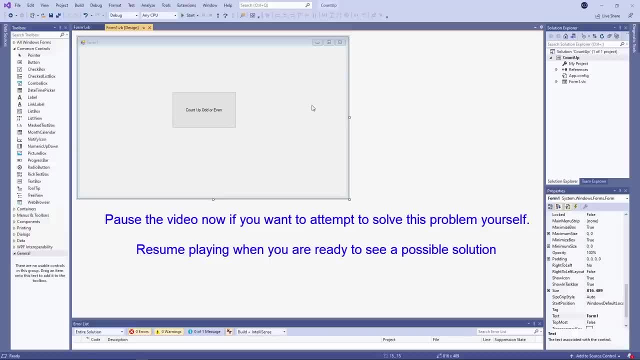 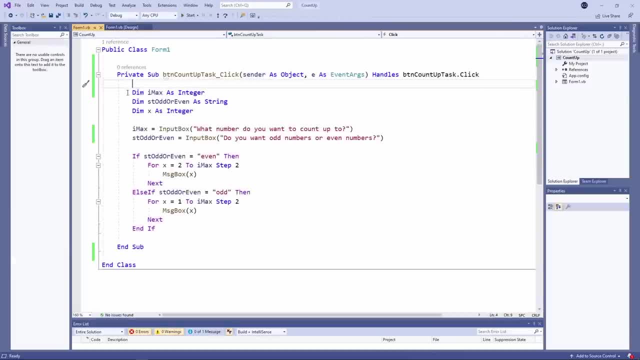 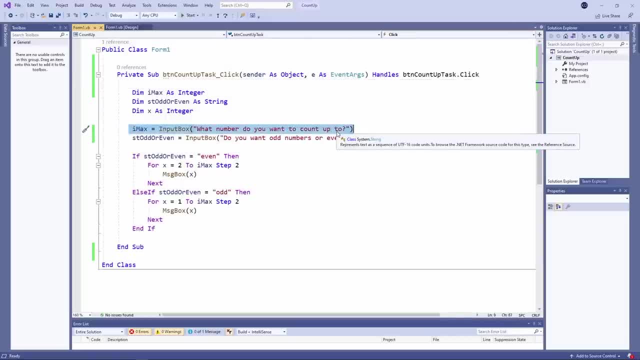 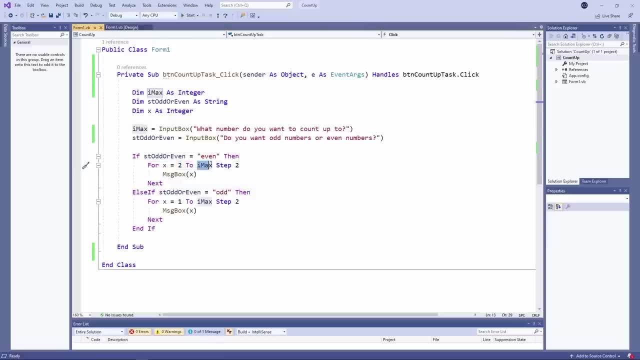 Bye, Bye, Bye, Bye, Bye. step clause to say that I want to step two at a time. So that's going to give me the even numbers up to the number that the user types in Else, if stod or even is equal to odd, then I have a. 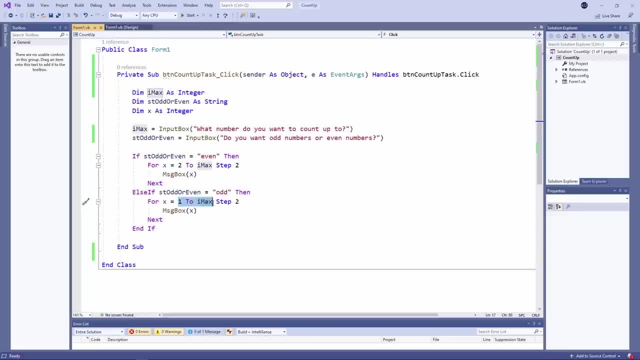 for loop which starts at one, runs to imax, but also steps two at a time. So we start with one, then we add two, then we add two, and so on. As I said, this is just my solution You might have. 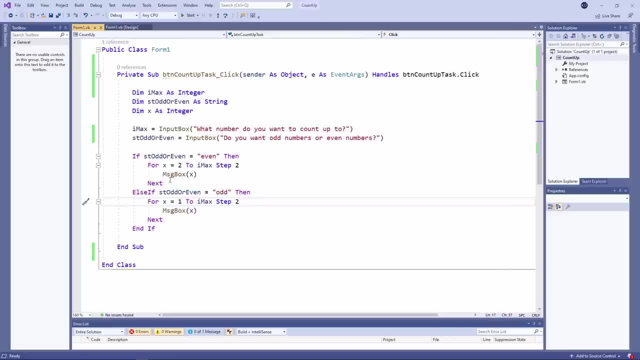 come up with something slightly different. For example, you might have used two separate if statements, like this, And that's fine because it will work. Having said that, using a single if block with an else if clause is a little bit more efficient, because this program will have to. 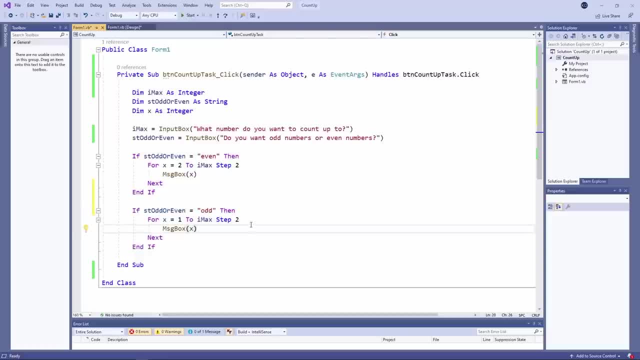 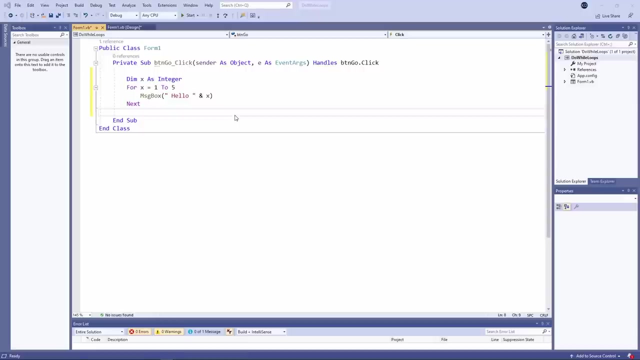 perform both tests. Did you get something similar? Did yours work? If not, why not try my approach? You previously saw how to make a line of code, or indeed a block of code, execute repeatedly using a for next loop like this one here: 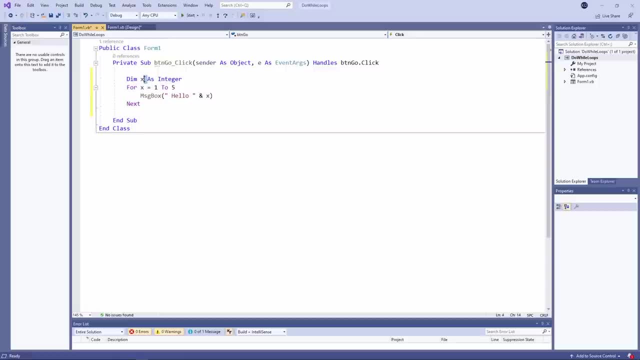 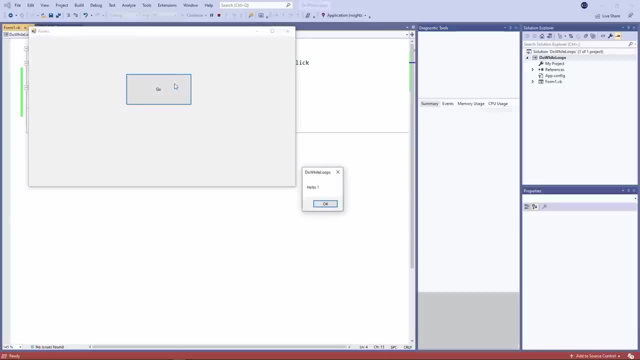 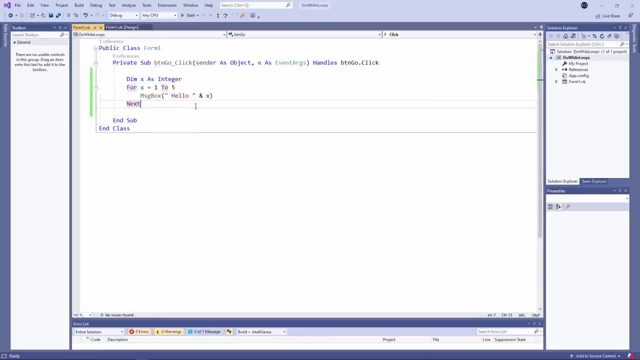 I'm using a variable, which I've named x, to count my way through the loop. Let's just remind ourselves what it does. Personally, I tend to avoid using letters of the alphabet for variable names. I like the names to be a little bit more meaningful. So I'm going to rename x to something a little more appropriate. 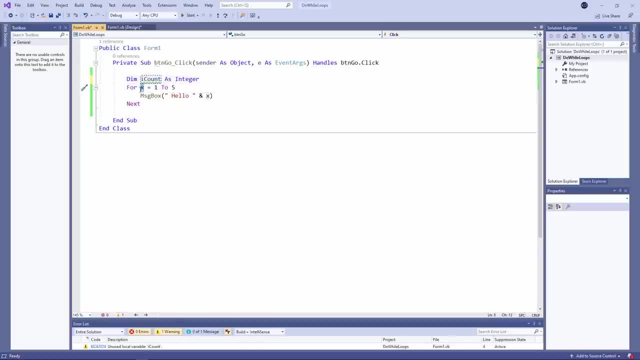 I'm going to rename x to something a little more appropriate. I've called it iCount instead. i because it's an integer, and count because that's what it's for It's: to count my way through the loop. In this video, I want to show you an alternative way to make a line of code or a block of code execute. 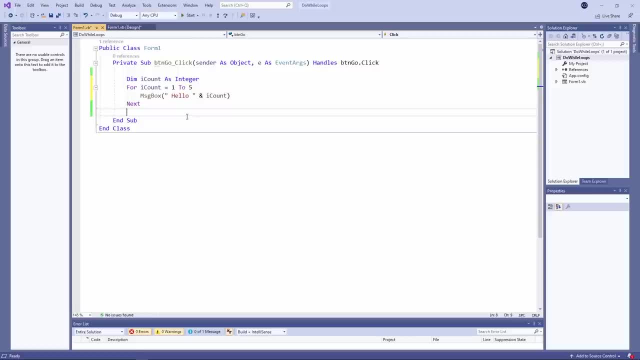 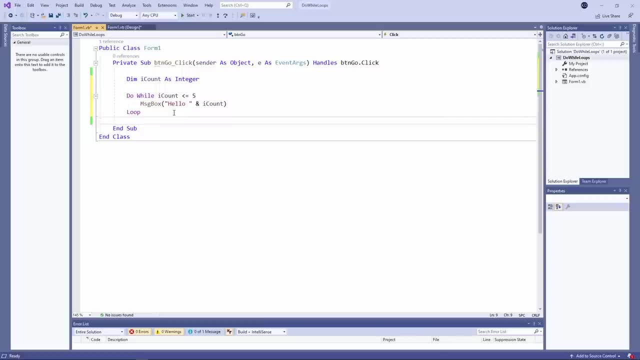 Now you might be tempted to give this a try. as it stands, I strongly recommend that whenever you're writing code that contains looping constructs, you should always save your code first, And that whenever you're writing code that contains looping constructs, you should always 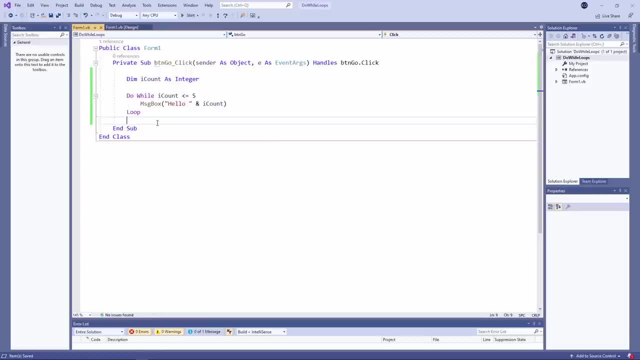 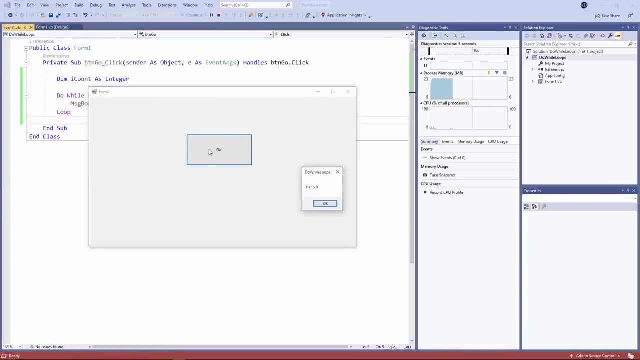 save your code first. Watch what happens when I run this: Hello zero, hello zero. This will go on forever just saying hello zero. Let's see if we can work out why I need to stop the program. Fortunately, I can still see this red square here. 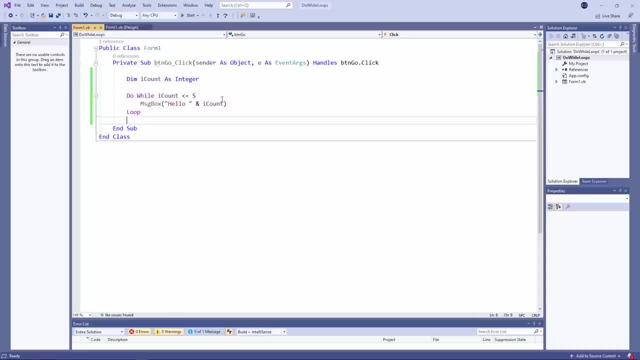 So that will force the execution to stop. I've said that I want the loop to repeat. while the value of iCount is less than or equal to five, Immediately after you've declared a numeric variable, it will contain zero. So by the time we get to this line of code, iCount contains the value zero, which, of course. 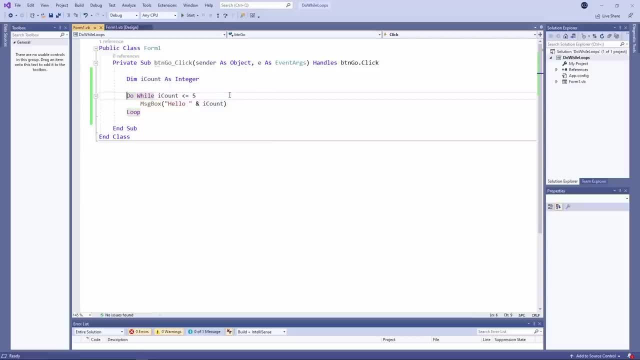 is less than or equal to zero, Less than or equal to five. So we output hello zero. When the loop repeats: iCount is still zero, Its value hasn't changed. So we output the message again, And then the loop repeats again, and again, and again. 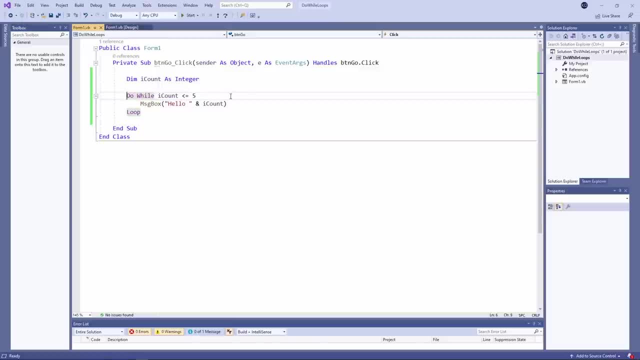 It's called an infinite loop. It will go on forever. Because I'm using a do while loop, I need to make sure that I write some code to increment the value of iCount. I'm going to increment the value of iCount before I do the output, like this: 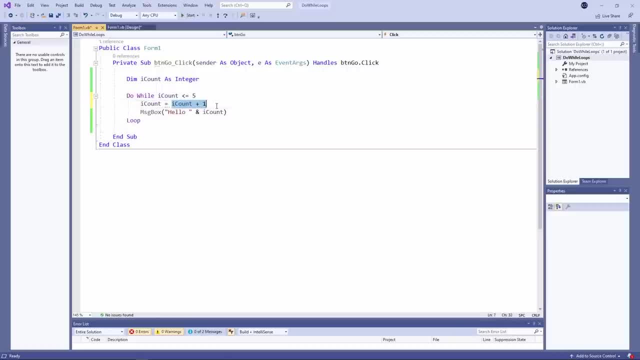 So all this line of code says is take the value of iCount, add one to it and then put the result back into iCount, overwriting what's already there. In other words, add one to iCount. So at the top of the loop we check if the value of iCount is less than or equal to five. 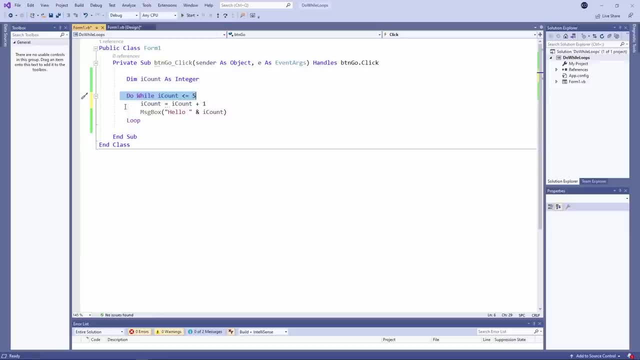 which first time around it is It's equal to zero. Then we increment it. So now iCount has the value one, Then we do the output hello one, We go back to the top of the loop and because iCount is still less than or equal to five, 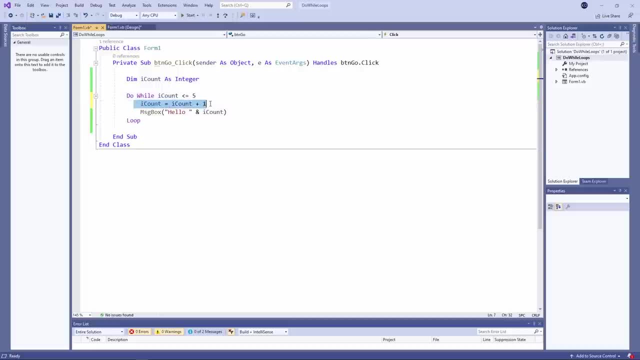 we get back into the loop code and we add one to it. iCount now has a value of two, So we can output hello two And around and around. we go until such time as iCount is no longer less than or equal to five. 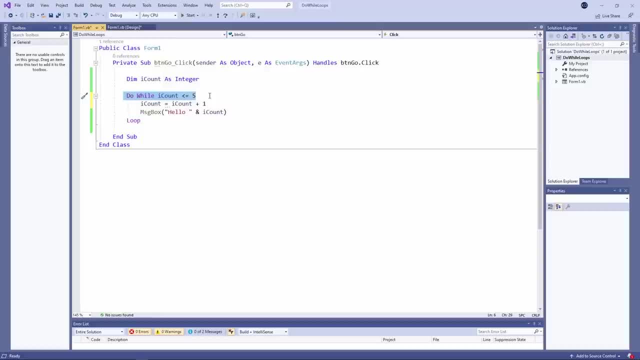 We've met the so-called exit condition of the loop, So we can exit the loop and the program will continue down here. Let's just put a line of code in here just to prove that the program has dropped out of the loop. 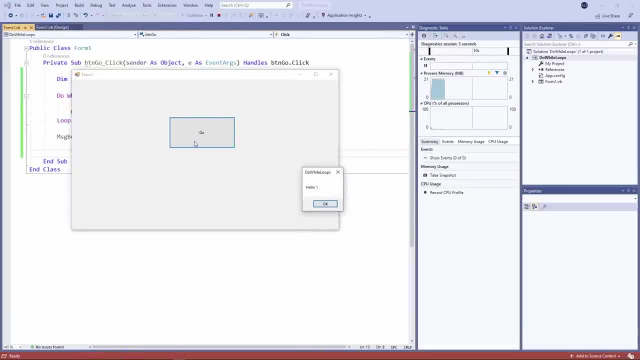 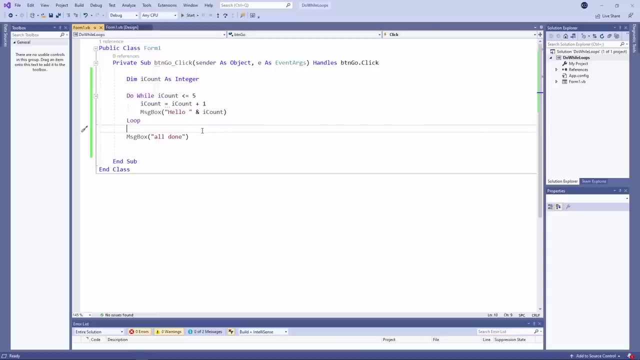 Now let's give it a go. Hello, one, two, three, four, five, six. We'll have to look at that and think about what it is, Think about why that's happening, and then all done. I only wanted to count up to five, but it actually counted up to six, and that has to. 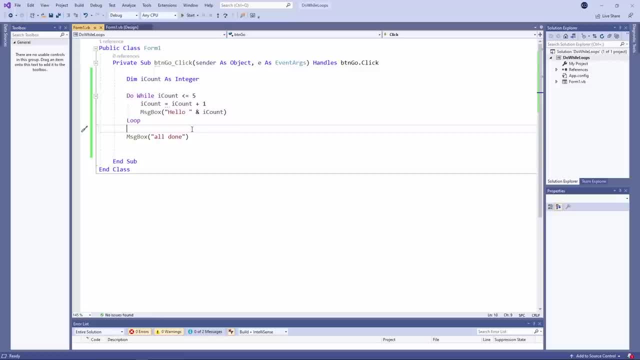 do with the exit condition of my loop. I said I want to loop while iCount is less than or equal to five, which means my loop will continue if iCount is equal to five. When iCount is equal to five, I add one to it. 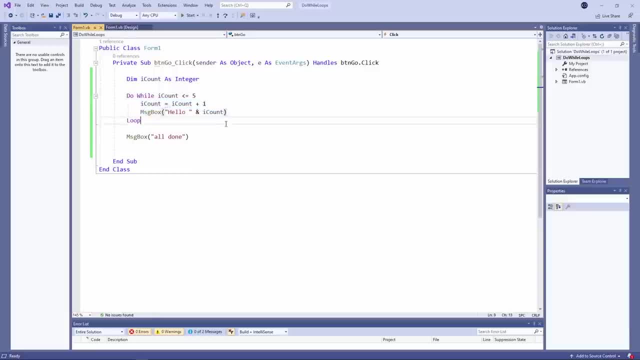 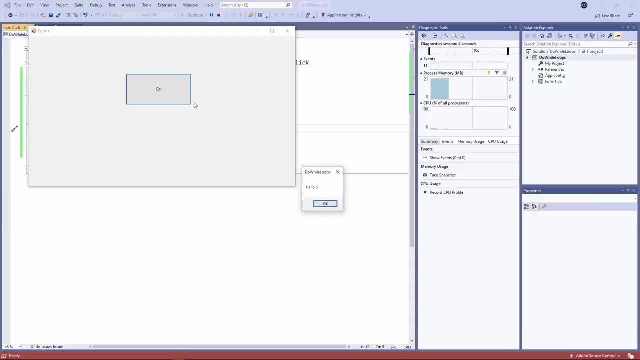 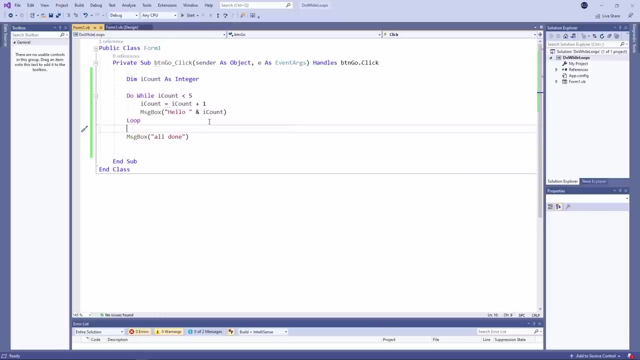 So it becomes six and I do another output. All I need to change is that exit condition Do while iCount is less than five. That's better. You need to be mindful of the contents of the variable which you are using to count. 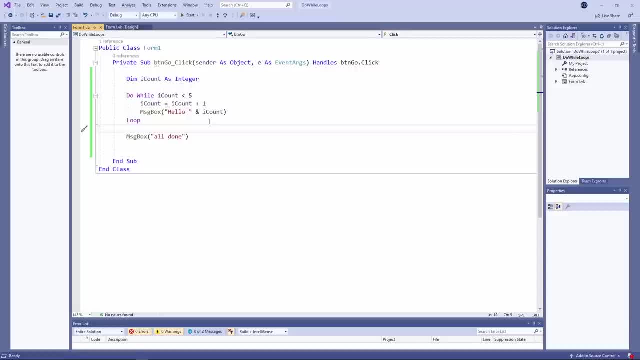 your way through the loop. Now you might be wondering: Why do we bother with do while loops when we have four next loops? I've had to write more code to get the same effect. The answer to that question is that the do while loop is more flexible. 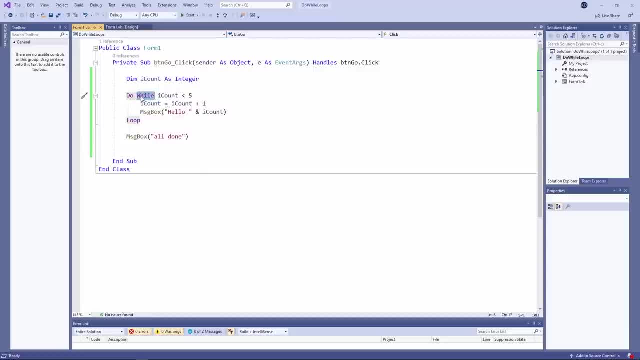 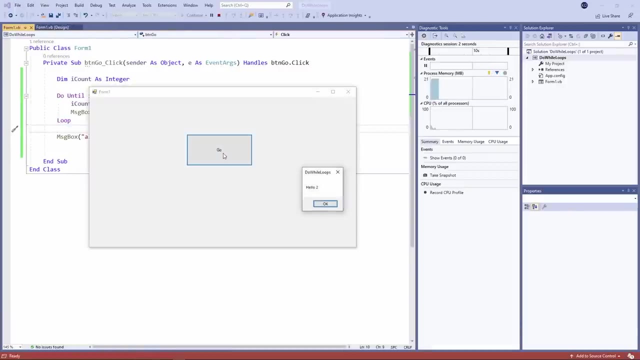 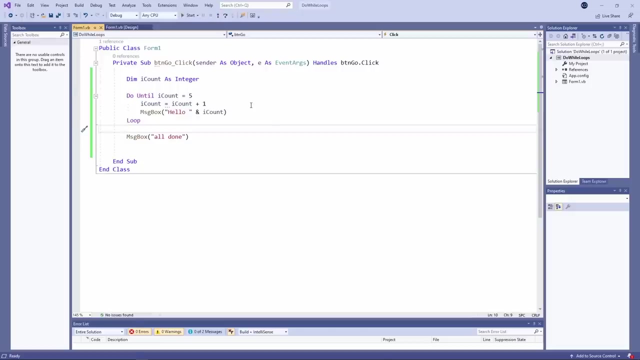 For example, I can say: do until iCount is equal to five. Strictly speaking, this is not a do while loop, This is a do until loop. Watch what happens when I run it: Exactly the same effect, But it means that I can build an alternative exit condition for a loop. 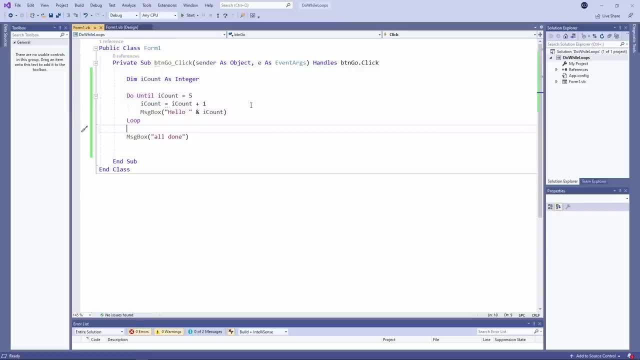 And, as you'll see later, sometimes it's more appropriate to use do until rather than do. while I can also do this, I'm just going to move this piece of code. So I'm saying: do This block of code And loop until iCount is equal to five. 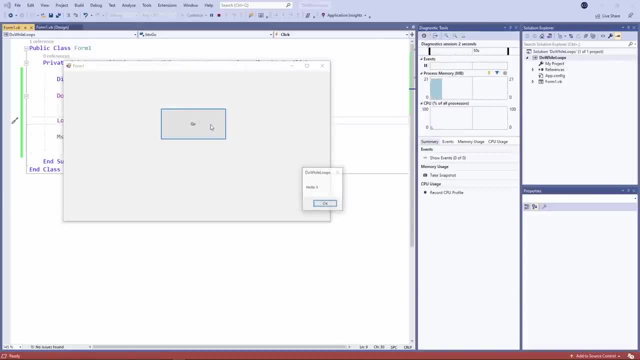 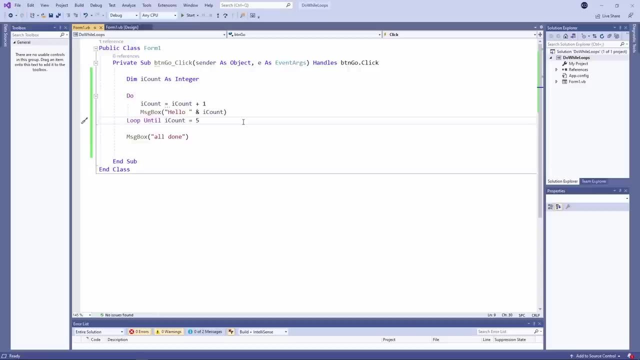 Let's take a look. Exactly the same effect, But sometimes it's appropriate to put the exit condition at the bottom of the loop. This means that the code inside the loop will execute at least once. If the exit condition is at the top of the loop, it might not execute at all. 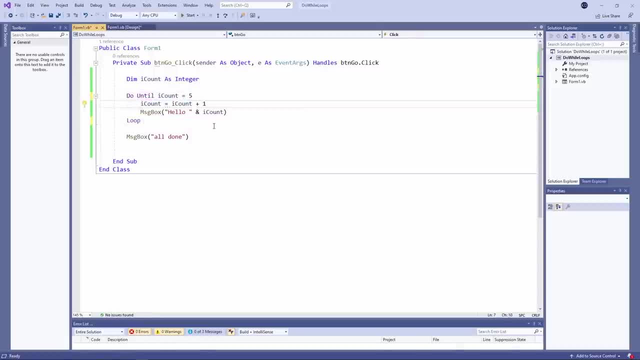 If, for example, something has set the value of iCount to be equal to five before we go into the loop like this, then the code inside the loop won't execute at all. We've already met the exit condition, And there's one more form of the do while loop, if I may call it that which I'd like. 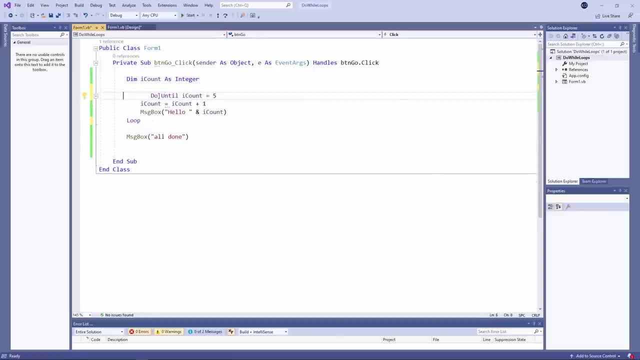 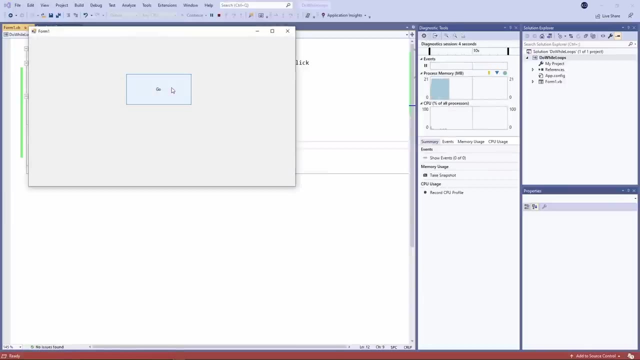 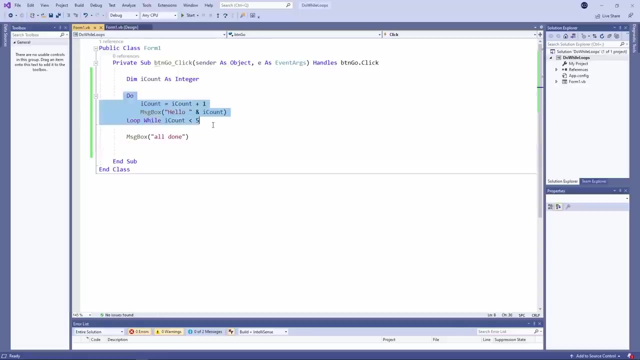 to show you. And there's one more form of the do while loop which I'd like to show you. And there's one more form of the do while loop which I'd like to show you Does the same thing. Let's look at those four variations next to each other so we can compare them. 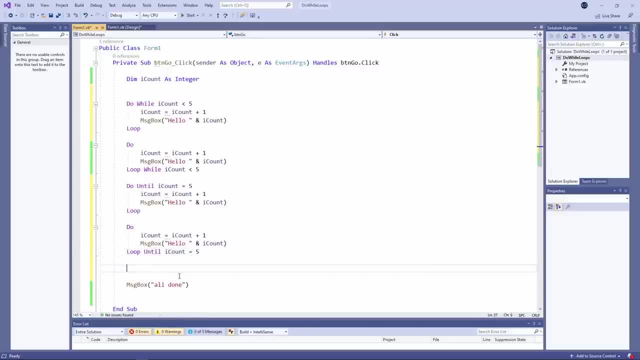 Four loops that do exactly the same thing. Now we need to be careful Here. I need to reinitialize the value of iCount in between each of these loops. It starts off here with a value of zero, But by the time we've dropped out of the first loop it will have a value of five. 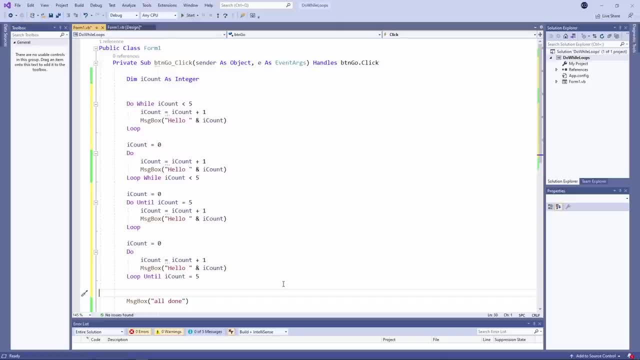 As I said, you need to be mindful of the value inside the variable which you are using to count your way through the loop. For good practice, I'm going to explicitly initialize it here as well, Although I know in this particular program it will have a value of zero at that point. 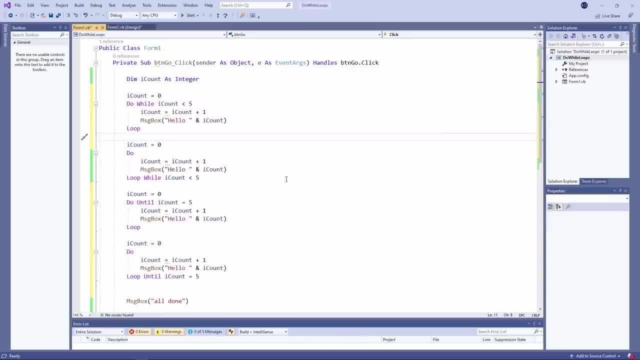 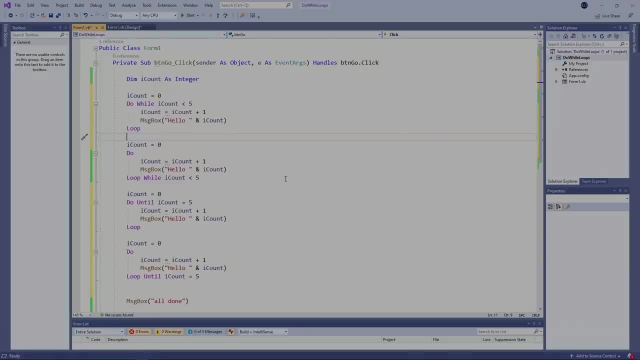 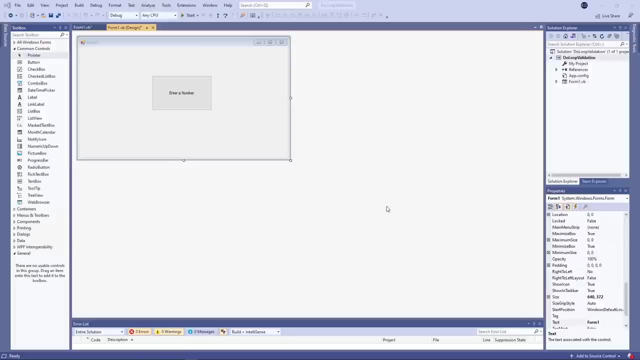 So there you have it: Four different variations of the do while loop, Or the do until loop, if you'd rather call it that. I'm going to show you a useful application of do until loop. do-while loop. I want the user to enter a number, and only a number. A do loop can. 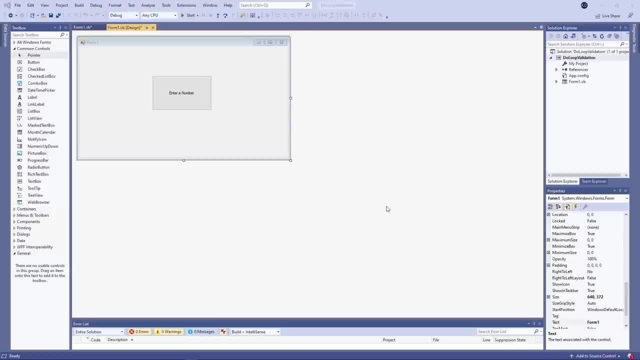 be used to repeatedly prompt the user if the data is invalid. I'm also going to show you why a do loop is called a condition-controlled loop. You might remember that a for-next loop is called a count-controlled loop. Let's write some code. 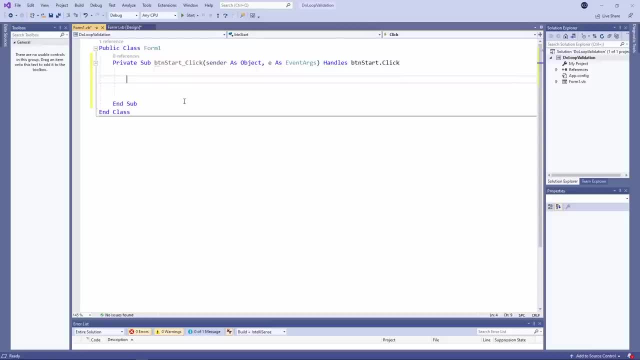 Let me show you something which might strike you as rather silly, but it makes a very important point. I'm using an input box function to prompt the user to type in their name, but the name must be Kevin, so I've placed this instruction inside a do-while. 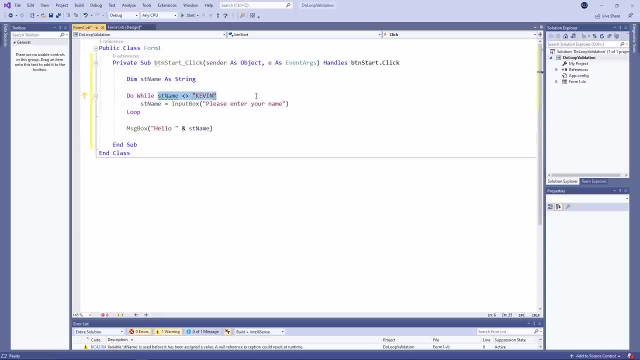 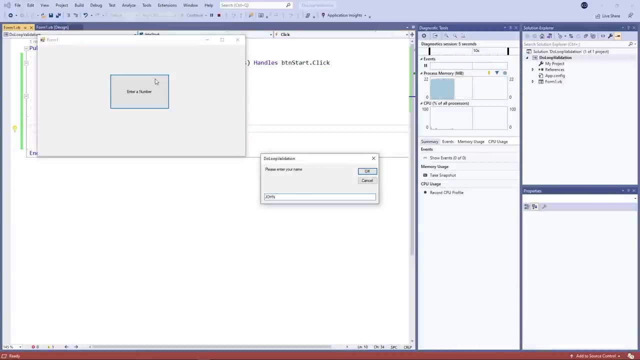 loop And look at my exit condition. Do-while stname is not equal to Kevin. When we drop out of the loop, I simply output the name that was entered. Let's give it a try. I'll try, John. That's no good, Ben, Nope, Enzo. Anything I type is invalid. 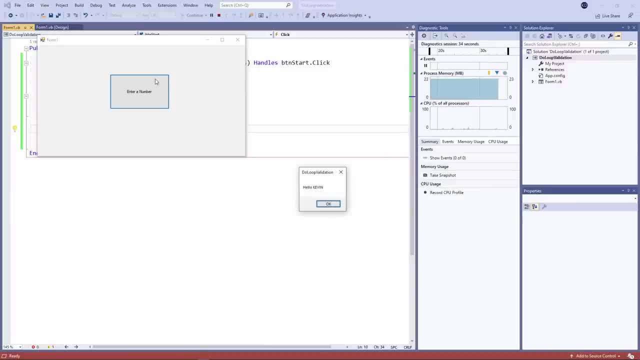 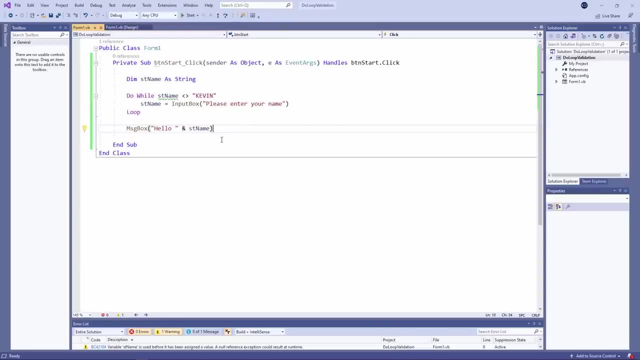 unless it's Kevin. You can see why this is called a condition-controlled loop rather than a count-controlled loop. I'm not incrementing a variable to determine how many times I pass through the loop. There's no loop counter involved. Let me show you another approach. Do-while true equals true. I could have just as easily. 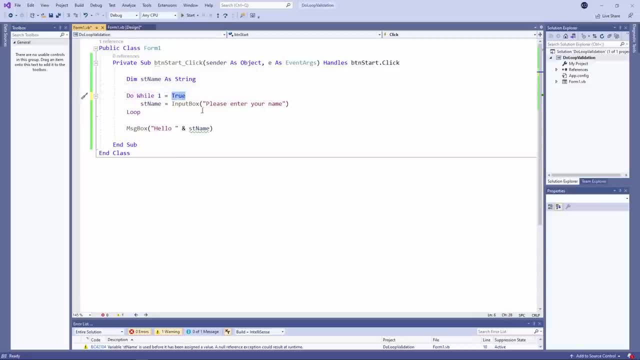 said: do while 1 is equal to 1.. That might strike you as a rather ridiculous exit condition, because 1 always equals 1.. Essentially, what I've written here is an infinite loop. True equals true is more typical, In fact. I can just say: do while. 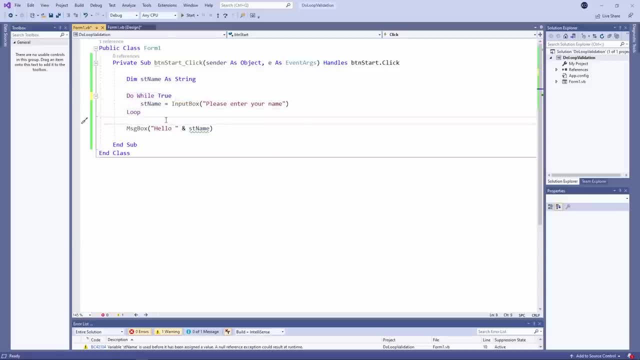 true, It means exactly the same thing. But if I have an infinite loop, well how do I get out of it? I can do this: I capture the input, test it to see if it's what I'm looking for, and if it is, then I force an exit from the do loop by using the. 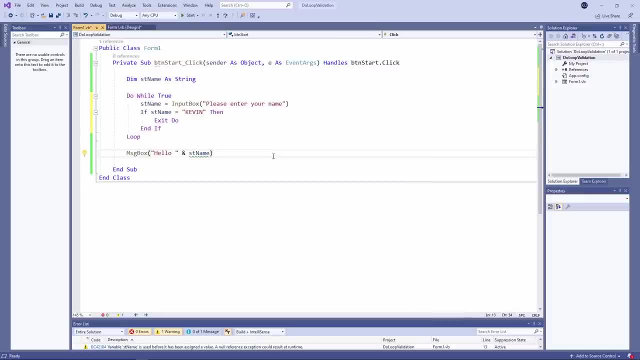 command exit, do. Once again, you can see that I'm not counting my way through the loop. I'm exiting the loop in a different way. So how is all of this useful? Well, as I said, I want to write a program to prompt the user. 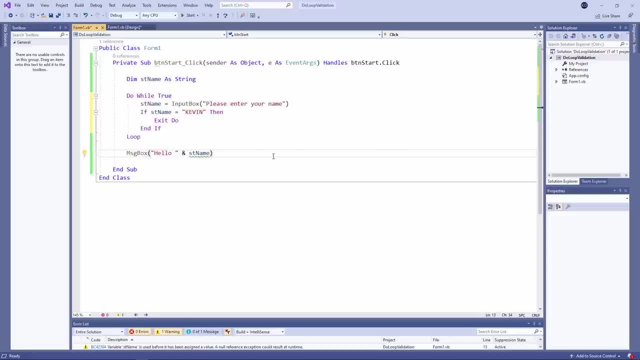 to want to exit the loop. So I'm going to write a program to prompt the user to enter a number, and only a number. Take a look at this. I've declared two variables, one called sth, because I want to capture. 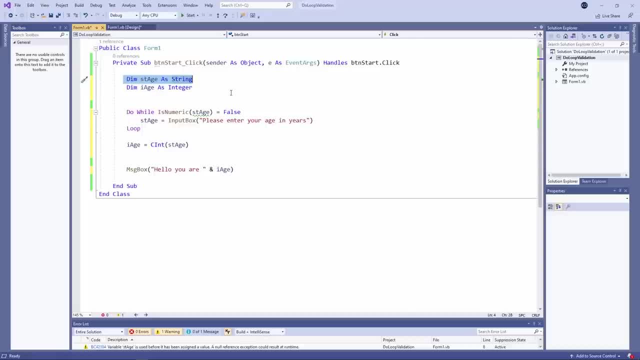 the user's age, but notice I've declared it as a string And then I've declared another variable called iage, which is an integer. I'm prompting the user to enter their age and I'm assigning the value to sth. This is a temporary measure so that I can test. 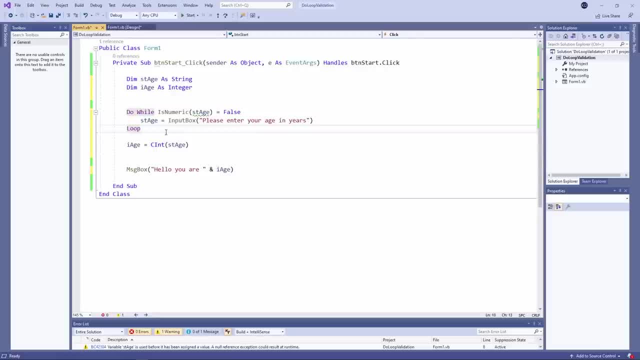 sth And look at my exit condition. Do while is numeric sth equals false. I'm going to do while is numeric sth equals false. In other words, while, whatever the user types in, cannot be converted into a number. To understand this, you need to appreciate that the input 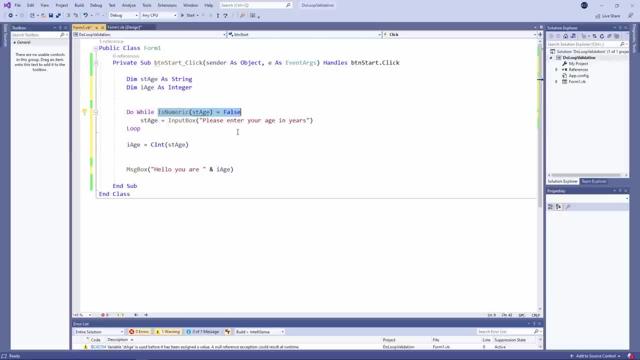 box function always captures a string. So, for example, if I'm prompted to type a number and I type, let's say, 59, I'm actually typing the string 59. If I attempt to assign that string to a numeric variable, I'm actually typing the string 59.. If I attempt to assign 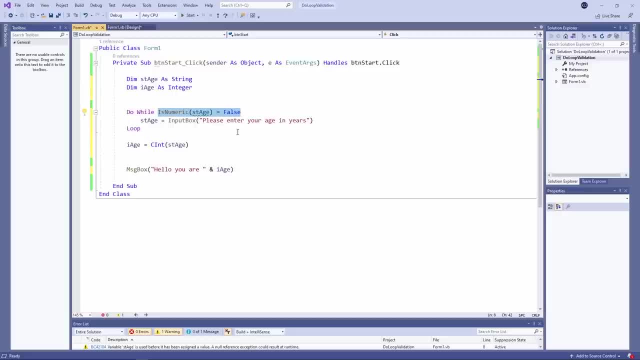 that string to a numeric variable. I'm actually typing the string 59.. If I attempt to assign that string to a numeric variable like iage, it'll be fine. Visual Basic will do something called implicit type conversion. It will automatically convert it into an integer because it can. 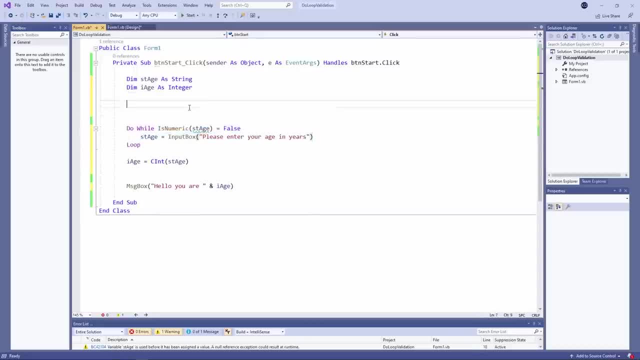 For example, this line of code will be absolutely fine as long as the user types in a string that can be converted into an integer. If, however, when this line of code executes the user types in a string, it carries the value less than the integer. 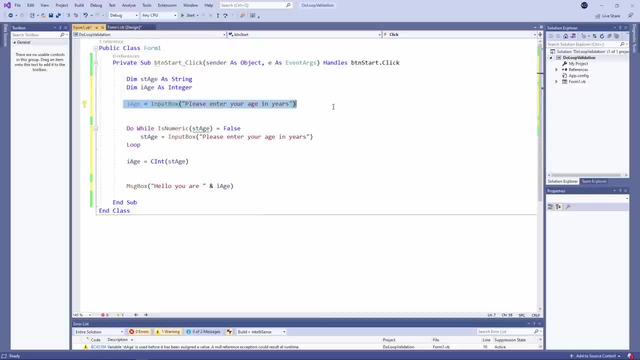 Now you've solved this 식. Now you can actually convert this ¯ and ¯ as string And you'll get an answer like this: just press Enter. If I want to go back and say, iage, I haven't like, hello, it will crash the program because visual basic can't automatically. 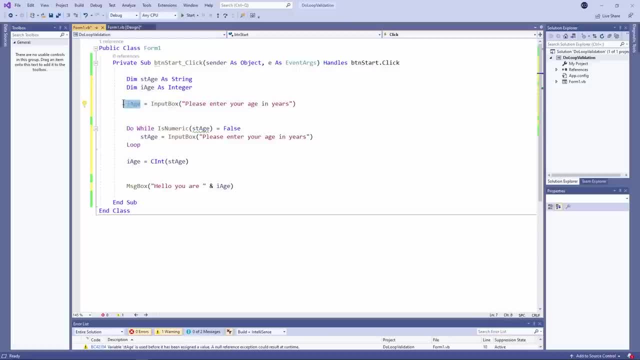 convert that string into something we can save into an integer variable. I'm trying to prevent my program crashing for that reason, so instead I'm asking the user to type in their age, but I'm storing it into a string variable. it doesn't matter what they type. when we assign it to a string variable, it'll. 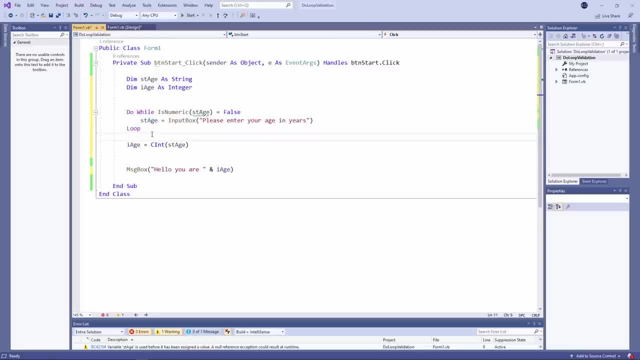 work, but because I want a number, I keep asking the user to type something until such time as I can convert it into a number, and that's what is numeric is telling me whether or not a variables contents can be converted into a number. I could ask the same question in a slightly different way, like this for: 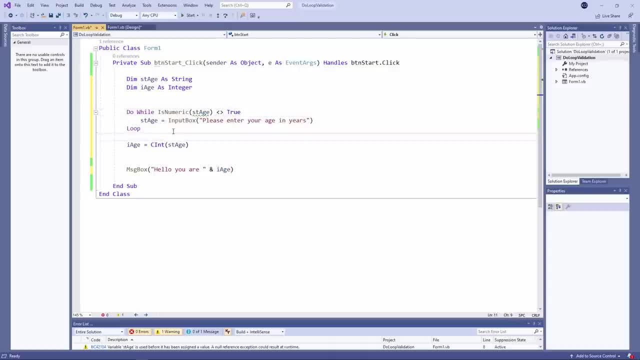 example, do while is numeric is not equal to true. it means the same thing as do while is numeric equals false. I can even ask the question like this: do while not is numeric? it's the same exit condition, just phrased in a different way. I'm using a logical 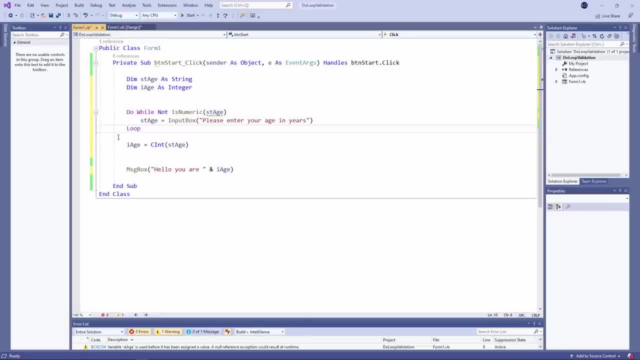 operator this time instead of a relational operator. it really is a case of take your pick. so we are repeatedly prompting the user to type in something we can convert into a number, and when the user finally types in something that we can convert into a number, we can convert it into a number. and when the user finally types in something that we can convert into a number, 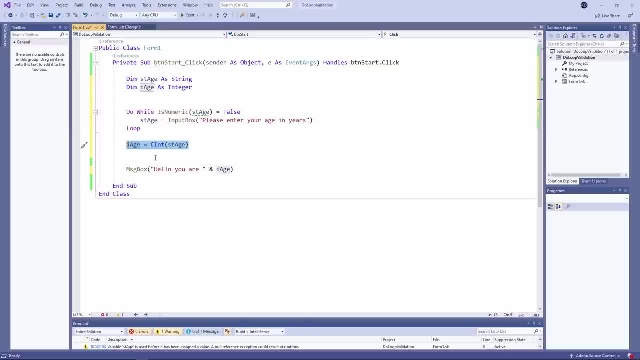 we do so. I'm using one of the type conversion functions, this time see int, that's short for convert to integer. so I'm converting this string into an integer, and I know that this line of code is not going to crash, because we wouldn't have got this far in the program unless the user typed in. 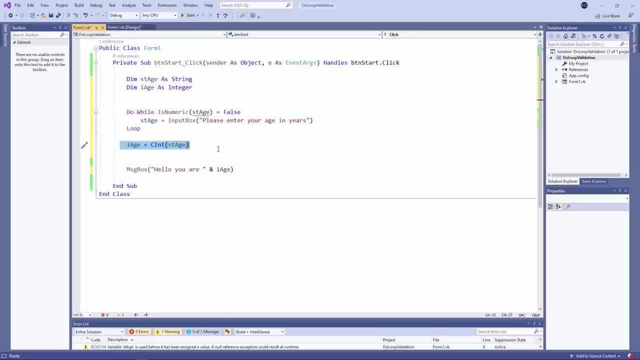 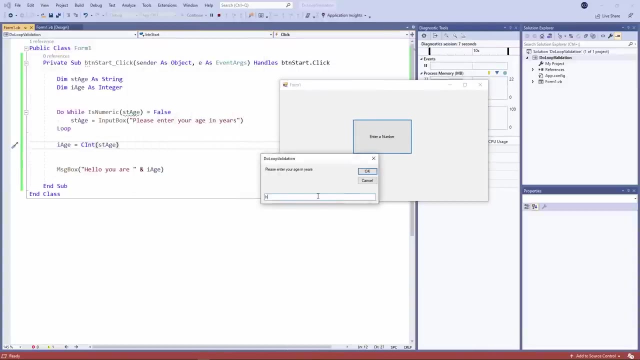 something that I could convert. this is called explicit type conversion. it's also called casting, when we change the data from one data type to another. let's give it a try. I'll start with some text. that's invalid, so I'm being prompted again. let's try some different text again. I. 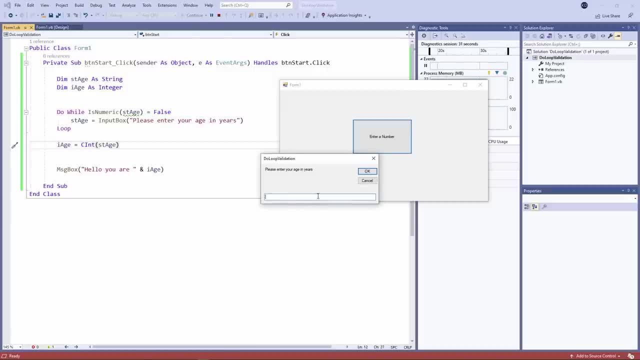 didn't type something which can be converted into a number, so the loop continues. let's try typing nothing at all. I'll just click OK. well, that's no good either, because that's what we call a zero length string. think of a pair of quotes with nothing in between. if I press the cancel button again, that's. 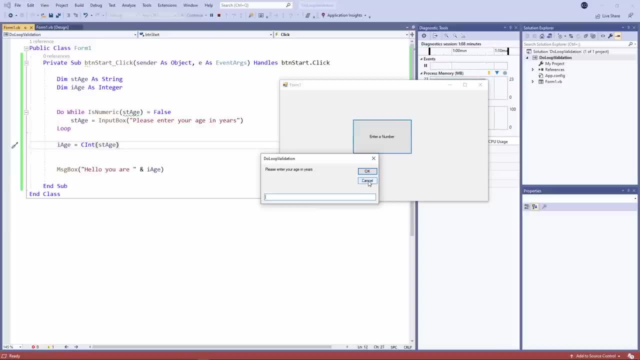 invalid. I can't get out of this until I typed something that can be converted into a number. remember that might look like 123, but it's actually the string one, two, three, but it's a string that can be converted into a number. so we drop out of the loop, convert the input into a number, store it in IH and then. 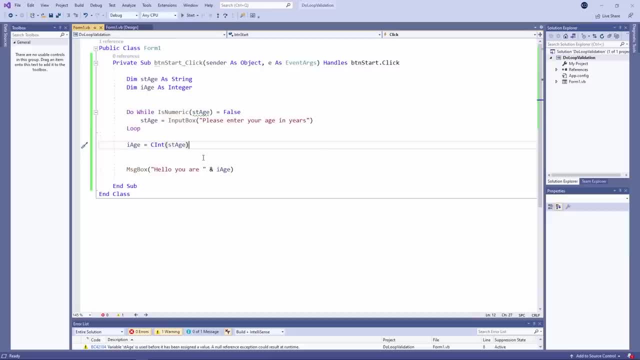 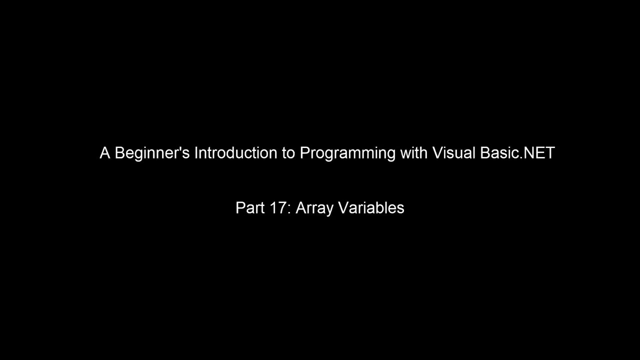 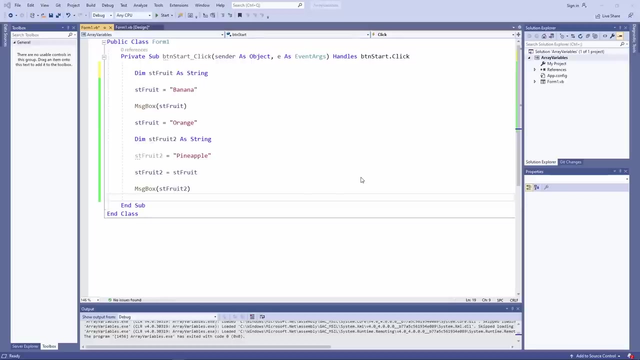 display it in a message box. so there you go, a condition-controlled do-while loop which I'm using to capture input and validate it at the same time. in this video, I'm going to talk about array variables. as you'll see, array variables are particularly useful when you want to 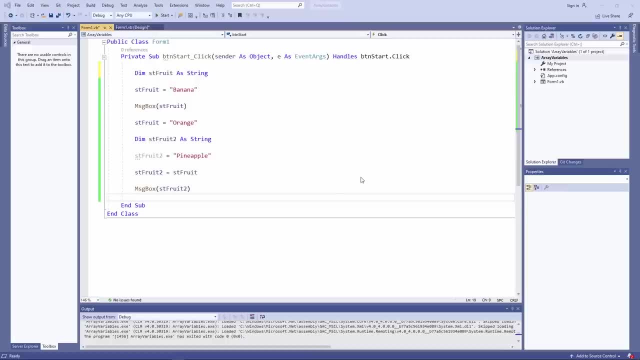 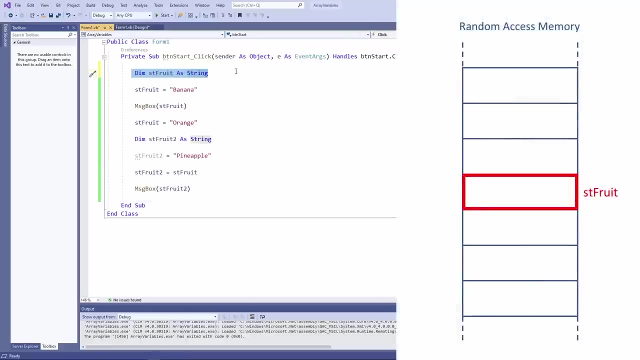 store a large number of related data items. in fact, once you've learned about array variables, you'll be able to write some very, very useful programs. before I begin, let's quickly review what's going on inside the computer's memory when we use regular variables. when this line of code executes, the operating system will. 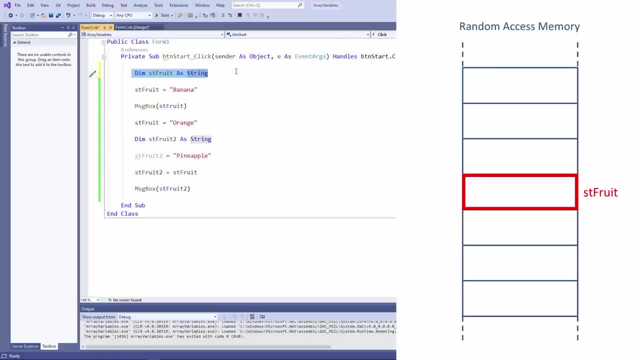 set aside a piece of memory and it will give it the name stfruit. the exact location of this piece of memory is entirely up to the operating system. it doesn't really concern us as programmers. but suffice to say no other program can use that piece of memory. it belongs to this program immediately after a string. 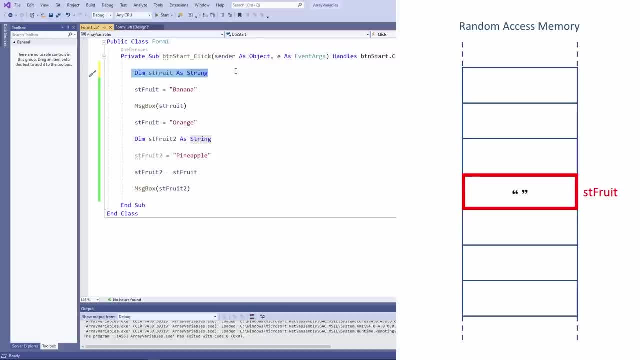 variable has been declared, it will contain something. it contains a zero length string. think of a pair of double quotes with nothing in between them. if you declare a numeric variable, for example an integer, then immediately after declaration it will contain the value zero for the purposes of this. 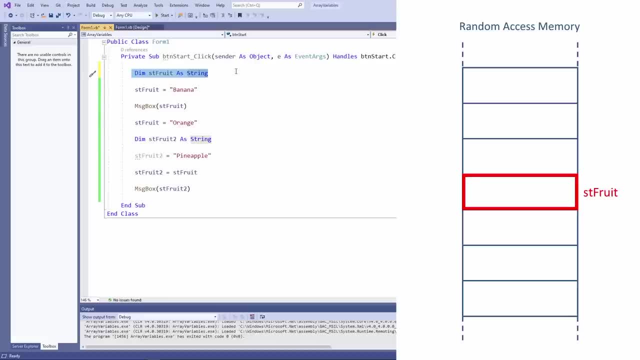 discussion. we don't really need to worry about this zero length string when this line of code executes. I'm assigning a value to the variable. I'm putting the text but not the value of the variable. I'm putting the text but not the value of the variable. I'm putting the text but not the value of the variable. I'm putting the. 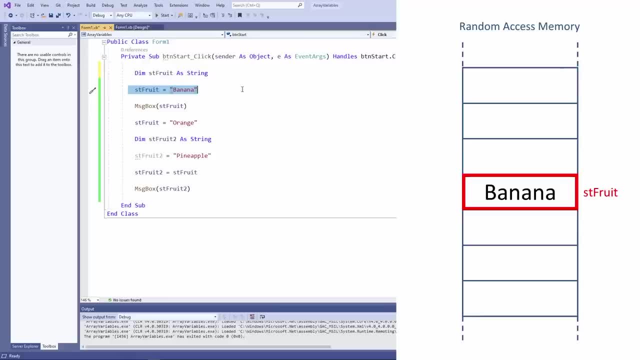 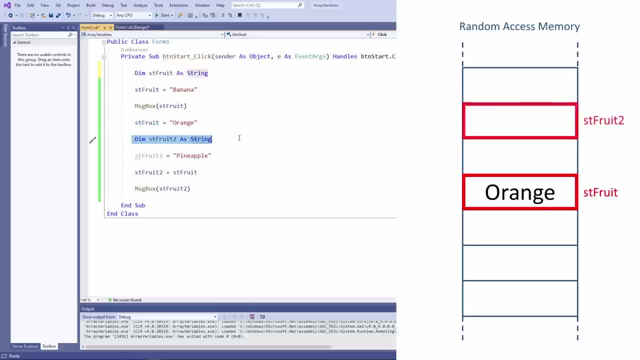 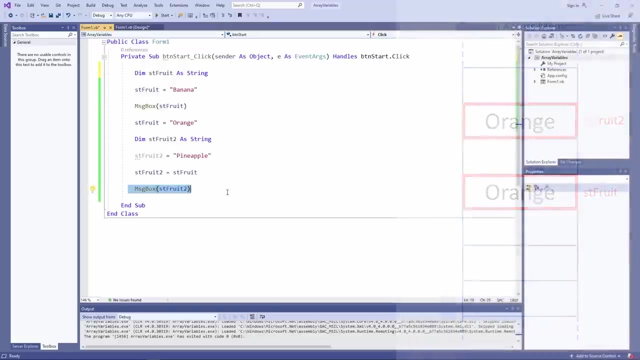 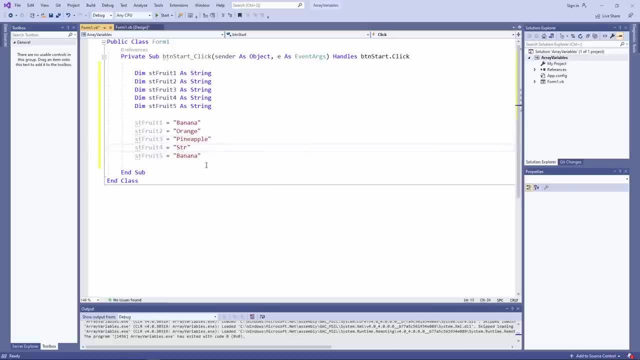 I've declared five separate variables and I've initialized them individually. If I want to output the contents of one of those variables, that's straightforward enough. as long as I know the name of the variable, That will output pineapple. But using regular variables like this to store a group of related data items is actually. 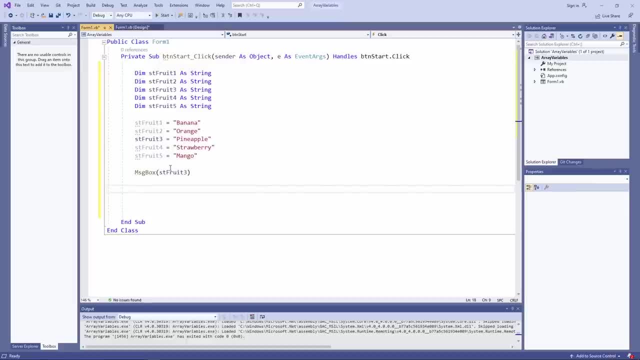 quite cumbersome. What if I wanted to store ten items of fruit, or even a hundred items of fruit? I'm going to end up with rather a lot of code. Instead of using five separate string variables, I'm going to use one array variable, like. 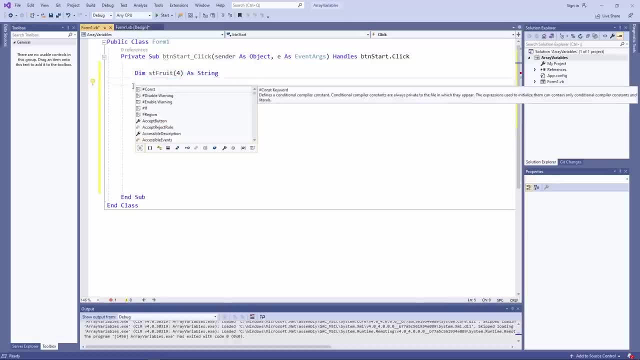 this. I've used quite a lot of copying and pasting. to speed things up, I'm also going to change the name of this variable, just to indicate that it is actually an array variable. I'm going to prefix the name with a. 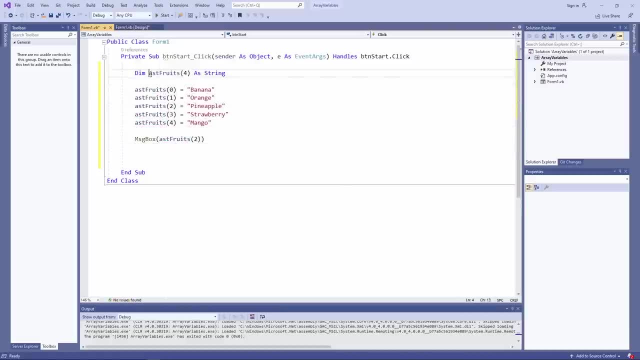 a because it's an array. st because it's an array of strings, And fruits because, well, that's what these are. You could actually call your array anything you like, but as you write more code, you'll see the benefits of a naming convention. 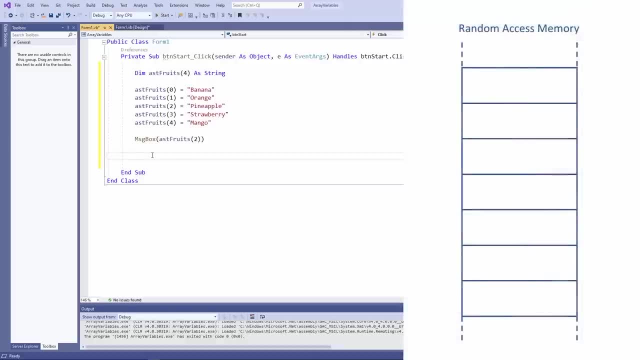 To understand what's going on here again, we should visualize what's going on inside the computer's memory. When I declare an array variable like this, I'm actually saying that I want to set aside a group of memory locations. To be more precise, I'm setting aside a group of contiguous memory locations. 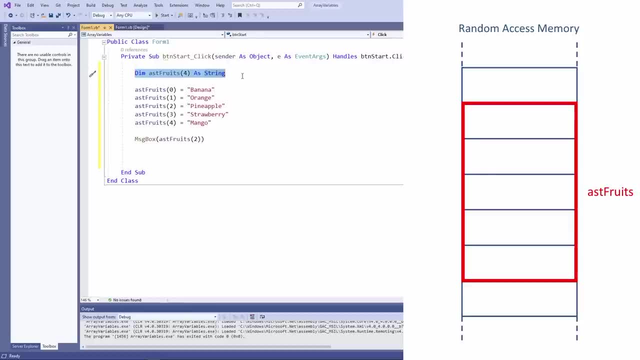 Contiguous means adjacent next to each other. The number 4 means that I want a group of 5 memory locations. It might strike you as odd, but in computer science we generally count from zero. We say that the array is zero-based. 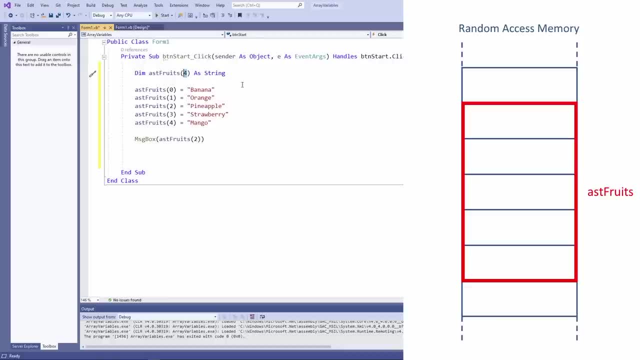 Each location in that group of memory locations is referred to as an element. So I have 5 elements numbered from 0 to 4.. When this line of code executes, I'm putting the text banana into element 0. This line of code puts orange into element 1, pineapple into element 2, strawberry into 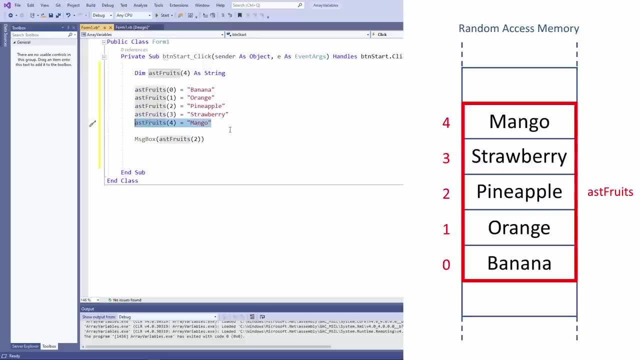 element 3.. And mango goes into element number 4.. I'm referring to each element by its index number. When I want to reference one of those data items again, I use the index number. So in this case I'm outputting the contents of AST fruits to element number 2, pineapple. 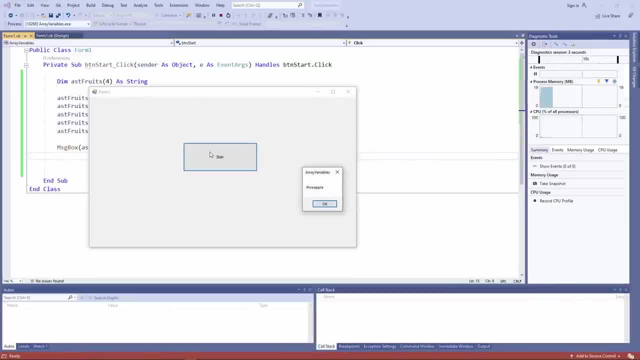 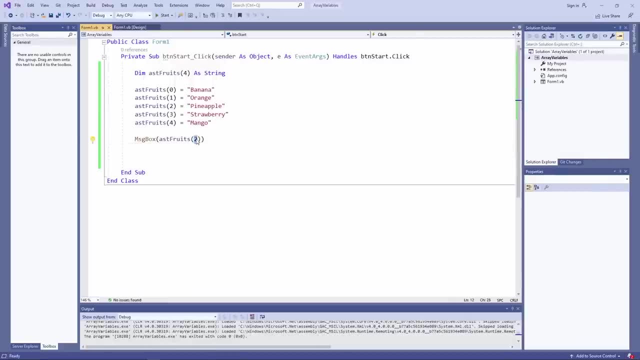 Let's give it a try. As expected, Let's output orange. I just have to change the 2 to a 1.. If I want to output mango, I'll type a 4 here. I can also reference an element of an array less directly. 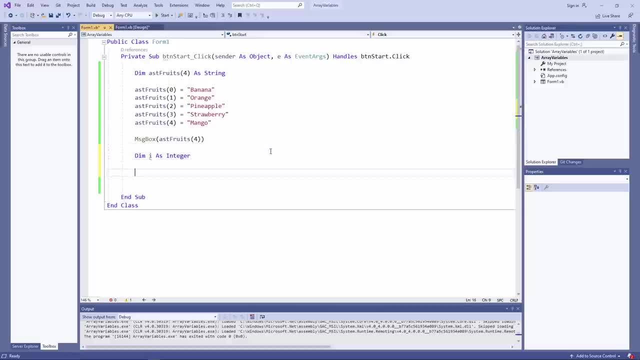 Let's declare an integer variable. I'm just giving it the name i. I'm going to assign a value to that variable. value to that variable. And now I'm going to use the contents of i to reference an element of the array. Can you see what the program will output this time? i is. 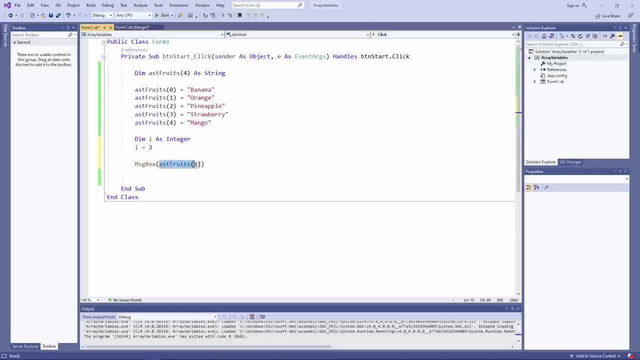 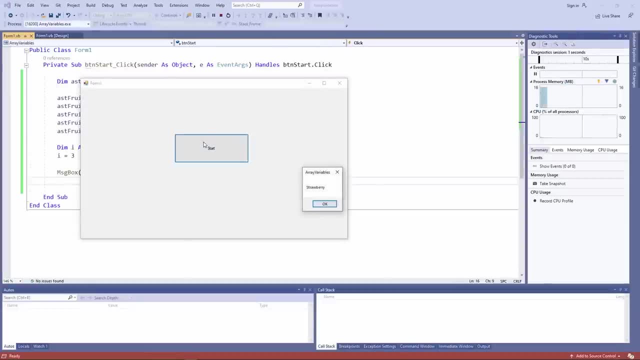 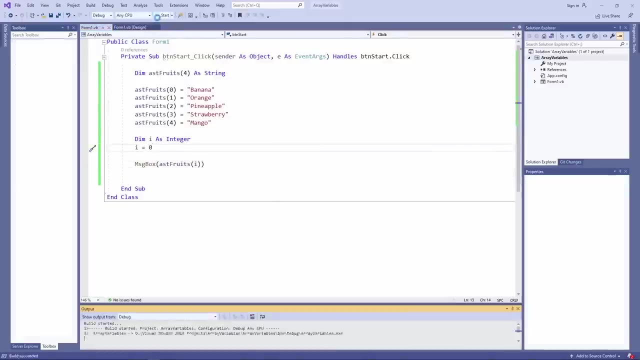 equal to 3, so this reads as AST: fruits 3.. It will output strawberry. Indeed, it does. Let's change the value of i to 0.. Now I'm outputting banana. Banana is the 0th element of the array. We can run into trouble, though. Watch this. I'm setting the value of i to. 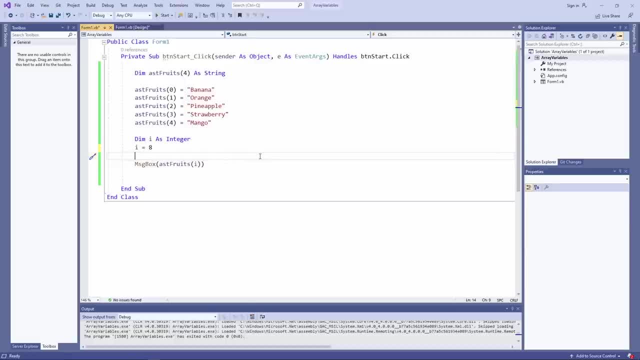 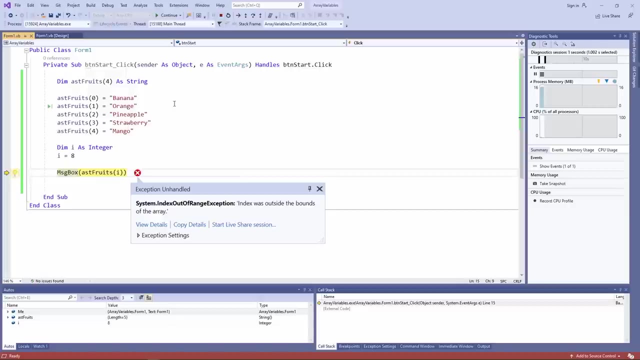 be equal to 8.. My array variable only has 5 elements numbered from 0 to 4.. There is no element number 8.. So what happens? What happens when I run the program now? Index out of range exception. My program has crashed. 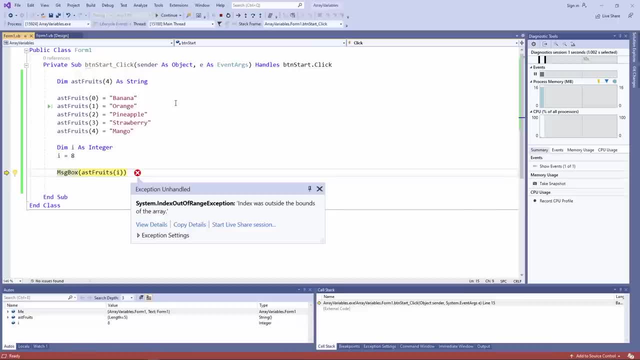 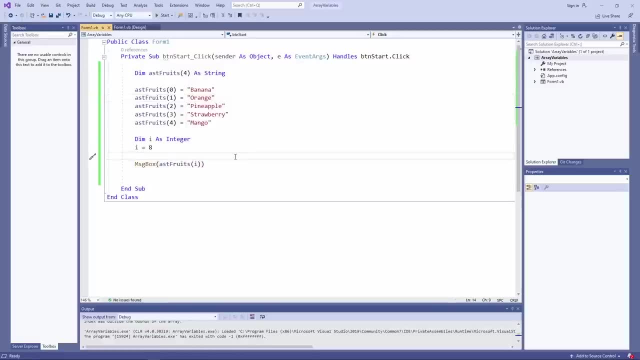 It's crashed because it can't find element number 8.. There's no such thing. Let's reset the program. Now. there's one more thing I would like to show you, which is where the real power of array variables comes in. I want to output. 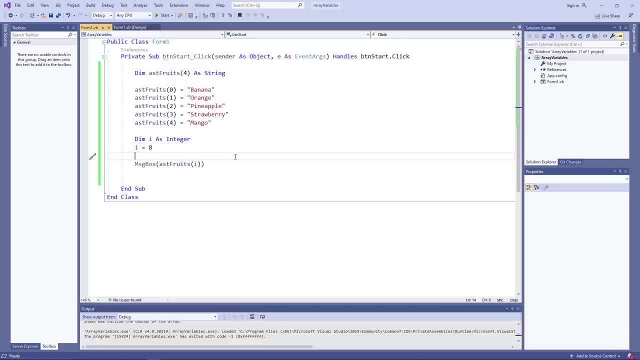 each of those items in turn. So I am going to iterate through the array using a for next loop. Watch this, For i equals 0 to 4. output AST fruits: i First time through the loop. i is equal to 0.. So 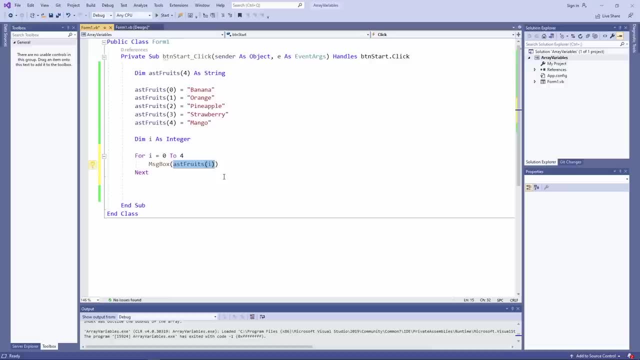 this will output Banana. Second time through the loop, i will be equal to 1.. So we output orange. Each item should be true either. In the same way, theensen'scot letters are interesting to see. I don't know if these are fair. I know winning this will lead me into some kind of. 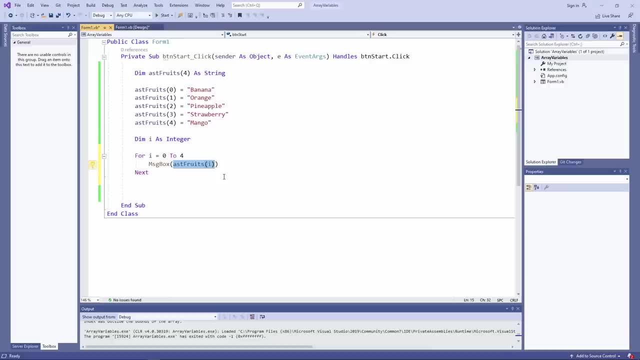 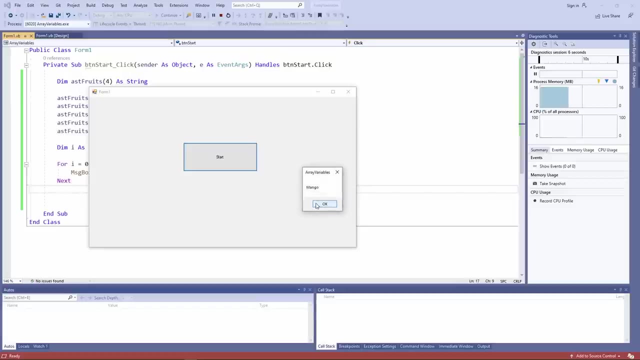 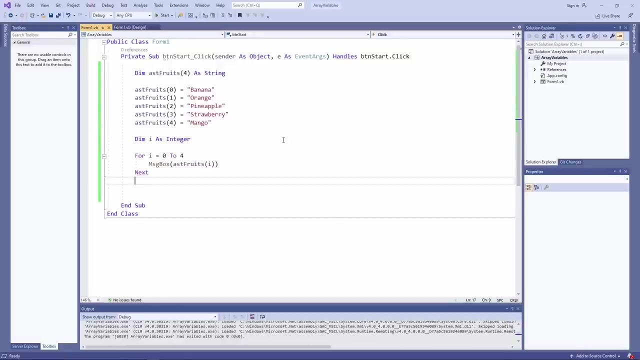 then I is incremented to two and we output pineapple and so on, until such time as I equals four. Let's give it a try And you can imagine: I can iterate through a hundred array elements just as easily as I can iterate through five. Give this a try yourself, Perhaps you can. 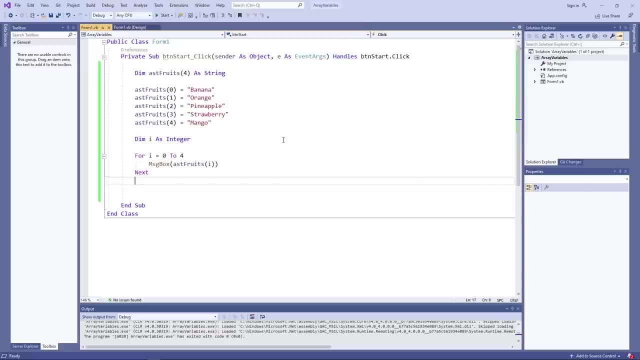 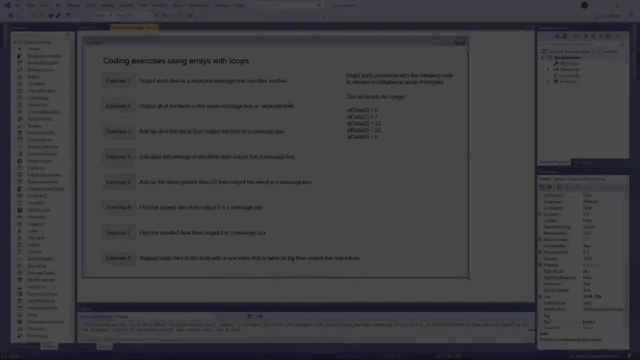 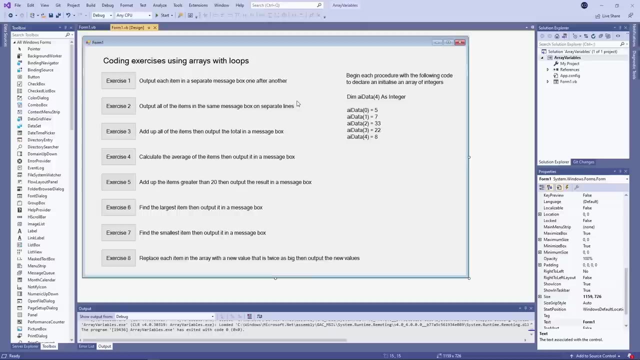 set up an array with ten elements instead of five. In this video, I'm going to invite you to practice what you've already learned. There are eight exercises here involving array variables and loops which you might like to try coding up yourself. I'll show you what they do and then it's up to you if you want to give them a go. 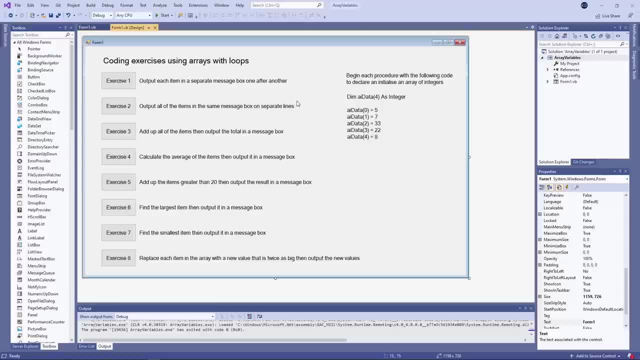 Alternatively, you can jump straight to my solutions later on in this video. By the way, all of these programs start with the same six lines of code. All of them declare an array variable of integers with five elements, and then the array is initialized as you can see here. But it's important to realize that your programs 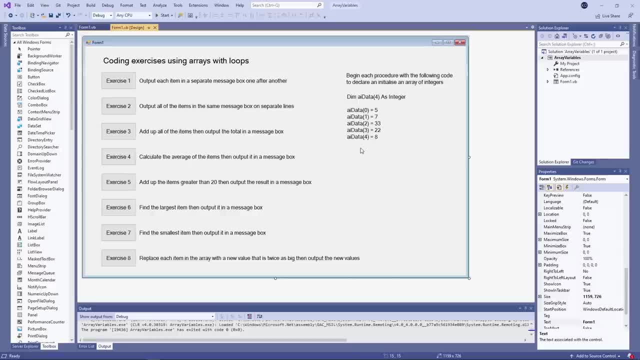 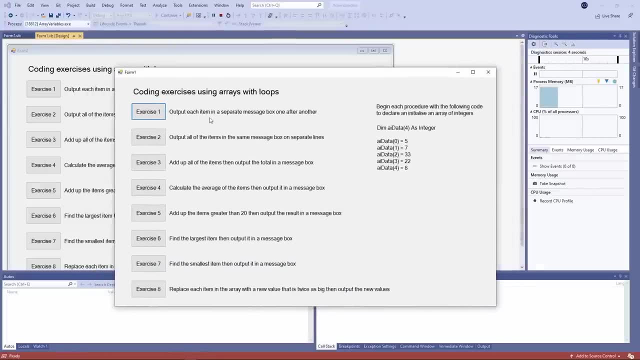 have to work with any data, Not just these. So let's see what they do. The first exercise is to output each item in a separate message box, one after another. Well, you've already seen how to do this in a previous video. I'm using a. 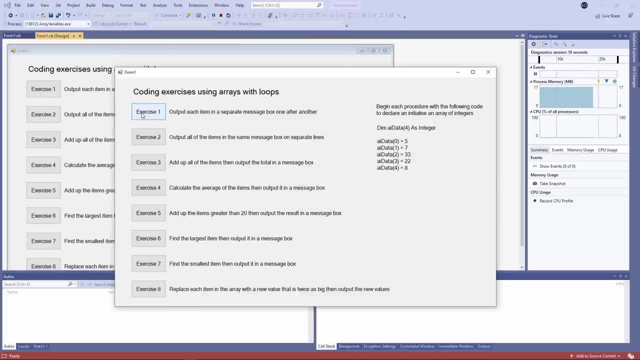 loop to scan through the array. Exercise two output all of the items in the same message box but on separate lines. Exercise three is to add up all of the items and output the total in a message box. They add up to 75.. In exercise four we calculate the average of the items. The 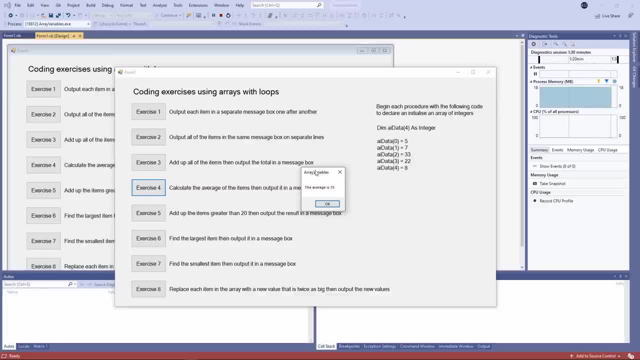 average value is 15.. Very similar to exercise three, except with dividing the total by the number of items. In exercise five, we are only adding up the items that are bigger than 20.. There are two items in the array which are bigger than 20,, namely 33 and 22.. And 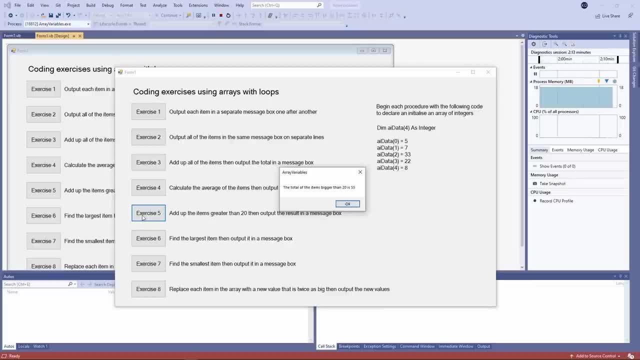 they add up to 55.. We're still doing this with a loop, but as we visit each item, we're deciding whether it's bigger than 20 or not. In exercise 6, this is a little bit trickier. you have to find the largest item and output it. 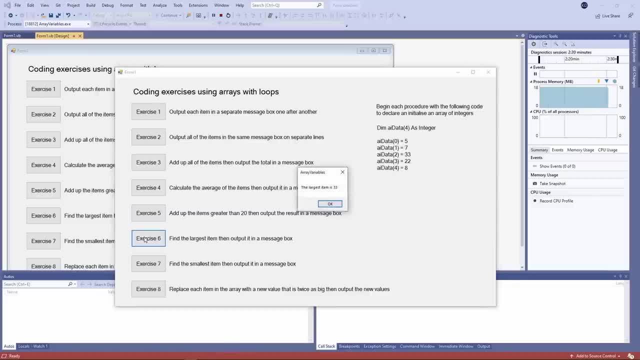 in a message box. the biggest item is 33 and let's be clear, the program is working out which is the biggest item. if you can do exercise 6, you'll find exercise 7 very easy. exercise 7 is finding the smallest item and exercise 8 is replacing each item in the array with a new value that is twice as big. 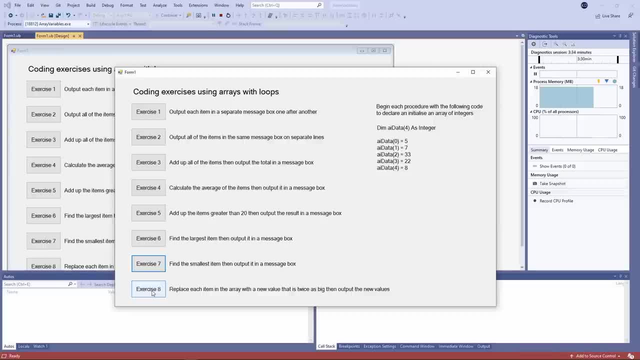 and then we output those values in pretty much the same way as we did in exercise 2. so if you want to give them a try yourself, pause the video now and see what you can come up with. alternatively, you can jump straight to the solutions. so let's take a look at my solutions. the 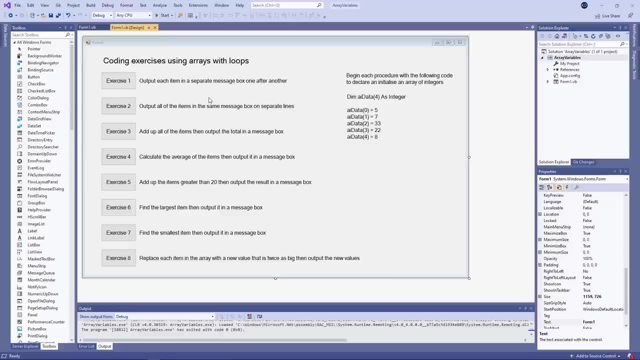 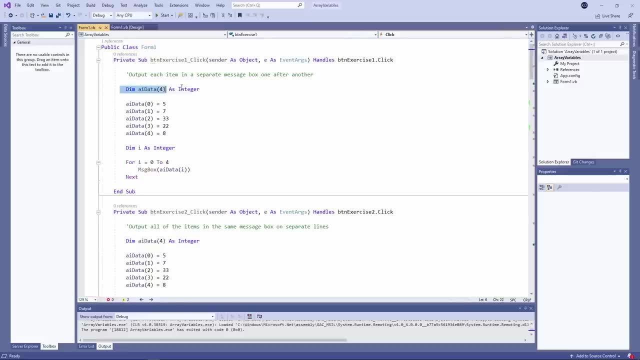 obvious answer is yes, and the obvious answer is no and the obvious answer is no. objective of exercise 1 was to output each item in a separate message box, one after another. you've seen how to do this in a previous video. I start by declaring an array of five integers and then I initialize the array in order to 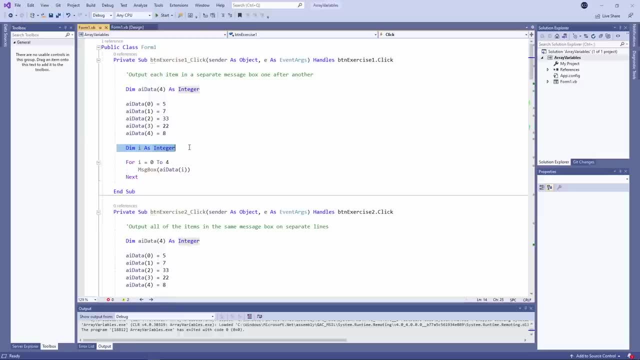 scan the array. I need a loop counter. so I've declared an integer variable called I and that controls the number of passes through the for loop. then I say: for I equals naught to four, output AI data element number I. so first time through the loop, I is zero. that 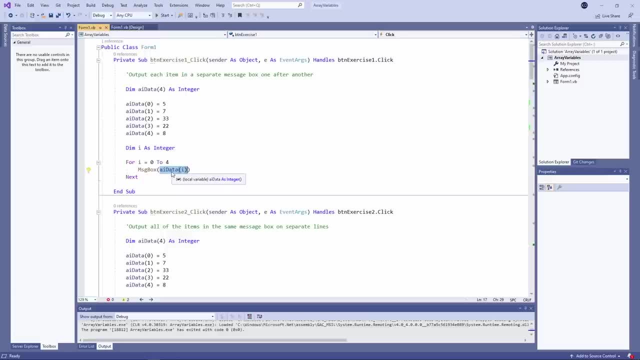 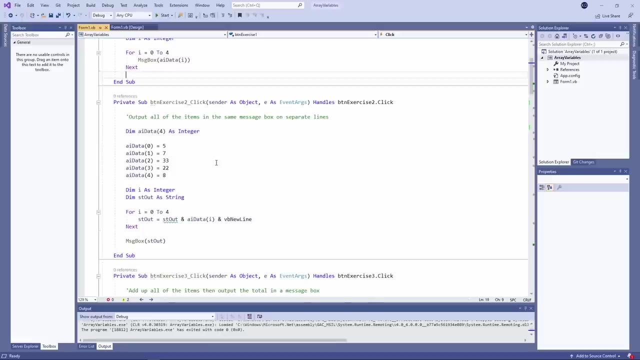 outputs the first item. second time I is 1, I output the second item, and so on. until I is equal to 4, we output the last item and we drop out of the loop. in exercise 2, we want to output all of the items in the same message box. 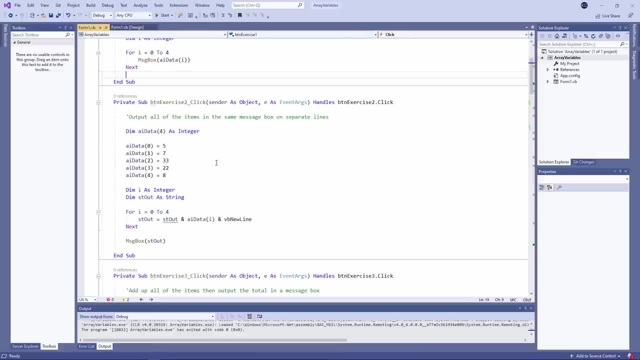 so we don't have an output command within the loop. we're simply building a string. I've declared a string variable called st out, and inside the loop I say: st out equals whatever it used to be, plus the next item in the array. I'm also concatenating a new line operator on there as well, so the string actually. 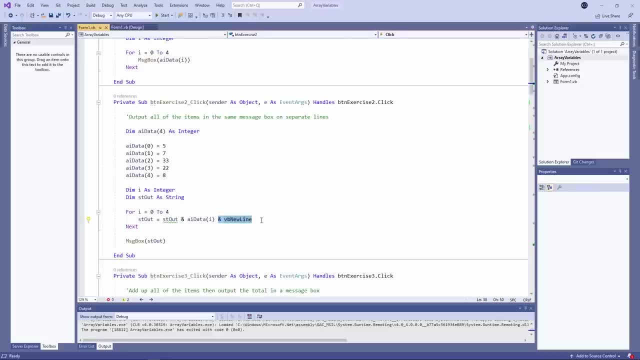 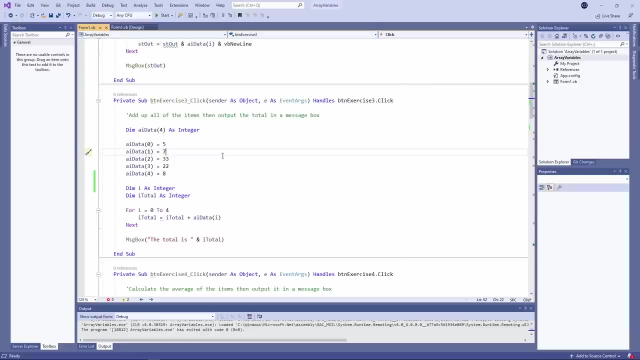 contains the information needed to throw a new line between each item. when we drop out of the loop, we display the output string in one go. The solution to exercise 3 is similar to the solution to exercise 2.. We want to calculate the total of the data items, so I've declared a variable called 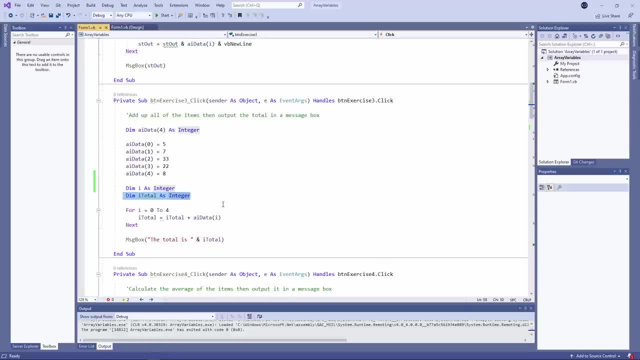 itotal to contain this, and then, as we visit each item in the loop, I say: itotal equals whatever it used to be, plus the next item. I'm using the addition operator instead of the concatenation operator. this time, When we drop out of the loop, I display the total in one message. 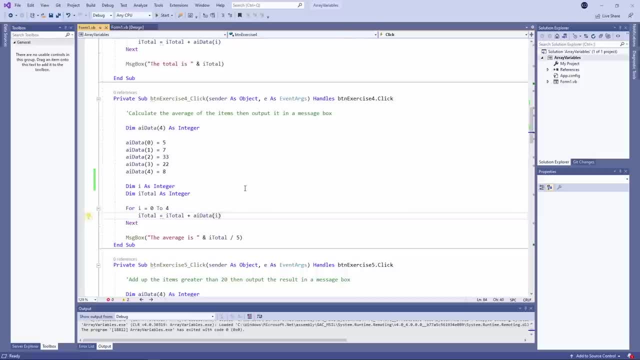 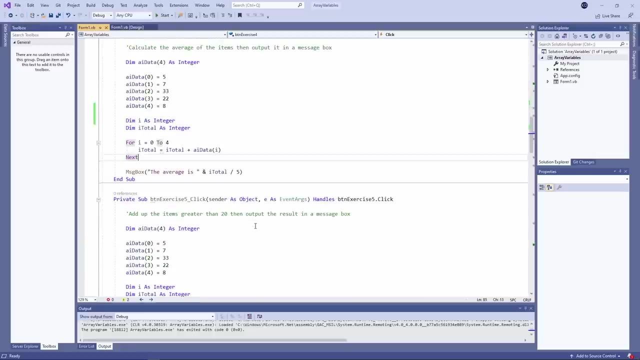 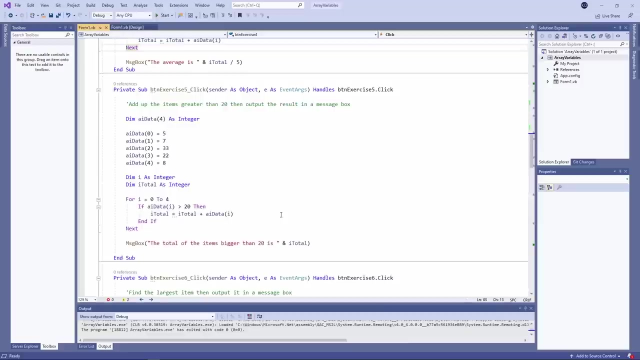 The objective of exercise 4 was to calculate the average. Well, this is pretty much the same as the previous exercise. I calculate the total first And then, when I display the message, I simply divide the total by 5.. With exercise 5, the objective was to add up all of the items bigger than 20.. 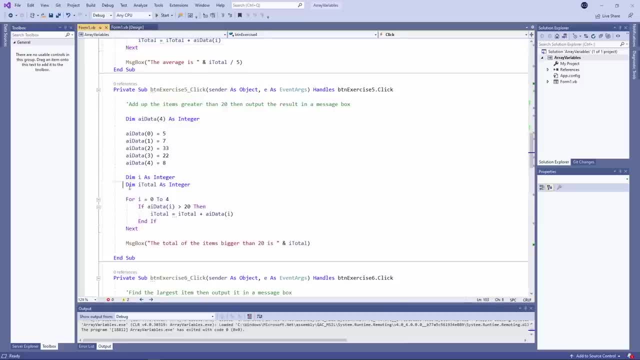 So in some ways it's similar to the previous program. I've declared a variable to hold the total, But look what's going on inside the for loop. I'm adding the next value to the total conditionally. OK, I'm testing each value first to see if it's bigger than 20.. 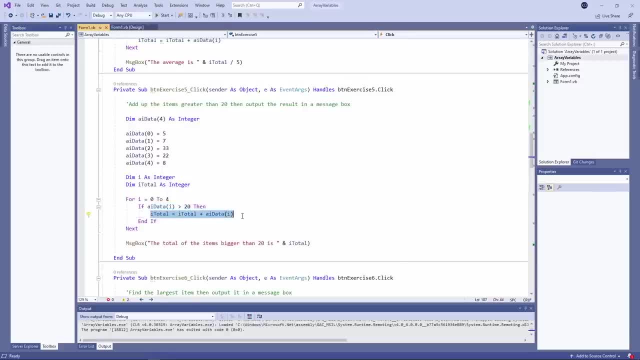 And if it is, I add it to the total. If it isn't, well, I don't. If you think about it, adding up all of the items which are, let's say, smaller than 20 would require a very simple change. 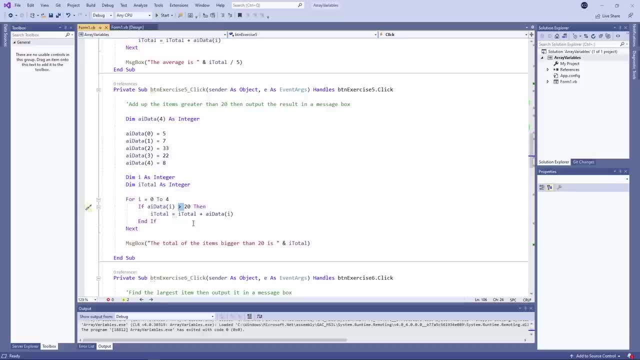 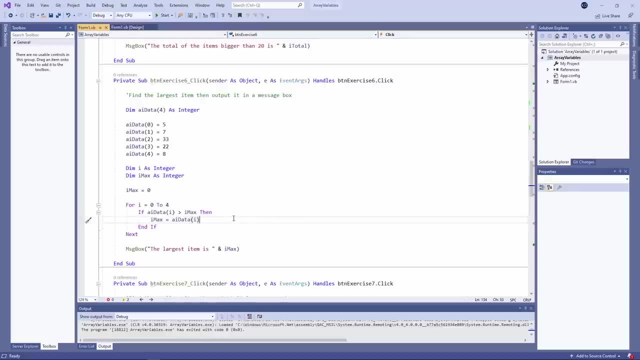 All I'd need to do is change this relational operator to a less than sign. In exercise 6, you were invited to write a program to find the largest value. In exercise 7, you were invited to write a program to find the largest item in the array. 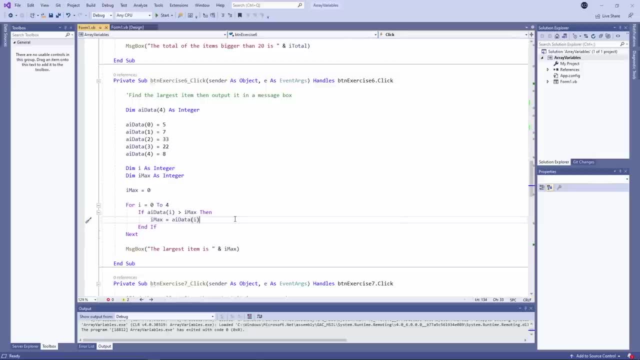 The principle behind this program is to visit each item in the array and if it's bigger than the previous item, then keep a record of it. So I've declared a variable called imax, which will hold the maximum value, And I've initialized it to 0, which pretty much guarantees that everything is going to. 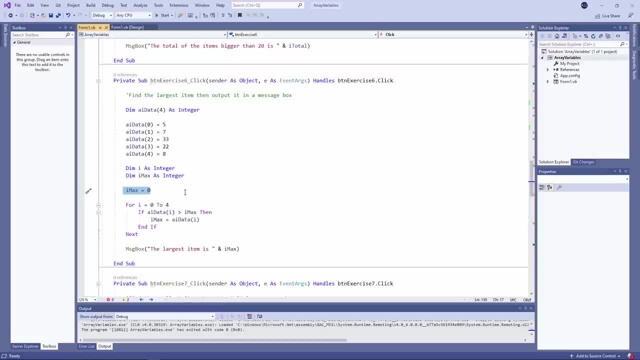 be bigger than imax. to begin with, Assuming I'm only working with positive numbers, OK, OK, OK. So I've got an item inside my loop. I ask: is it bigger than imax? Well, of course, item 0, the number 5 is bigger than imax. it's bigger than 0. 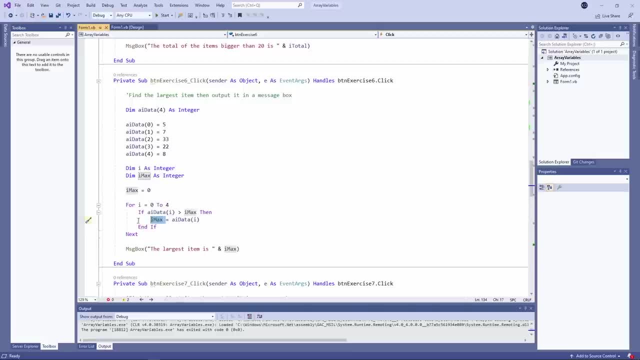 So I'm assigning the first item to imax, overwriting its previous value. Imax now contains a 5.. 5, is the biggest item we found so far. Second time through the loop, I examine the second item and I ask: is it bigger than imax? 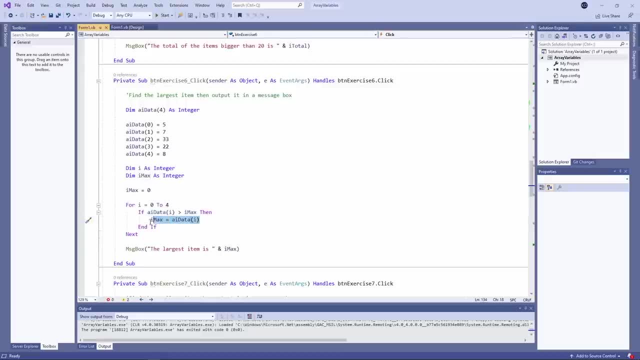 In this case. well, 7 is bigger than 5, so I replace 5 with 7.. I'm keeping track of the biggest item. Third time through the loop, same question, and I replace 7 with 33.. But fourth time through the loop, I find that 22 is not bigger than 33, so this line of code doesn't execute. 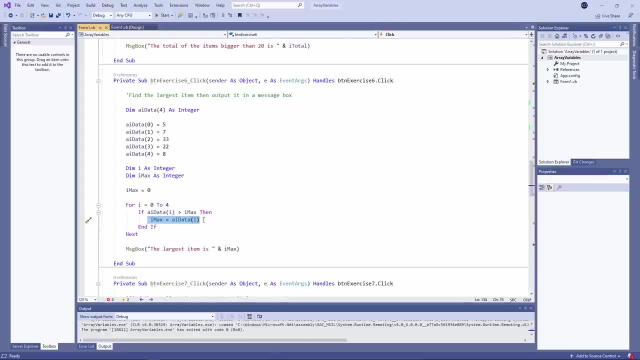 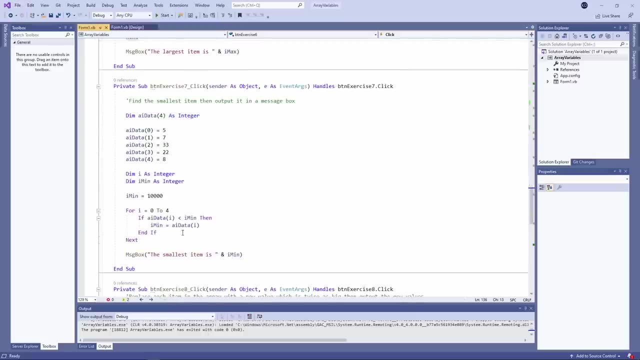 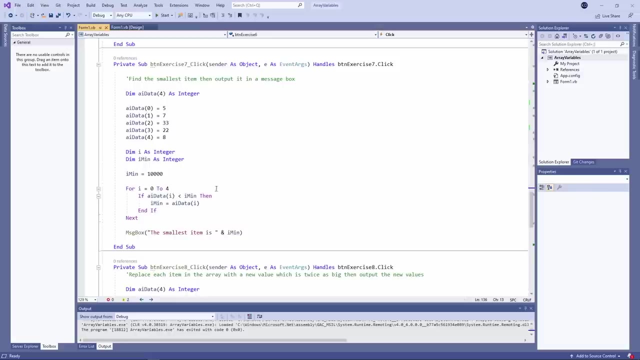 By the time the program's finished, Imax contains the biggest value. If you can solve exercise 6, then you can solve exercise 7 very, very easily. This time I have a variable called imin, which is going to hold the minimum value. 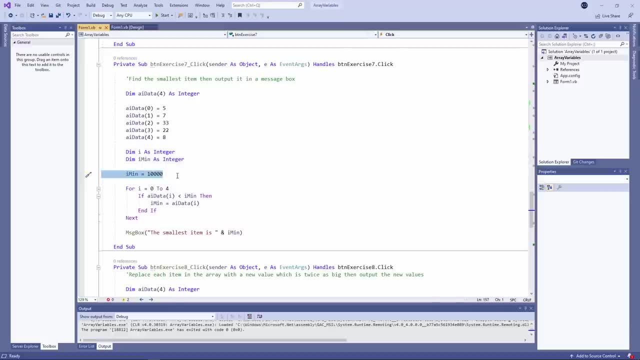 And I'm initializing it with a very large value, something that I know is bigger than anything else in the array. I've made it 10,000.. When I visit the first item, I ask: is it smaller than imin? Well, of course it is. 5 is smaller than 10,000.. 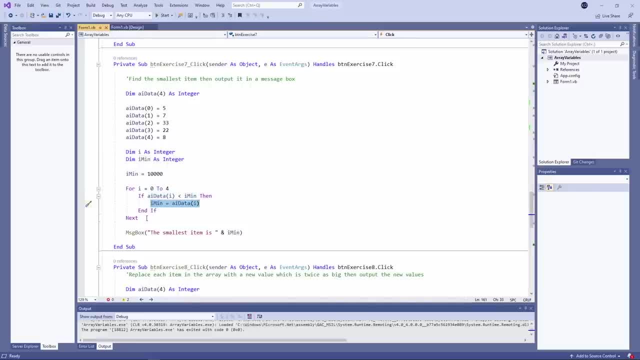 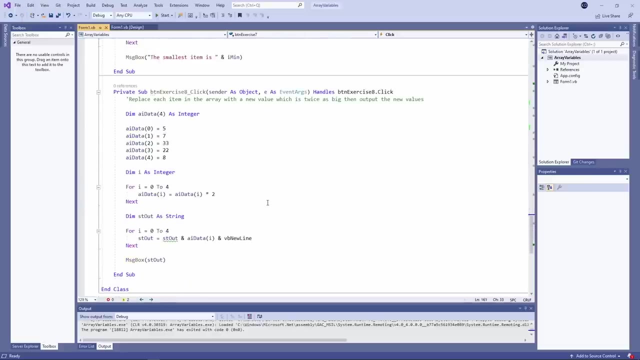 So imin becomes the first value, And then we proceed pretty much as we did in the previous program. By the time we drop out of the loop we have the smallest value. The objective of exercise 8 was to replace imin, So I'm going to replace each item in the array with a new value twice as big. 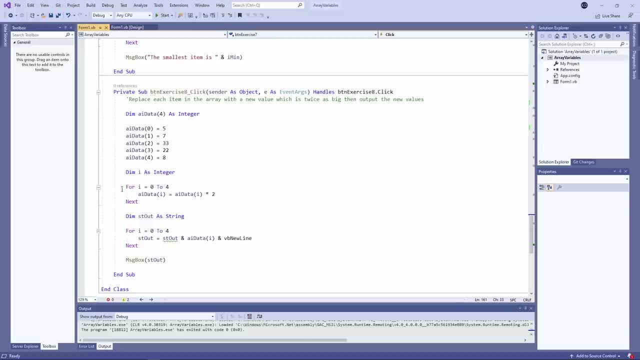 I actually want to change the contents of the array, And that's what this loop does. It's actually very simple. I say: let aiData- the item I'm looking at- be equal to itself multiplied by 2.. So by the time we drop out of this loop, the array contains a completely different set of data. 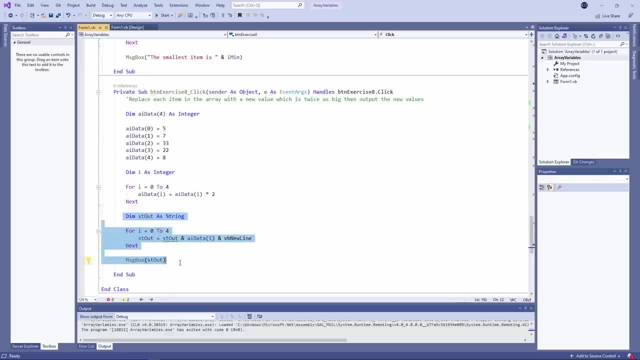 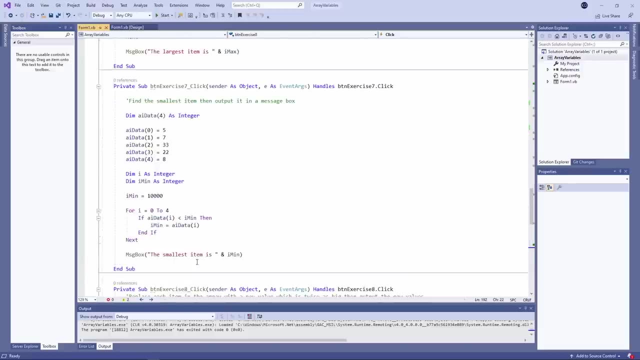 And then the remaining code simply outputs those data In a single message box, just like in exercise 2.. Now, even if you didn't solve these problems yourself, it's well worth trying to duplicate the code that you can see here. It will definitely help you get a feel for using array variables with loops. 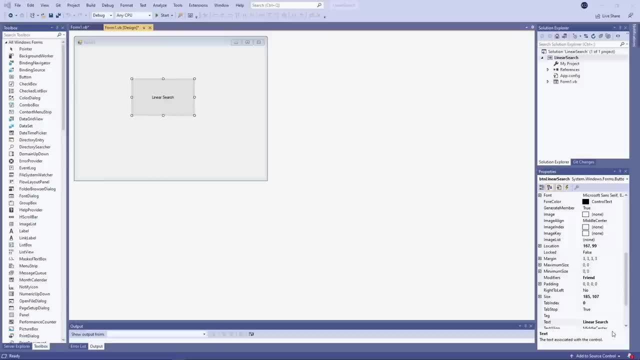 In this video, I'm going to show you how to implement a linear search. A linear search is one of many standard algorithms that you'll come across as a programmer. The principle of a linear search is to examine a list of items one at a time. 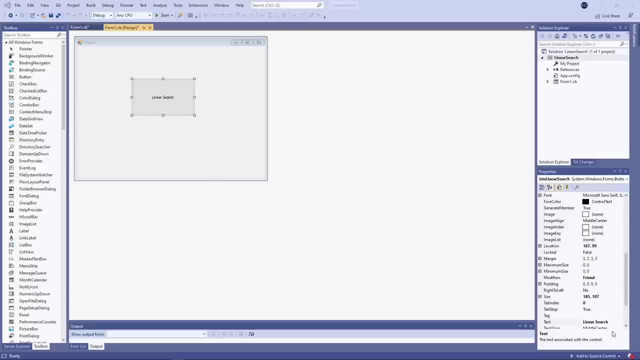 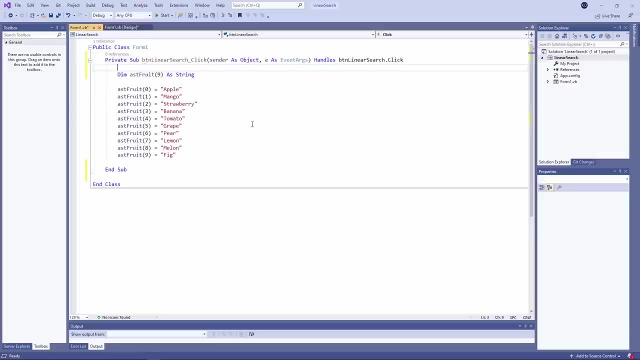 to see if it contains an item that we're looking for. I've already declared an array of 10 strings And you can see I've initialized it with various items of fruit. By the way, you can see that the program contains the data that we're going to search. 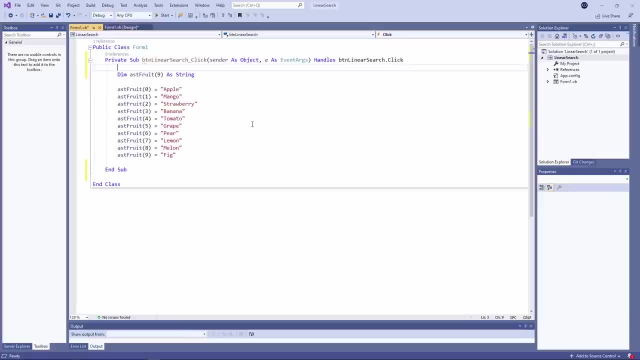 We say that the data has been hard-coded into the program. This is untypical. In reality, a program wouldn't normally have the data written into it like this. You'll see in later videos that a program can actually read the data in from an external file. 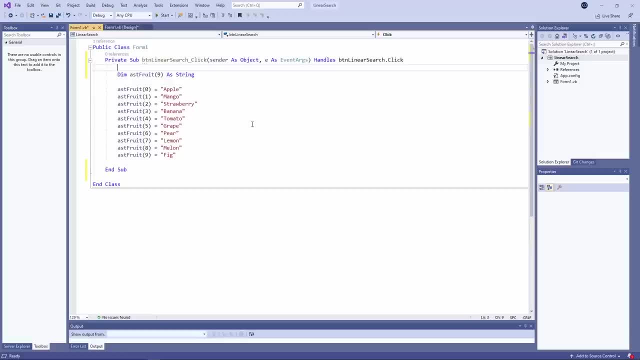 Perhaps a database or a text file or a spreadsheet or even a web page. You'll also see how one program can call another and pass it some data to work with For the purposes of demonstrating a linear search. hard-coding the data like this is absolutely fine. 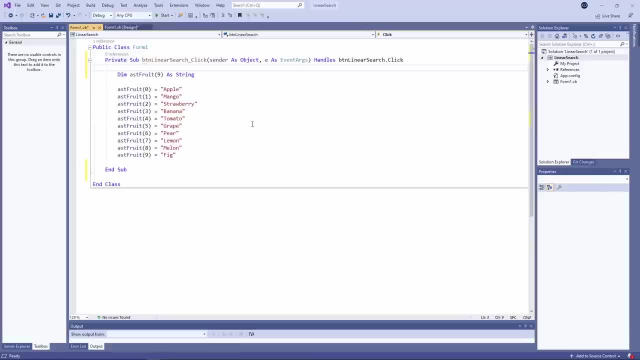 We'll start by prompting the user for an item to search for. We'll call it the target value. So I've declared a variable to store it And, to keep things simple, I'll use an input box to prompt the user. Now I'm going to use a loop. 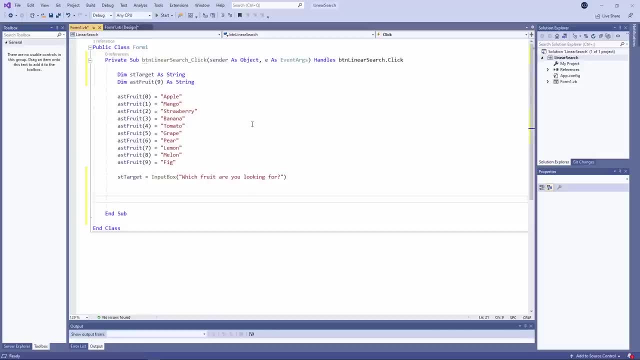 to scan through the array, to visit each item one at a time. I'll need a loop counter And I'm going to use a for loop. I could use a do loop, It's a matter of preference. A for loop will mean I can write slightly less code. 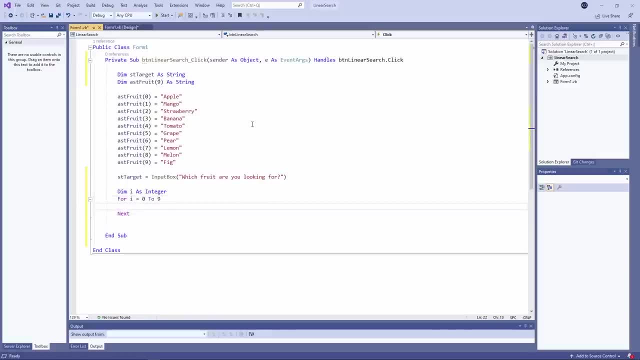 As I visit each item, I'm going to check to see if it's the target value. I can do this with an if statement. Now, this isn't the finished product, but it's well on the way. Let's see what happens. 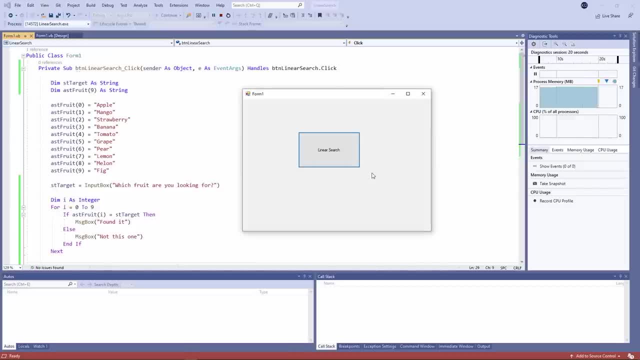 I'm getting a message for every item which is not the one I'm searching for, But I did get a message saying it found it. Let's try it again. I'm looking for a starfruit. this time. There is no starfruit in the list. 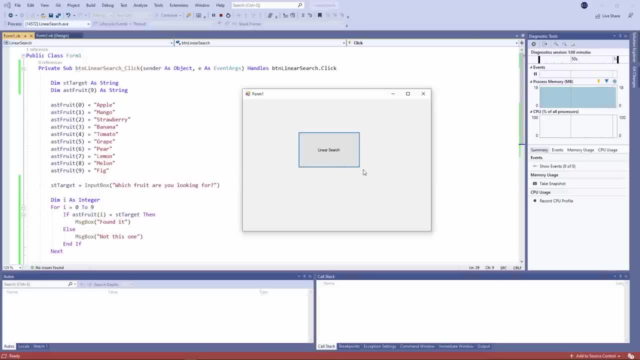 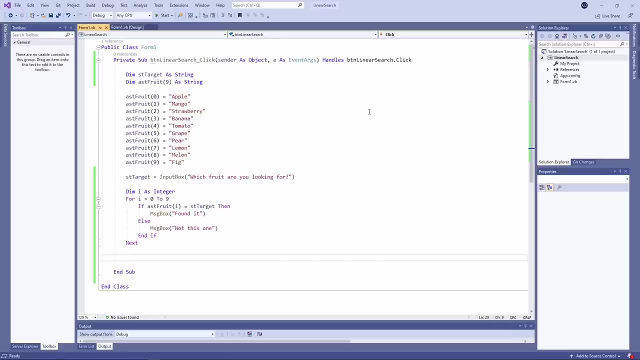 Well, it's on the way, but I don't want a message for every item which isn't the one I'm looking for, So let's improve it. Rather than doing some output inside the loop, I'm simply going to keep a record. 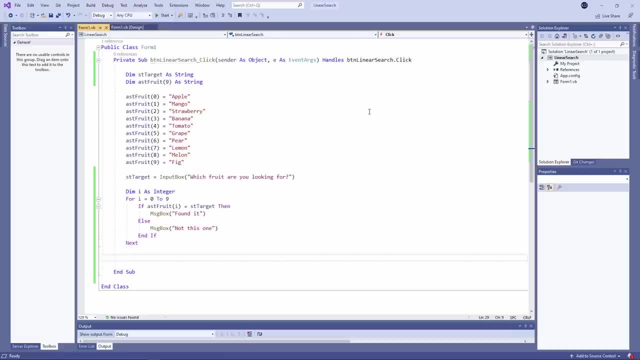 of whether or not I found it, And to do this, I'm going to use a Boolean variable. A Boolean variable can have one of two possible values: true or false. Immediately after it's been declared, it'll have a value of false. 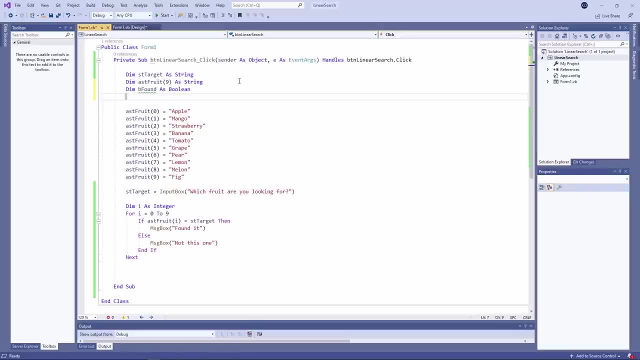 So, inside the loop, if I find what I'm looking for, I'm going to set be found to be equal to true And I don't need an else clause because if we don't find what we're looking for, be found will never get set to true. 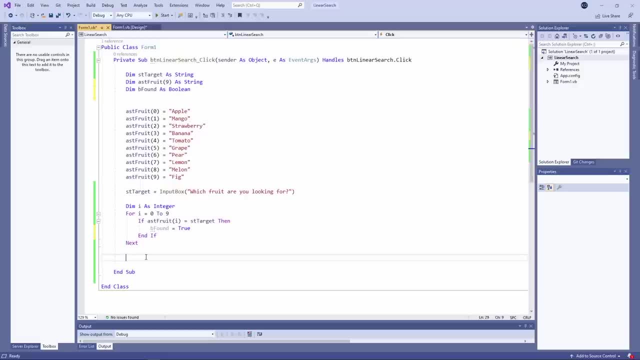 And when we exit the loop, be found will still be false. All that remains to be done now is to test be found once we get out of the loop, to see if it's equal to true. Let's see what happens. We'll start by looking for something. 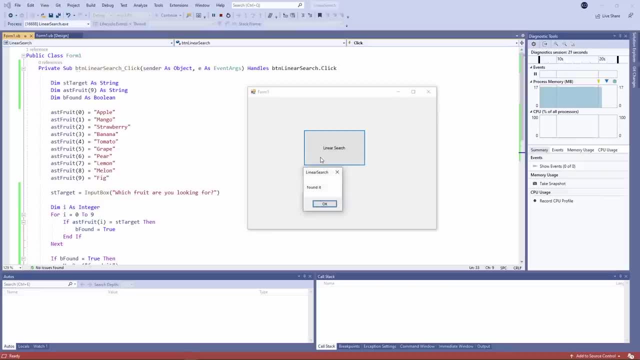 that we know is in the list. Found it, Just one message. Let's try again. We'll search for something else that we know is in the list. Yes, there's a fig. What about something that isn't in the list? 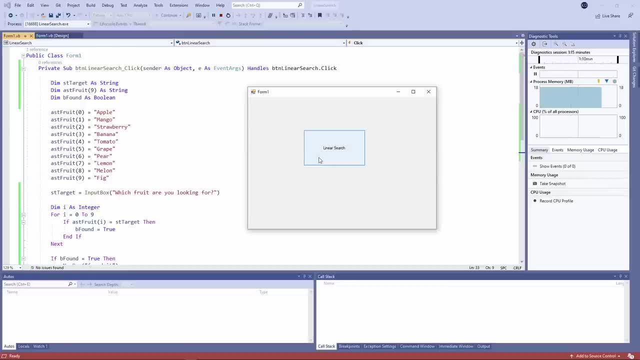 Not found. Now just a couple of words of warning. When you're comparing strings in VBNET, string comparisons are case sensitive. So, for example, if I search for banana with a small b, not found, However, banana with a large b. 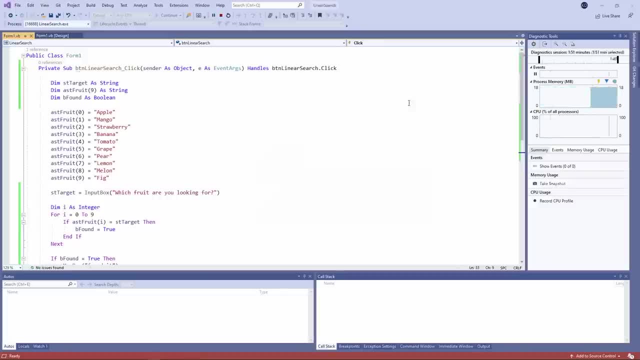 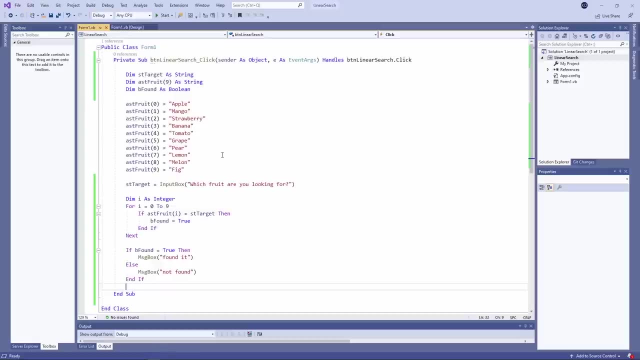 is found. You've seen something similar to this in an earlier video. I can remove the case sensitivity of a string comparison like this, So I'm comparing the uppercase version of the target with the uppercase version of the array item. I can achieve exactly the same effect like this. 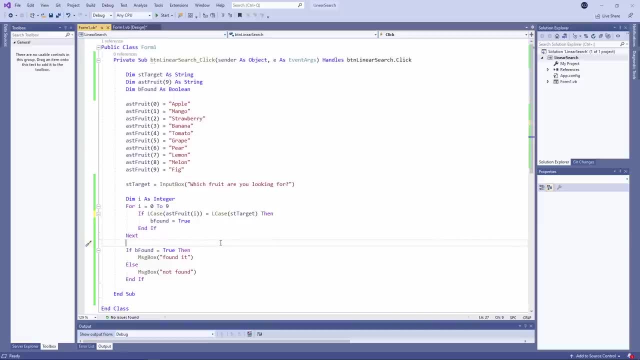 Lcase means lowercase, So I'm comparing the lowercase version of the target with the lowercase version of the item in the array, And it's probably worth mentioning this as well. I can use dot to upper instead of ucase. Now there's one more improvement I can make. 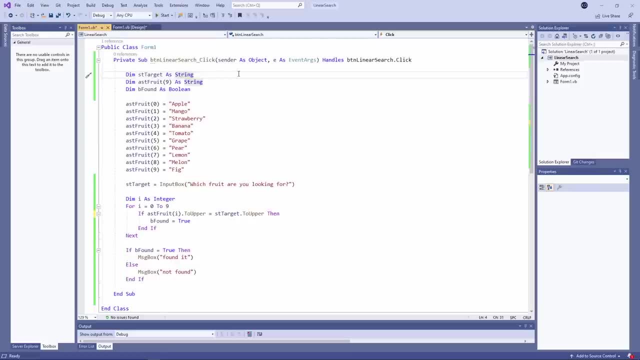 to the efficiency of my program. If I find what I'm looking for, there's no point in examining all of the other items in the array. If bfound gets set to true, then we can force an exit from the for loop, For example, if we're searching for 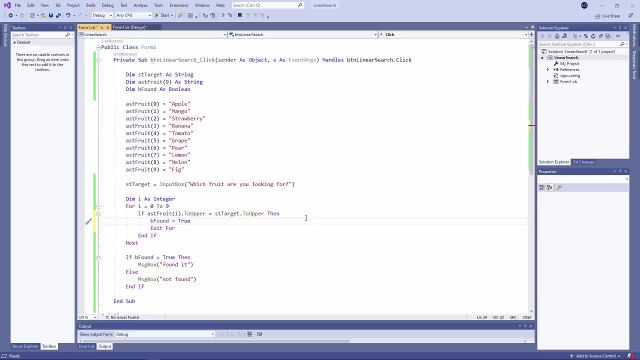 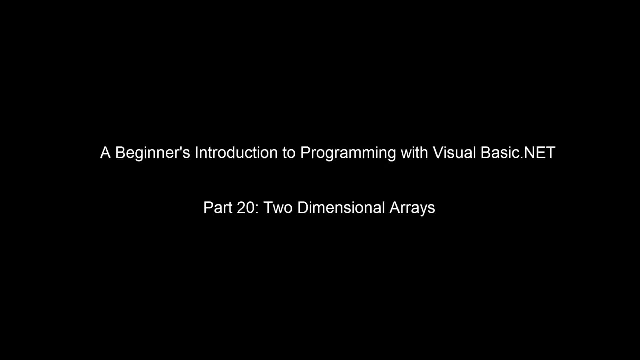 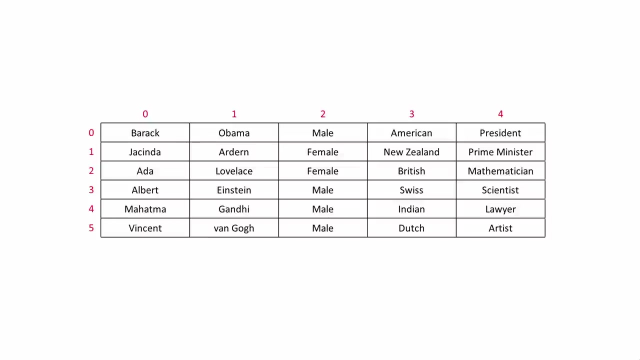 apple and we set bfound to true. there's no point in looking at all of the other items in the array. We already know it's there. So there you have it: A standard linear search If you're going to write code. 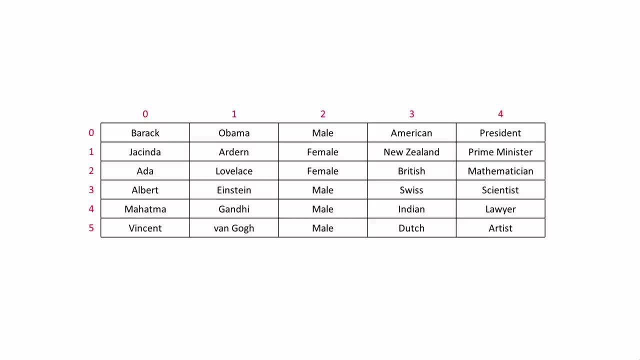 to create and manipulate a two-dimensional array variable, it's essential that you can visualize the data you're working with. Very often, a two-dimensional array variable is used to store groups of related data items, like the data you can see here. A two-dimensional array can therefore. 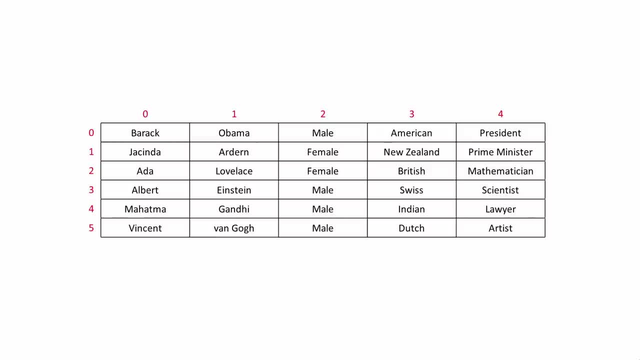 be thought of as a table. These are the data we're going to use in this video. Each row of the table contains the details of a different famous person. The first column contains their first names. the second contains their last names. the third column is gender. 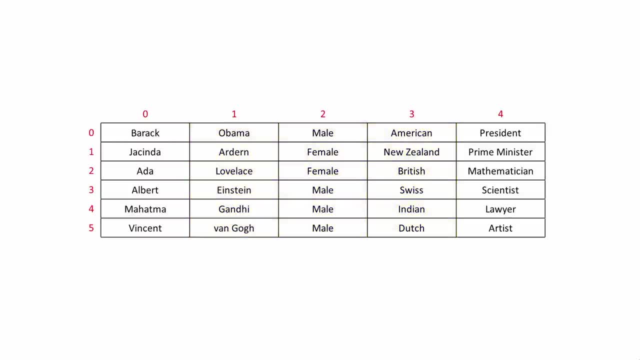 then we have nationalities and finally their occupations, what it is each person is famous for. Notice that each column has an index number. Counting starts from zero. so the fifth column is column number four. Each row also has an index number. 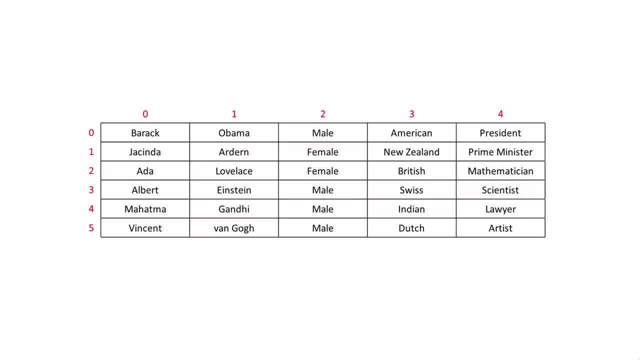 and these are also numbered. for the same reason, They are also numbered from zero. It's useful to think of this table as having a horizontal dimension, which we'll refer to as the X dimension, and a vertical dimension, which we'll refer to as Y. 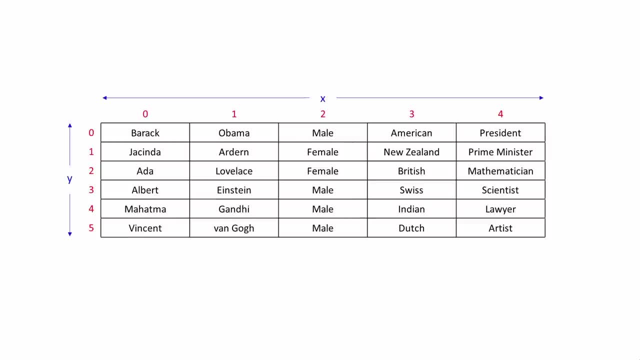 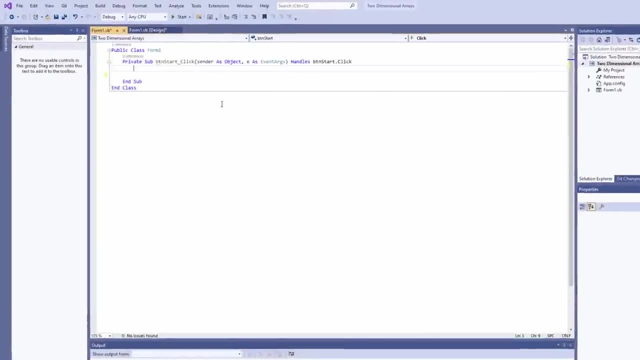 just like the X and Y axes of a line chart. When you're coding up a two-dimensional array for a different set of data, I strongly recommend that you keep a sketch of it handy, like I'm going to do now. I can declare my two-dimensional array variable like this: 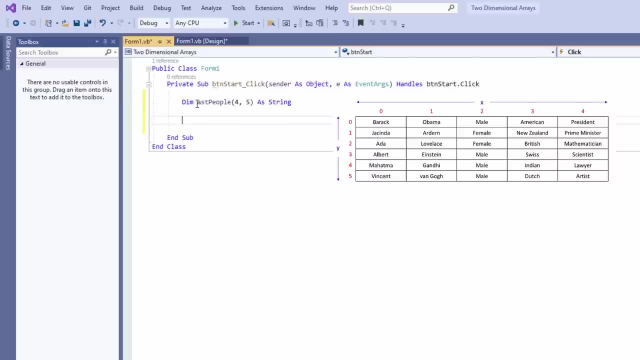 I'm using a naming convention here: A because it's an array variable, ST because it's an array of strings, and people because that's what the data is. In brackets, I've specified the X dimension first, followed by a comma. 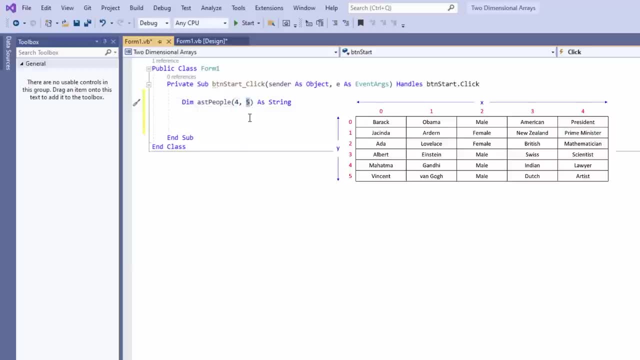 and then the Y dimension, And I've used the AS clause to specify that this is an array of strings. Now I'm keeping my sketch of the data handy while I populate this array. It's important to get this right, otherwise you might get some very peculiar behaviour. 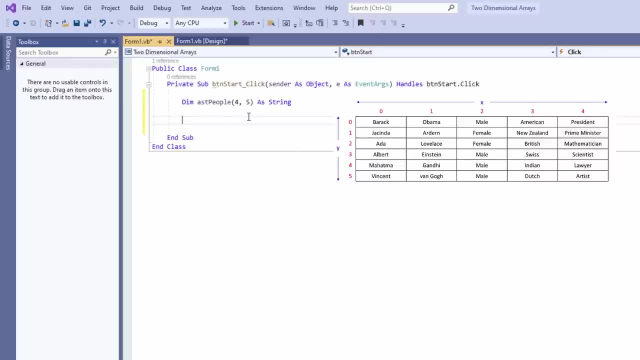 when you run your program. I want to put Barrack in the first column and the first row. I want Obama in the second column and the first row. The third column, first row, contains male, And column number three, row number zero, contains American. 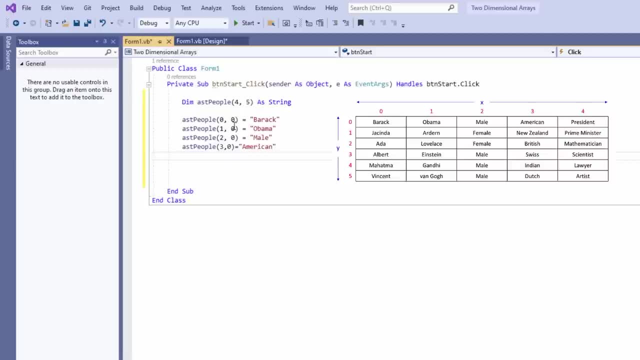 It takes a little bit of getting used to counting from zero, And the final piece of data for this person is President. Now it's tempting to start copying and pasting, but I want to make sure I get this absolutely right, So I'm going to continue entering the values individually. 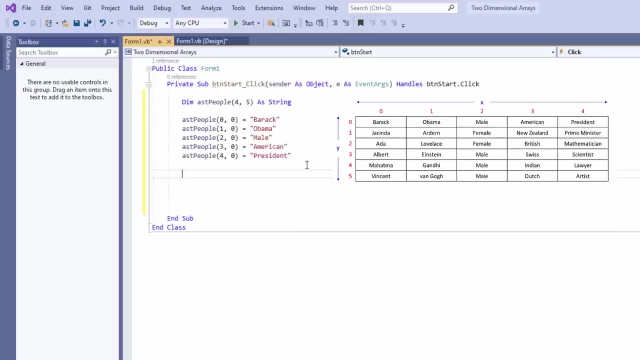 just for now, working from my sketch, Let's get the New Zealand Prime Minister in next. As with the previous famous person, I've specified the column number first, followed by the row number. I've specified x, followed by y. Notice that the value of x is different for each data item. 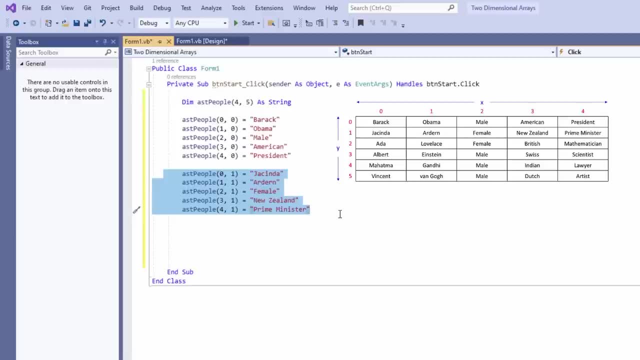 but the value of y is always the same because y is the row number. Let's do one more very carefully, and then I'll speed things up with a bit of copying and pasting, And I've just realised that I've made a mistake. 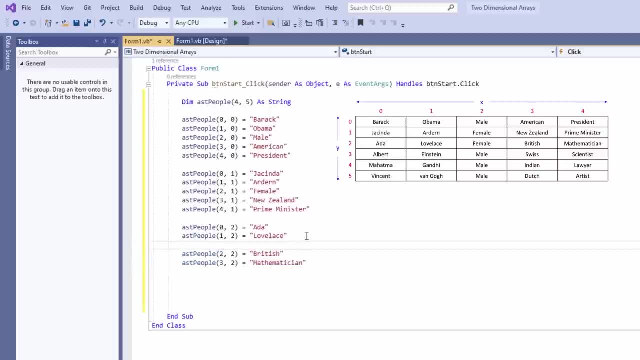 It's very easy to do. That's more like it Now. you could initialise each individual element of this array in any order you like, the important thing being that it's fully initialised. But taking a systematic approach like this will help to ensure, if not guarantee, 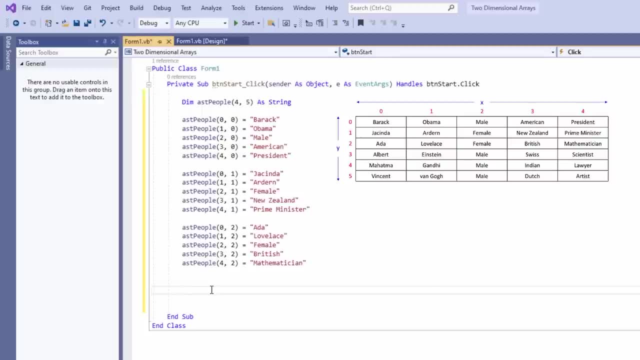 you won't make any silly mistakes. A systematic approach will also help to ensure that all of the data gets in there, But I can see a pattern emerging now, so I'm going to start copying and pasting to speed things up a little bit. 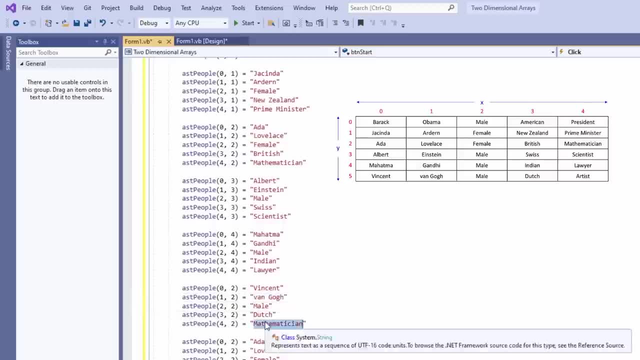 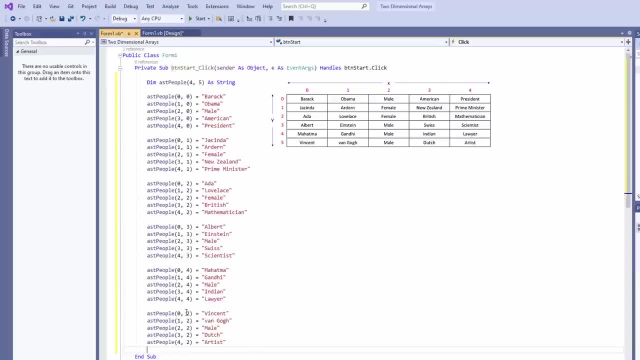 Now one last look at my sketch just to make sure I've got everything there that should be there And straight away. I can see I need to change these 2s to 5s, And there it is, The code I need to declare and populate my two-dimensional array. 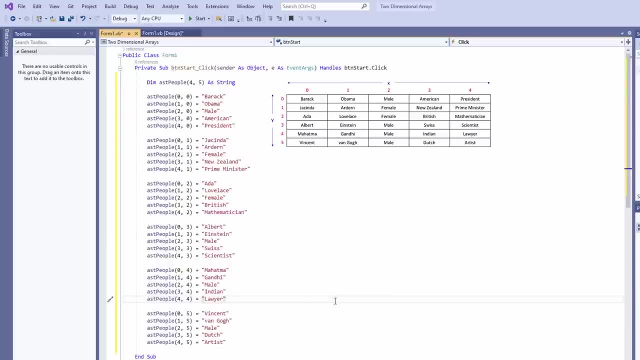 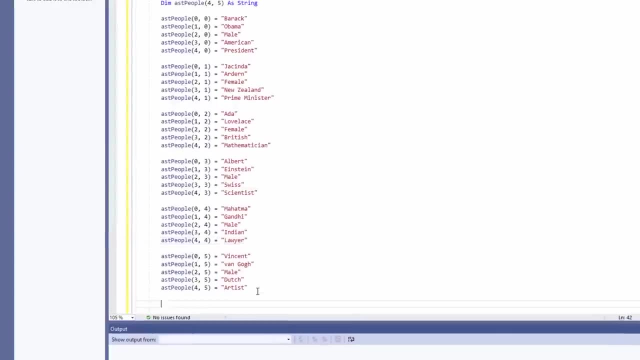 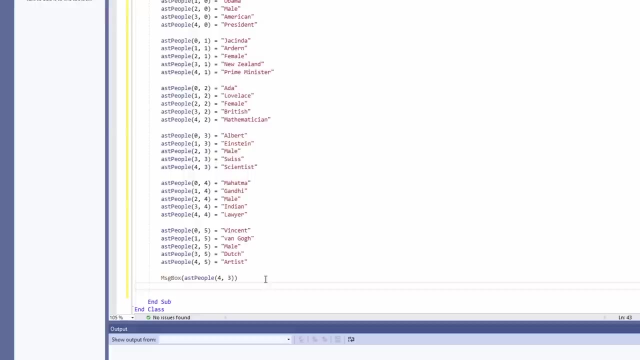 So that's how we get data in. How do we get data out? It's actually very simple. If you've ever played a game like Battleships, With this message box statement, I'm going to output whatever is in column 4, row 3.. 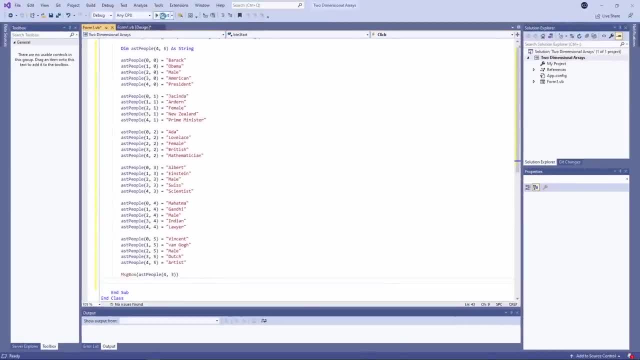 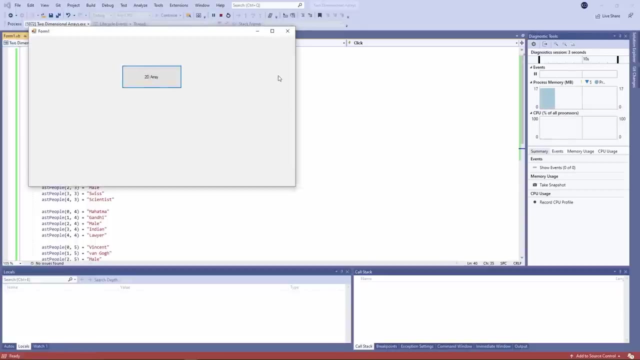 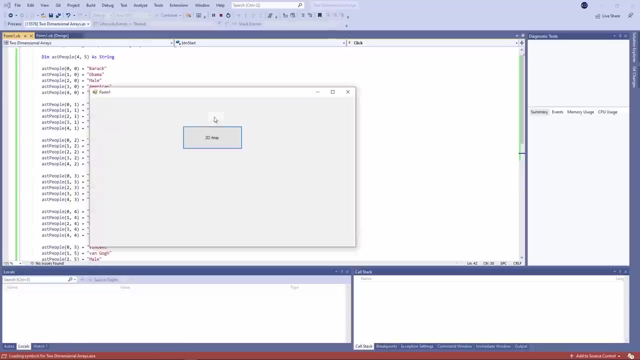 In this case the word scientist. What if I want to output, let's say New Zealand? That's in column 3, row 1.. Or perhaps the word Swiss? That's row 3,, column 3.. It's just a matter of supplying the appropriate coordinates. 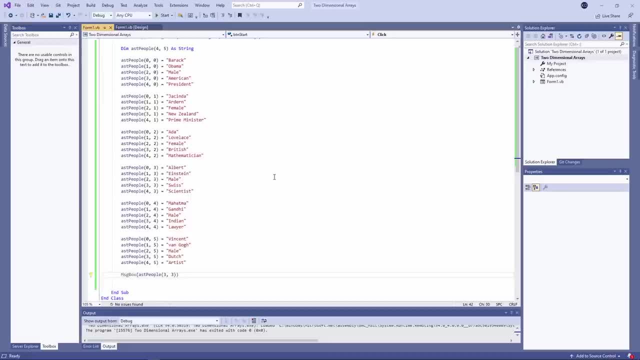 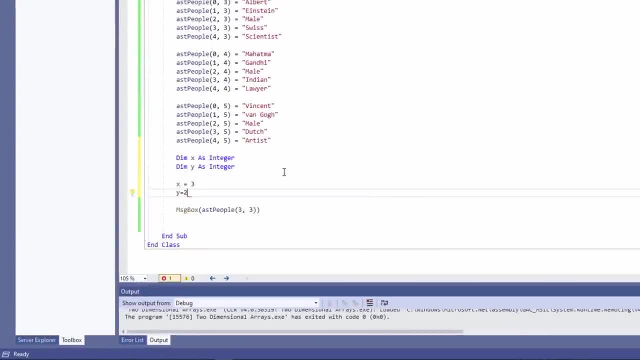 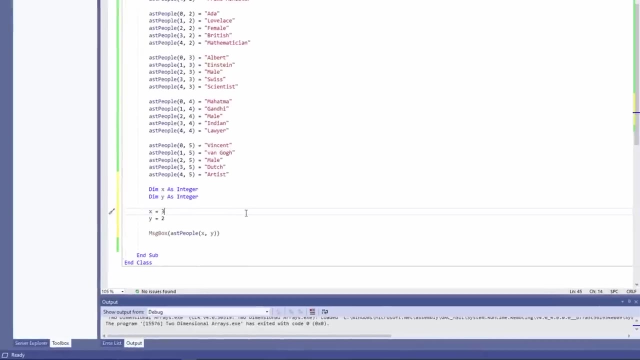 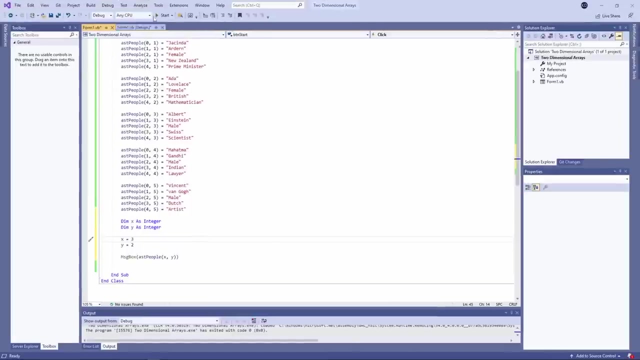 I can also supply these coordinates using variables. Now I could call these variables anything I like, but it makes perfect sense to call them x and y. Can you see which data item will be output by this message box? Let's see Now just like a one-dimensional array. 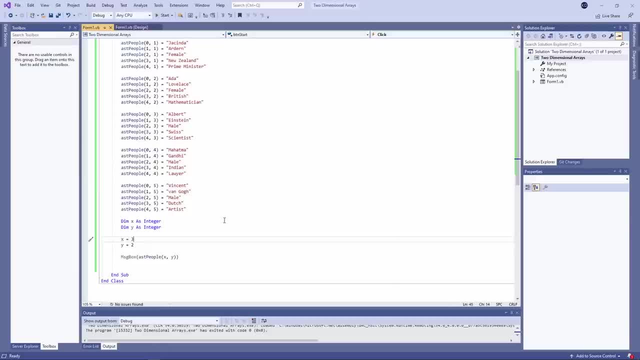 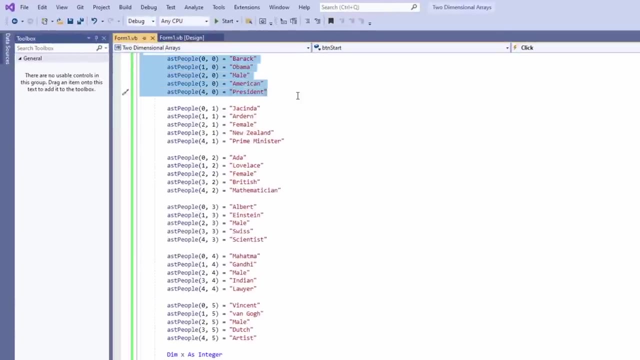 the real power of a two-dimensional array is realized when you combine it with looping constructs. Let's suppose I want to output all of the information about Barack Obama. Notice that with Barack Obama, it's the x dimension which is changing from 0 to 4,. 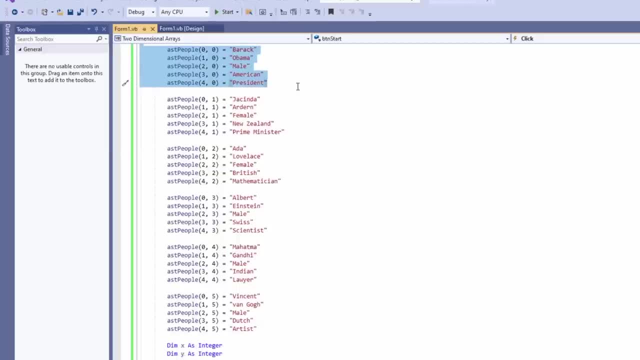 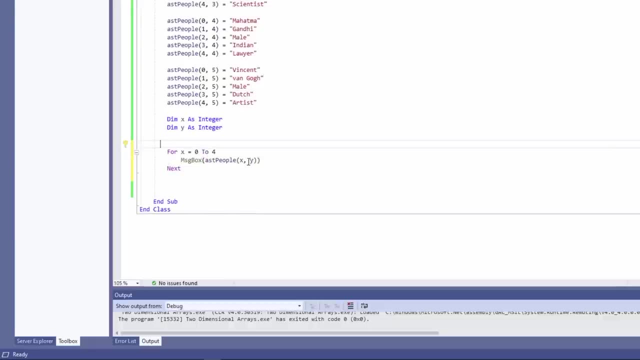 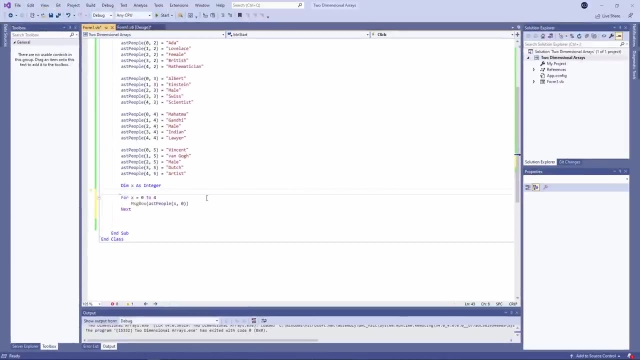 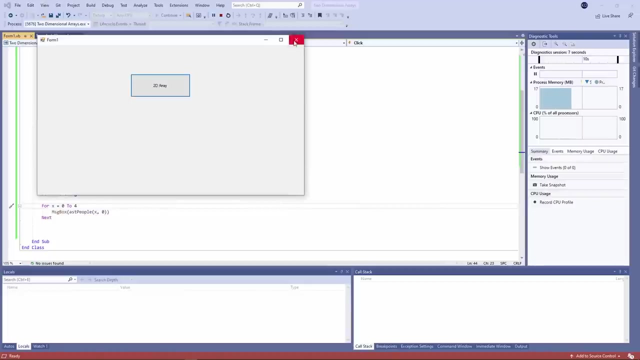 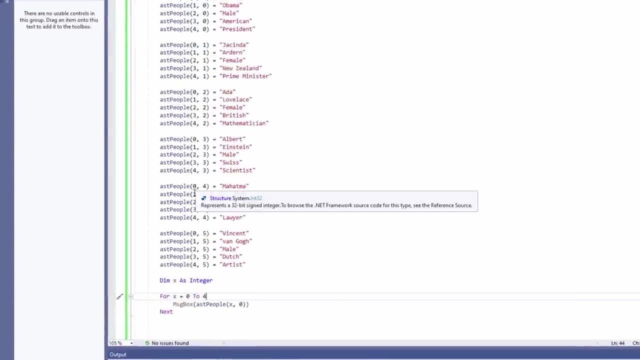 but the y dimension remains at 0.. I can do this. In fact, I don't even need the variable y. Suppose, instead, I want to output the details of Mahatma Gandhi. Again, it's the x value which varies, but the y value stays the same. 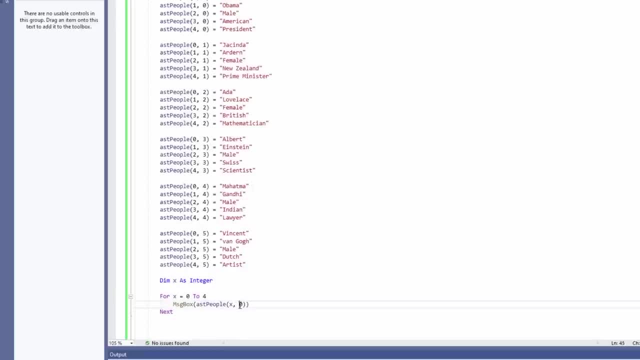 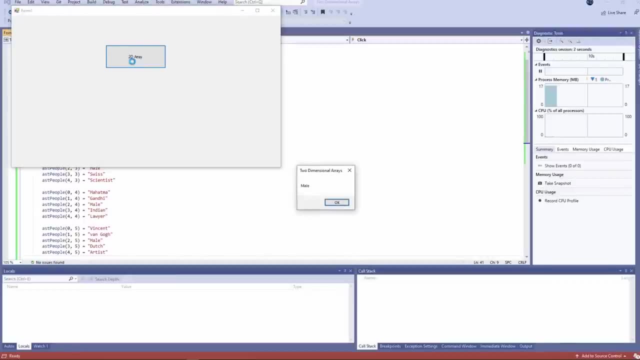 In this case, y remains at 4.. Now, let's say I want to output the details of Mahatma Gandhi. Notice that with Barack Obama, it's the x dimension which is changing from 0 to 4, but the y value stays the same. 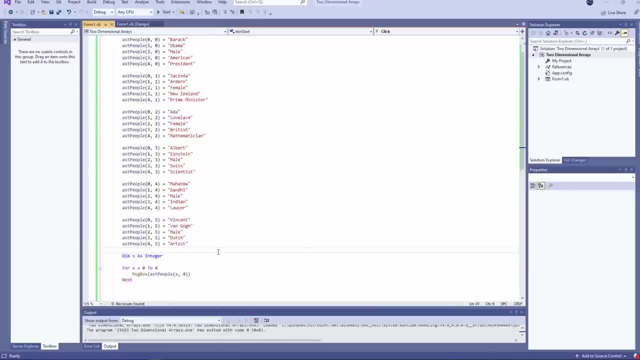 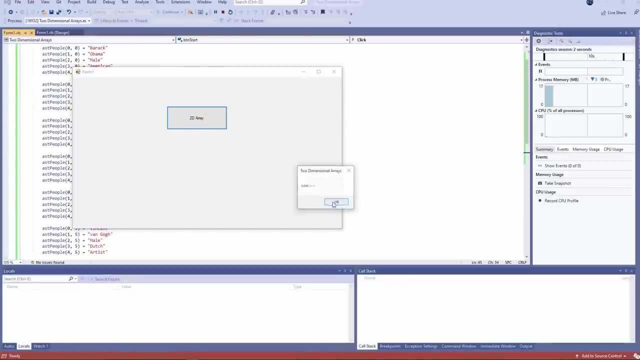 You should make sure that you're comfortable with this idea before you continue. Let's try Ada Lovelace. Ada Lovelace is in row number 2, so the value of y has to remain the same inside this loop. It has to be 2.. 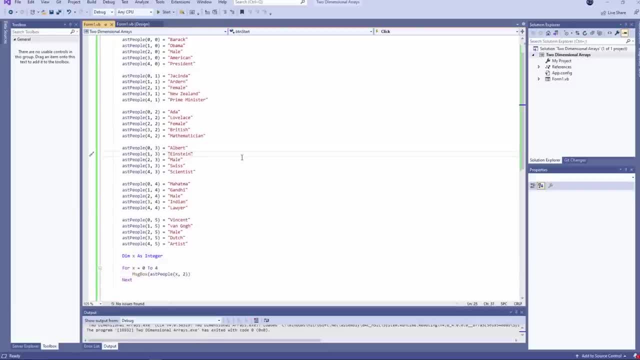 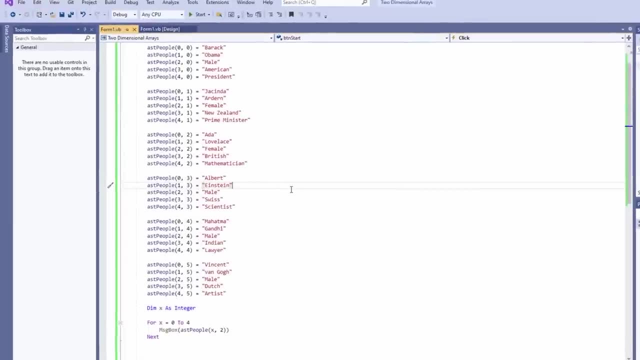 Alternatively, I might decide that I want to display all of the values in a particular column. For example, I might want to display all of the last names. If we examine the data, we can see that every last name has the same value of x. 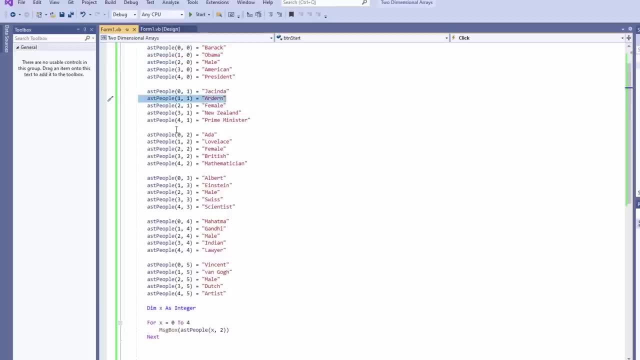 Obama is 10.. Ardern is 11., Lovelace 12., Einstein 13., Gandhi is 14. And Van Gogh is 15.. It's the value of y which is changing this time, So I could write my loop like this: 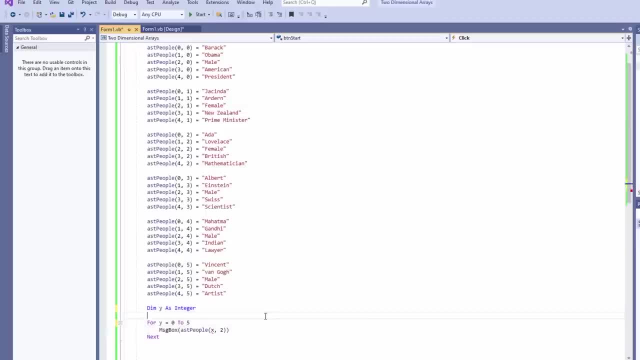 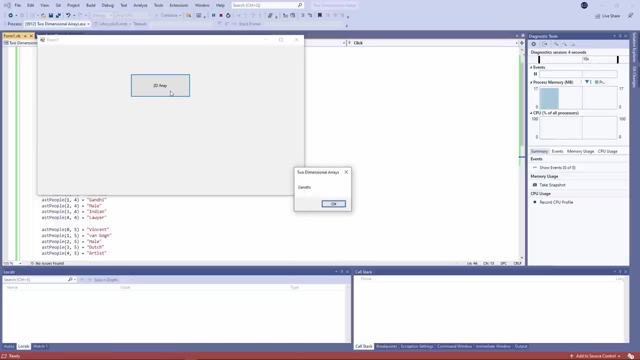 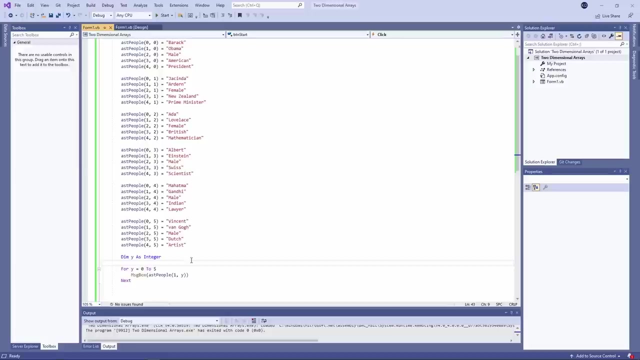 But notice that y varies from 0 to 5.. So this time it's the value of x which is remaining the same inside the loop, but y is the value that changes. Perhaps I want to display all of the nationalities. Looking at the code. 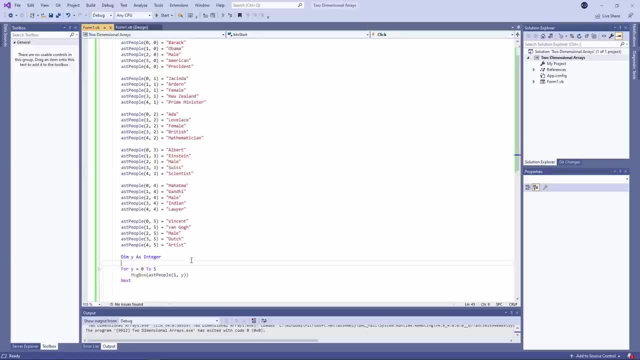 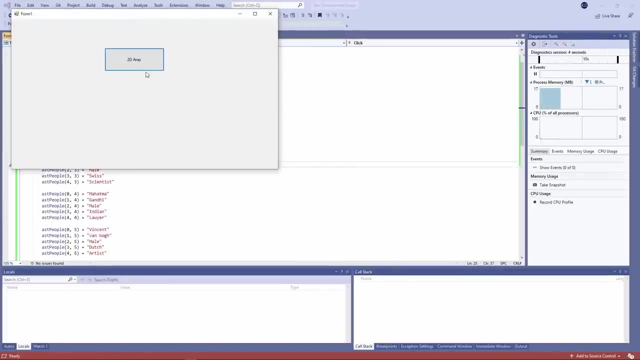 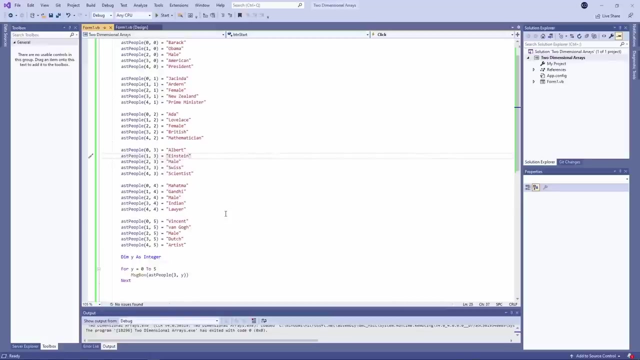 I can see that all of the nationalities have an x value of 3.. Again, you should make sure that you're comfortable with doing this before you proceed. In the next video, I'll show you how we can get all of the data out. 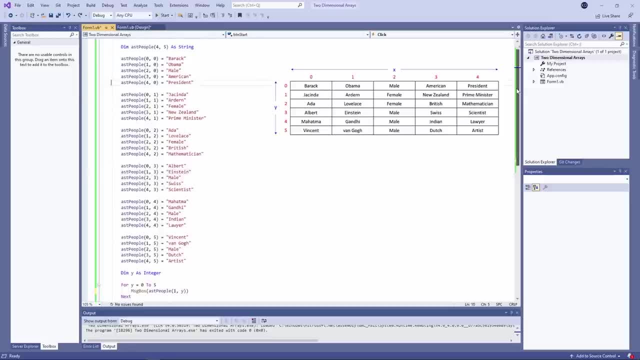 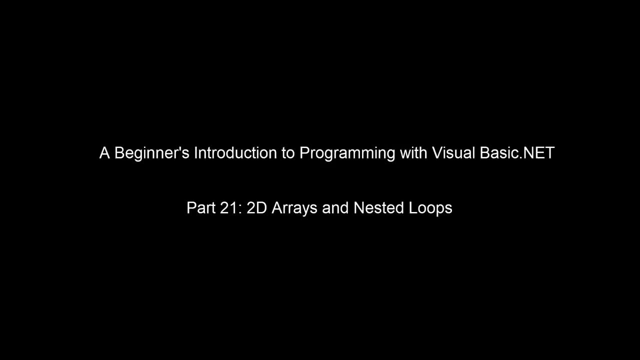 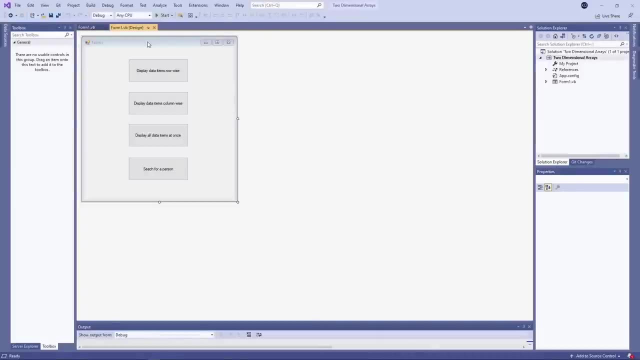 using nested loops. In this video, I'm going to show you how you can systematically visit each and every item in a two-dimensional array. As in the previous video, I recommend that you keep a sketch of your data handy to help you visualize what's going on. 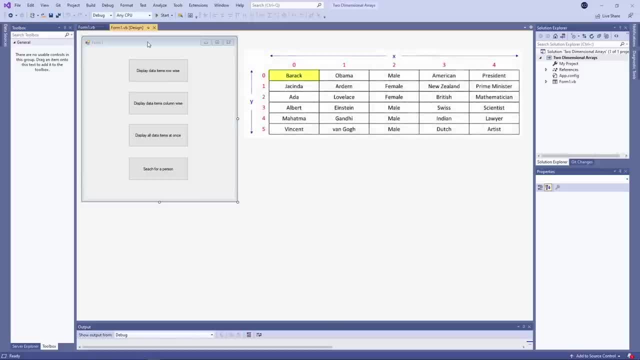 Here's a sketch of the data I'm working with. You may, for example, want to display all of the data items one at a time, row by row. like this, The data are being visited one whole row at a time, but as each row is visited, 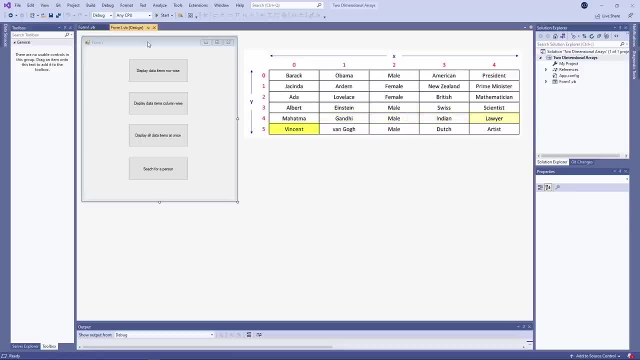 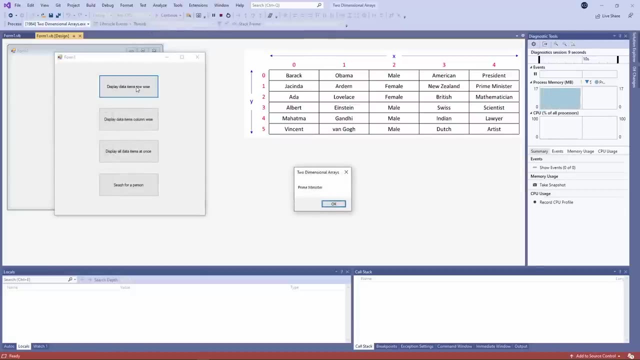 every column in the row is visited. We say that the data in the array are being visited row-wise. Here's what the output of a program that does this looks like. Alternatively, you might want to visit the data column-wise, like this: 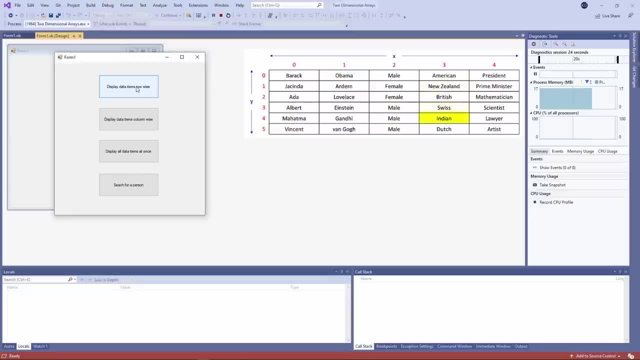 A program that does this deals with one complete column at a time, but as each column is visited, all of the rows in that column are visited, And here's what the output would look like. If you can systematically visit all of the data items in an array, 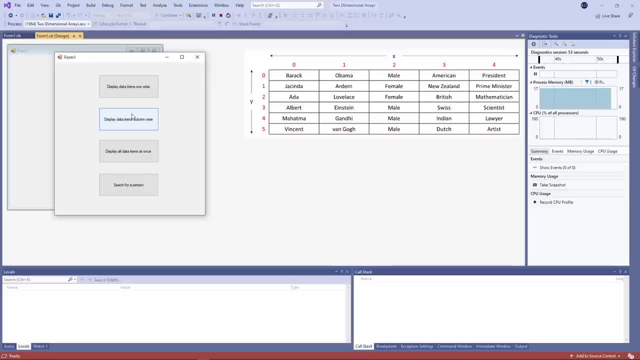 one way or another, then you can collect the data into a single output string, then output everything at once, like this. Systematically visiting the data also allows you to search for something in particular. For example, you could ask the user for a surname. 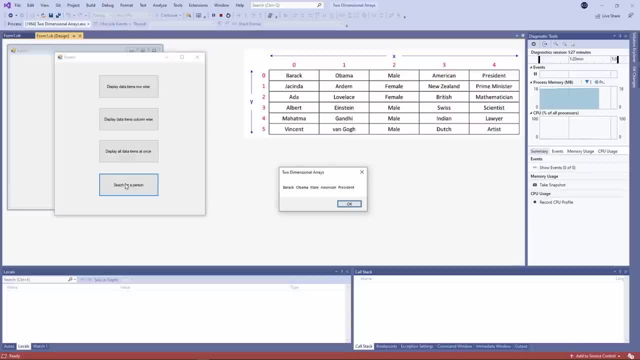 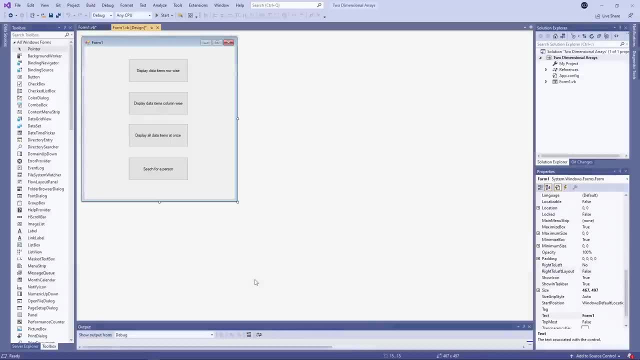 and then find all the details of that person like this. So let's take a look at some code and see how this can be done. I'll begin by writing some code to display the data row-wise. I've already declared the array. 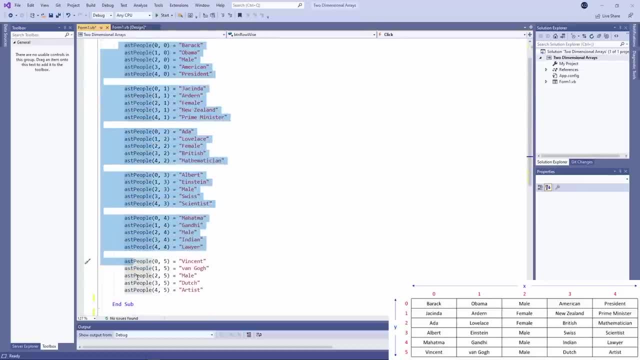 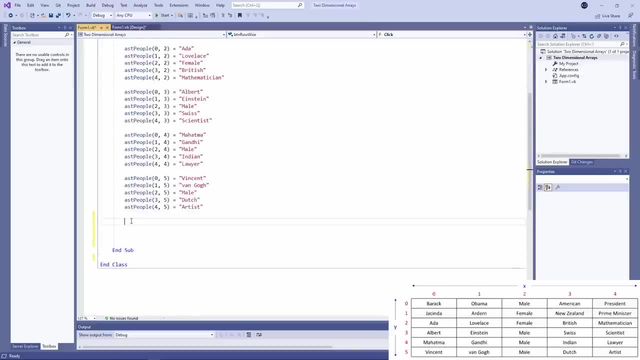 and I've already initialized all of the elements of the array. Just to speed things up, this is the same data which you saw in the previous video. I need two loop counters because I'm going to use nested for loops If I want to visit one row at a time. 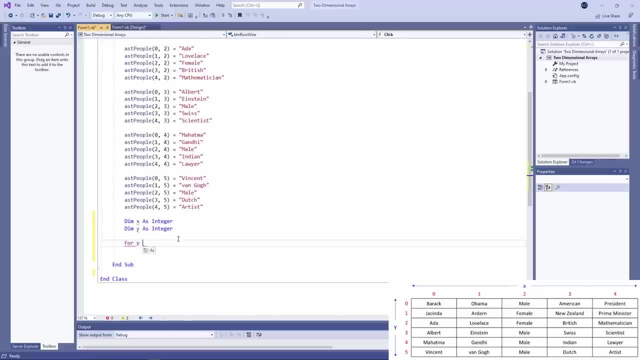 I need a for loop like this because each row is numbered from 0 to 5.. But while I'm visiting a particular row, I want to visit each column, and I can do it with a for loop like this: The columns are numbered from 0 to 4.. 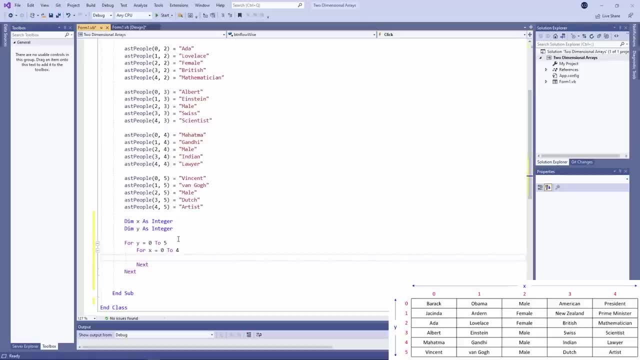 Think of it this way: For each pass of the outer loop, there will be several passes of the inner loop, And now I'm going to output a data item for each pass of the inner loop. Let's see what happens when we run the program. 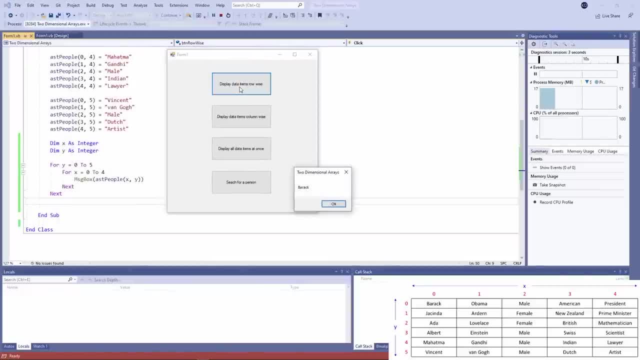 So I have a state at the left and I've already entered the delta. It's a default value. I'm going to enable this and I'll run the program And the data item is going to be the value I want to have. 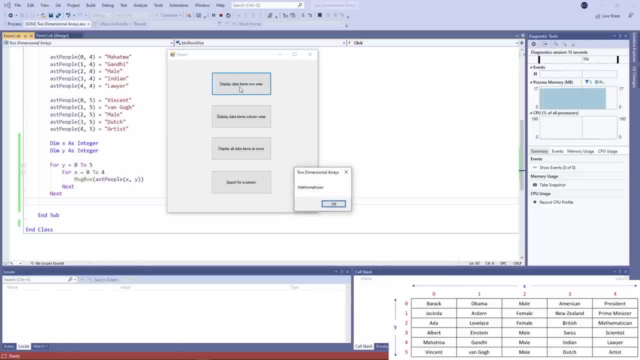 It will say that I have TimeLapse value for the space at my pass. But now let's do the same thing for my pass. Let's say we're running a functional query here And here the state data item is going to be: 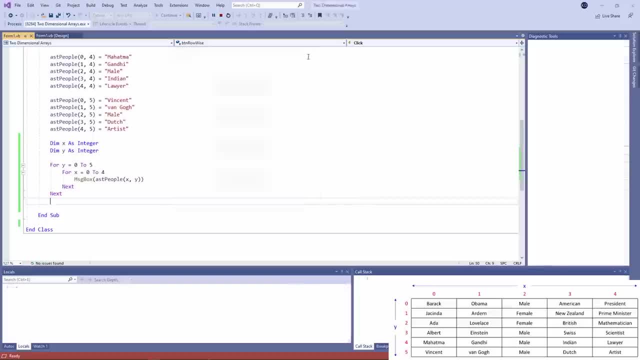 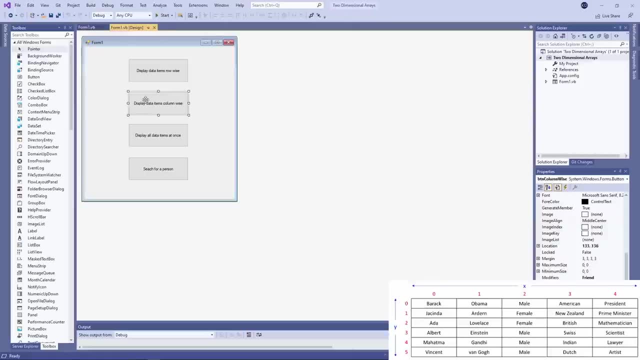 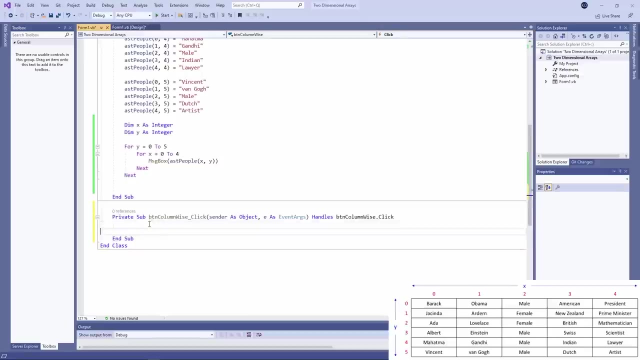 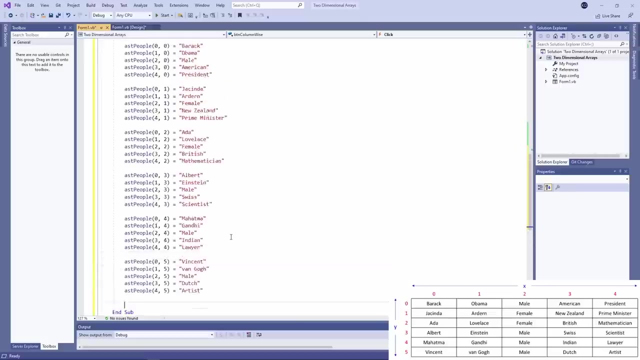 the value I want to have, and this will come back and I can enter the data item. Now let's display the data column. wise, I'm using a different button to run this program, but I'm going to copy and paste some code. It's the same code I used to. 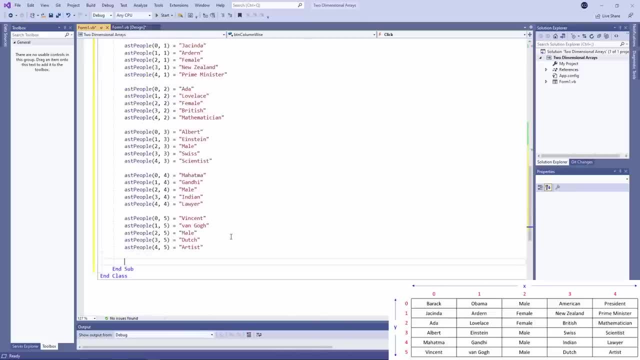 declare and initialize the array. In a later video I'll show you how two different procedures can share the same data. For now, we'll proceed like this: To visit the data column: wise, I'm going to use nested loops again, But this time I'm going to scan the columns primarily. so I'm going to scan. 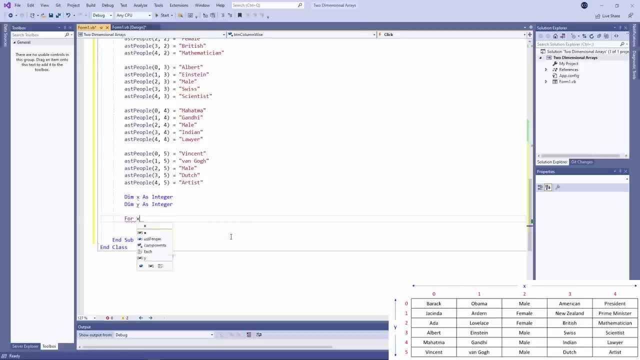 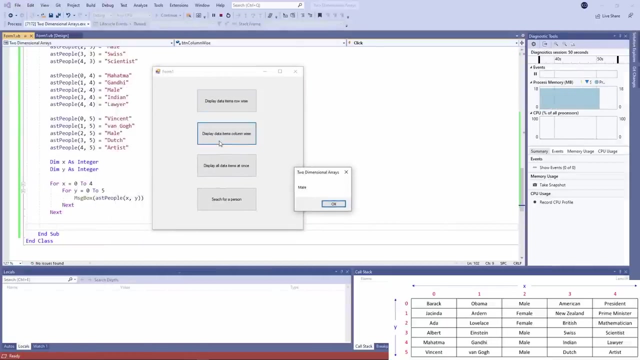 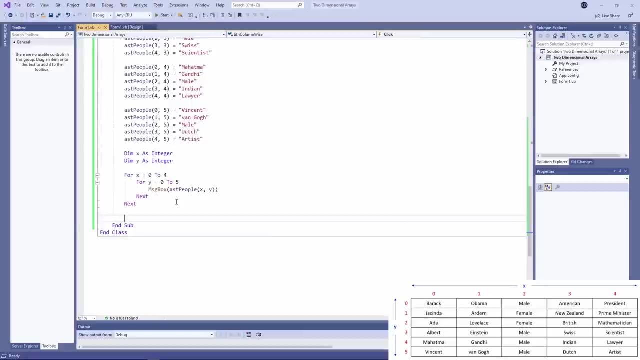 across the X dimension using my outer loop And as I visit each column. I'm going to visit each column And I need another message box, as before. Let's see how it looks this time- To display all of the data in a single message box. I need to decide whether I'm 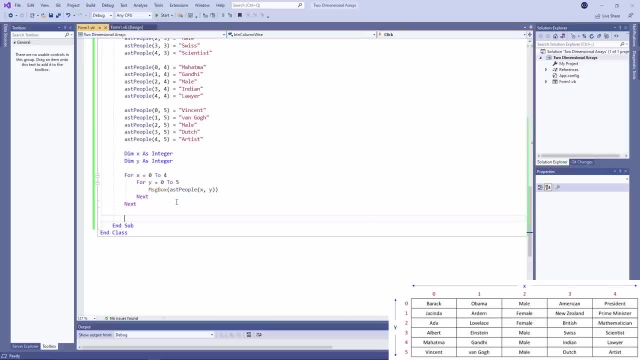 going to build the output string or not. To do this, I'm going to go to the data column. I'm putting in, aСТring in a row wise fashion, or a column wise fashion. I'm going to do it row wise. so, again, I'm going to borrow some code. 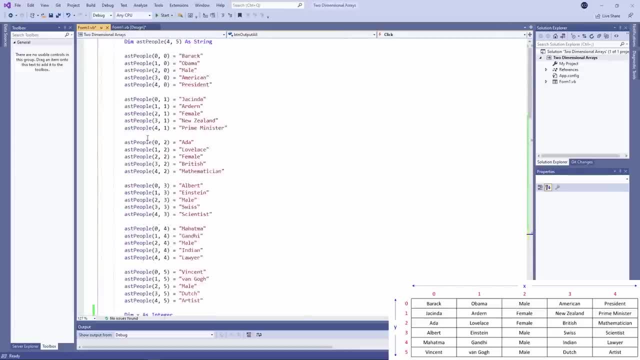 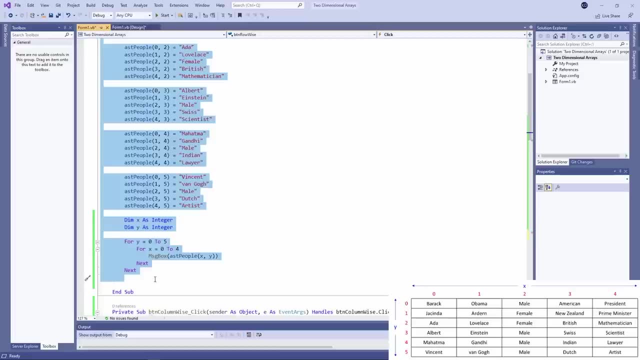 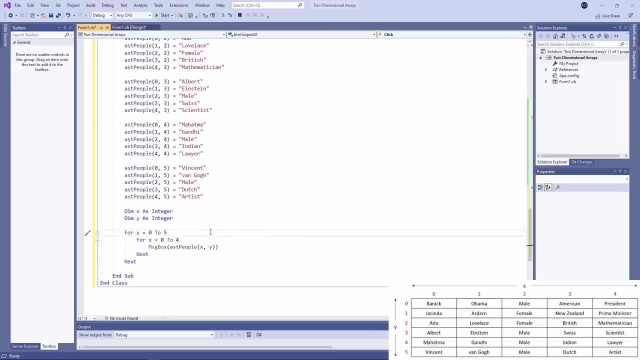 This is the code that displays the data items individually, but column wise. I need a string to collect the data into, And then, rather than displaying the stats, I'd like to execute a string classes argument, And then, rather than displaying the data items individually, but column wise, rugましょう. I'm going to do this over again and I need string variables to collect the data into. And then, rather than displaying the data item functions, I will enter a string variable. And then, rather than displaying the data items functions, I'm going to enter a string variables. 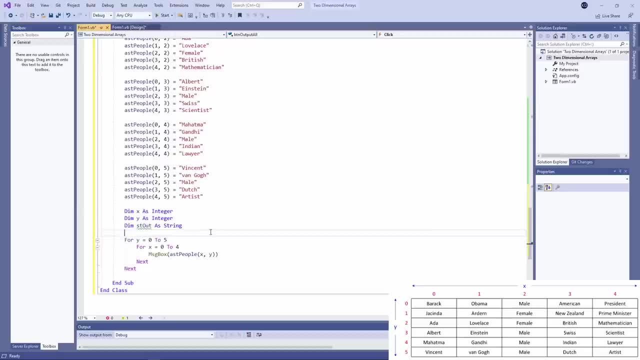 Soy vexem. the compositions for dataok amon: the Соic시면 is equal~~~. I will show you what we've added here. I've placed here the string variables in this form, laying a message box for each pass of the inner loop. 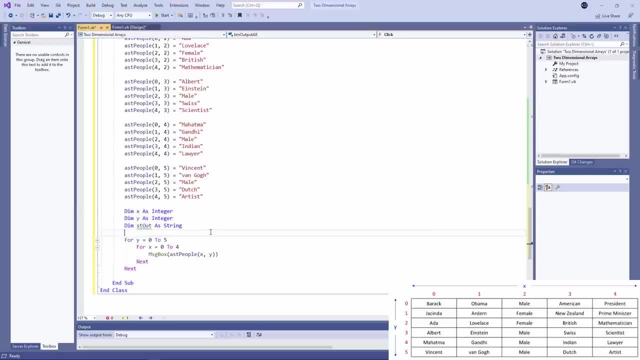 I'm going to concatenate some new data to the output string And between each data item I'd like a space Because I want each row of data to appear on a separate line within the message box I'm going to concatenate a VB new line character. 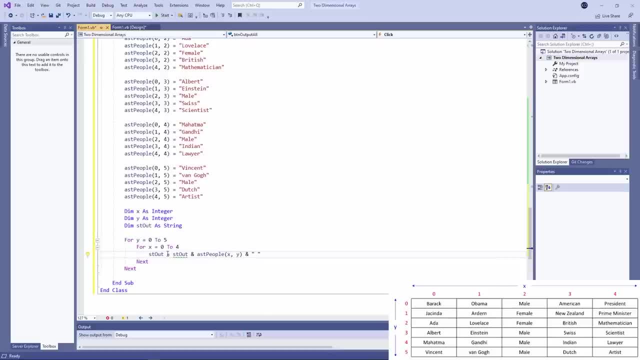 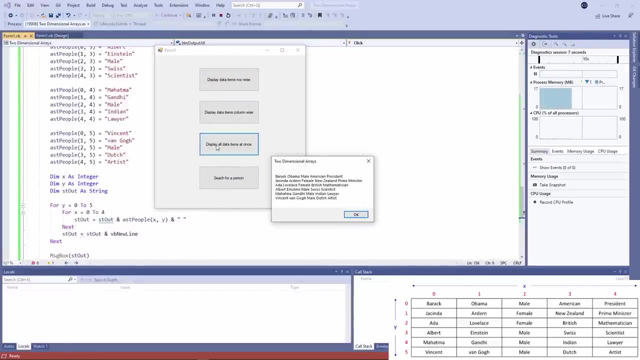 onto the output string, but only with each pass of the outer loop, And once the nested loops have both finished, I can do one output with a single message box. Let's see if it works. The final thing I want to show you is how we can search. 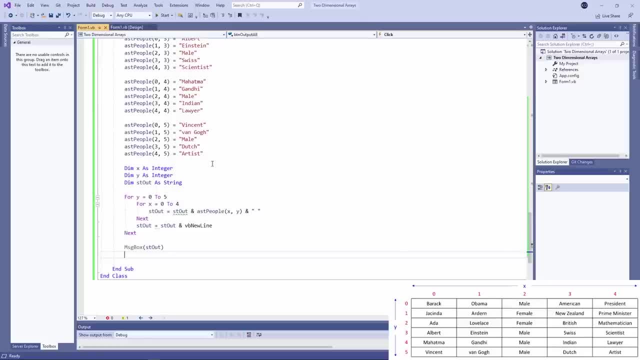 for the details of a particular person based on their surname, for example. I don't actually need nested loops to do this. I'm going to use the same technique which I showed you in the previous video. Let's start by declaring and initializing the array. 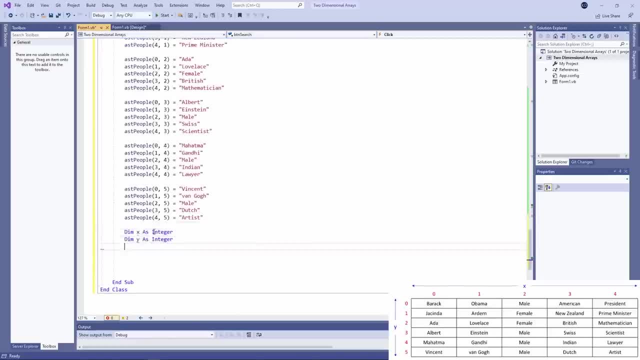 And I need some loop counters And I'm going to use a Boolean variable to record whether or not I found what I'm looking for. I'm going to initialize it as false, although, to be honest, I don't need to do that. 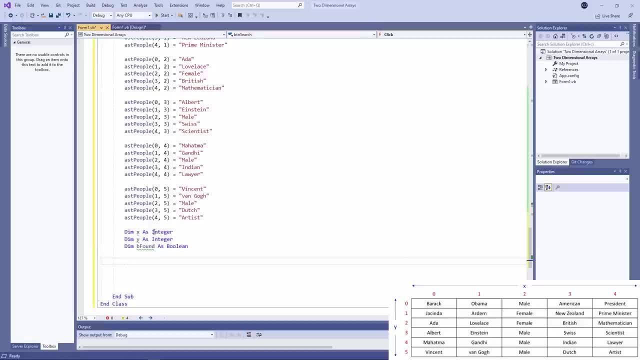 because immediately after it's been declared it will have a value of false. I just want my code to be explicit. I'll prompt the user for the target surname using an input box, just to keep things simple. So I'm going to need a variable to hold the target value. 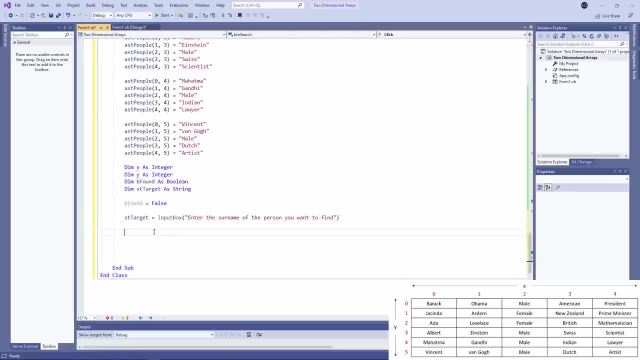 I know that the surnames are in column number one, so I'm going to write a loop to scan down the rows of column number one, only testing each value. as I go, Notice how I've hard-coded the value of the X dimension here. 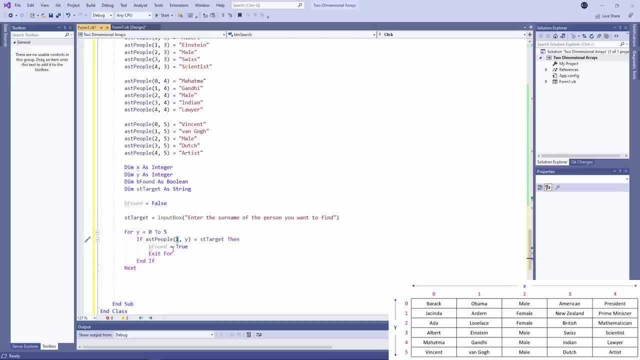 I'm always looking at column number one As I scan down the column. if the data item which I'm looking at matches the target, then I'll set my Boolean variable to false. I'll also set my Boolean variable to be equal to true. 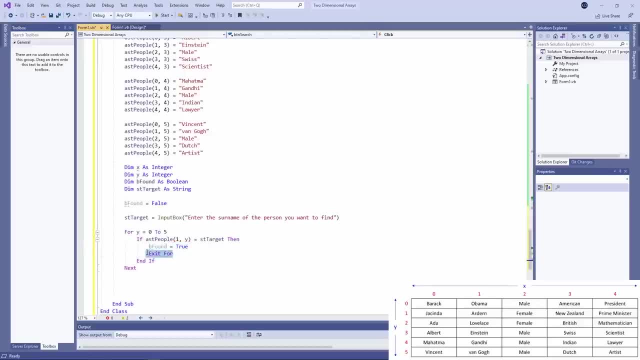 and I can force an exit from this for loop. By the time I've dropped out of the loop, I know whether or not I've found what I'm looking for. If I have, then I can retrieve the rest of the data for that particular person. 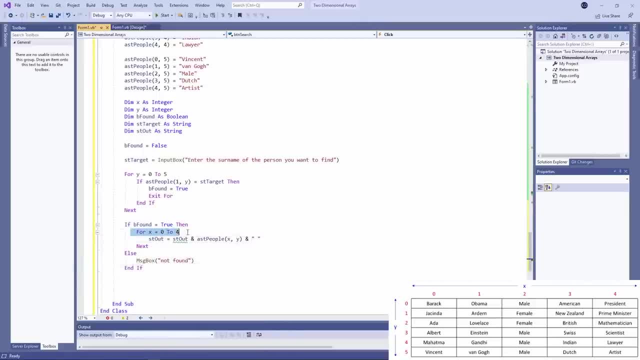 Notice. this time I'm scanning across the row, The value of Y will be whatever it was when the first for loop came to an end, so I know this loop is looking at the correct row. If be found was equal to false, then we simply display a message saying: 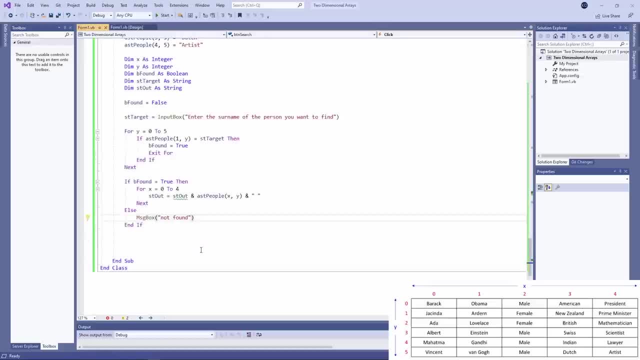 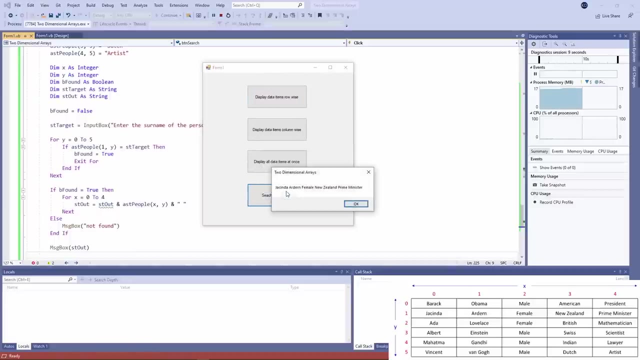 that we can't find what the user was looking for. There's one final thing we need to add to this code. Let's see it in action. That seems to be working fine And, just to be sure, let's look for somebody who isn't in the array. 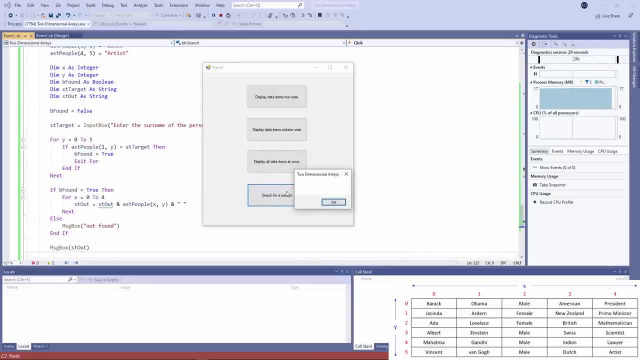 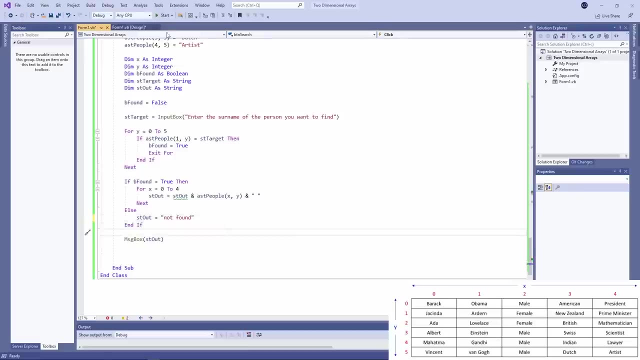 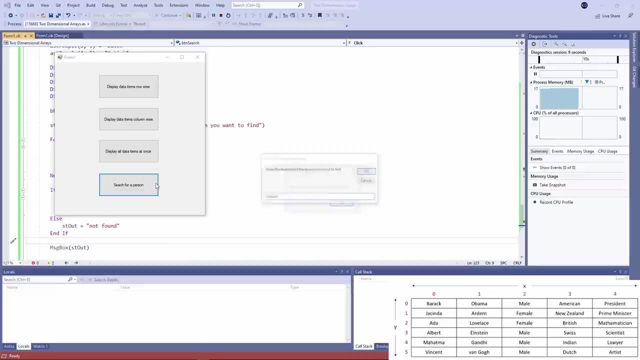 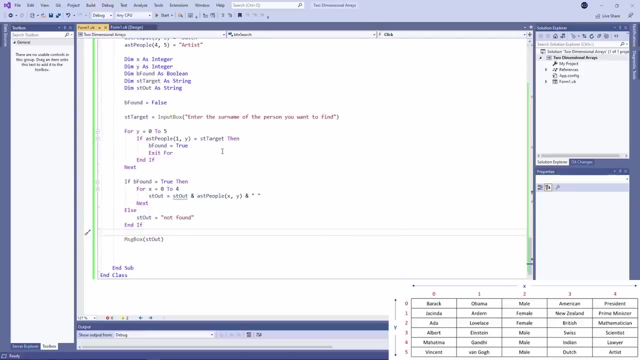 That looks okay as well. Having said that, we have an additional message box here, which is rather untidy. Let's put this right. That's better. You should try writing some of these programs yourself. Perhaps you could display the data column-wise.